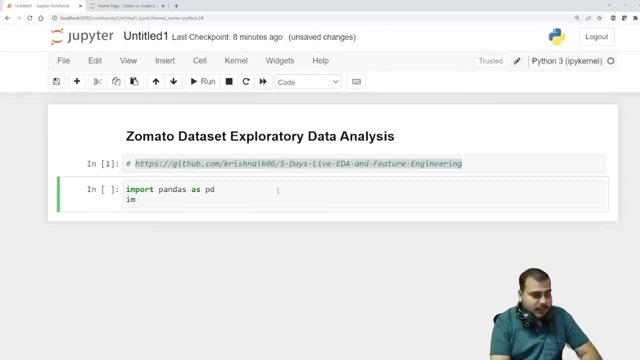 Import pandas as pd, Import numpy as np, Import matplotlibpyplot as plt. And one more library that I'm going to use is something called a seaborn, And finally we will be using matplotlib inline so that the images or any visualization gets displayed here itself. I'll keep it restricted. 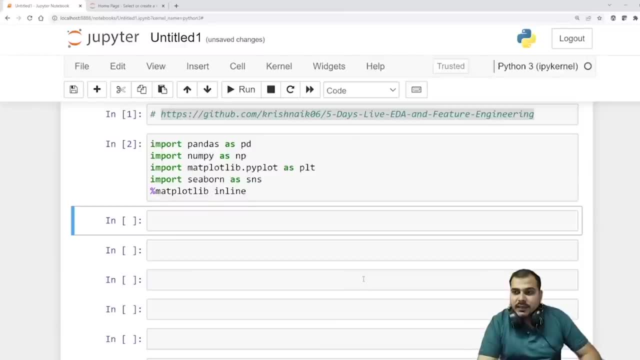 to all these things and understand the main thing. The main thing is that whenever you are performing EDA, that is, exploratory data analysis- you really need to think about the data, what the data is basically seeing or telling you right. That is most important. So whenever you have a specific 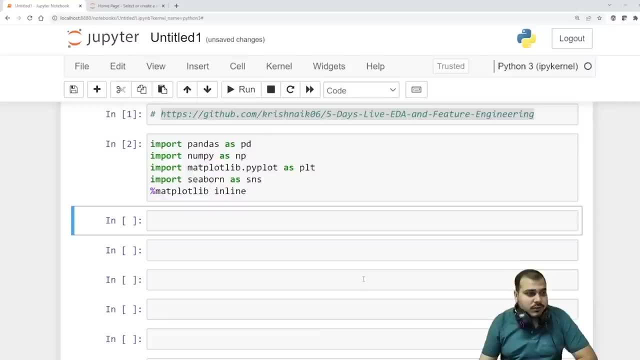 data set, some basic information. definitely you'll be able to capture it. So what we are going to do over here is that till now, we have actually imported all the libraries. Now let's go ahead and first of all, let's download the dataset from here. So here you can see that there is a dataset. 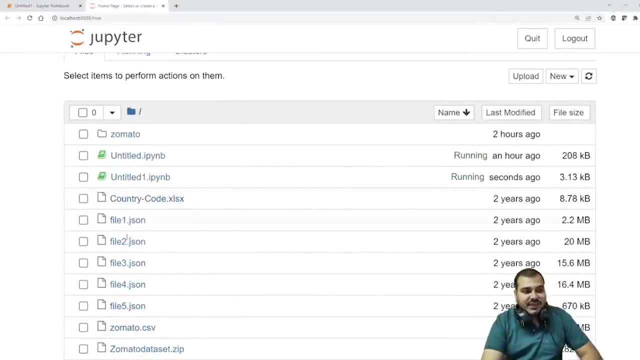 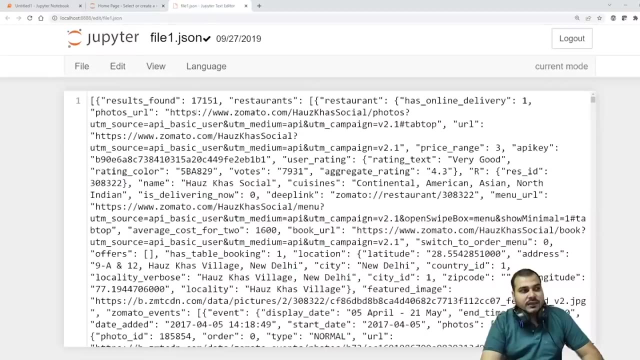 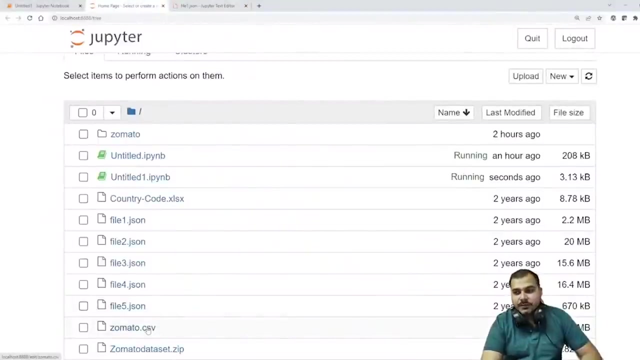 called as zomatocsv- countrycodexlx And there are multiple JSON file. Now why this JSON file was given, guys? Because this JSON file is in the form of this JSON format. Okay, This format has been converted already into zomatocsv. Now how it has been converted. you really need to write a. 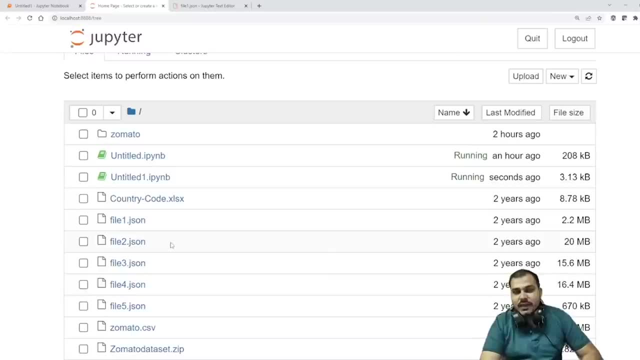 Python script to convert this. We will not see this right now but in the later stages I will also show you how we can convert this JSON file into zomatocsv. That part we will do it in the later stages, in the upcoming classes. But today we have one xlx file, one csv file. We'll try to combine. 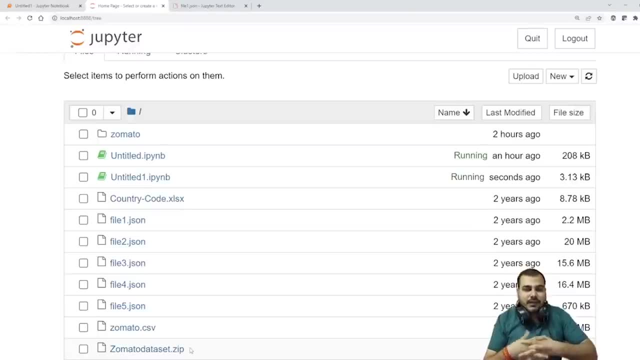 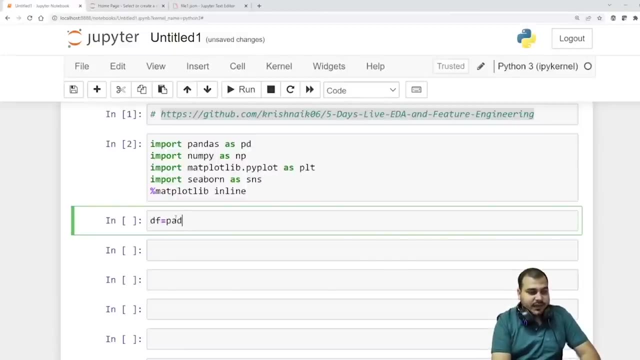 this file. also, We'll try to see what all information you have in this specific file. So let's start here. So first of all, as usual, I'll just write df- my dataset, and I'll write pdread underscore, csv, And I will read the dataset, which is zomatocsv. Now, when you are actually importing the zomatocsv, 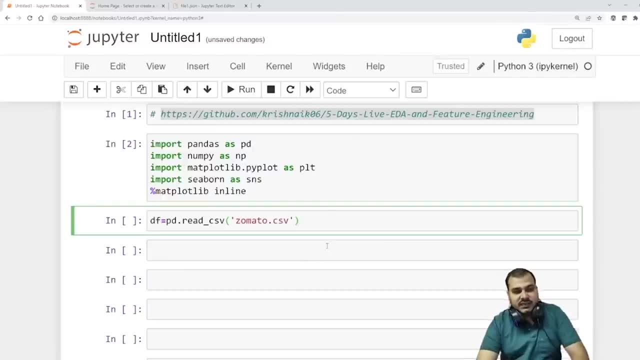 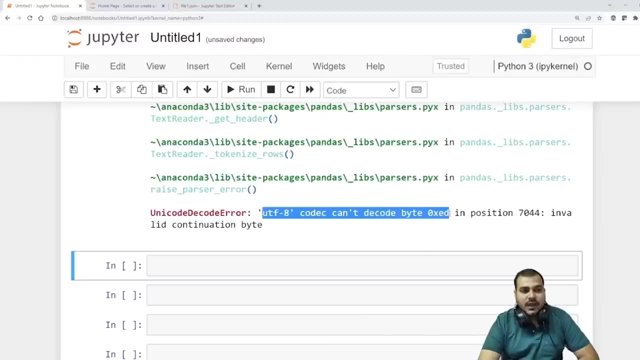 the other thing that you need to see is over here is that if I just execute it like this, so here I will be getting some errors. It says that UTF-8 codec can't decode byte 0xed in position 044.. Whenever you get this kind of error, always remember that you have to use some kind of encoding. 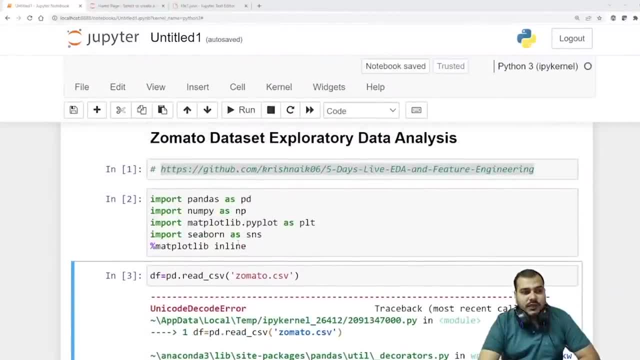 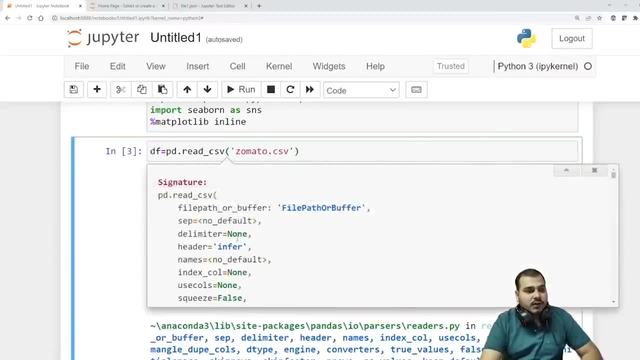 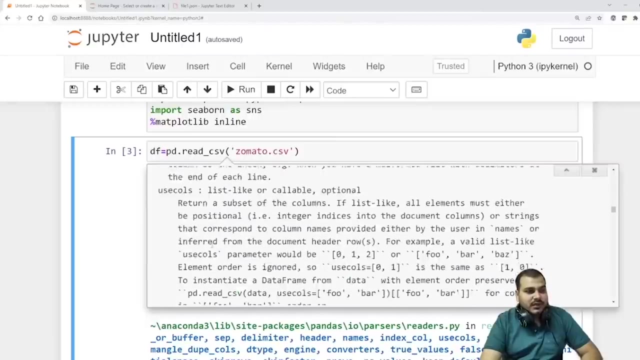 format Now, in this case, what encoding you will be using. if you probably go and see in read underscore csv and press shift tab here you will be able to see a lot of options. So one options I'll see over here: encoding- encoding somewhere it will be, or you can see the parameters You can. 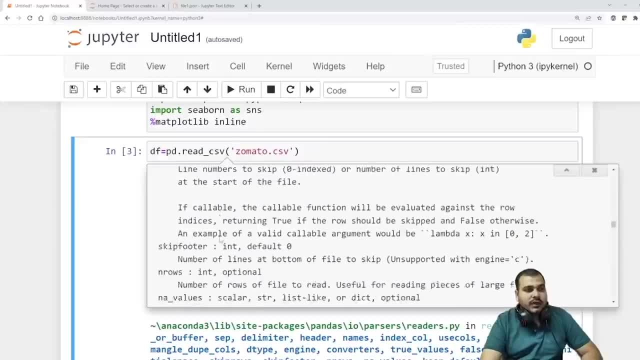 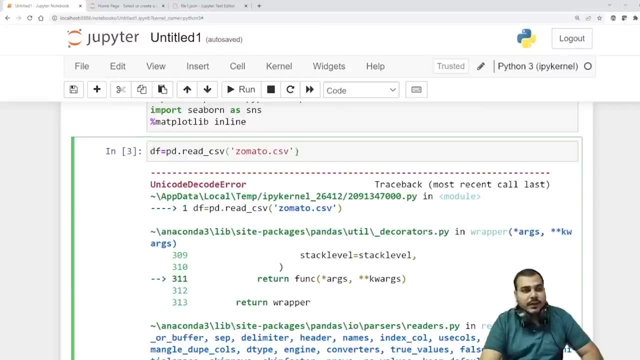 search the parameters over here with respect to encoding What you need to put over there, but understand, you need to have UTF-8 encoding. So for this, what I'm going to do, I'm going to use an encoding. And remember, this encoding I did not understand, I did not use directly in. 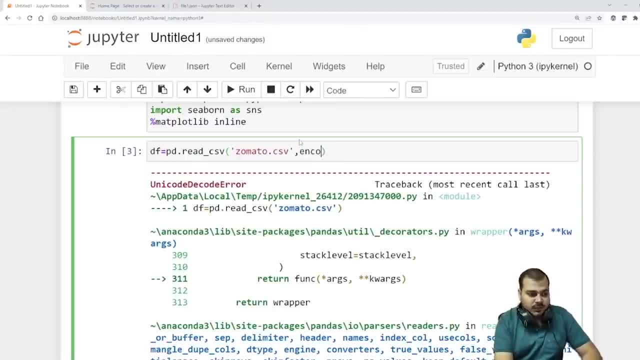 the first instance, but I used, after exploring some of the things over here with respect to the kind of error. So, encoding: here I'm going to use Latin dash one. You have different, different encodings, Again UTF-8 encoding. you can just check out the documentation over there. So I'm 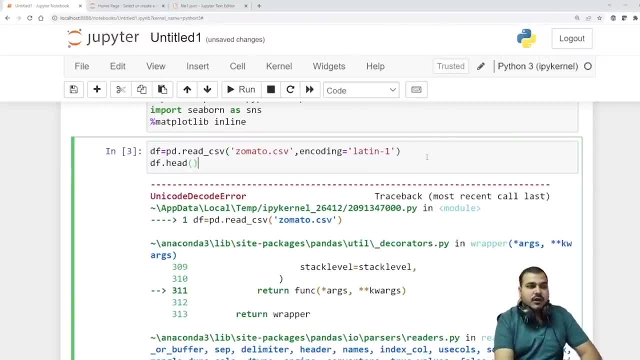 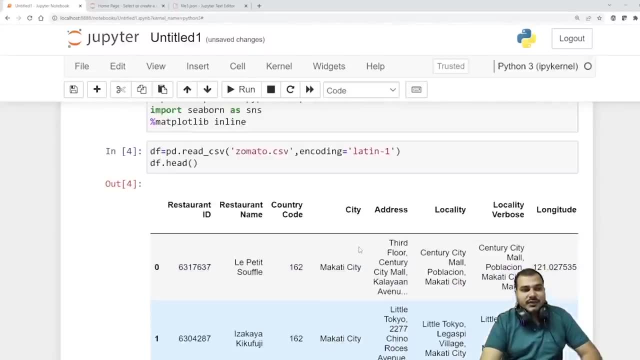 just going to use Latin one And then I'm going to basically say: DF, dot head. Now if you go and see over here, these are all my data sets that are available over here. It's a huge data set with respect to the number of 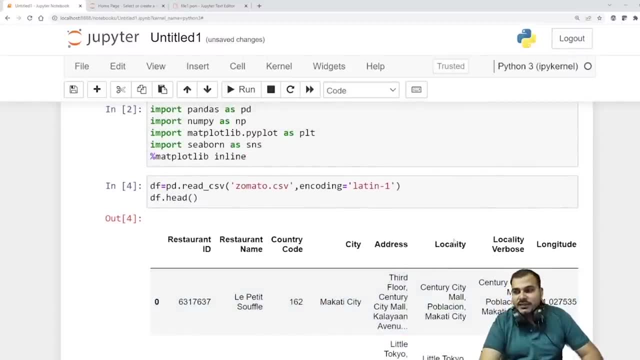 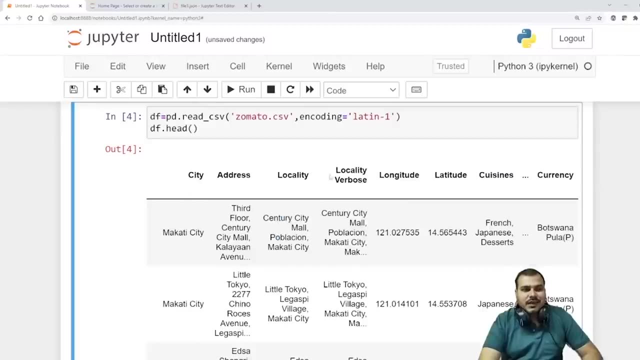 columns, but understand, this is how we read the data set over here And, with respect to this, you can check it out, all the features and all, but now one thing that we have done is that we have imported all the data set over here in my, inside my DF. Let's go to the next step now. So 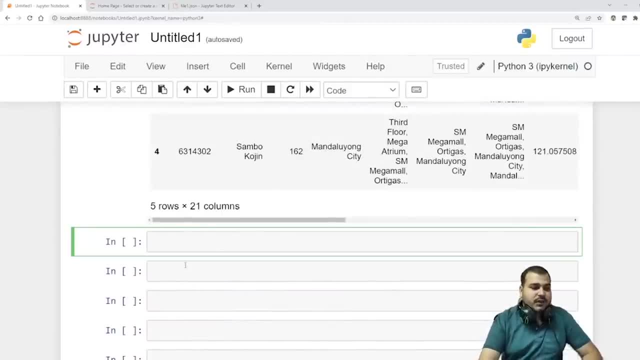 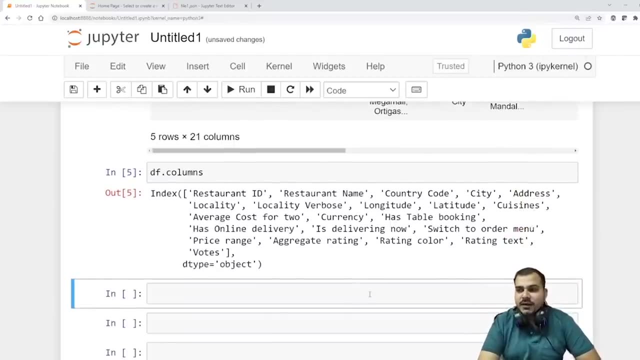 this is my data set over here. that is present. Now the next step, what I'm actually going to do. I'm just going to see what all columns I have inside my data set. So now this is in the basic EDA part. So over here you have restaurant ID. 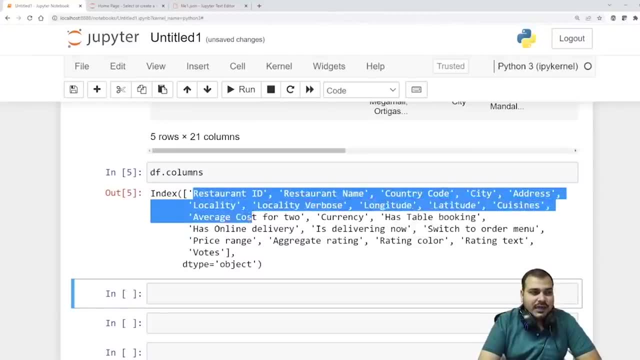 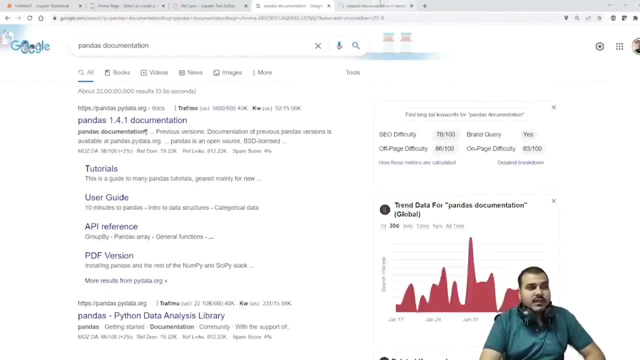 restaurant name, country code, city address, locality, locality, verbose, longitude, latitude, questions, average cost for two currency And many more features are actually present over here. Just go and search for Pandas documentation Anytime you have any kind of queries with respect. 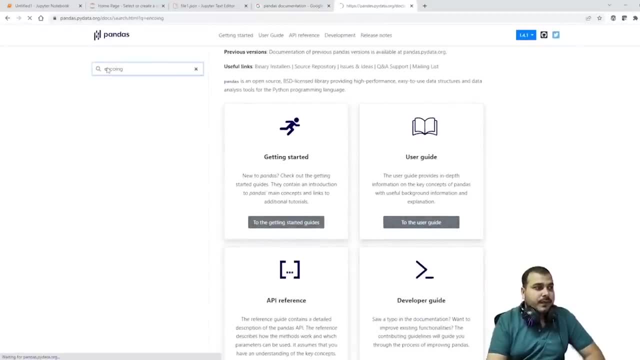 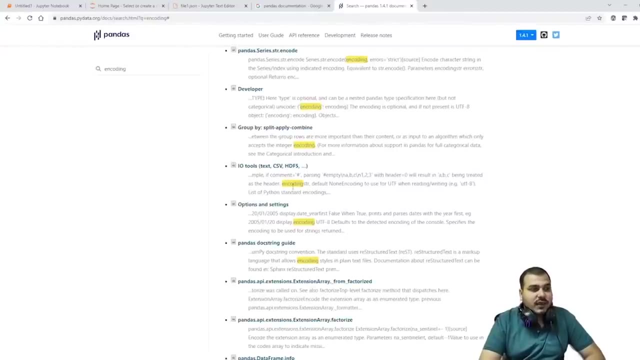 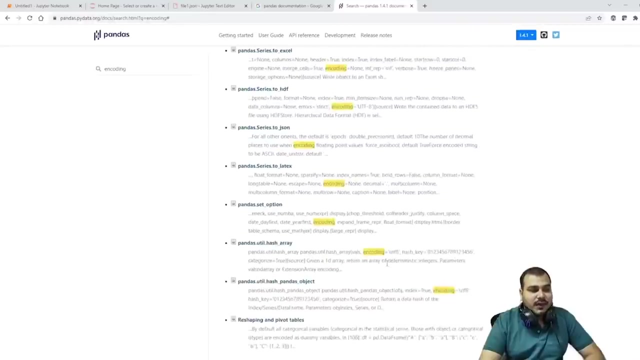 you have to write and all, you can just directly search for it. you can search from here. when you search from here, anyhow, anywhere you will be able to see it- why encoding is used, why utf-8 is used. so from here you have to explore it over. here you can see encoding as none right, why it is basically. 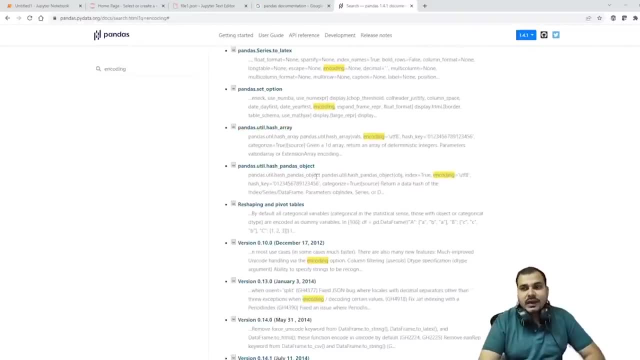 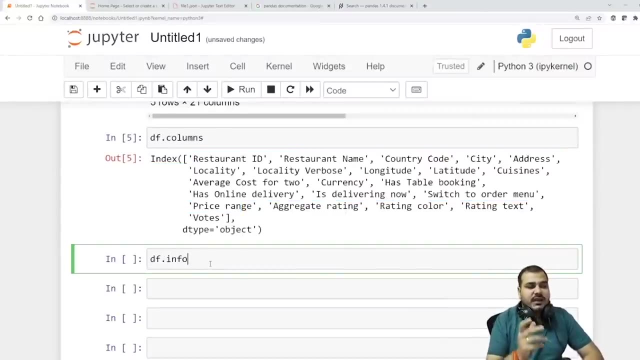 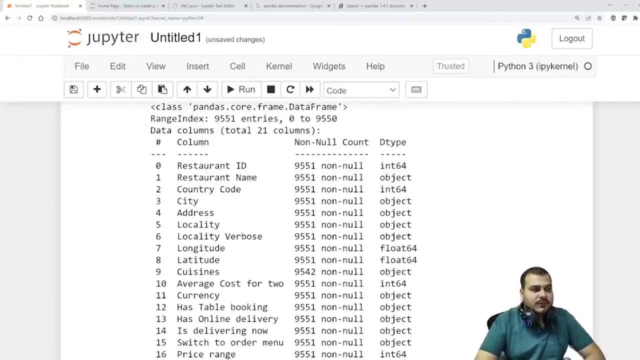 used. just click on this. try to understand that specific keyword. now the next thing over here- let's go ahead and let's see one more way of understanding about the data set is like dfinfo. if you write dfinfo here, you will be able to see what all columns are there, whether this column is. 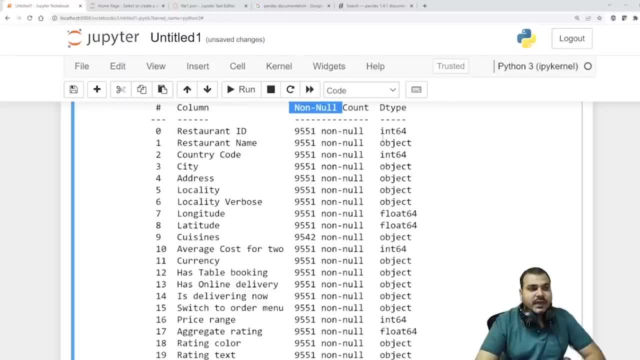 non-null or null, whether it is. what is the data type of this? here you can see int64. int64 is specifically for integer variables. whenever you see objects in pandas in data frame, object basically means strings. it can. it can also mean like it is maybe a categorical variable. it may be a text variable, it can be anything over here. so here: 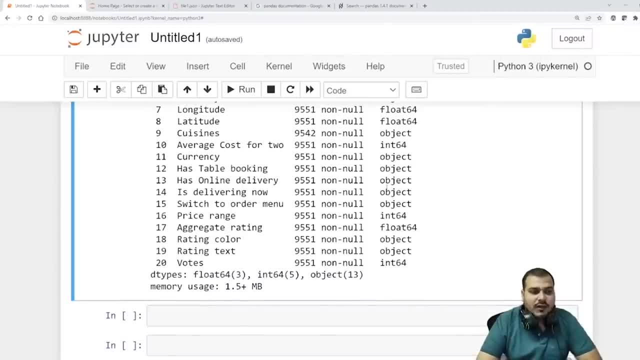 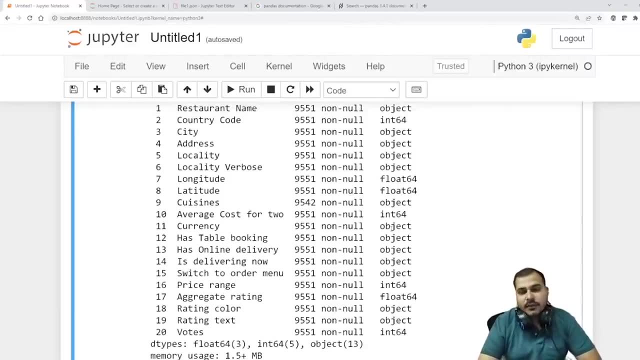 you can basically see all those things. you also have float. you have objects, objects wherever objects is there. just consider that. it may be a categorical variable, it may be an integer variable, it may be a text data. initially, always you do this, you try to find out what are the columns. 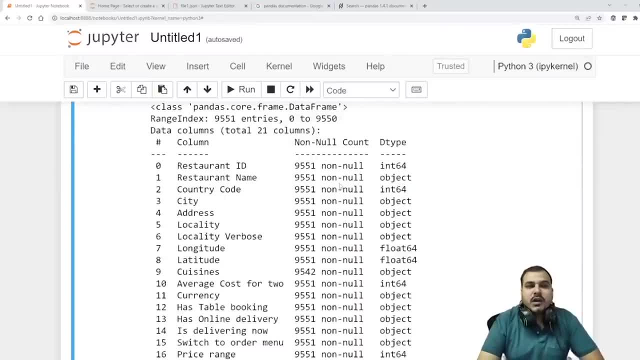 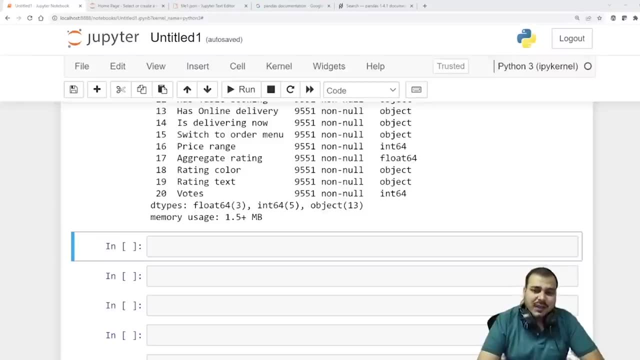 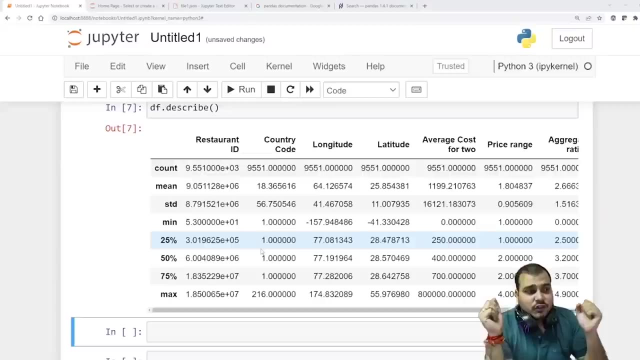 try to find out. what are the important information about the columns with respect to the data type. now coming to the next step. now let's see what we can further do, what, what actual information we can actually come up with this. there is also an inbuilt keyword which is called as describe. so this is a basic inbuilt function. 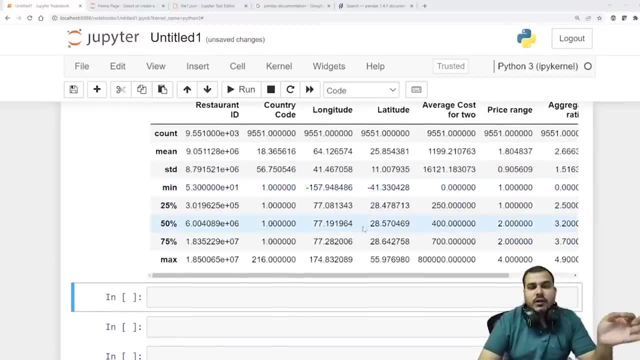 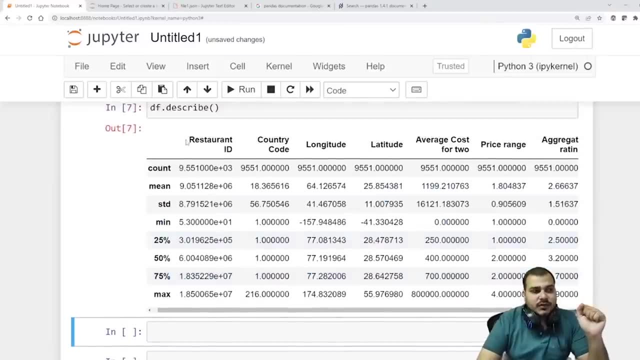 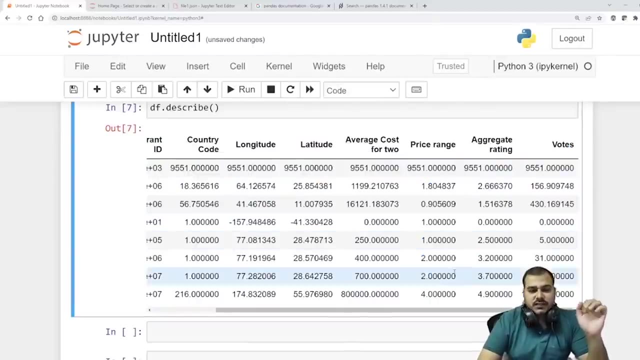 which is called a describe, which will actually help you to find out all this specific information. now, one key, important information from this is that here you will be able to see that all the features that are basically taken inside this describe function right. these are only integer features. you will not be able to find out any categorical features, any text. 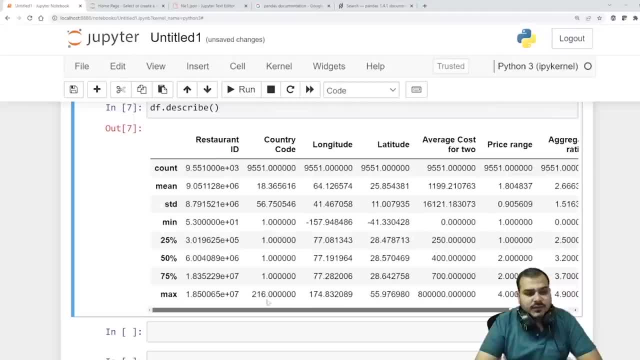 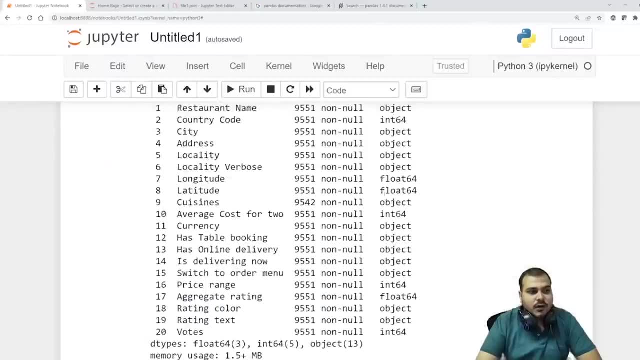 features, any object features over there. so here definitely see with respect to any feature that you see, restaurant id. if i go and see restaurant id it is int 64. if i go and see country code it is basically, uh, int 64. if i go ahead with longitude it is always float or int 64. see over here. 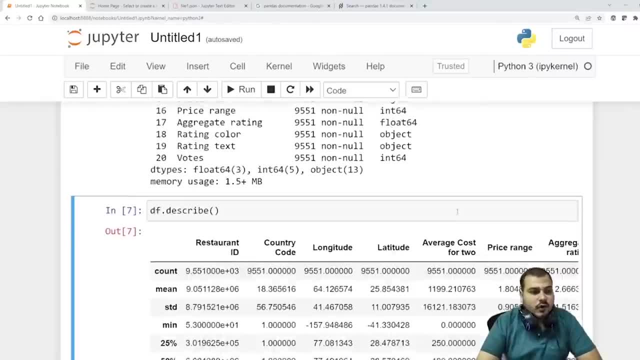 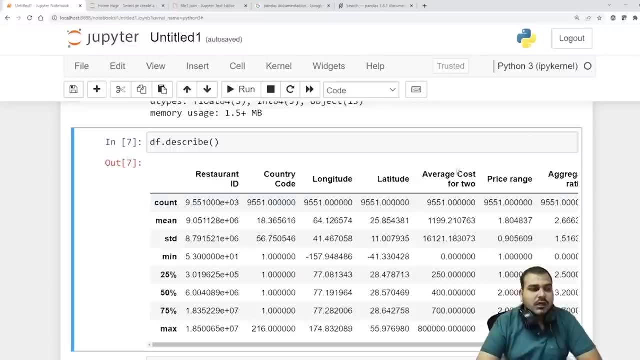 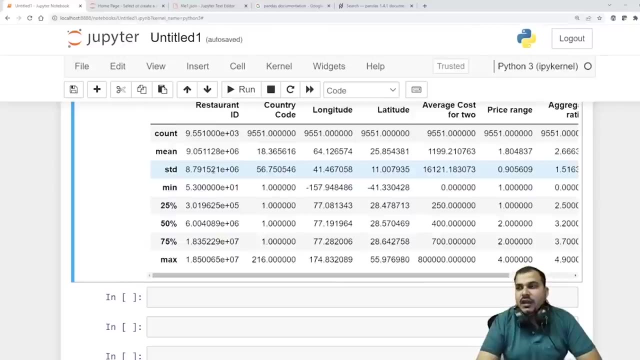 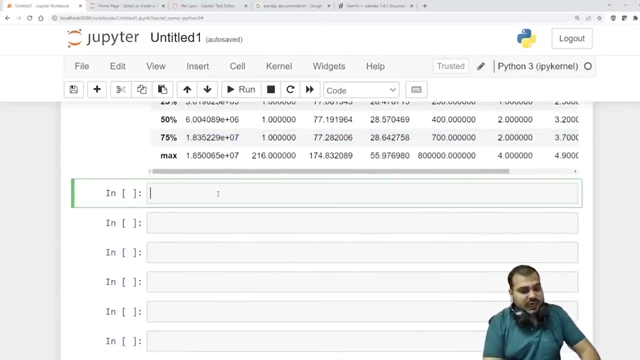 longitude, latitude, float 64. so all these values that you are actually able to see over here. this is completely based on your integer variables, because whatever thing you are doing, like count mean, standard deviation mean you have to basically find it out in the integer and numerical variables. now i'll just give you a basic information in data analysis. the first: 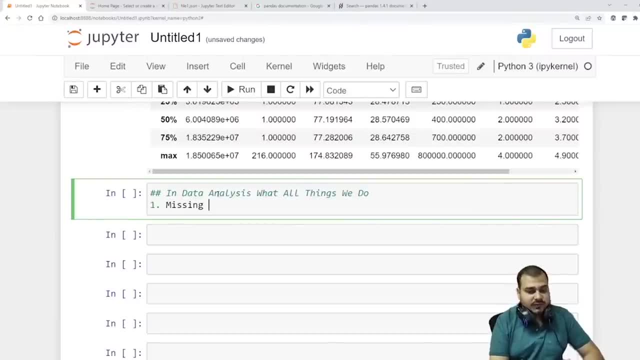 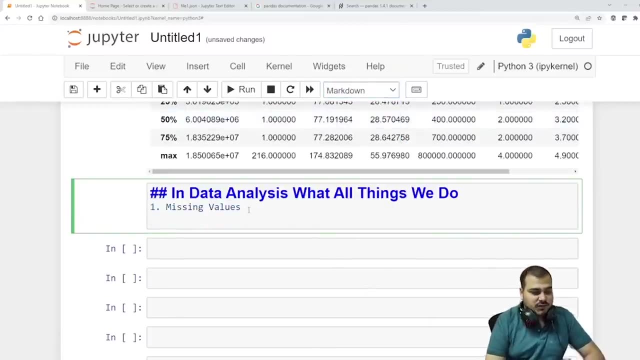 thing that i would like to find out is that we'll try to find out missing values first of all. always, it is very much important in our data set. do we have missing values? The second thing that we may probably do: check explore about the numerical variables. 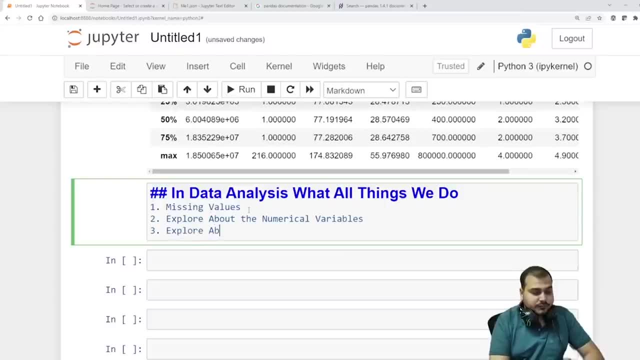 Third, I would like to definitely explore about categorical variables. These are some basic things because I need to know that how many categories are there? how many numerical variables are there? The fourth major thing that we probably do is that finding relationship between features. 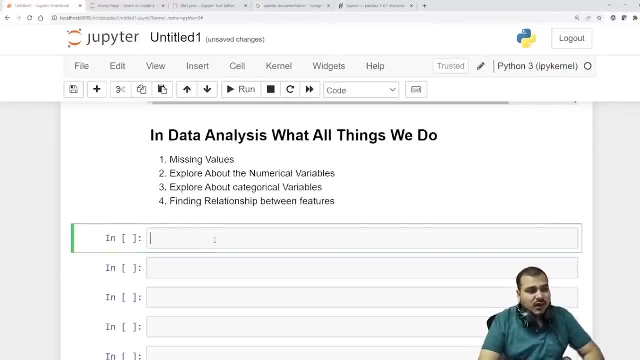 Let's go ahead and try to find out what are the missing values. In order to find out the missing values, you can basically write dfisNullsum. So if I go and search over here, you will be able to see that with respect to every feature. 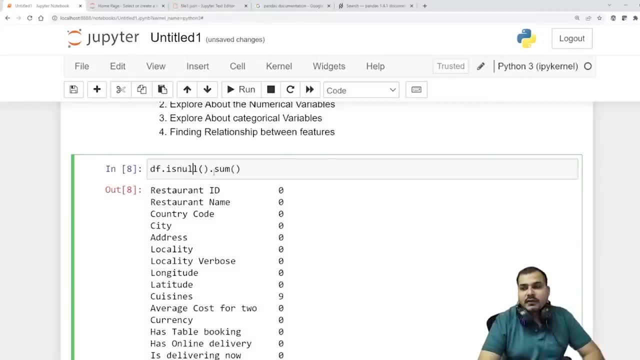 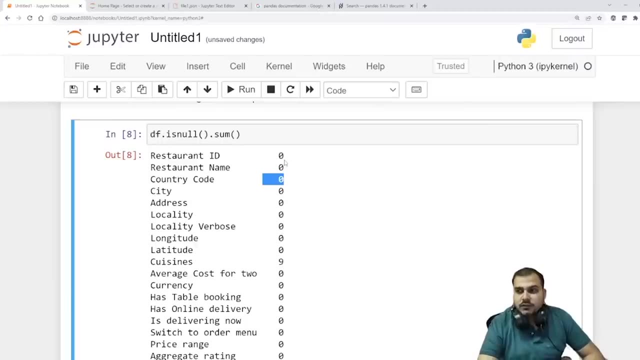 it is just saying that how many features are basically having null value? Here you can see that 00 is there, 0 is there, 0 is there. What about duplicates? I'll talk about duplicates also. So here you can see in city: 0 is there. 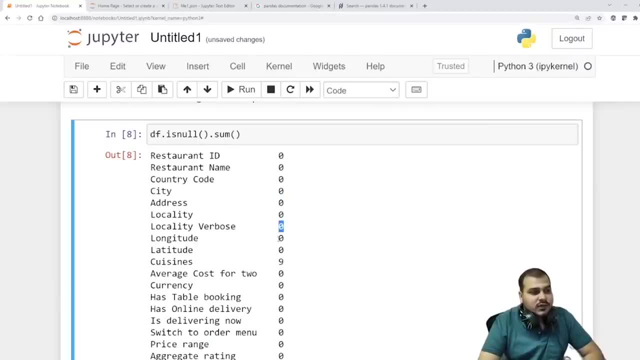 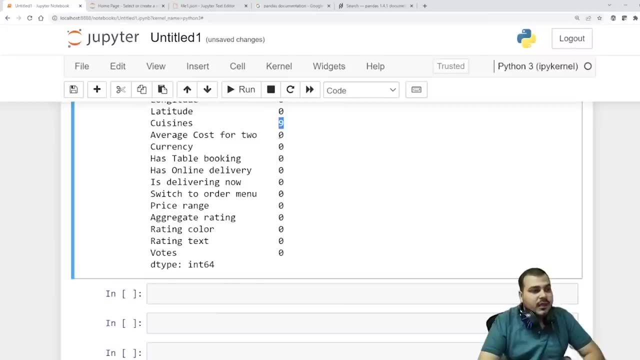 Address: 0 is there. locality 0 is there. locality verbose: 0 is there. longitude latitude: 0 is there, But in cosines you can see that there are 9 missing values, Remaining all you have 0 missing values. 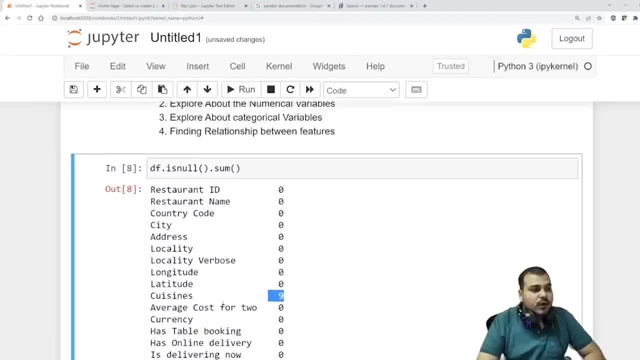 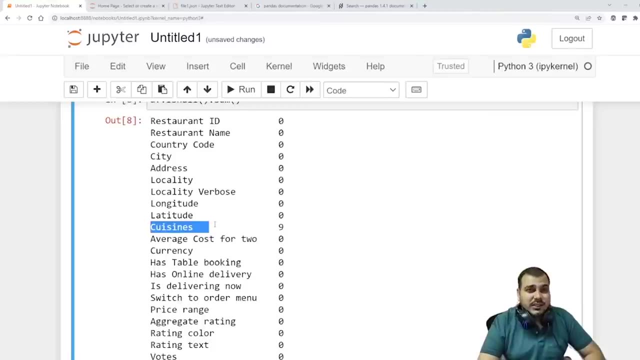 So here in cosines you can see that there are 9 missing values. If you want to do anything with respect to the missing values, you basically have to work on this specific feature. Now. can I find out any relationship with respect to cosines with any other target variables or any other independent features? 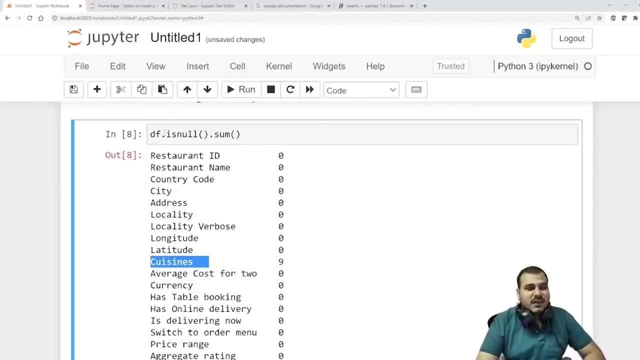 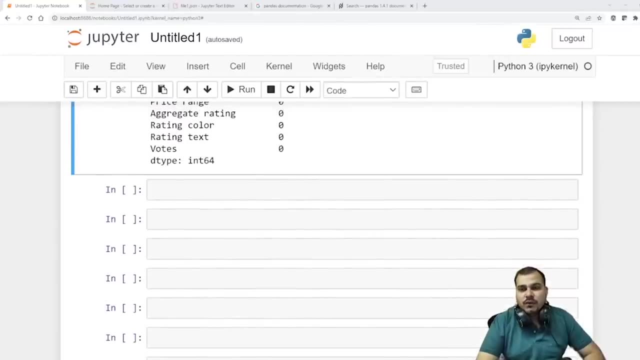 That we will try to do. But right now you have got this specific information that that many number of missing values are there. Now this is one way. In another way, I will just write a simple code which will actually tell me all the information, all the features that have missing values over here. 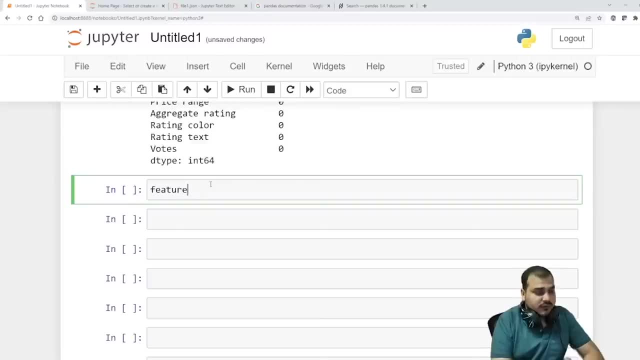 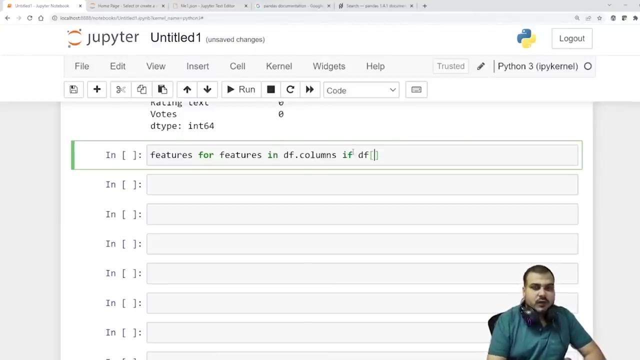 So what I can basically do, I'll say that features for features. so I'll write dfcolumns. I want to check which all variables have missing values. So I'm saying that, for every feature in dfcolumn, go and check if dfcolumns- dfcolumns, which is represented by featureisNullsum- is greater than 1.. 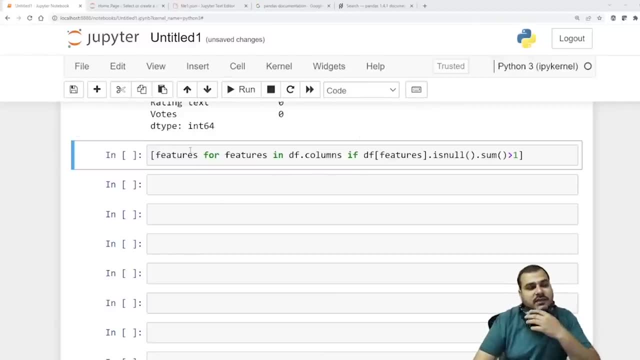 So this is basically a list comprehension. So here what I'm saying is that features for features in dfcolumns. that basically means we are using this temporary variable, called as features, which will iterate through dfcolumns, and then I will say that if that specific feature is null, 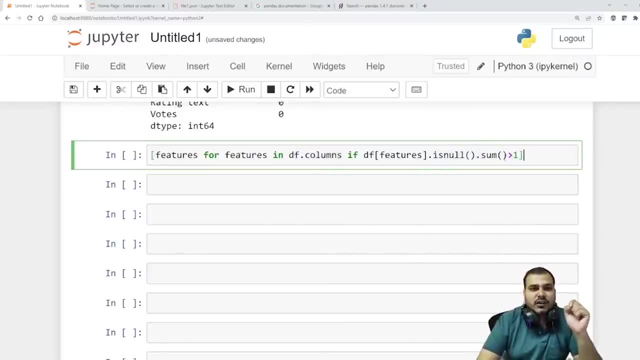 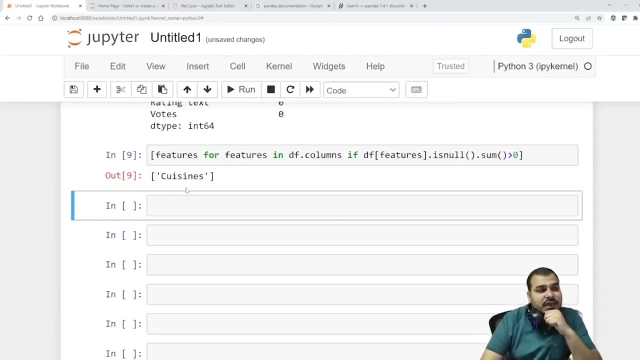 or dfcolumnssum is greater than 1,. I should not write greater than 1, but instead I can write greater than 0 also. So if I go and execute it here, you can see that I'm having cosines, So definitely I'm able to get. what is the specific thing with respect to this? 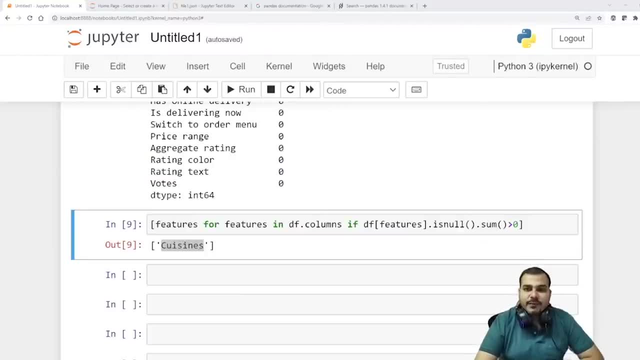 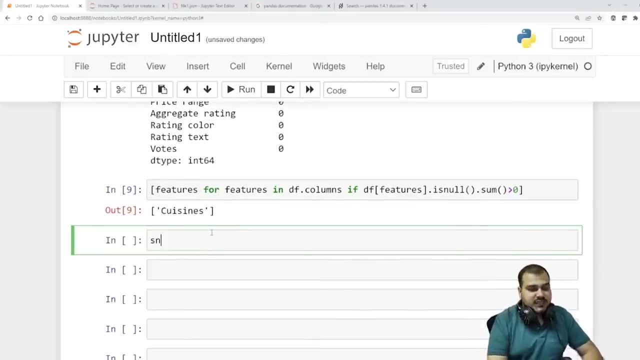 that I'm able to see the null values. Now let's go to the next step with respect to heatmap. can we plot something? So for heatmap I will basically be using snsheatmap, And here I'll basically put the condition which says that dfisNull. 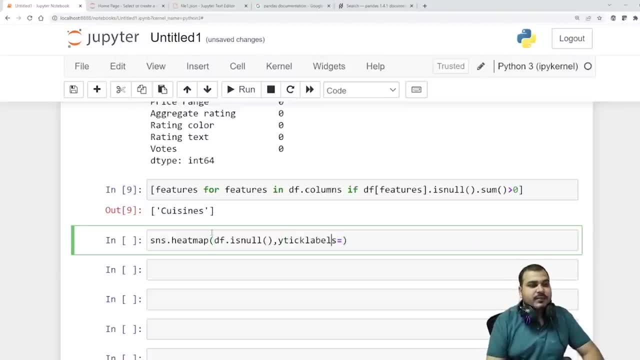 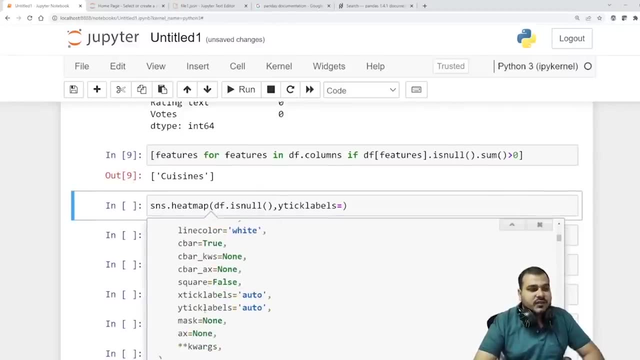 And here I will say that in y, because my second parameter is y tick labels. If I go and press shift tab over here, always try to see this feature. And with respect to this particular feature, what are I'm actually using? X tick label is there? y tick label is there. 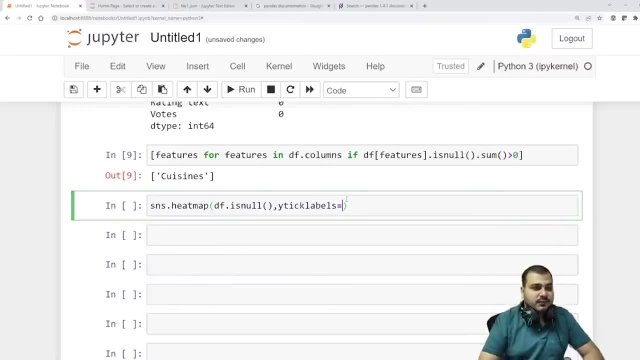 Right now I don't want to show much things in y, So I'll just keep it as false, Because I'm focusing only on df. with respect to that, Then I can also say that I want to keep it as false. I can also use cbar. it is also another feature over there. 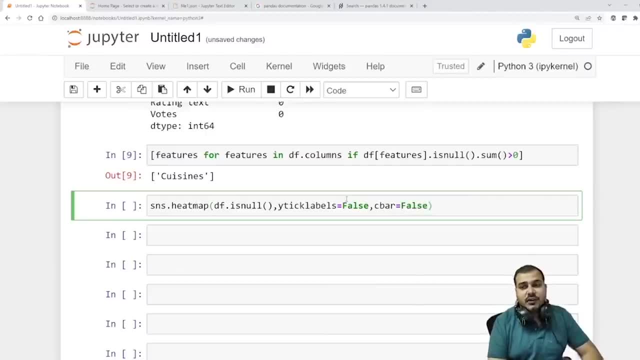 You can understand by just seeing the documentation what all things it can do. And then I will use a cmap And inside this cmap I can use any one. I'll basically search for it Over here. you can see here more options. is not visible. 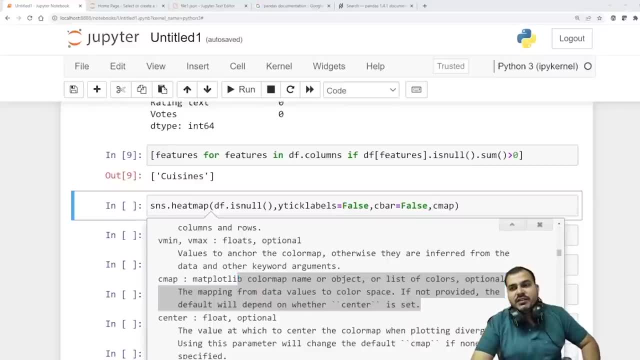 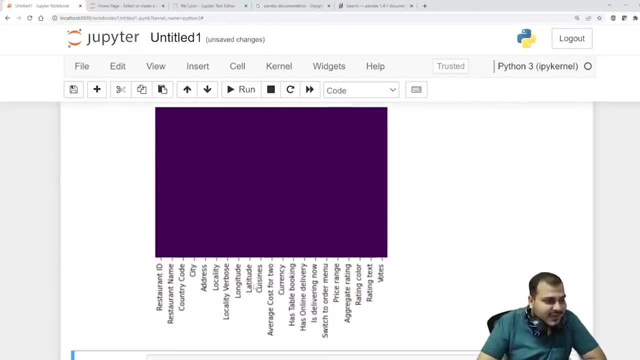 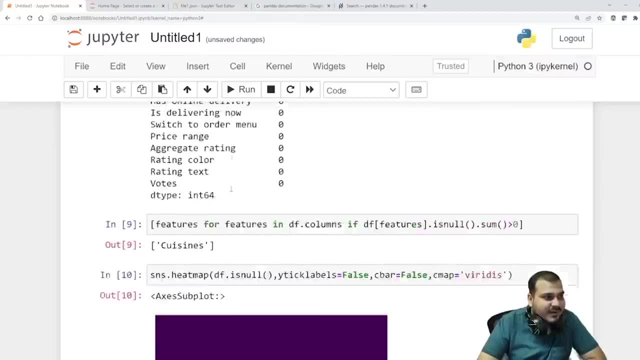 So here obviously I'm not going to use varidice. So here obviously I'm not going to use varidice. So here obviously I'm not going to use varidice thing i should have that right. let's see some. some cosines has nine. okay, the total number of 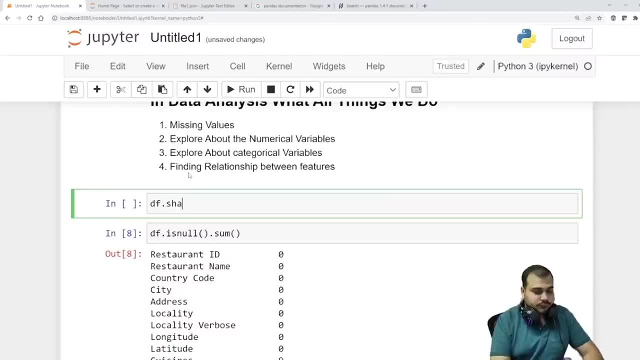 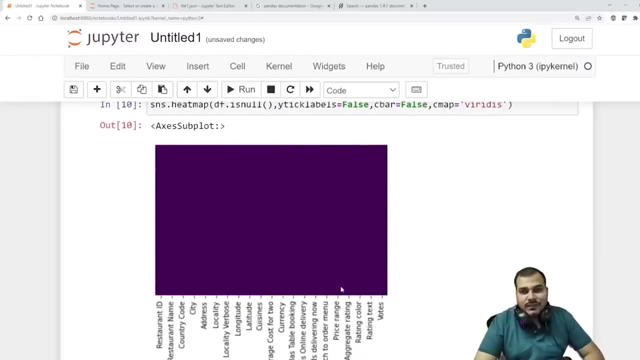 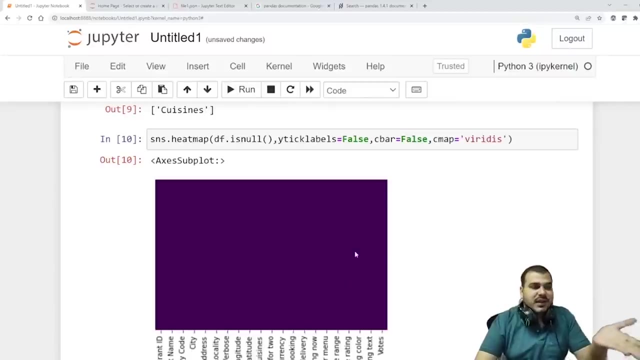 let's say total number of df dot. they are around 9551 rows. so because of that it is not getting visible over here very small number of nan values, so that is the reason we cannot see it. but if there are many, many, you can definitely check it out. so we have. we have understood about the missing. 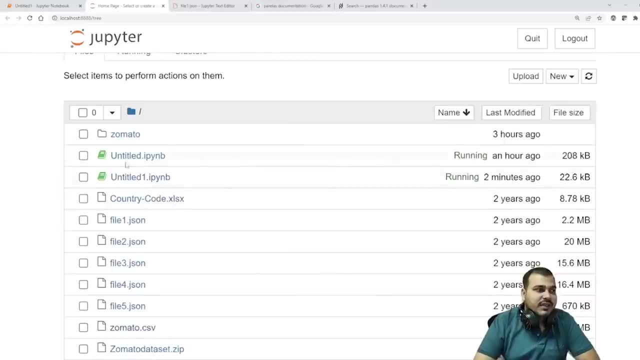 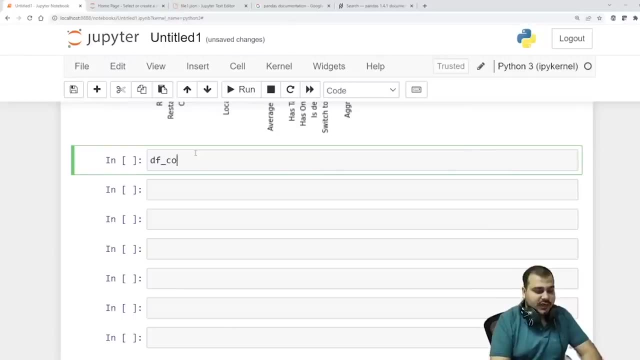 values and we have seen that now. i have already told you that there is another data set which is called as country code. now let's try to see that what this data set basically has. so i'm going to write df- dot underscore country, and i'm going to say pd- dot read underscore csv, and i'm going to 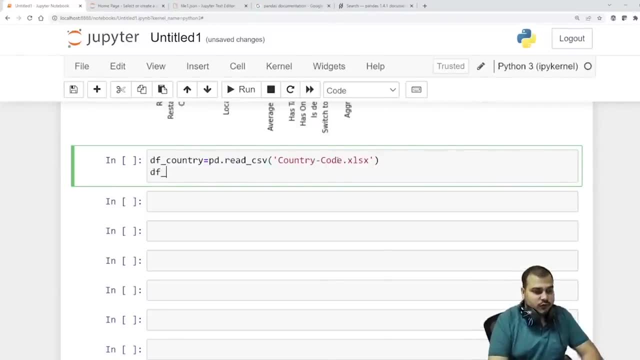 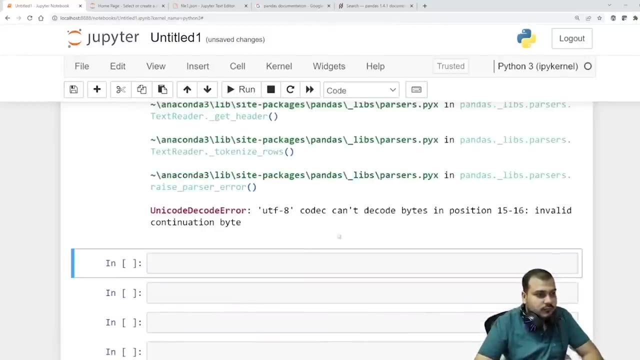 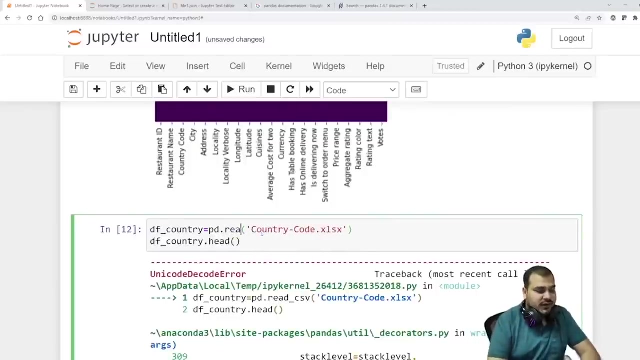 use and then i'm going to basically write df, dot, country, dot head. it is giving me an error. let's see what is the error. you okay here. also some problems with respect to invalid continuation byte. i cannot use read underscore csv. i have to use read underscore excel because it is an excel file. otherwise 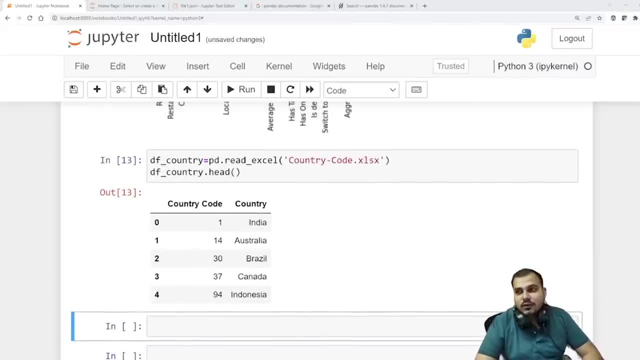 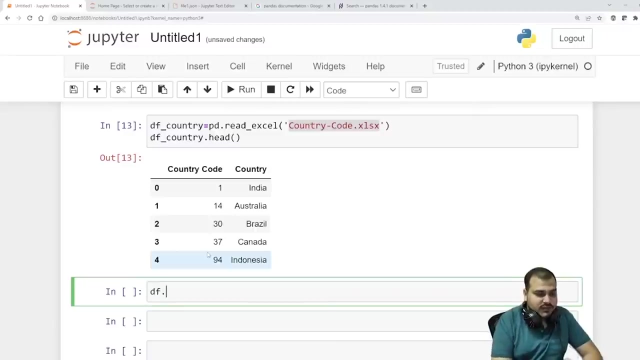 again, you have to use that same encoding things to make it work. how to deal with missing values, that i will try to show you in feature engineering. so here you have this one country code, country code xls. so what you have over here see country code, country, two features, if i go, and probably 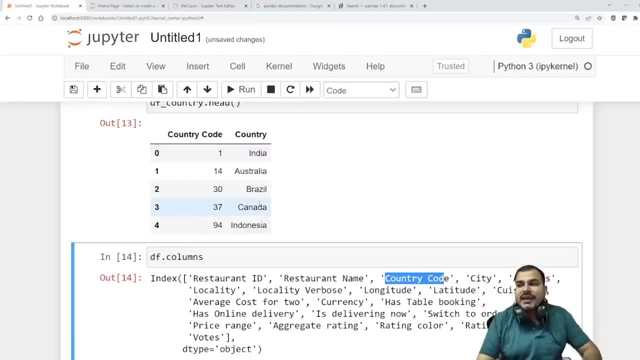 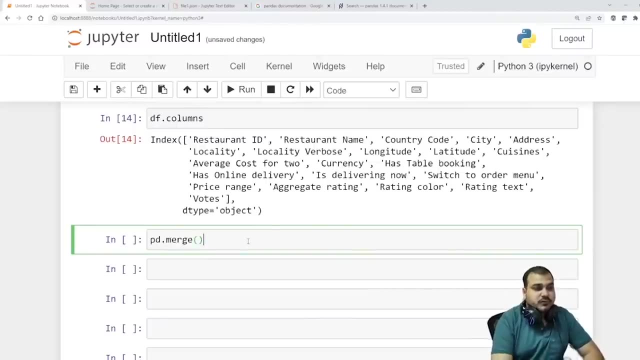 have country code over here. here also country code are there. can we combine these two data frames? so what we will do in order to combine, we will be using pd dot merge. so merge is a function which will actually help us to combine. in the left, i will give my another data set in the right. i can. 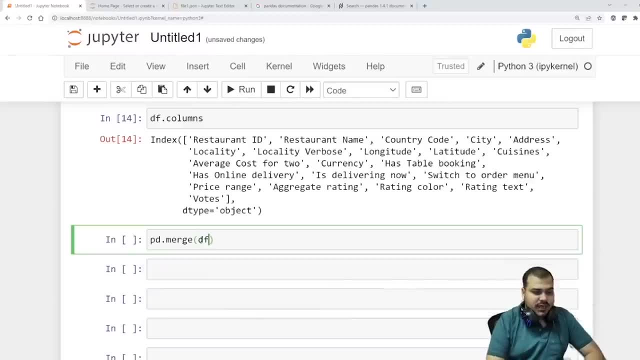 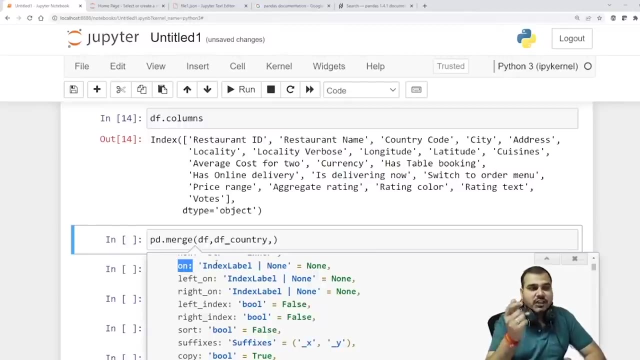 give another data set. so here i'll give df and here i'll give df, df, underscore, country. but let's see another feature. so there will be one feature which will be a function, which will be a function which will basically say: on this, on basically says that, on which feature you are basically going. 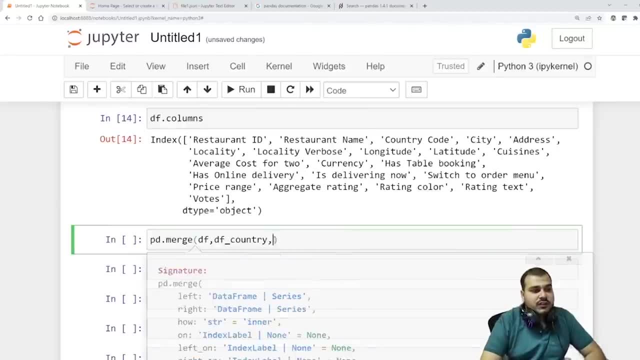 to combine that two tables. so here i'm just going to say: on is equal to. i'm going to copy this country code. so here i've copied this country code, and then it will basically be left as how. and here there is also one more keyword which is called as how. this how will basically specify: 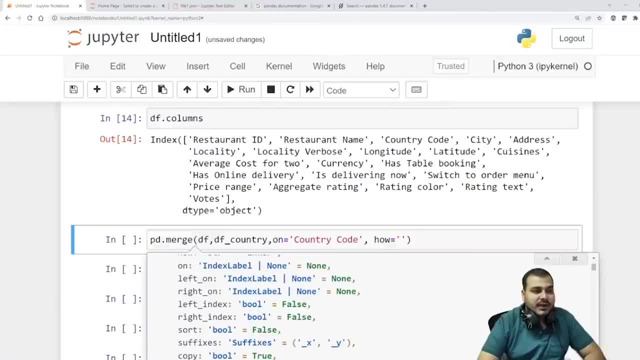 whether you have to focus on left table or right table. so here, probably somewhere you'll be able to see, this is how, whether you want a left join, the right join or a inner join, but right now i want to really focus on my left hand side of table, which is df, because 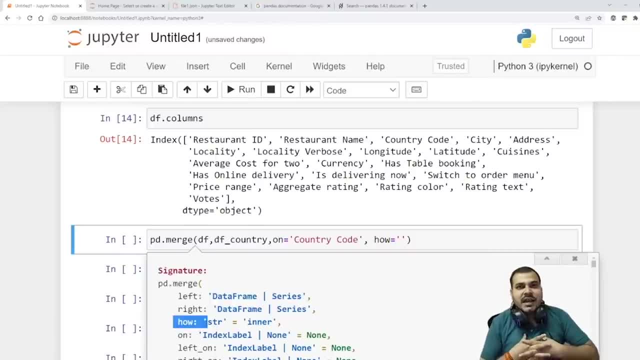 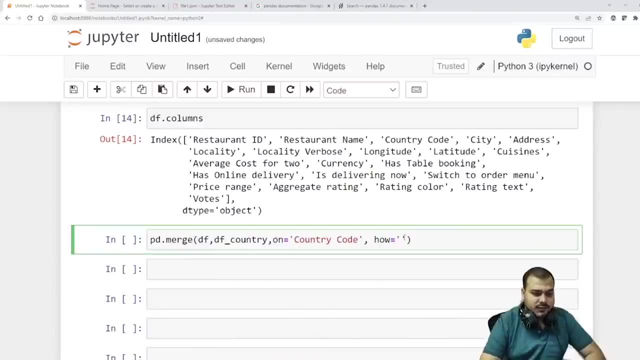 this has the entire data set in the right hand side. i just have one additional column that is country name. so, in order to combine it, what i'm actually going to do, i'm just going to focus on left. so here is my left, and once you see this, you will be able to see that i will be able to get. 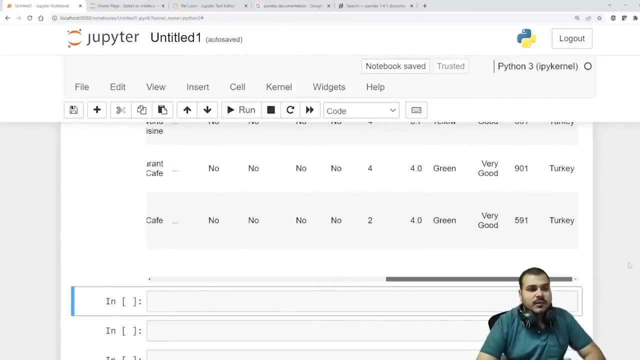 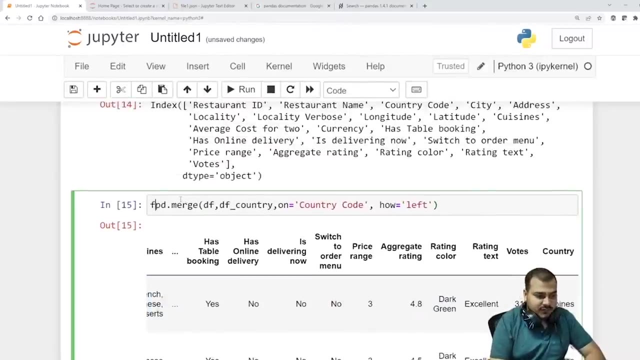 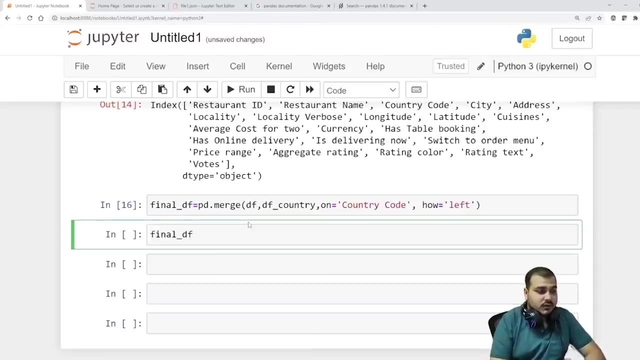 all the records and somewhere you'll also be able to see country. see in the last thing, country is getting added. i will just save this in my final data frame, which is called as final underscore df. so this is my final underscore df and now, if you go and probably see final underscore df, dot head, and if you check, 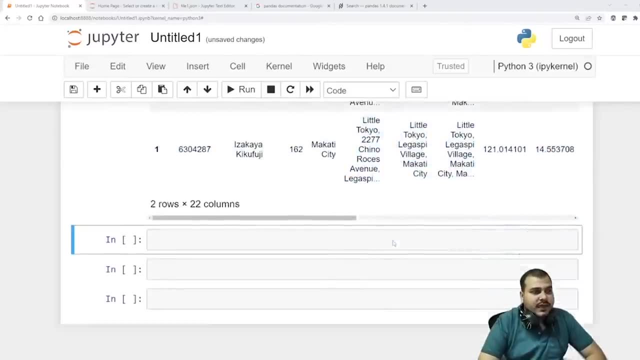 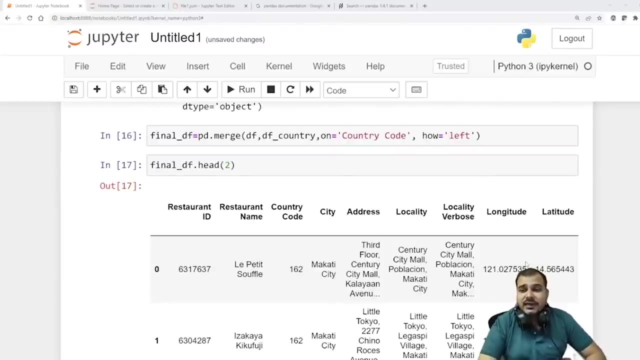 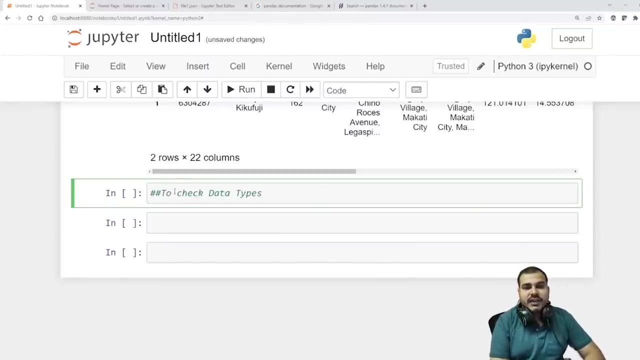 the first two records, you will be able to find out everything. so finally, final underscore df is my entire data set. now let's go ahead inside the data set and try to explore what all things we have. there is also another way to check data types, if you want to. 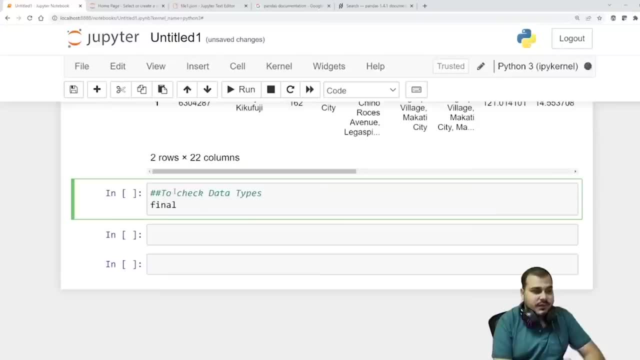 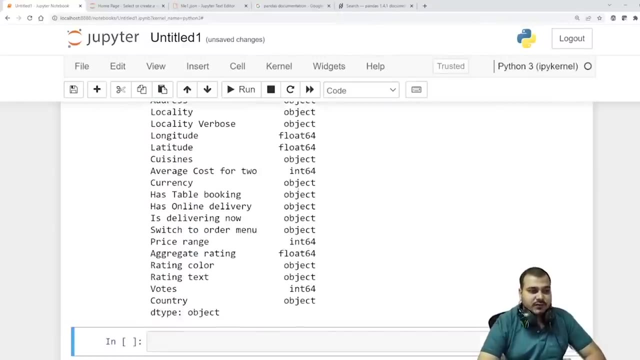 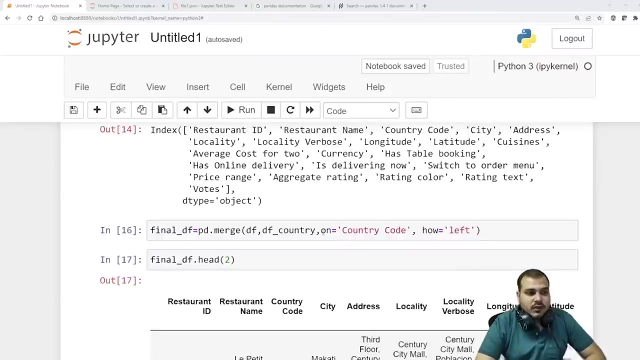 check data types. you just have to write something like this final underscore: df, dot d types. so there is also d types, which will actually help you to just get the data types information. so just use dot d types and there you will be able to see the entire data. this on is basically used to match on. 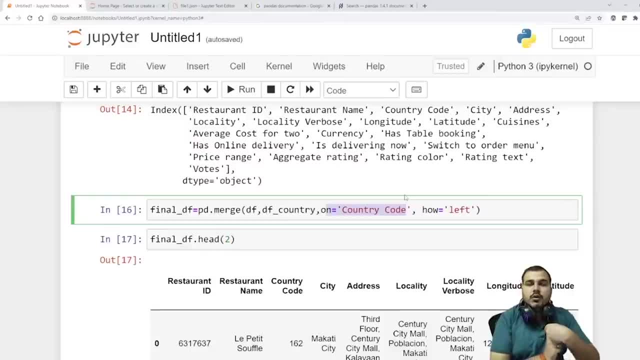 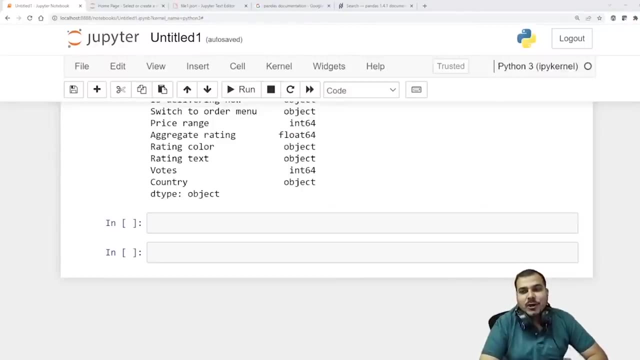 which column you are basically going to combine, just like how you do left join right, join on on a specific column if you- if you have seen my sequel of my videos i have already uploaded. let's go to the next step. now let's try to do something amazing. and now let's. 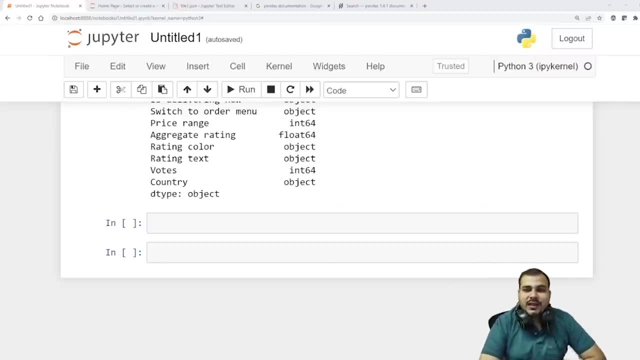 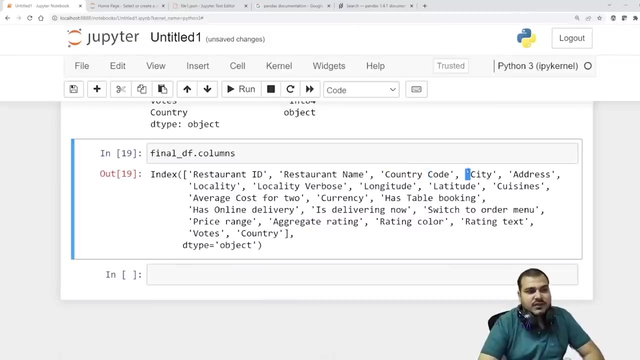 try to explore something from the data now understand one thing is that if i go and see this data, there are features like: okay, let's, let's open this, let's open this final underscore: df dot columns. here you'll be able to see features like country code, city address, locality, locality verbose- longitude, latitude. 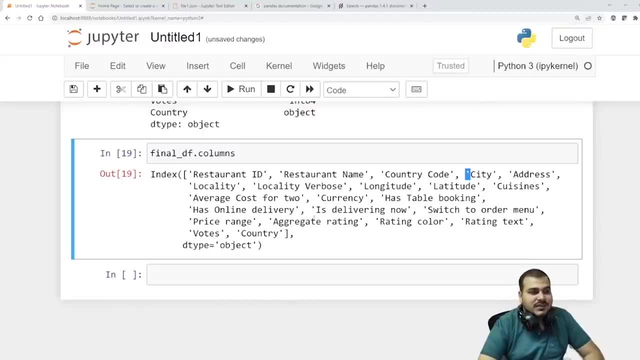 cuisines. average cost for two currency. this, this, this are there. let's pick up something, okay. let's pick up, probably. let's see that i i just want to find out something, okay, and mainly understand whatever things i will do right now. i will make sure that i'll write observations for those. so 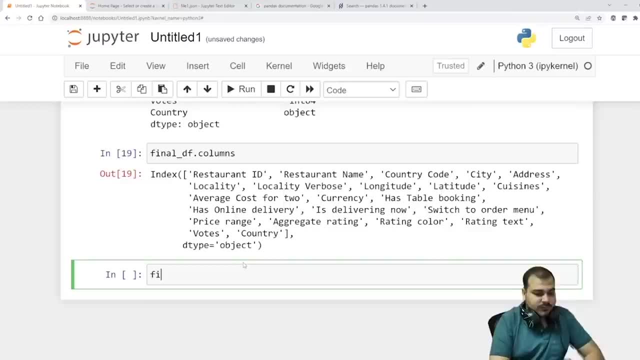 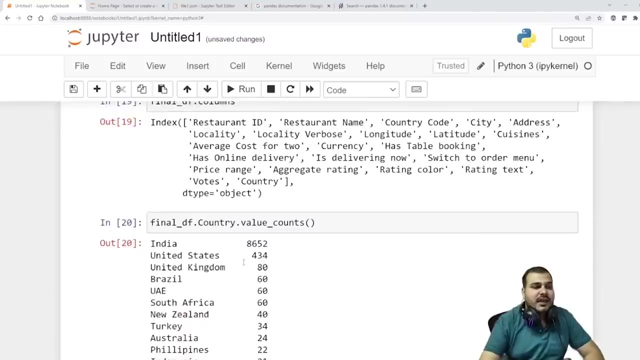 what i'm actually going to do over here is that let's say that i'm going to use something like this final underscore: df, dot, country, dot, value, underscore count. what i'm actually doing over here, i'm just trying to find out how many different countries are there and with respect to this particular countries. so 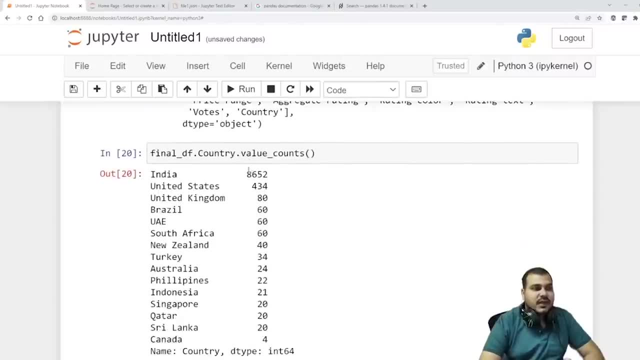 in this records right with respect to a specific countries, how many records are there? so, in india, you will be able to see 8652 records. in united states, you will be able to see 434. united kingdom: 80, 60, 60, 60, 60. so from this, 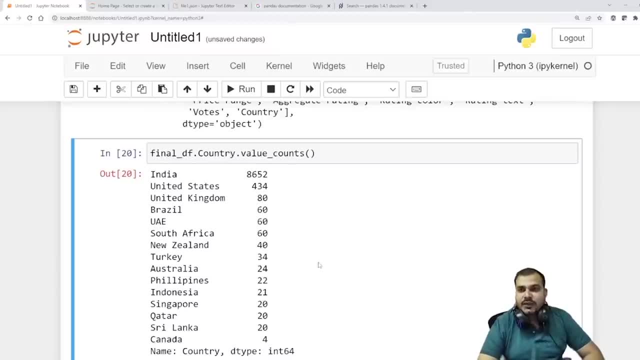 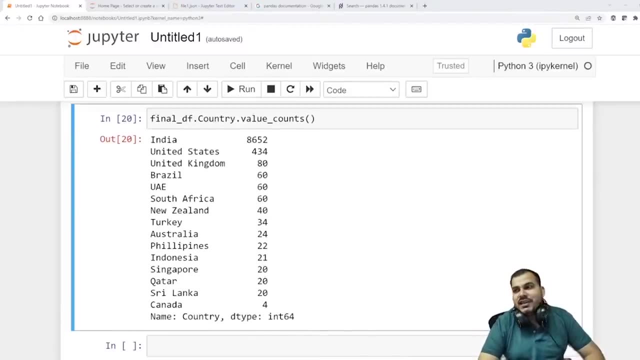 what kind of observation do you feel that you can come up with? can you say that zomato is mostly available in india itself? obviously in usa they just have a website which they will recommend some kind of restaurants. but just understand one thing over here is that 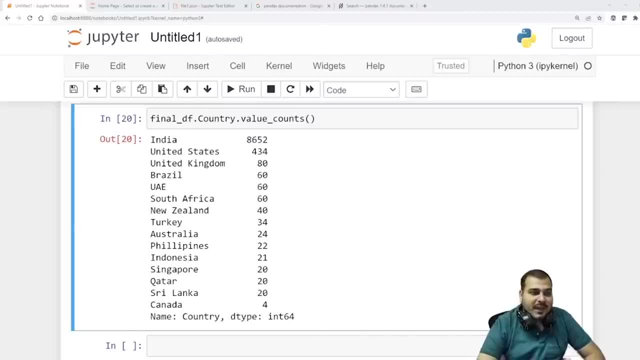 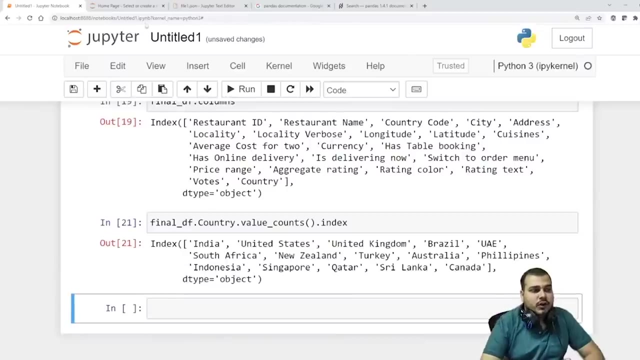 in india. the main base of zomato is there, so maximum number of transactions that may probably be happening is in india, right? i hope everybody is able to understand, right? so from this, this information you are able to get now, if i write dot index now with respect to the dot index, you'll 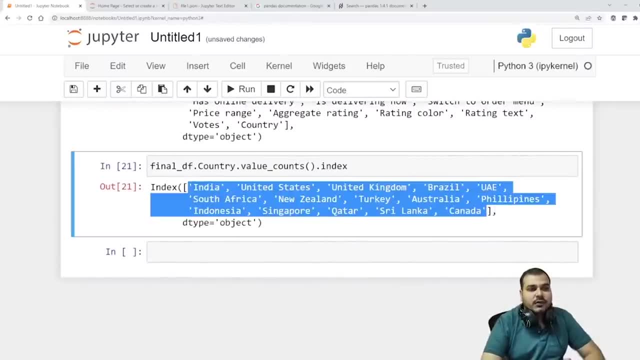 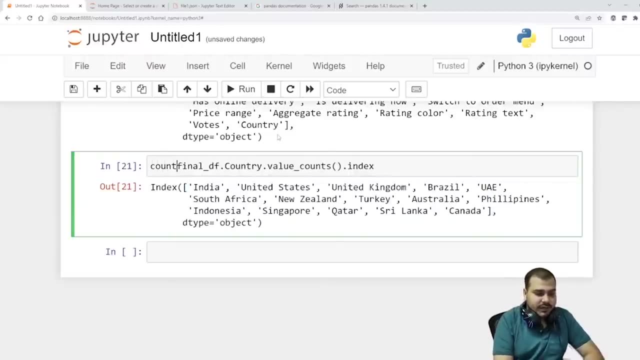 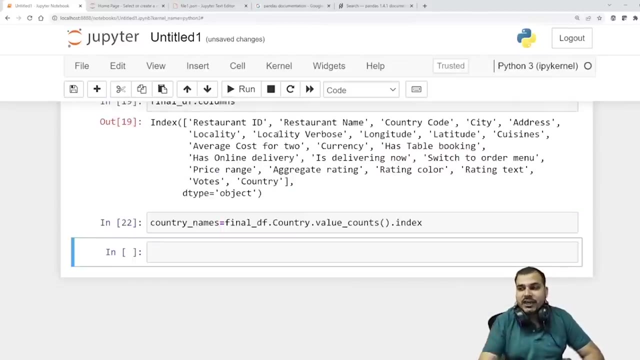 be able to see. i'm able to get all the country's name with respect to that specific records. okay, so let me just save this, probably in a variable which is like country names. i'll tell you why i'm doing it. everything will make understand completely. after this i'm going to plot some pie chart. 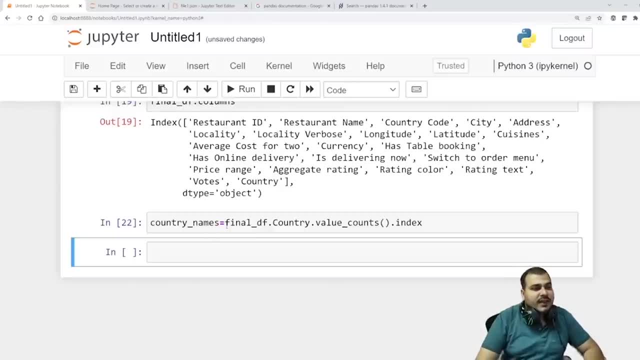 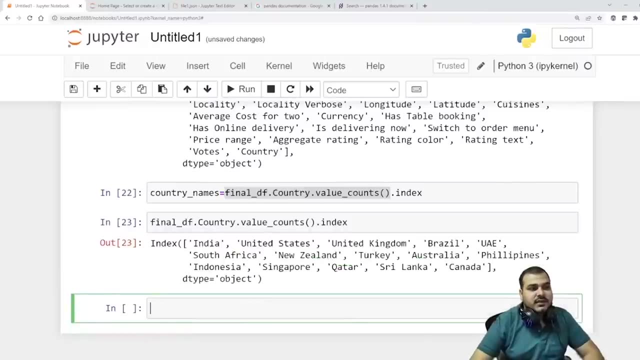 i'm going to plot some chart now. similarly, if i use the same thing and if i execute it with dot index, you will be able to see that i'm getting this country names, but with dot value counts i will also be able to get dot value counts. i'll be able to get. 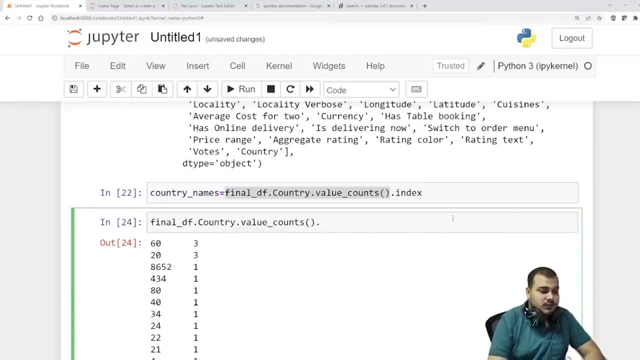 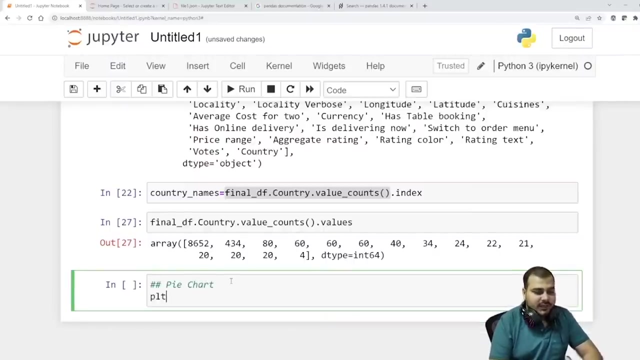 sorry country is dot. sorry value count. start valило dot values. let's see dot val values. okay, so with respect to dot values, i'm actually getting all the records for that particular country name. now this two i have. the reason why i am doing this here is that because i am going to create some pie chart. now, how do we create a pie chart? so 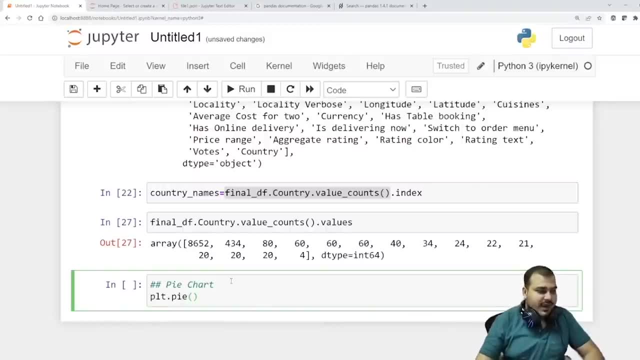 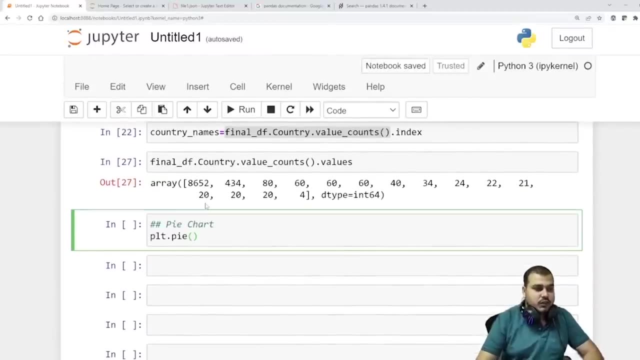 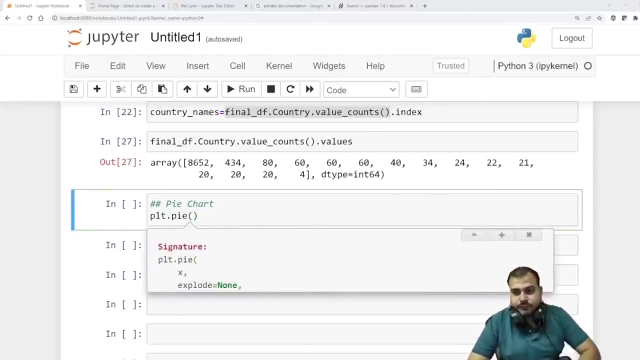 you use plot dot pi and, with respect to this, you use plot dot pi and, with respect to this, you can actually put out all your variables. so i am going to press shift tab. i need to have my x variable if i am actually putting plot pi chart over here. i definitely have to use this now over. 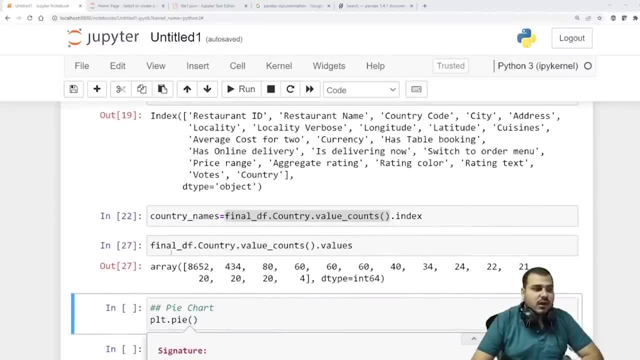 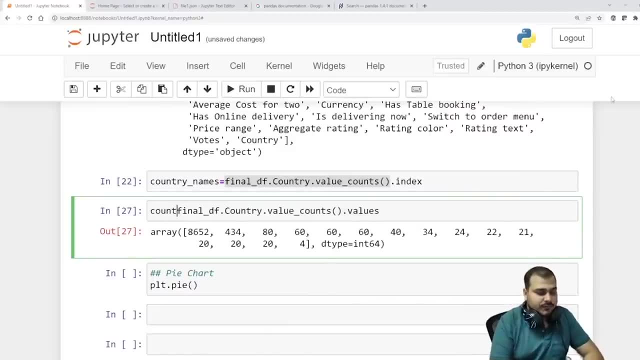 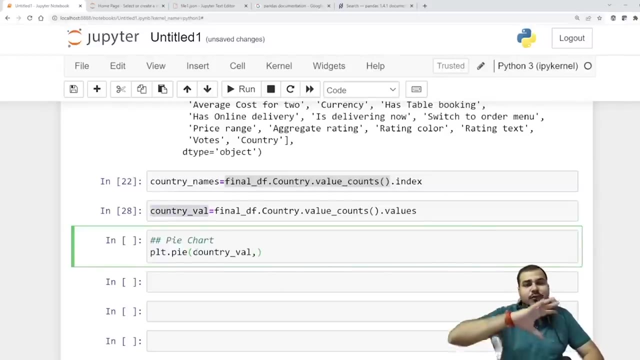 here in the x value. i will try to use my names or values, whatever things you want. let's say that i want to use my values, so here i will store this as my country value. so i am going to put this entirely over here in the x axis because i want to see in the pie chart. 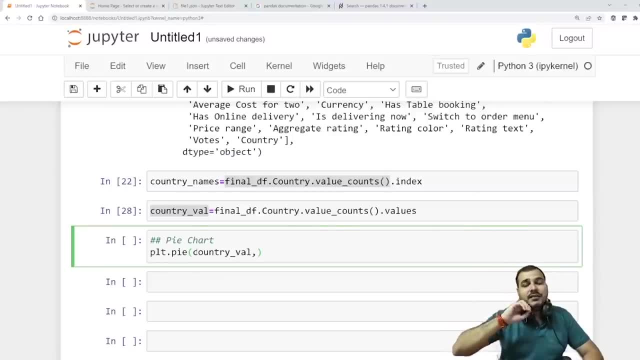 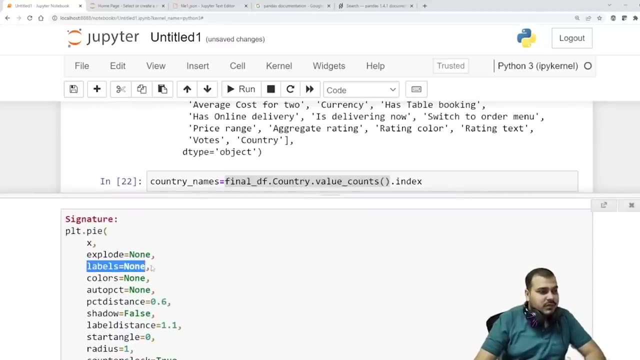 you which country has the maximum transactions or maximum online orders or maximum kind of orders over here. so i'm going to use this as my x-axis. so this is my x-axis in plotpy. so here, if you expand it here, you'll be able to see it. and then you have labels. this is important. okay, labels is. 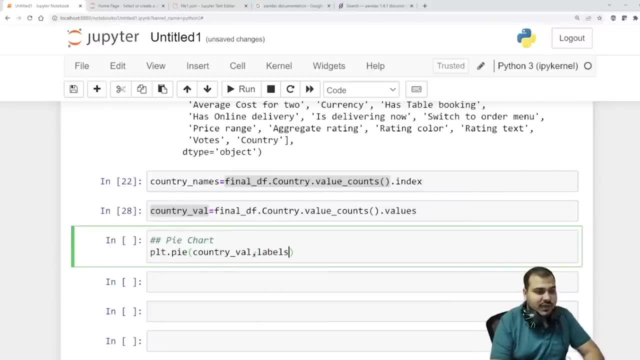 basically to give the labels on top of it. so i'm just going to use labels- is equal to: i'm going to assign this value to something like country name. okay, country name. so these two things are there now. if i execute it here, you'll be able to see that i'm getting a plot. now this plot looks really. 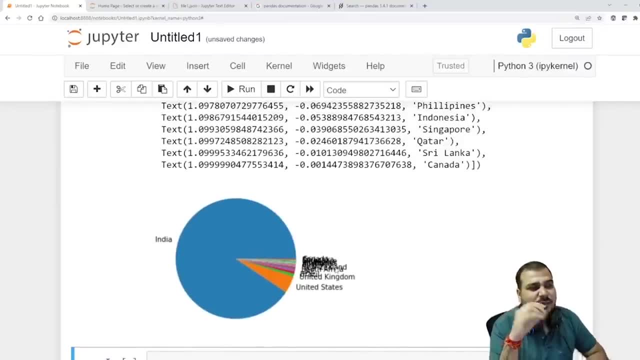 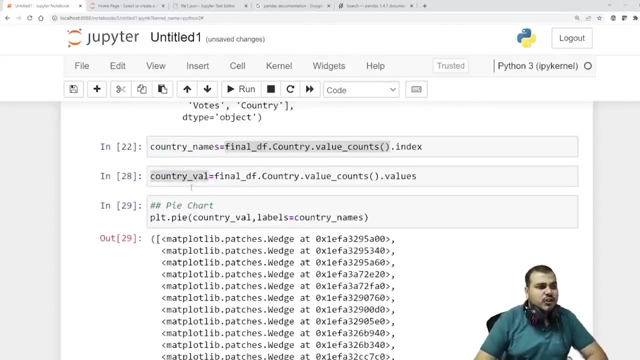 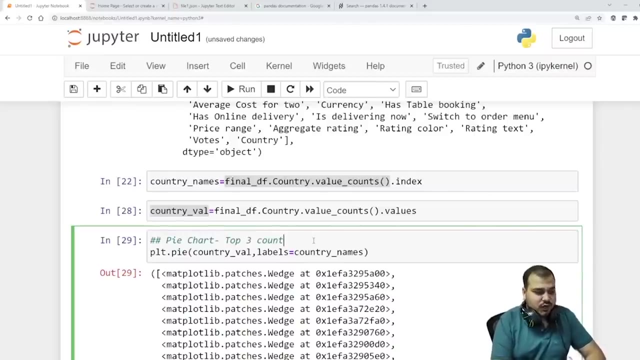 bad because obviously, the percentage of the information spread towards the different different countries is very less. so it is like jumbled up- complete. so what i'm going to do is that i'm just going to say which are the top five countries: top five countries or top three countries? so top three. 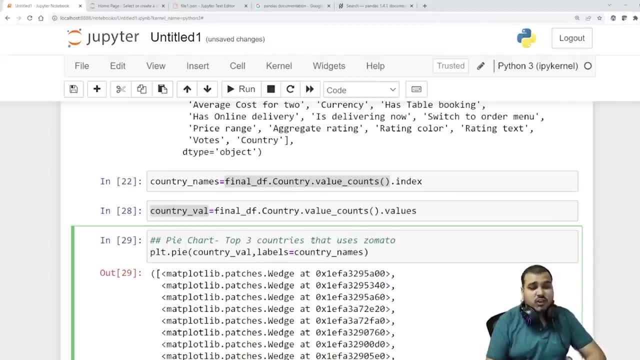 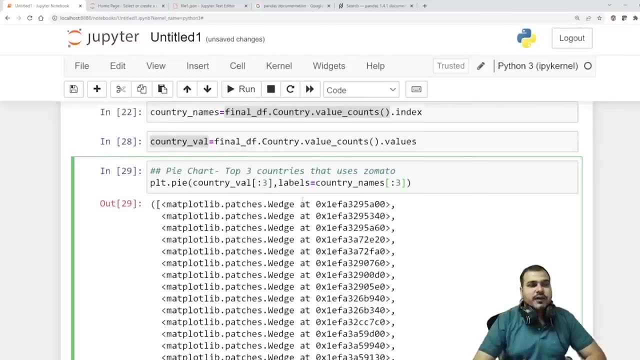 countries that uses zomato. that is based on your transaction right. so what i'm going to do here, i'm just going to use colon three. here also, i'm going to use colon three, colon three. so that basically says from entire, all the values over here i'm just going to take. 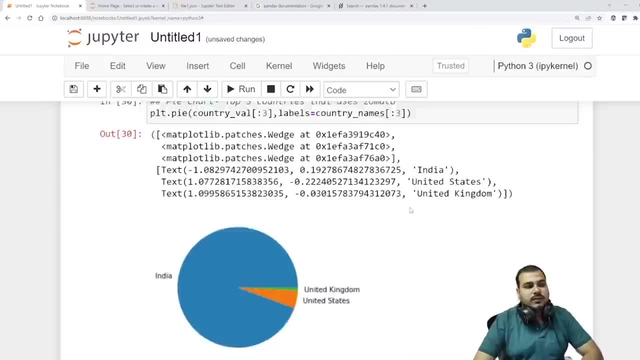 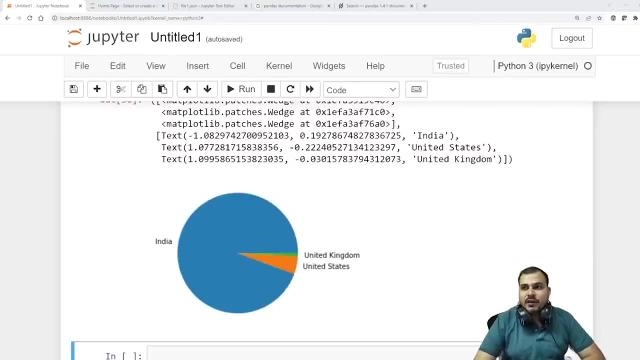 the top three values at top three countries and i'm going to just display- now it looks good now- which is the top three countries. that is basically using india, united states and united kingdom right, so i hope you are able to understand over here. with respect to the pie chart, like how is my 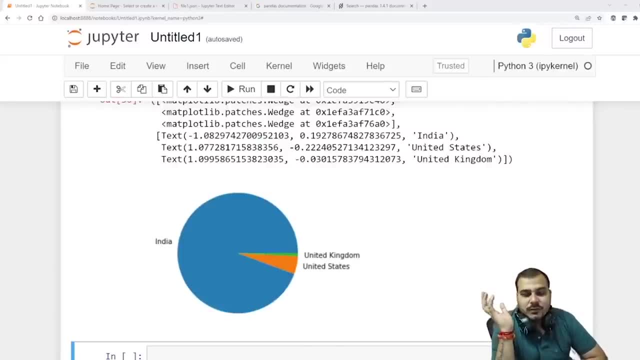 and over here, definitely with respect to zomato. zomato base company is in india, so obviously you can come to a conclusion that maximum number of transactions will happen in india. now, one more thing that i probably want to add is something called as percentage, because i need to see some 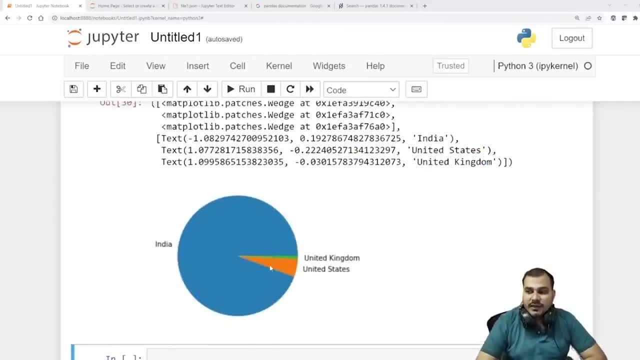 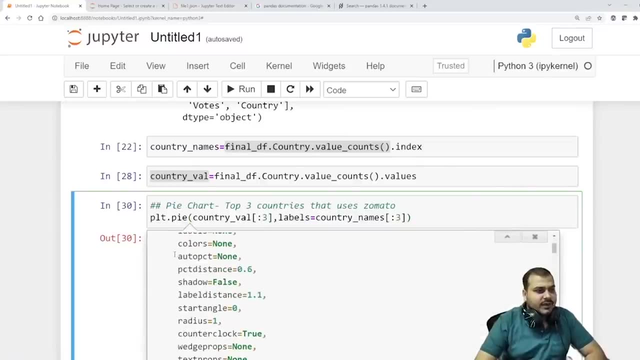 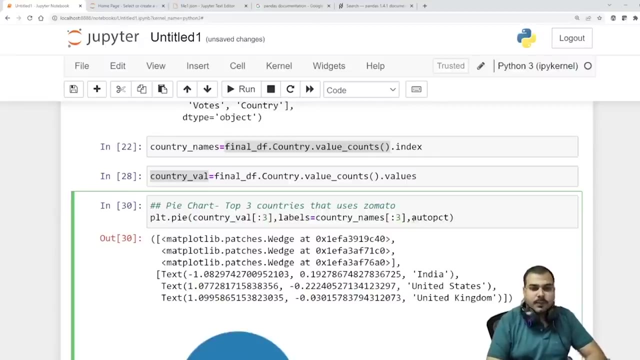 percentage also, right? that would be pretty much amazing, right? so what i'm actually going to do over here, there will be a parameter which is called as percentage also, and that parameter is something called an auto percentage. so i'll use this auto percentage and i'm going to use one property. if i want to see one property over here, what will i assign to this? 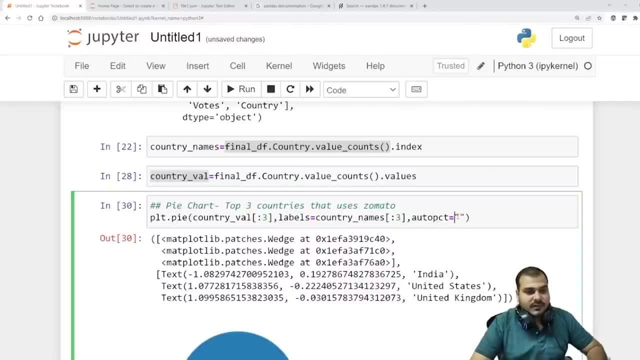 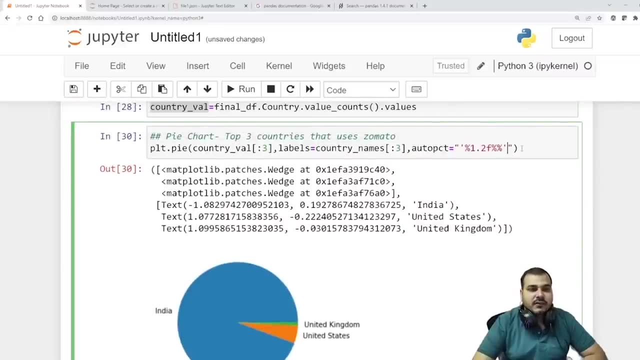 you can assign one format and that format. i can basically write something like this: this basically says that after this, after the decimal, two values will be mentioned when it is getting converted into percentage. so i'm just going to remove these double quotes, and this will definitely work then. 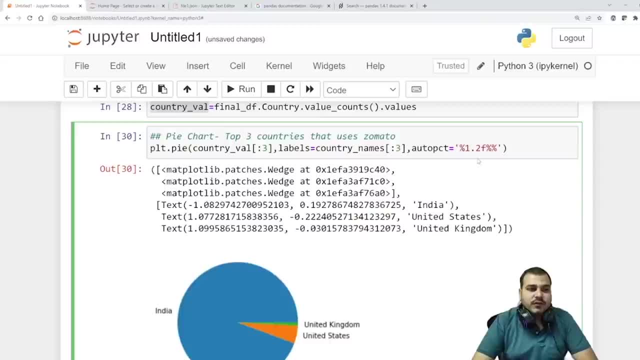 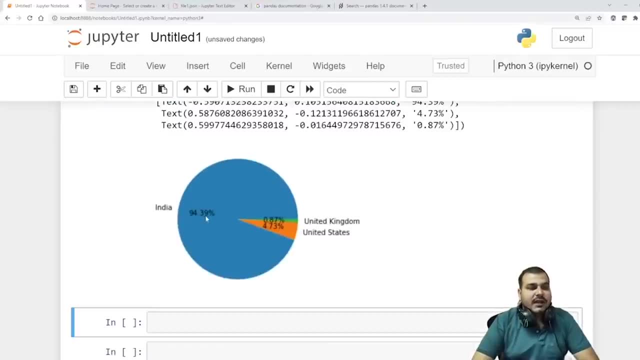 play with it. if i write: if i remove this two, what will happen? if i remove this? if i remove f, what will happen? just try to play with it now. if i execute it here, you can see now: 94.39 percentage is basically the orders are from india. 4.73 transaction is from united state. 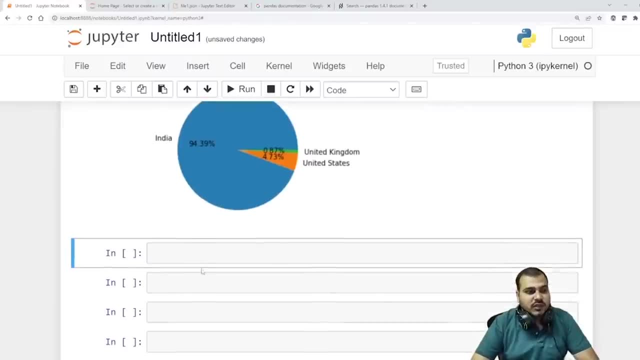 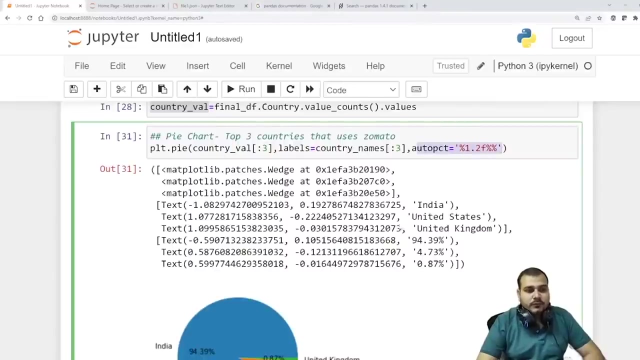 0.87 is from united kingdom. so here you need to write your observation. now tell me, suggest me, what observation should i write over here from this diagram, what kind of observation that you can see. you just need to add this particular property to get the percentage values. tell me what is the observation that you will write. 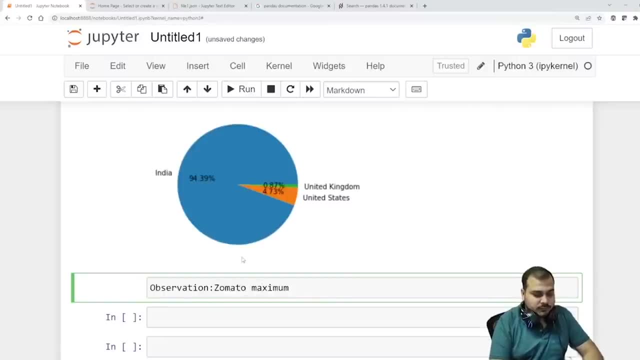 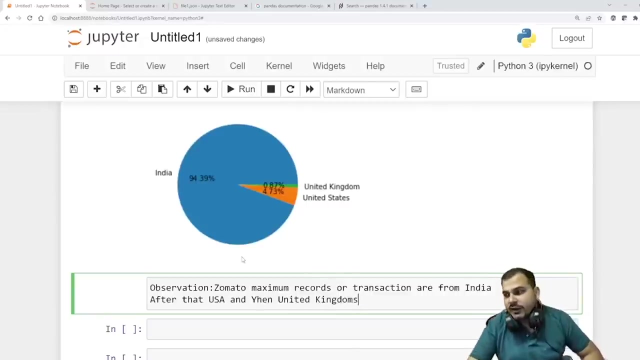 zomato maximum records or transactions are from india, okay, and then after that usa and then united kingdoms. you have to write your observation in your own words here. i have just written something, but just try to write so here. of the zomato maximum records, the transaction are from india, after that usa and 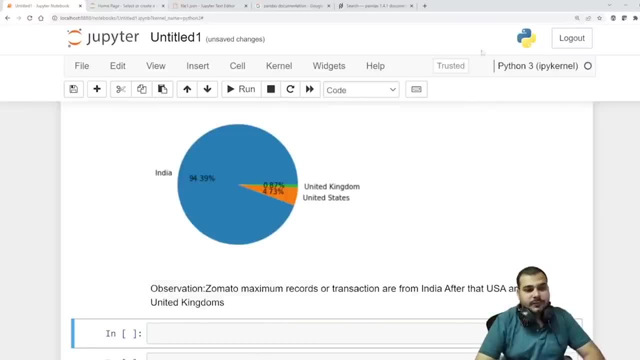 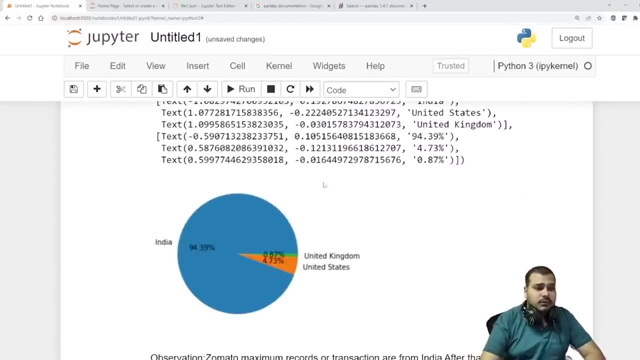 then united states, united kingdom. sorry, so this is my first observation that i have been able to take from this pie. major business is happening in india, you can say, and all a lot of things can come. okay, everybody is clear with this. i hope everybody is clear with this. i hope everybody is clear with this. i hope. 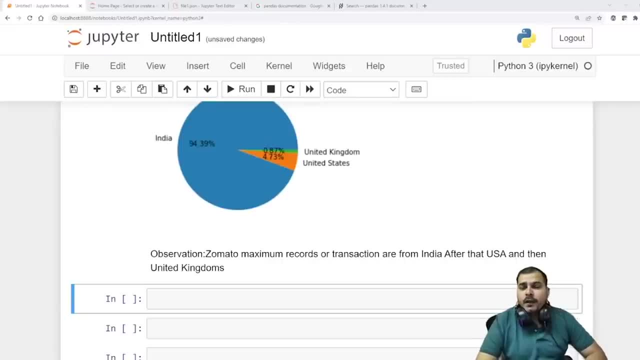 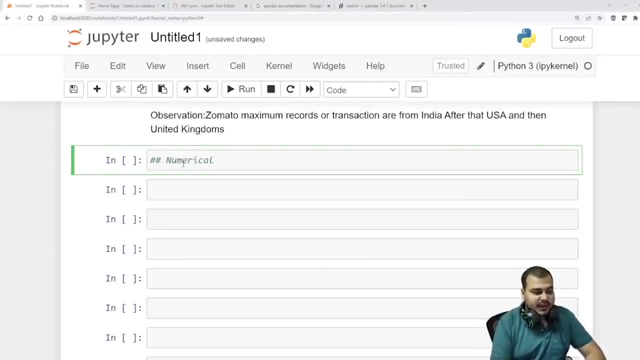 it's very simple till here. okay, now let's go with respect to the next one, that is, numerical variables. how do we identify how many numerical variables are there, how many numerical variables are? or? forget about numerical variables, let's do some exact relationship, uh, numerical variables. we can check it, check it in later stages, uh, but i want. 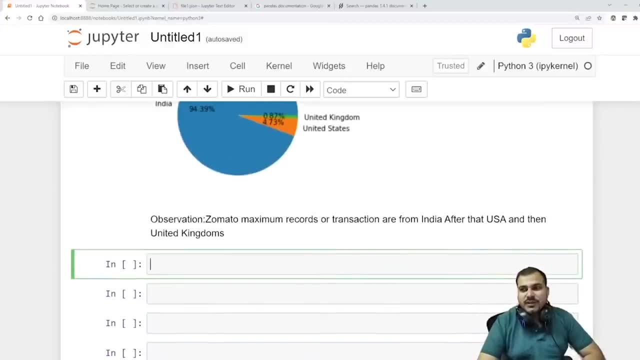 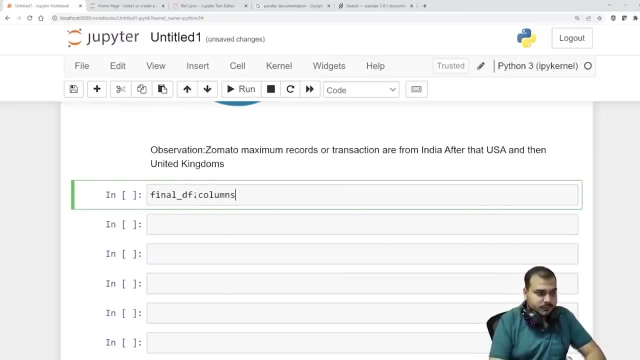 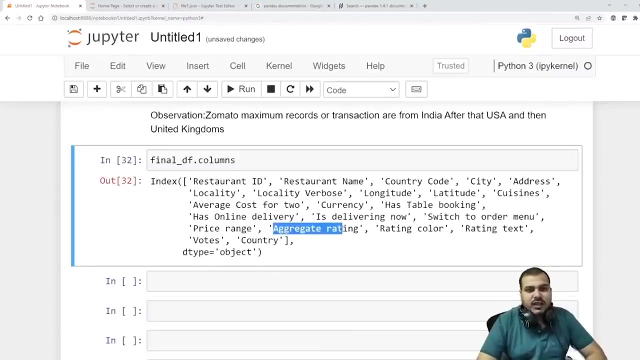 to really do more observation things, more uh relationships things, so that i will be able to see something now. if i go and write final underscore, df dot columns, if i execute this here, you can see some amazing features, which is called as aggregating rating, because i want to also 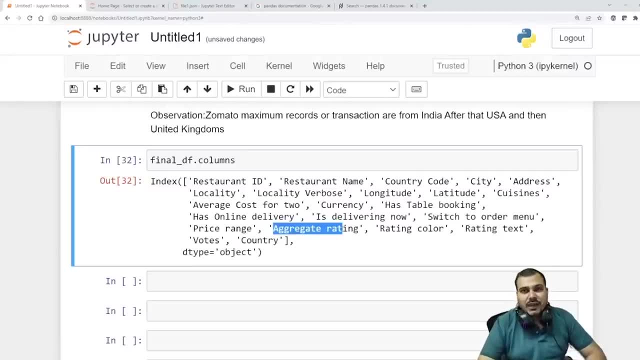 see, with respect to the rating, from which country more rating is actually coming, and i want to see this data, which is called as rating color, rating text and all okay. so what i'm actually going to do, i'll just write a small query. final underscore: df dot group by. i'm going to use a group by operation. 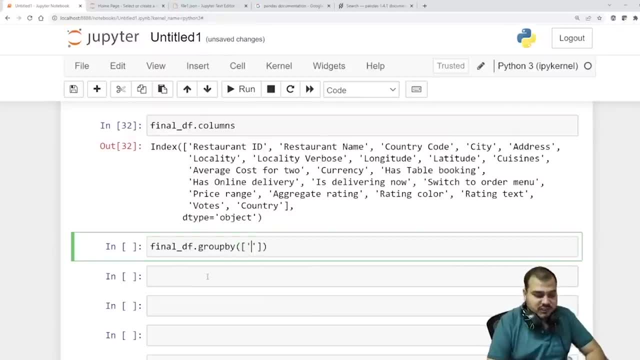 and with respect to a goodbye operation, here i'm going to use features which is called as aggregate rating, aggregate rating- and then i will also use rating color. see this, everybody: rating color. i'm going very slowly, guys, very, very slowly. i think you can write it down. i'm writing each and every line of code. 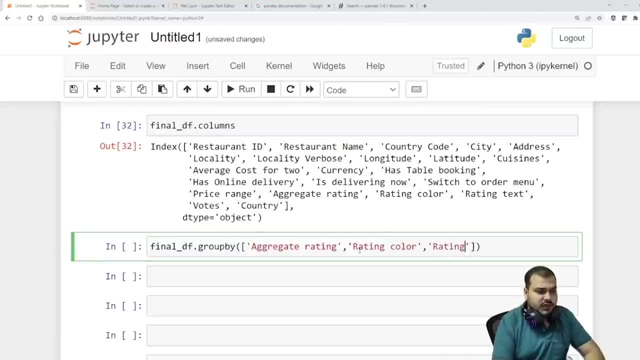 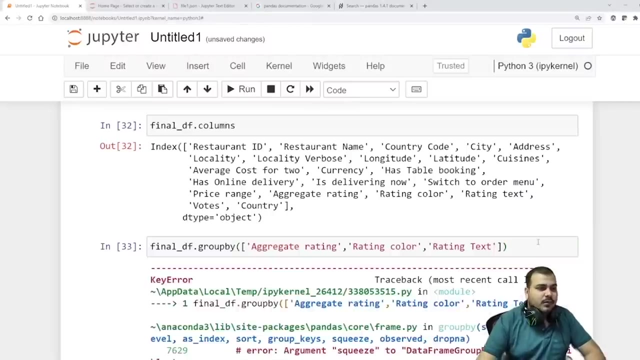 rating color, and then i'm also going to use rating text. so i'm basically going to uh, group by this three main features, and after this i'm also going to do one thing. so if i group by this and probably execute uh, i'll be getting an error. let's see. 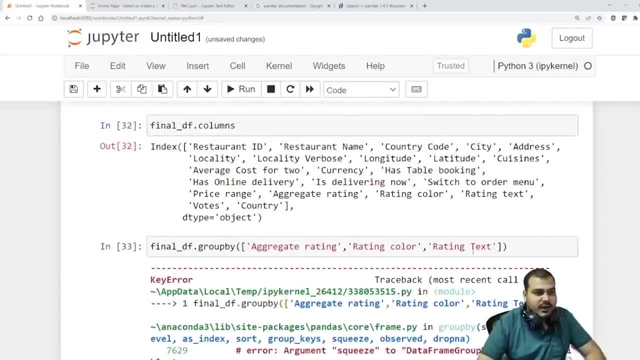 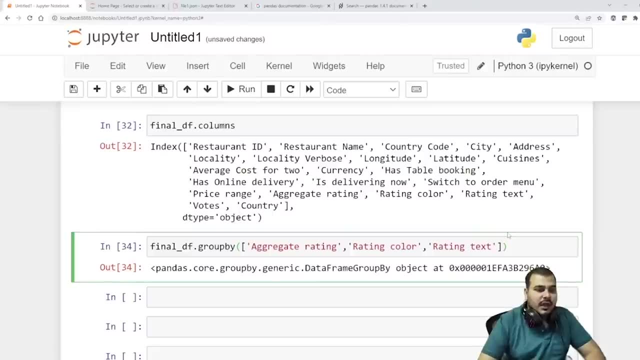 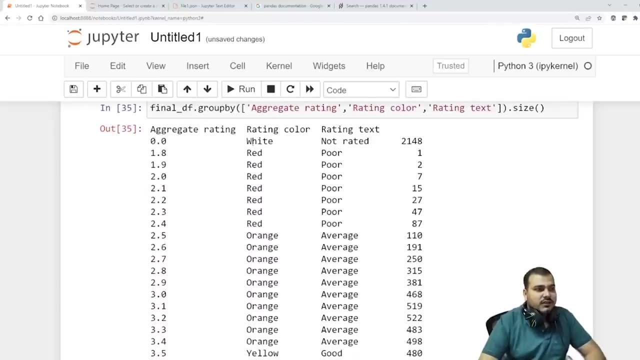 what is the error rating text? so it should be rating small t. so if i execute here, you can see that it is now a data frame group by object. now, if i write dot size, so if you, if i execute this dot size here, you will be able to see all the values like white, not rated, this, this. 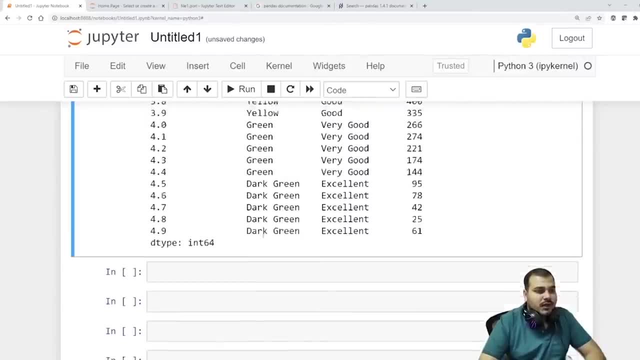 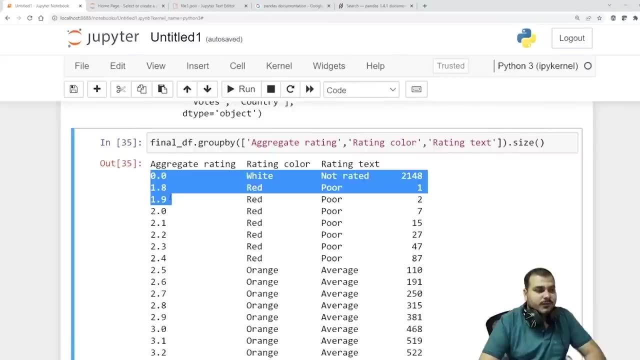 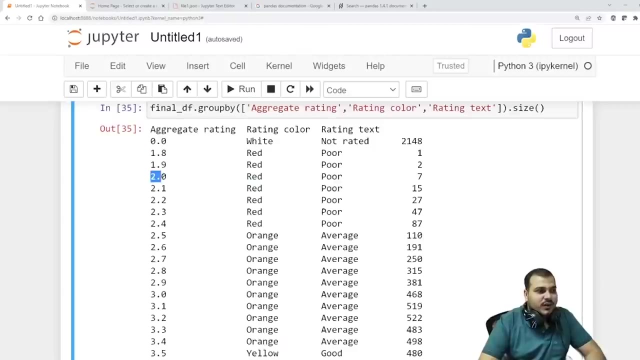 this, this, this are there and similarly good, good, good, very good. see over here one thing: you can see that when the rating color is white, that basically means your aggregate rating is 0.0. if your rating is red, then it is basically showing 1.8. 1.9 is also red, 2.0 is also red, 2.1 is also. 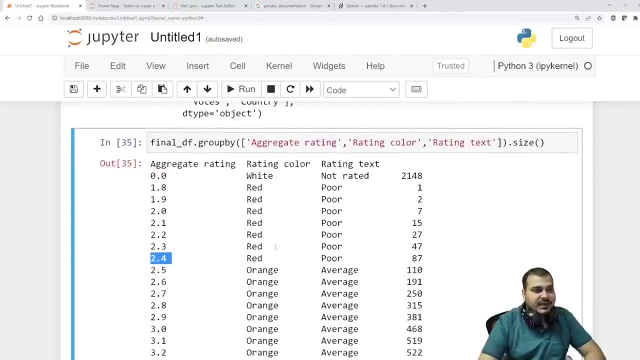 red, like this. 2.4 is also red, so all these are red. red basically means it is poor. it is poor, so these ratings are poor. with respect to this aggregate rating, you can see that it is poor. if i go with respect to the next one, which is in orange color here, you can see that these are my 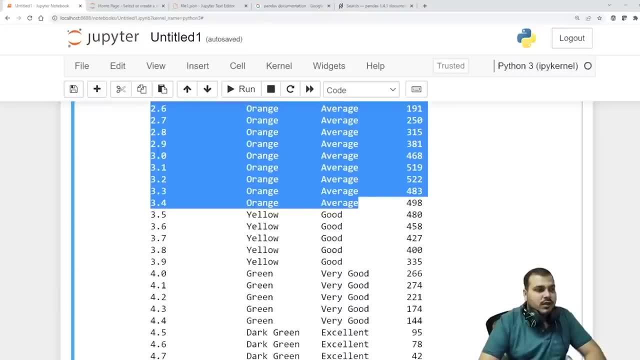 all average ratings from 2.5 to 3.4. then you have from 3.5 to 3.9. that is another rating over here here. you can also see that these are good, right, so it is displayed in yellow color. you can also see that these are good, right, so it is displayed in yellow color. 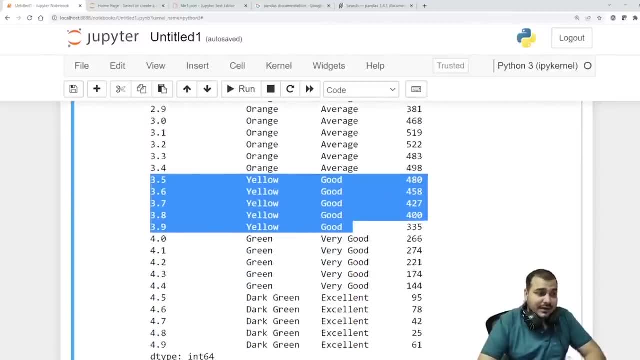 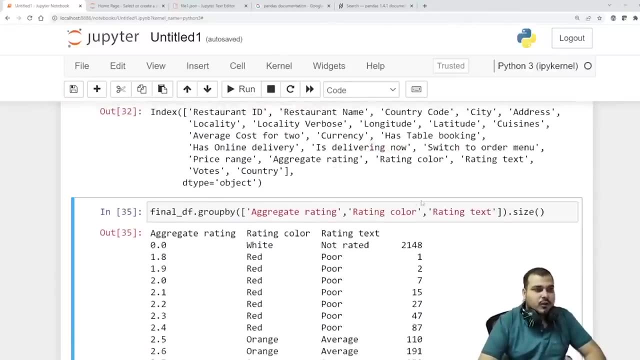 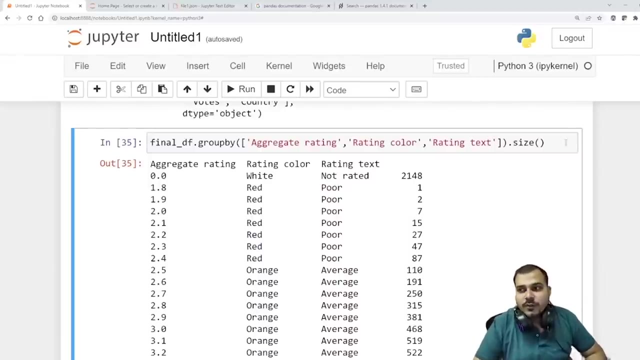 or the text is written in yellow color, like the rating colors are there and then from 4.0 to 4.9. we have very good and excellent. so this information i know i have actually able to find it out, so i'll also can write my- uh, i'll try to write my own observation over here now, what i'm actually. 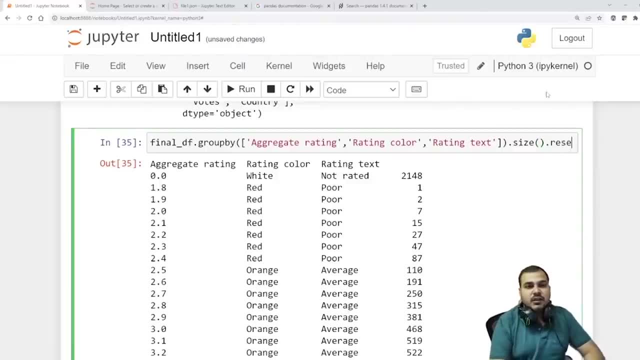 going to do over here is that, after i do this, i'll convert this into data frame. now, in order to convert this into data frame, what i will do is that i will just write reset underscore index and this is an invalid error. the reason it is an invalid error: because i have to continue over here. 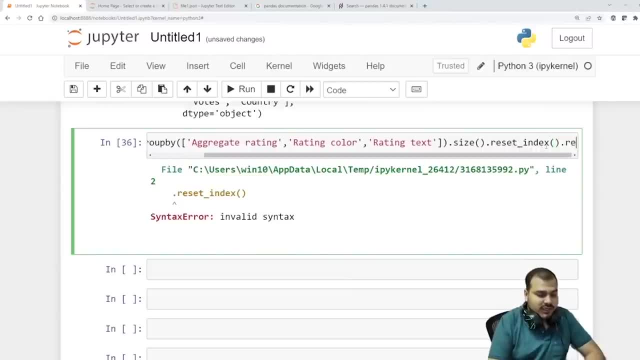 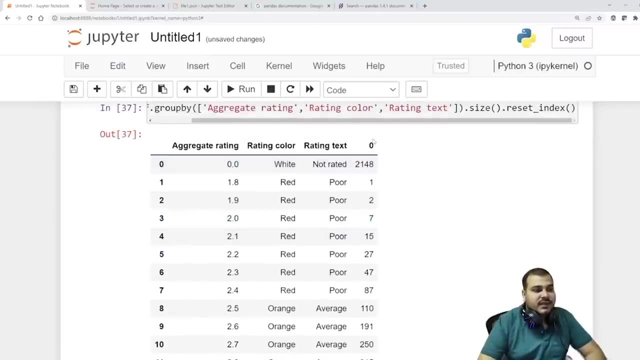 reset underscore index and then i'm basically going to just say that rename or if i just execute this, let's see what i'll get. so here you can get, see that i'm getting this particular things, and this is my zero value, since i've done group by with respect to 0.0. 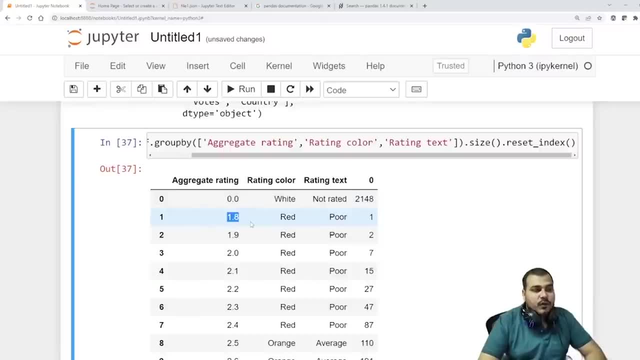 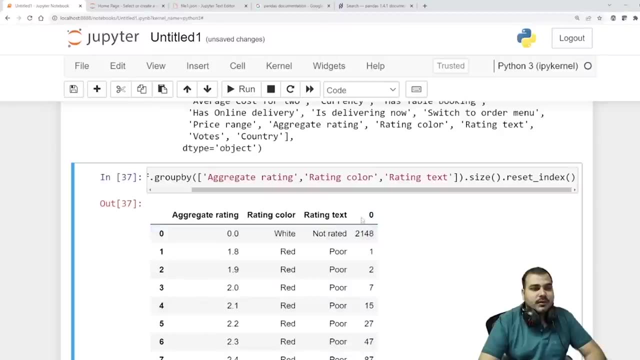 ratings. i have two, one, four, eight records. then, with respect to 1.8, i have one record, 1.92 record, 2.07 records over here, zero is coming. so instead of this zero, i'll try to rename it a different column. so here i'm just going to use after reset index dot rename and here i'm going to basically 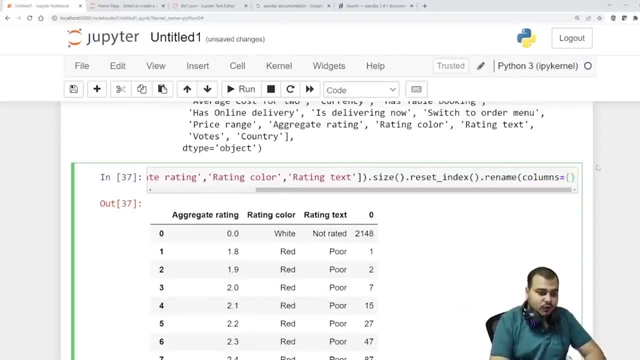 use columns is equal to, and i'm going to name it to 0 colon. let's say i'm using rating count. now let's do one thing. now see what i've done. after doing reset index, i'm using rename function and i'm saying: wherever the columns is 0, change it to rating count. 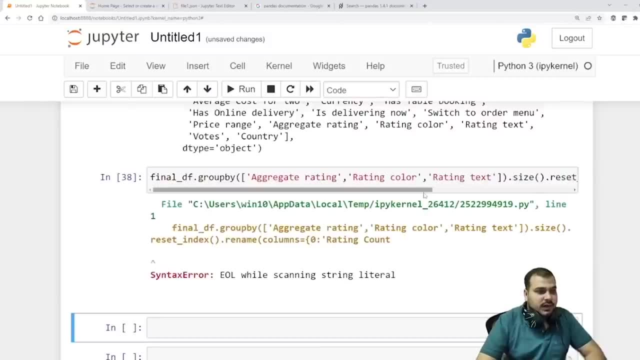 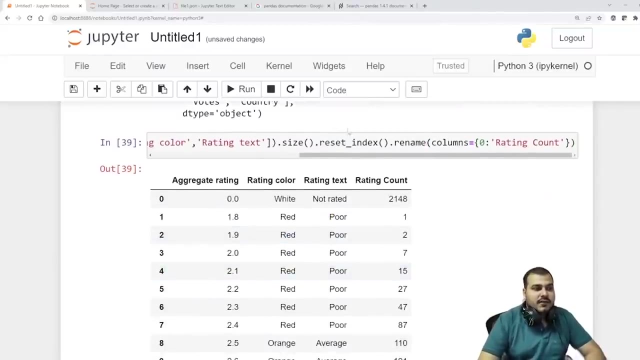 so once i execute this, you can see that i'm getting one error because i've not closed it. i will close it now. so here i've closed it, and here with this, and now here you can see that i'm actually able to see this. everybody, you just write down this: 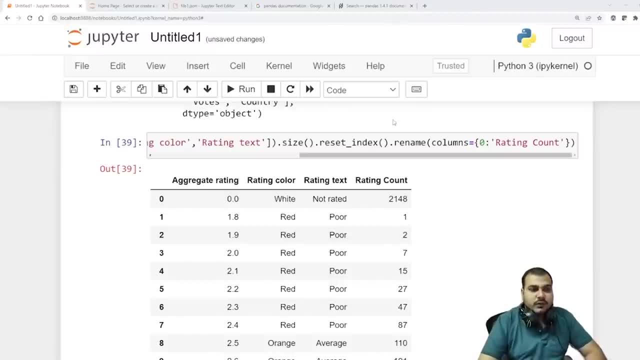 code. i know many people will get stuck over here now we'll we'll do multiple things with respect to what are the important information that i'm actually able to get from here. are they correlated? we'll try to find out. don't worry, right now i have still not gone into correlation. 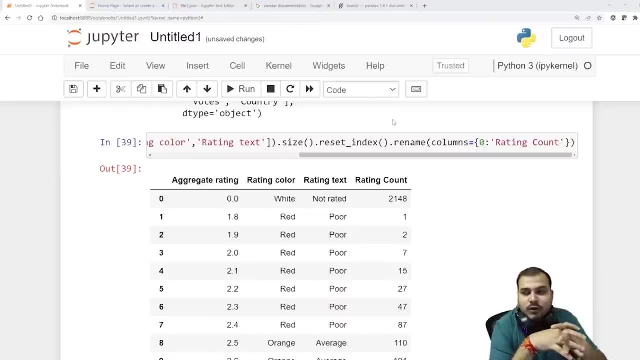 those are some inbuilt directly. you're using inbuilt. i don't want to go into inbuilt right now. now over here, main features: everybody has written this final underscore: df, dot group by: aggregate rating rating, color rating, text dot, size dot. reset, index, dot. rename columns: you are renaming from 0 to. 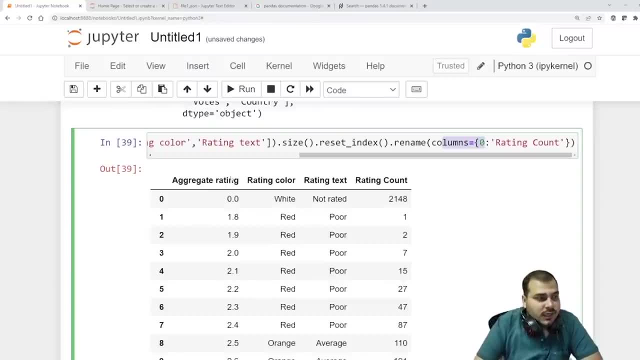 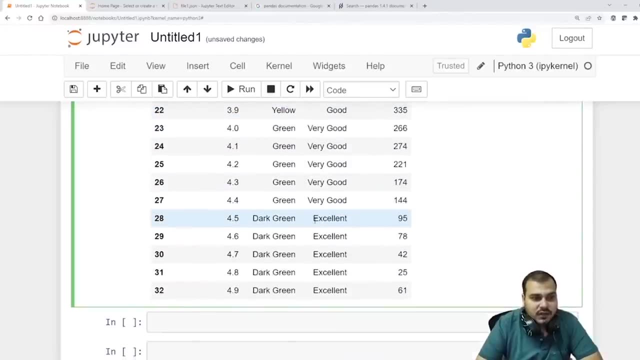 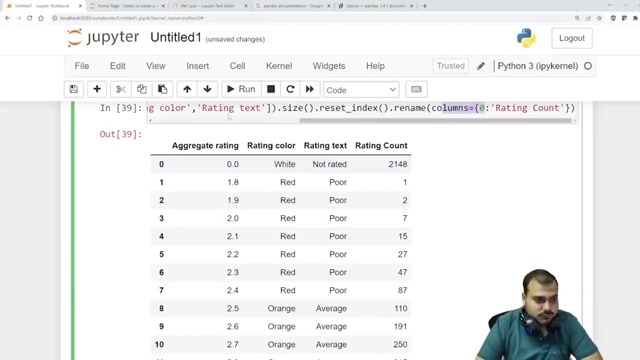 rating count. so here you can see that aggregate rating is there. rating color is there. rating text is there. rating count is there. so all these informations you have with yourself, right? all these amazing information you have over here now, let's go to the next step, now what i'm actually going to do. 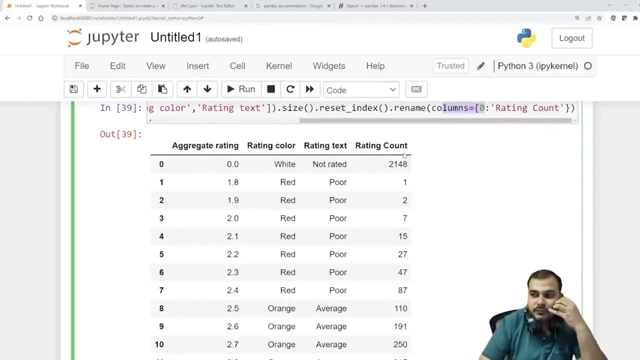 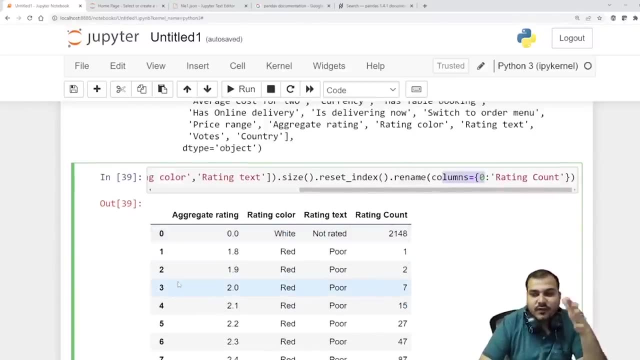 over here is that i have my rating count information. reset index basically means it will just reset this index, this index, by default. whatever index is coming, you have to reset that. so i hope everybody has done this now. i will just save this in a variable. this variable will play a very important role, guys now, so i'm i'm giving you another one. 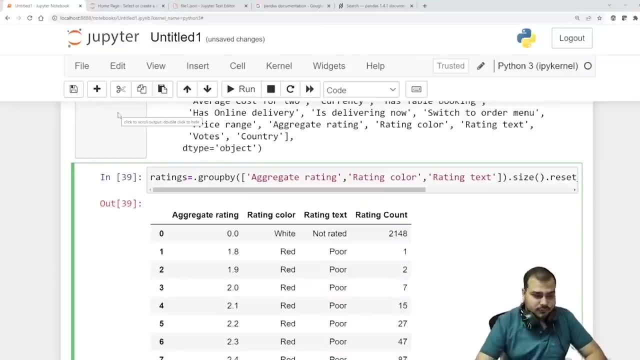 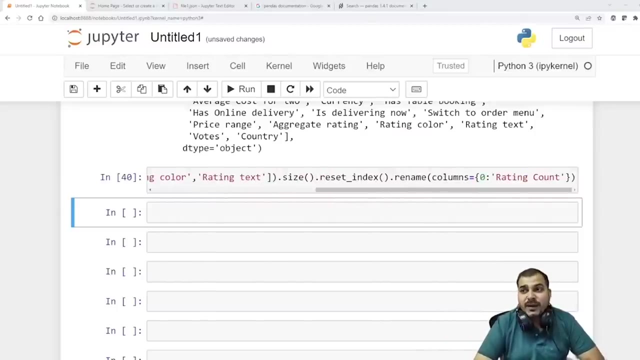 minute. please write it down so ratings is equal to this one. df. final underscore: df: dot. guys, please write it down. if anybody is not right written down, then again i'm going to share it to you here. please write them down, this particular code, because it will be very much important. 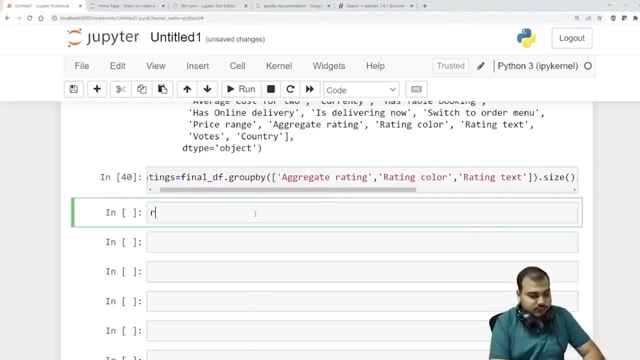 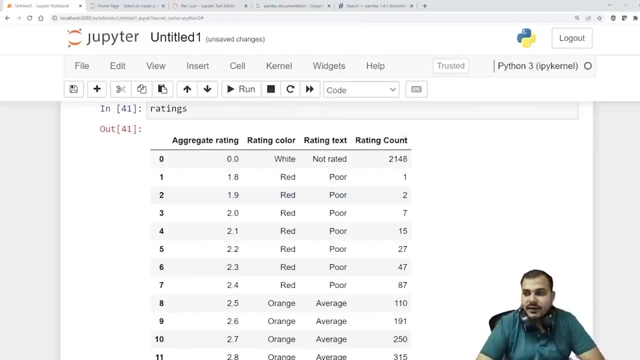 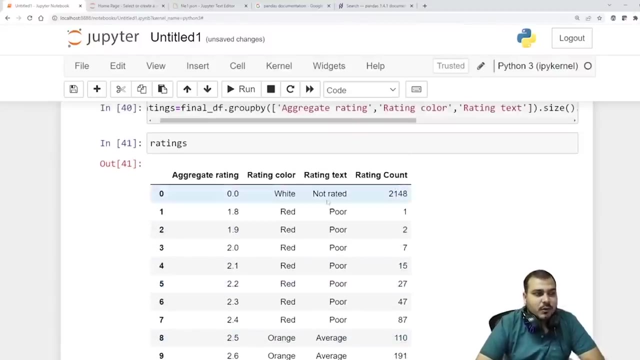 now i have all these things, if you go and see ratings. so here you have all the values: average rating, rating, color rating, text and writing. now let's go ahead, let's go ahead and let's plot some amazing, beautiful diagrams. now i want to really find out. this all relationship with 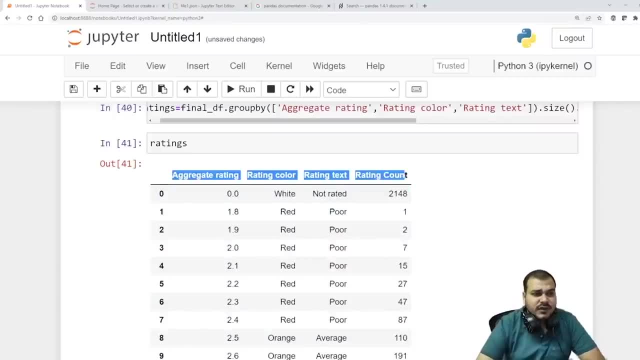 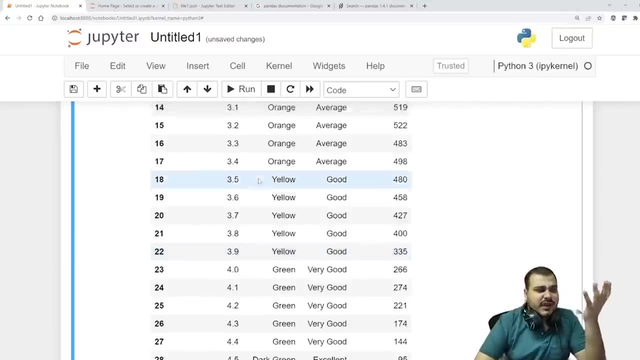 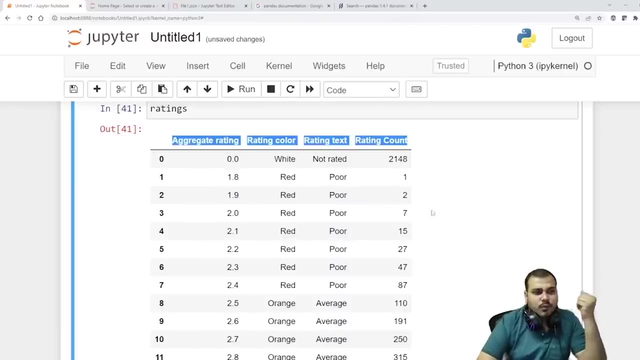 respect to different, different countries, with respect to different different problem statements, with respect to this: how see, how? as a data analyst, data scientist, you have to think: okay, this is my data set. okay, probably, what, what type of visualization i can draw from this because i want to do some kind of edn? okay, what, what kind of things i can do just by seeing the data i can. 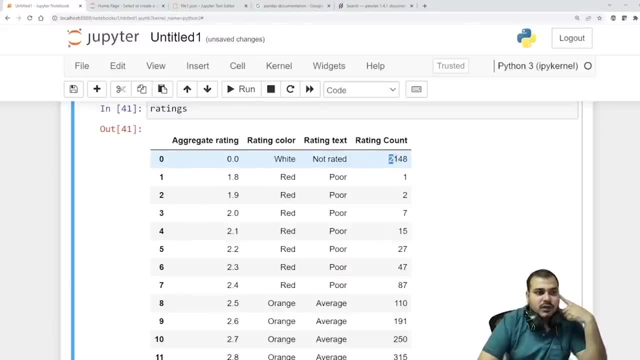 definitely come up with. one conclusion is that around 2148 ratings have zero rating. maximum number of people have actually given zero ratings. that basically means they have not rated the app or the entire zomato app. it's just a random thing and i'm afraid they don't get the same rating for. 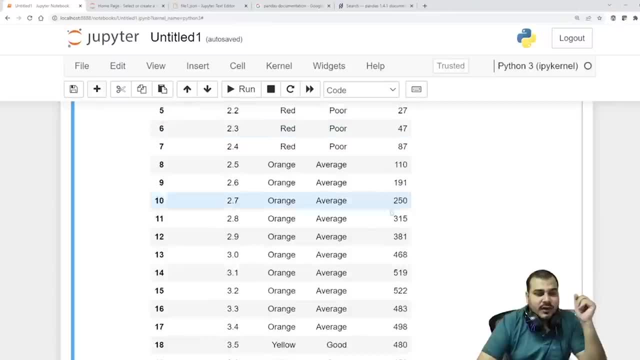 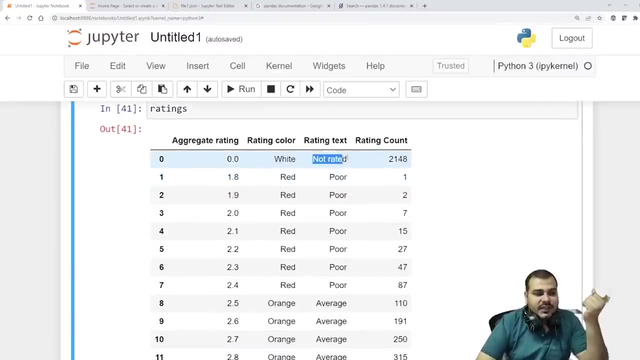 itself, right. so here what we are focusing on. we are trying to understand, okay, maximum number of ratings: zero basically means person has not given any ratings, right. so here you can see rating text is not rated right. people who are giving ratings: you can see poor, average, good along with that. 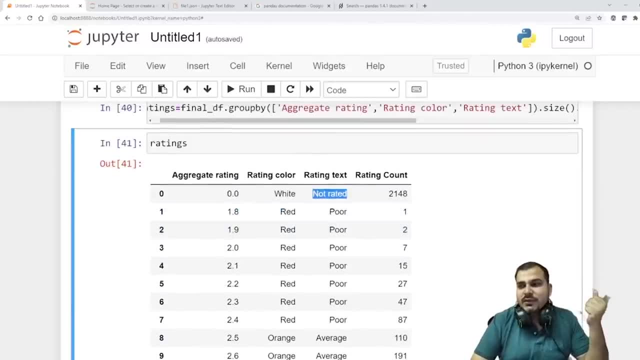 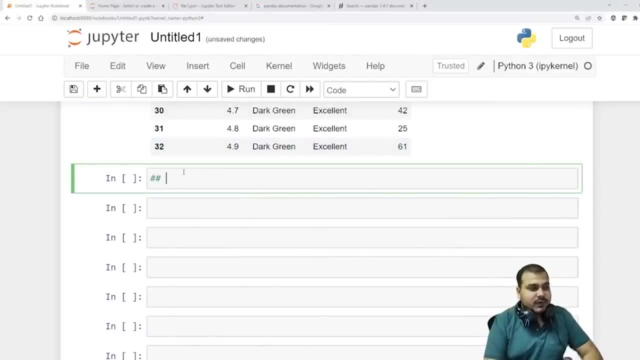 colors are also given. so can we plot this in an amazing way so that we can understand in a visualized way also. so let's go ahead from this. i can come up with conclusions again. i'll write conclusions. conclusions is very much important. observations- i can also say observation. 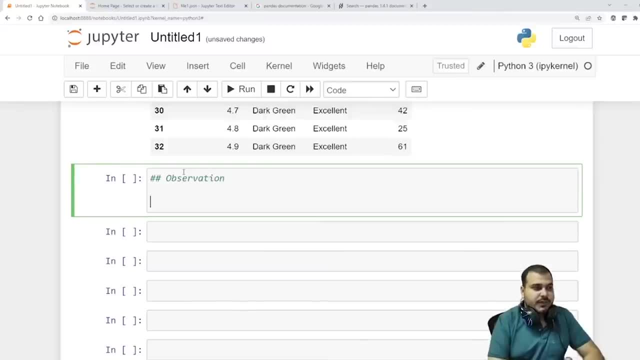 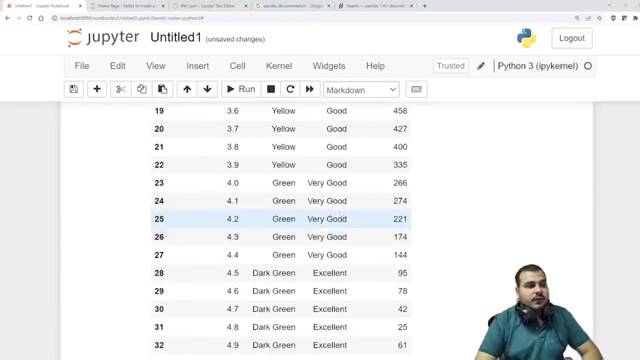 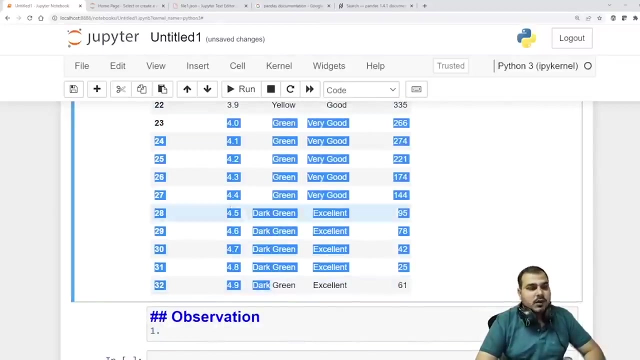 so this is my observation from this data set. the first observation is that. the first observation is that whenever the rating is from 4 to 4.9, or let's say from 4.9 to 4- sorry, 4.5 to 4.9. so here i'm going to write the observation. 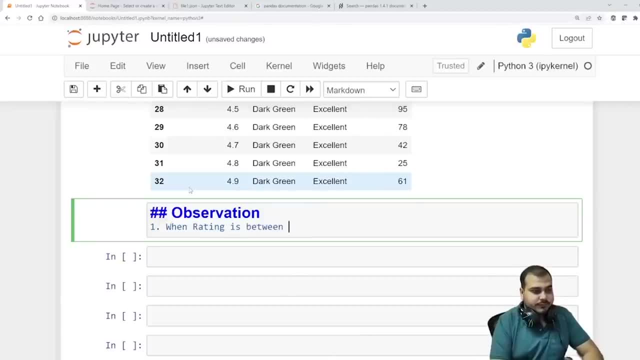 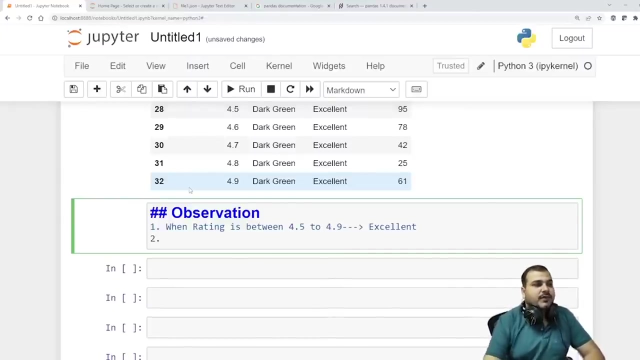 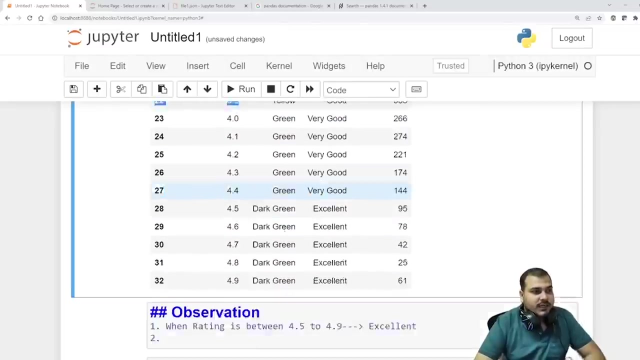 when, when, when the rating is between 4.5 to 4.9. this indicates. what does it indicate? it indicates that it is excellent. probably the foot that was delivered was basically excellent. second thing that we can come up with this observation is that here you can see that from from 3.5 to 3.9, when the rating when, 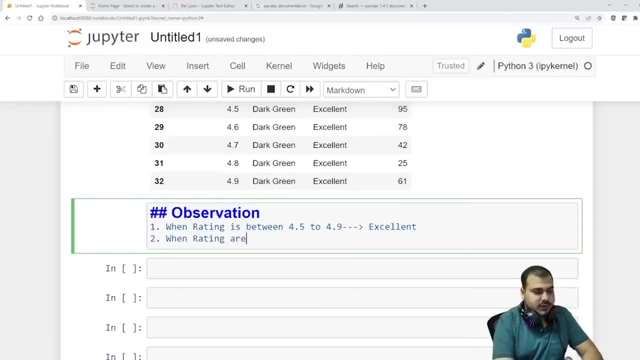 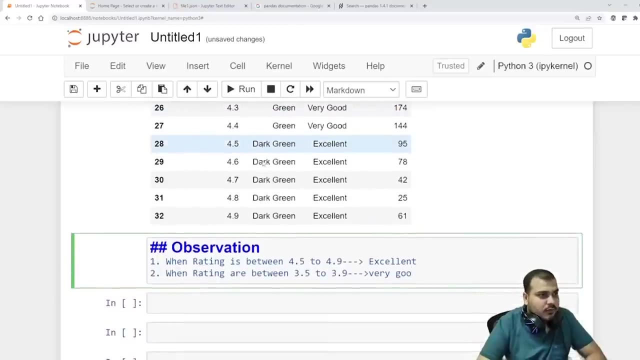 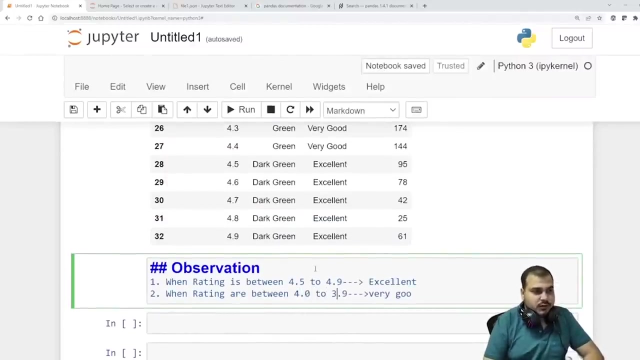 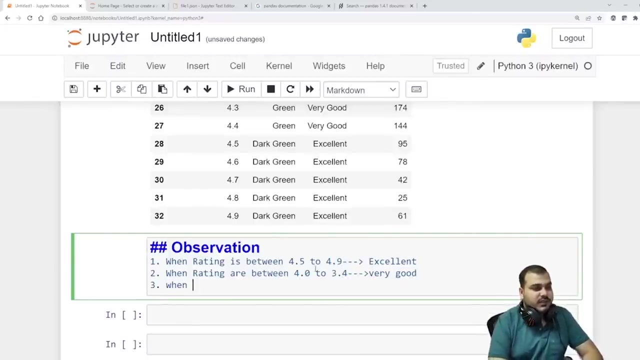 when ratings are between 3.5 to 3.9. here you can basically say that it is very good. i have 3.9, only right. no, 4.0 to 4.5. excuse me, sorry, i missed that. 4.0 to 4.4, the ratings are very good. the third thing that i can come up with this there that 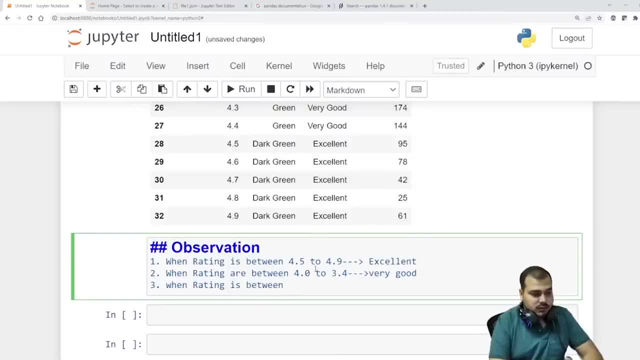 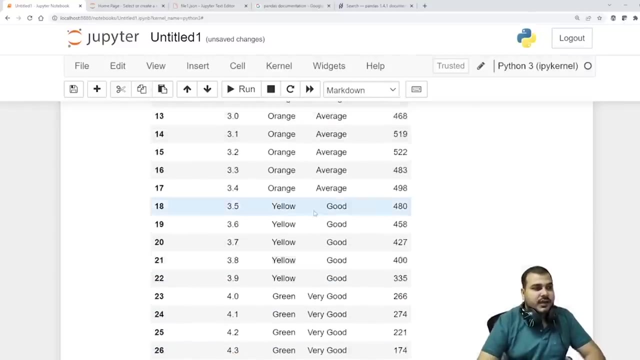 If the rating is between 3.5 to 3.9, here the rating is good. So this is my observation, because I can definitely see from the data right And remaining all. please go ahead and write it down, okay. 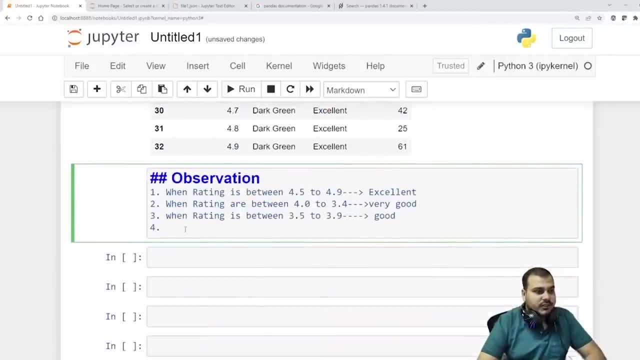 So another observation: from 2.5 to 2.9, it is average, So I am just going to copy this: So 2.5 to 3.0 or 2.9.. Wait, wait, wait, wait, wait. 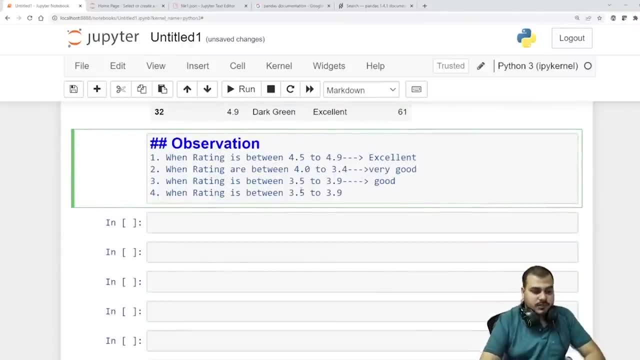 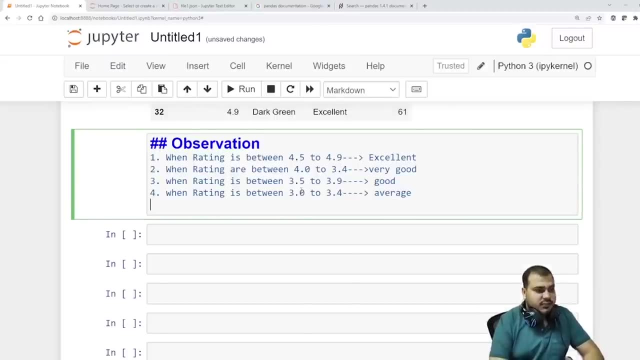 Average. 3.0 to 3.4 is average. So 3.0 to 3.4 is average. So this is my next observation. And fifth, I will go ahead and write When the rating. sixth, I am going to write. When the rating, when the rating is between 3.5 to 3.9,, it is between 2.5 to 2.9 and it is 2.0 to 2.4,. right, So 2.9,. how much it is? 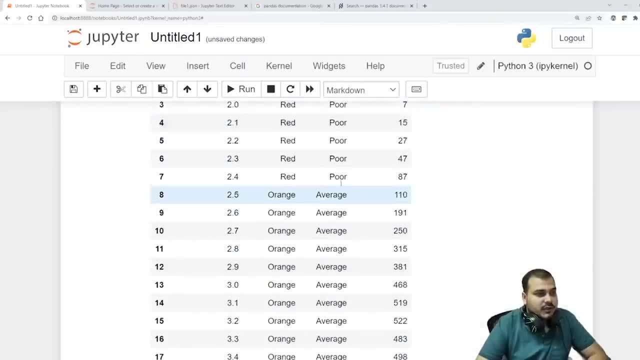 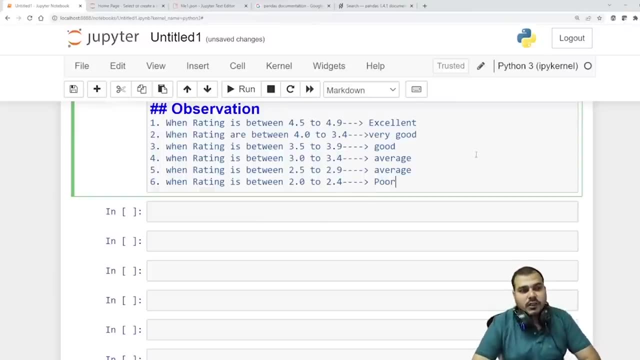 Average. again, this is also average. 2.0 to 2.4 is poor right. So these are some of my observations. Just complete down all the observations that you can find out from this. And one more thing that you can see: that 0 rating has been given by many of the people. 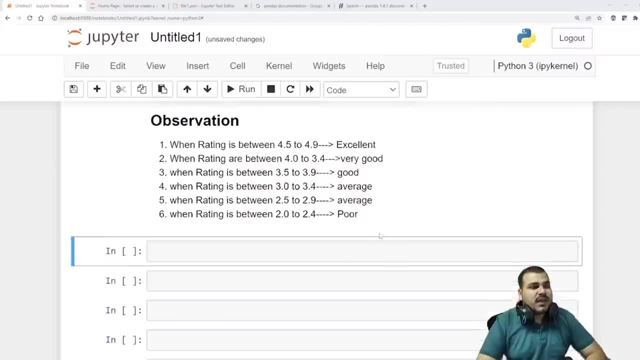 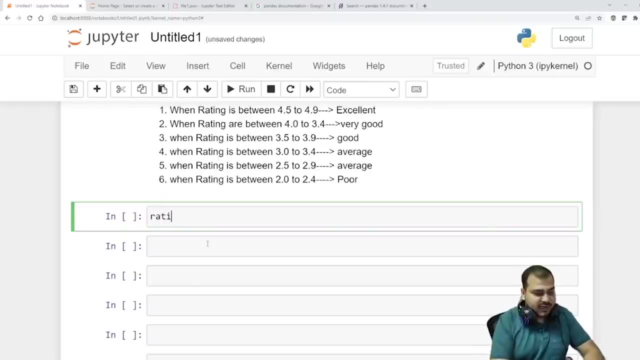 Right. So these are all my observations with respect to this. But if I am writing observation, it is better that we also draw some kind of diagrams. Now, here I am going to basically draw a diagram. So this is my ratings. So here I am going to use aggregate rating. 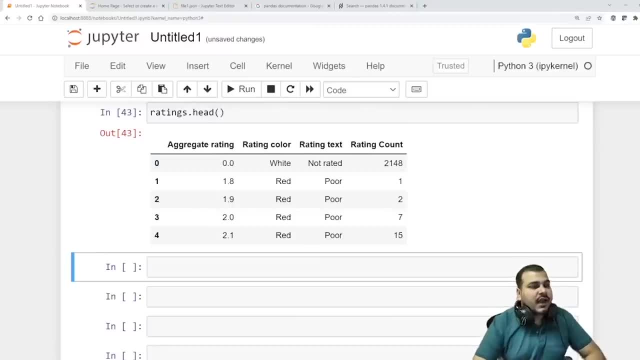 Let's say that this is my ratinghead. So here I have aggregate rating rating, color Rating, text rating count. So I am going to use now Seaborn bar plot. Let's see, can we visualize, with the help of bar plot, something in this? 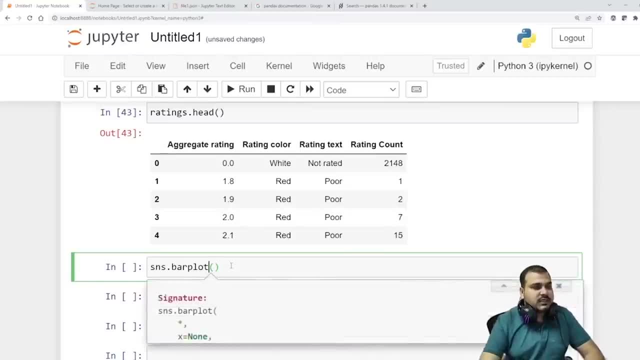 So here I am basically going to use in bar plot: always understand what all features you have. So here you have X, Y, we data order, we order. everything is there. But what I am going to do, I am just going to do a simple bar plot. 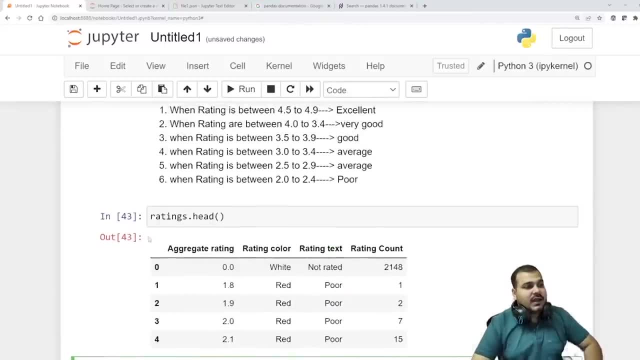 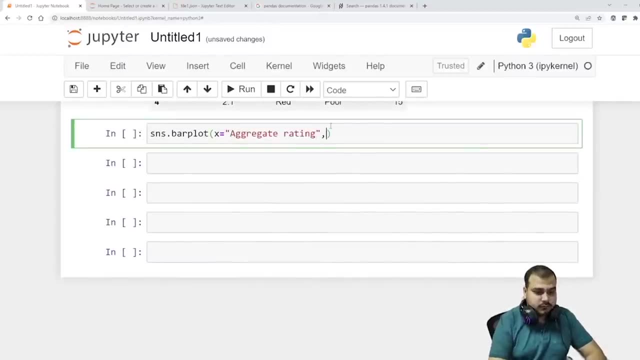 So here in the X axis, I am going to basically use aggregate rating. So I am going to use aggregate rating. In the Y, I am basically going to use rating count. Let's say that I am going to see the relationship between aggregate rating and rating count. 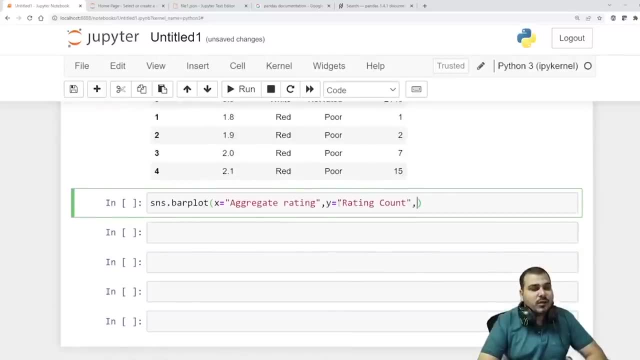 See, this is my aggregate rating and this is my rating count. I want to basically draw a bar plot and basically check how the graphs look like. So the third parameter here I am going to basically use data is equal to ratings, So 1x2.. 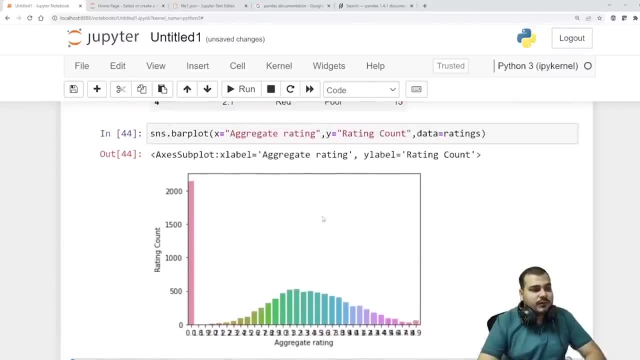 So 1x2.. Once I write this and execute it here, you can basically check out how beautiful it looks. Now the diagram looks smaller. so what I am actually going to do, I am just going to put one simple settings to increase the diagram so that you will be able to see it in a better 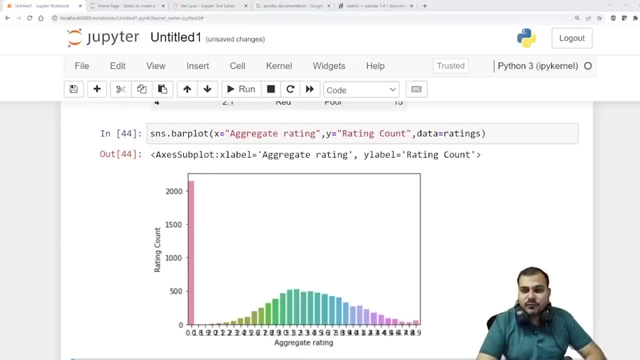 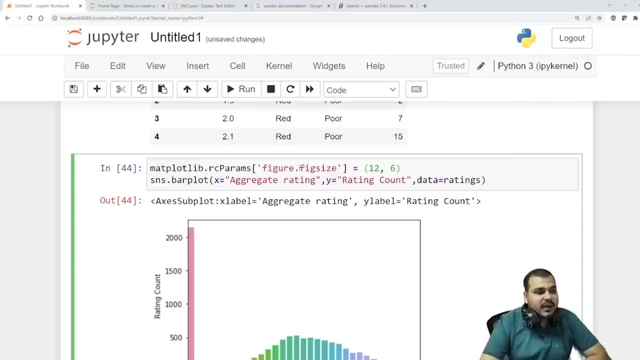 way And that settings is basically there in the matplotlib. So I am going to use something like this. And there is another setting which is called as matplotlibrcparamsfigurefiguresize. Here you can give with respect to width and height. I am now giving 12.6.. 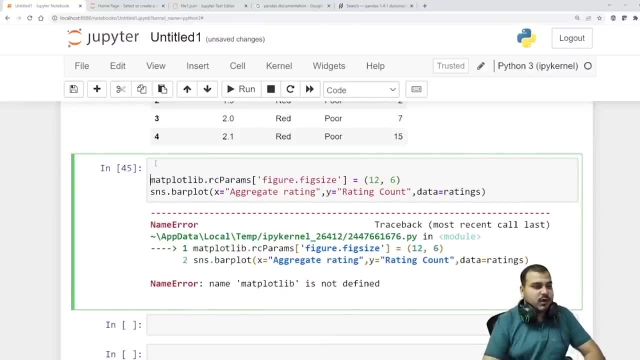 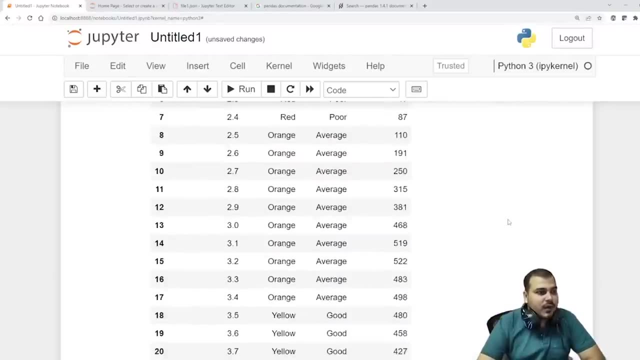 So here, matplotlib: ok, import matplotlib. I am just going to write it down. So now here you can see the diagram looks quite bigger. Now, if I probably go and execute the heatmap over here again, let's see whether it will change or not. 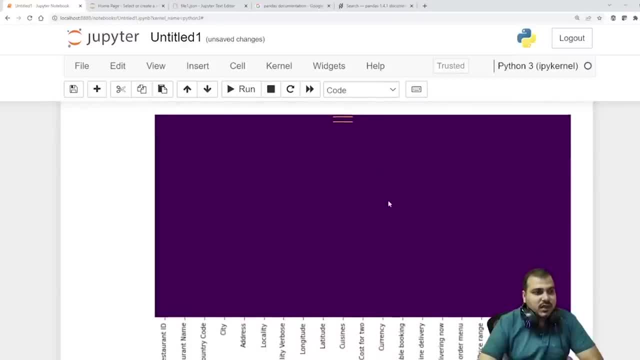 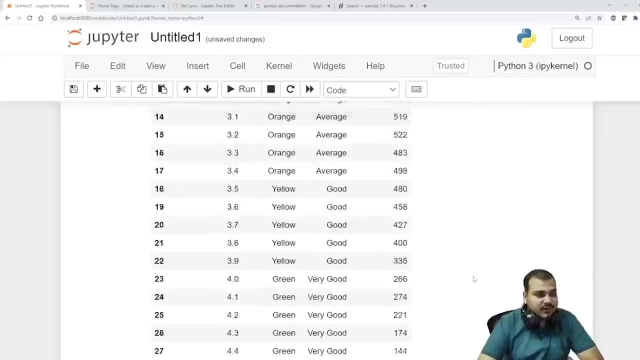 So now you can see these values, right, the missing values. Once I made the diagram little bit bigger, you can see this. I have done it Now. what is this? This missing code that we have missed with respect to increasing the figure size? 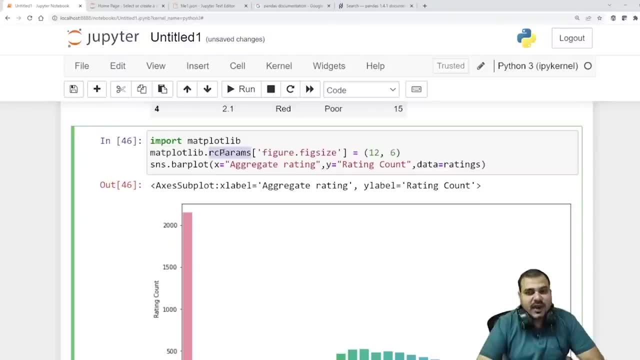 Just write matplotlibrcparams. So, with respect to any parameter that you want to change, you can basically use this. Here I have set it to 12.6.. Now, once you see this diagram- from this diagram, you can definitely find out a lot of information. 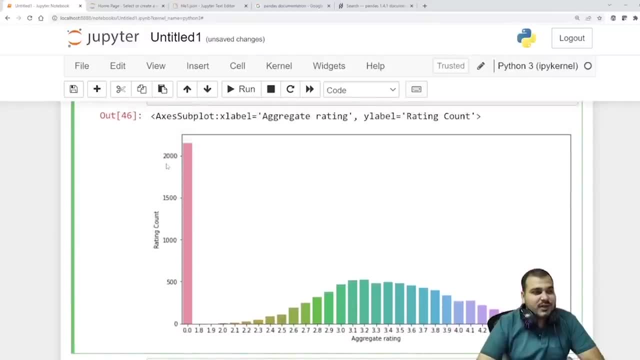 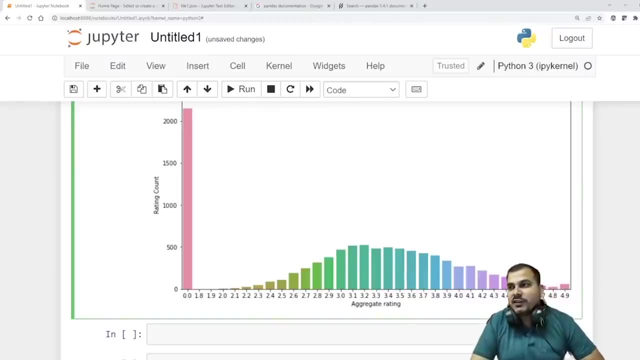 This diagram looks super cool. Zero rating is more than 2000 over here. Then you can see 2.2,, 2.3,, 2.9, complete. It looks like a Gaussian curve, right? Whenever you have a Gaussian curve, you get a good sense of feeling. yes, 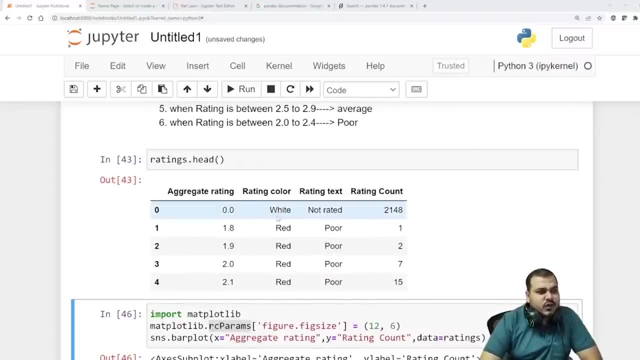 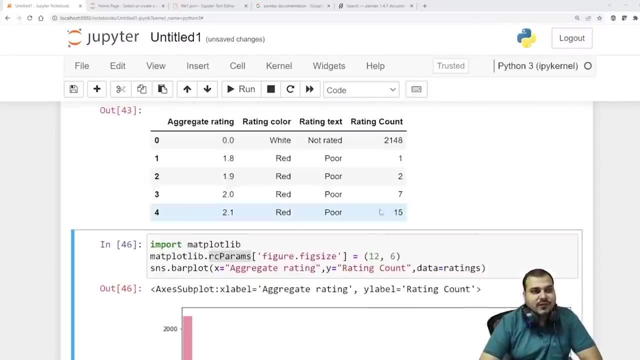 Now let's do one thing over here. you can see that rating color is also there, So it is always a good way that we should also color this aggregate rating with the help of colors that is given over here. So this is the code. everybody write it down. 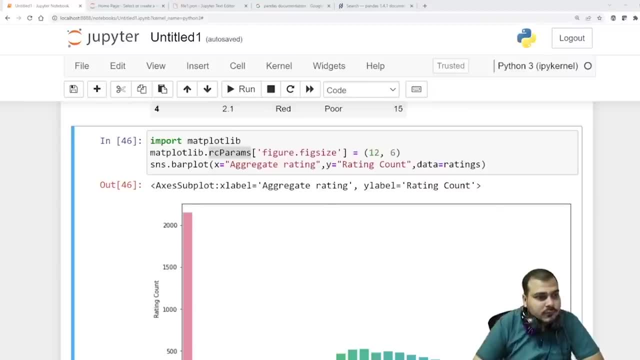 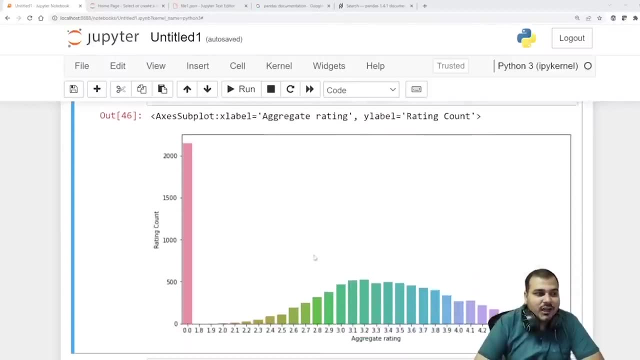 X aggregate ratings. Y rating count. Now, as I said, ok, I have written it down. I have written it down. Ok, I have this coloring text rating color. I have this white, red and all. Should we use this colors over here also and probably try to get in the form of colors? 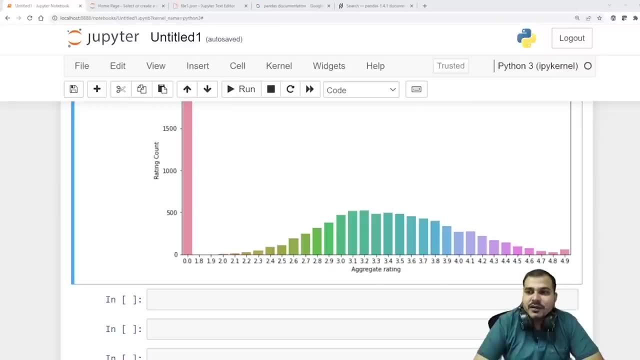 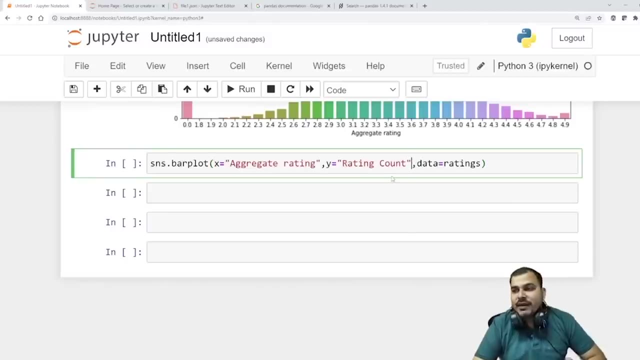 and then try to see it, So that also we will try to do it. ok, So to get the colors, what I am actually going to do, I am just going to copy the same thing entirely. There is one more parameter, which is called as hui. 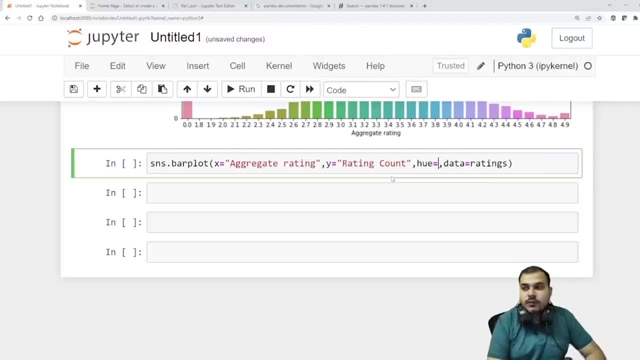 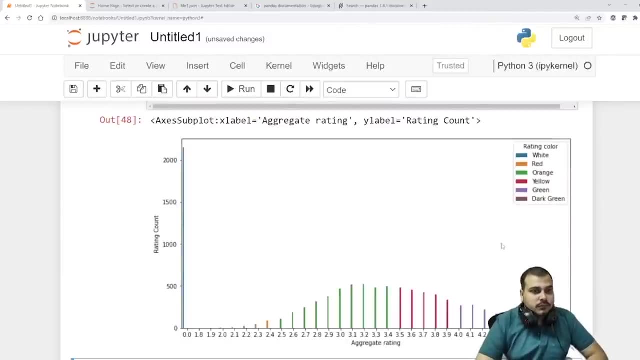 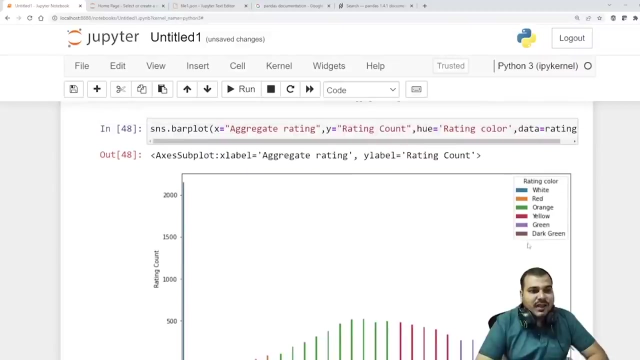 So if I write, hui is equal to rating color, If I write this and execute it, you will be able to see. see over here orange color, green color, red color and all, But understand whatever color is there. this is not matching right. 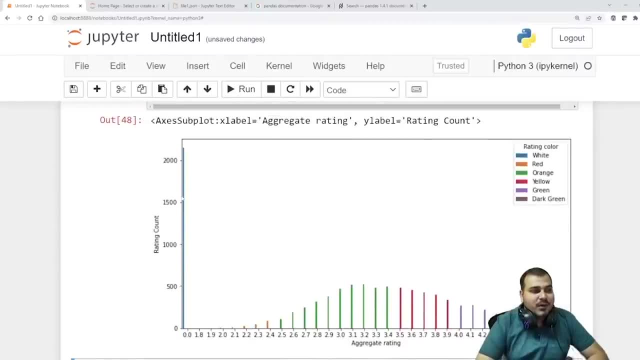 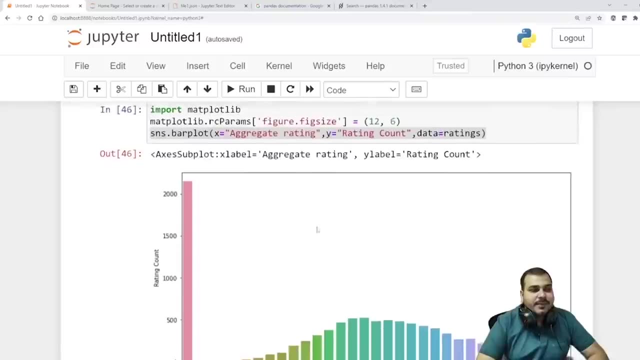 White looks like blue. So this is wherever you can see blue right. it is basically showing you zero rating, But according to this, this zero should have white color, right. So what I am actually going to do over here is that we have to map the colors also. 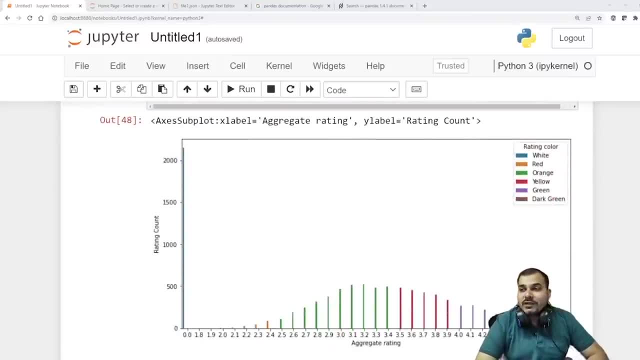 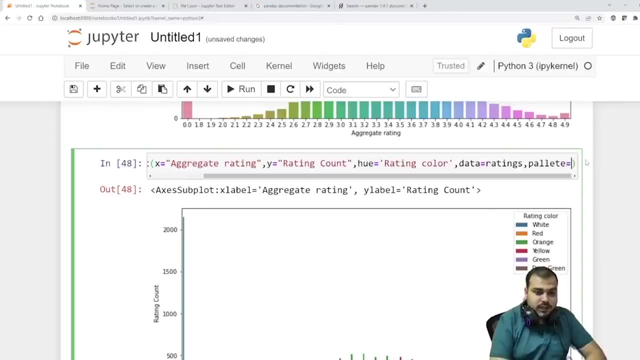 Ok, Ok, Ok, Now how to map the colors, We will try to see. So, mapping the colors, let's see over here. So mapping, I am going to basically use palette and inside this palette, I am going to basically use different, different colors. 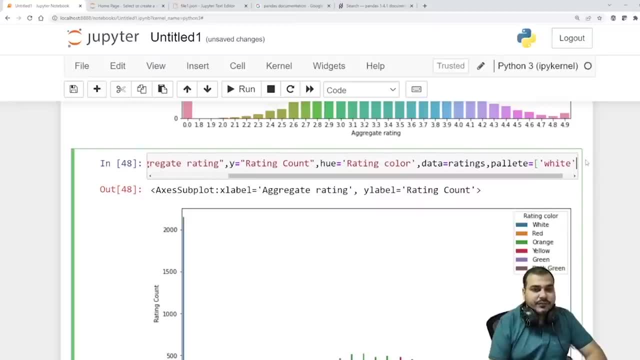 So the first color that I want to show over here is something called as white. The second color that I want to show is red. The third color that I want to show is orange. It should be in the list, ok. The fourth color that I want to show in yellow. 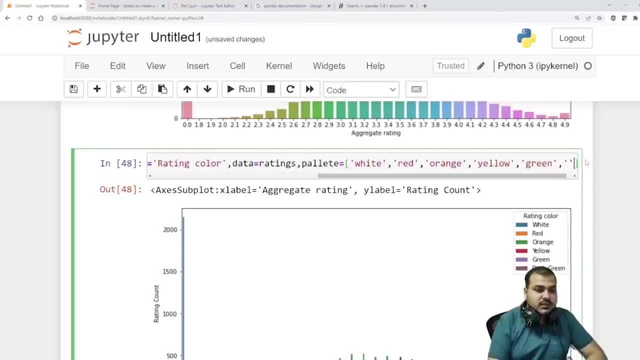 The fifth color that I want to show is in green. The sixth color also, I want to show it in green. So here is what I have written in palette. This palette is a feature that is present, is an attribute that is present in barplot. 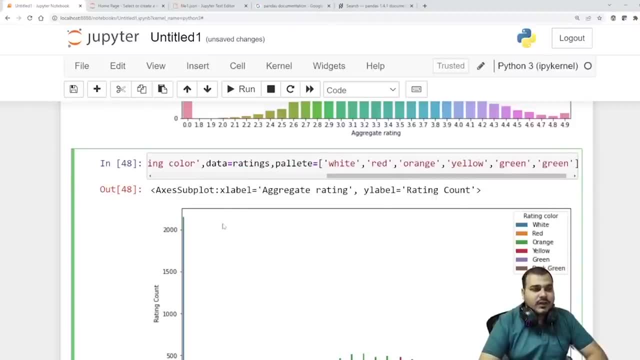 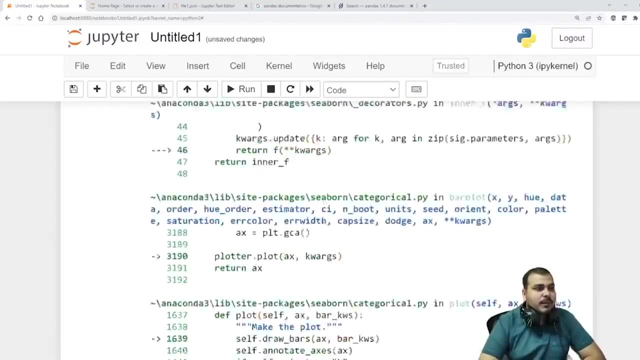 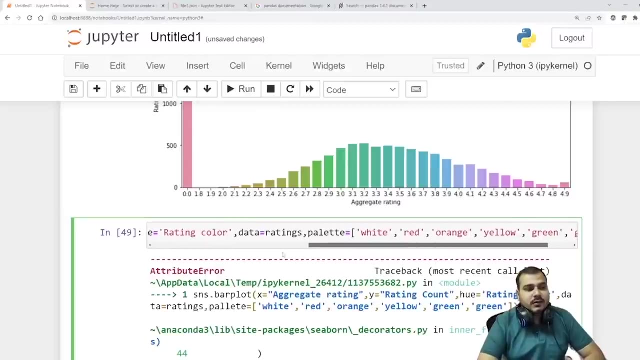 where you can give your own colors as it is required, based on your requirement. So once I execute this, now let's see some error is there. has no ok palette. spelling is wrong. I guess It should be tte: p-a-l-e-t-t-e palette. 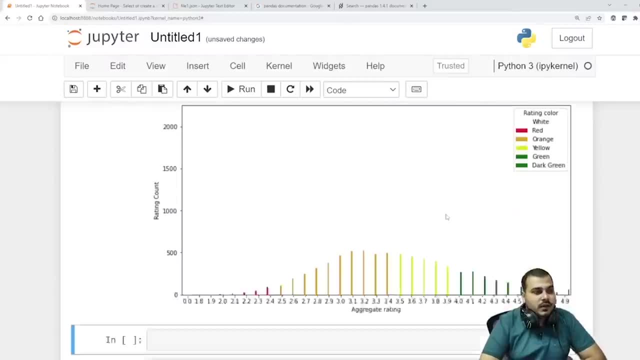 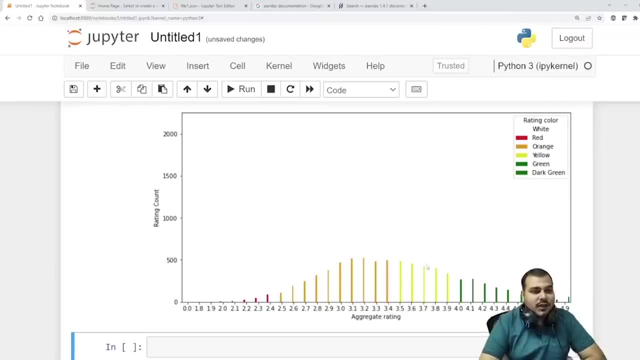 So once I execute this and let's see now- So now you can see that I am getting the perfect color right: White is white, then red, then orange, then this, then this, then this. Now from this also what kind of observation you can basically get right. 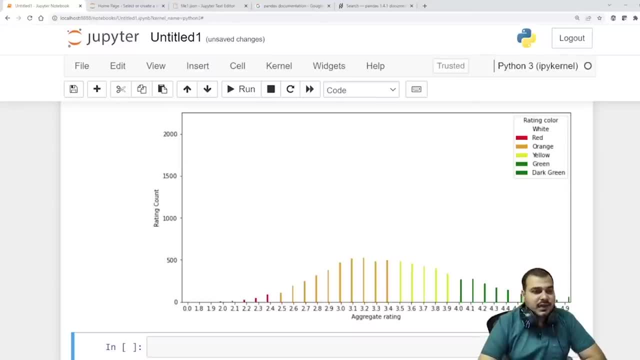 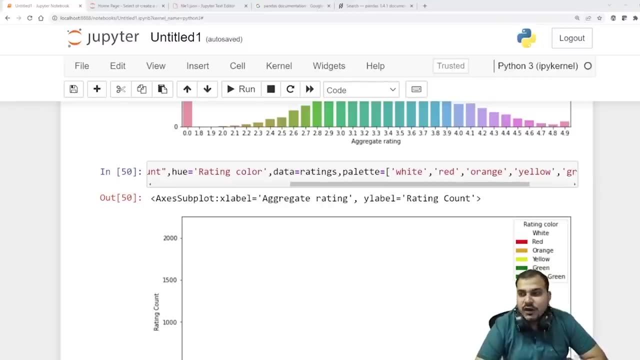 What kind of observation? Maximum number: see. I will again write observation. First of all, you write down the code, Everybody, you will be able to see that I'm getting the colors. but just go ahead and write down the code and quickly see that. what type of graphs we are able to get over here. 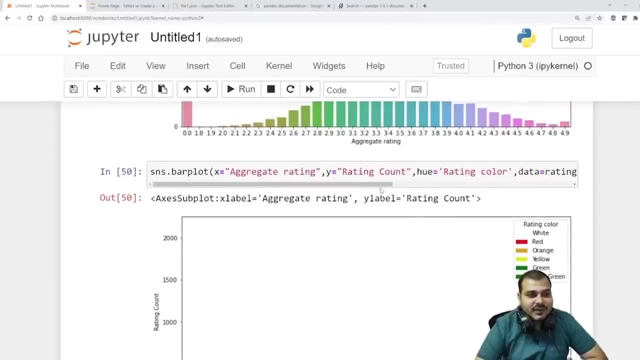 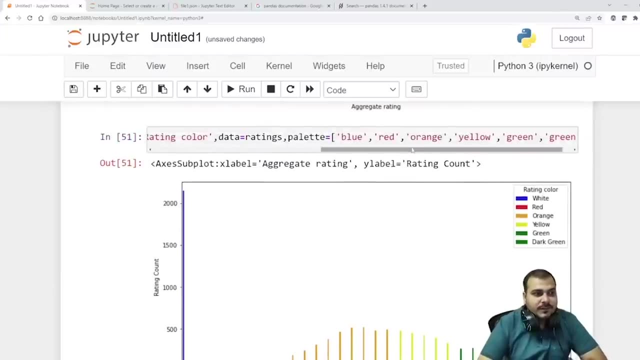 White is invisible, Don't worry, That's fine. You want to make it in different color? then make it instead of white, use it blue. Now, here you have this right Now. from this, what kind of observations we can actually get? 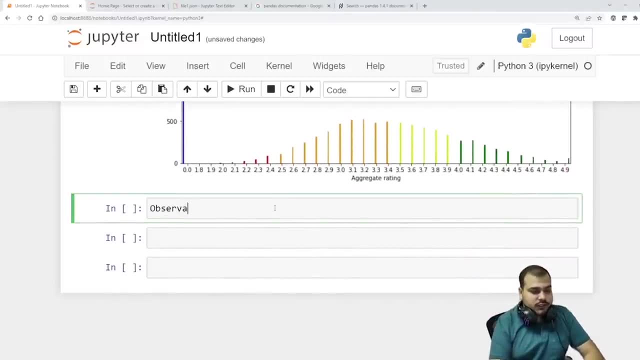 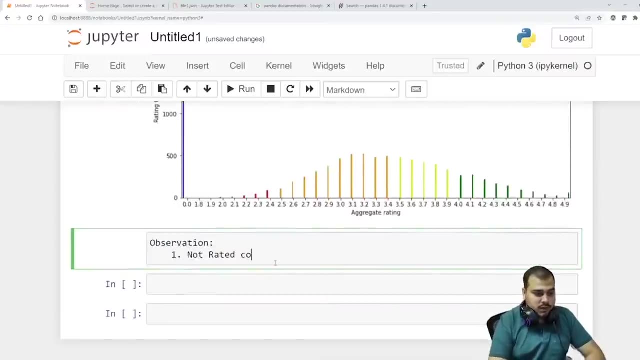 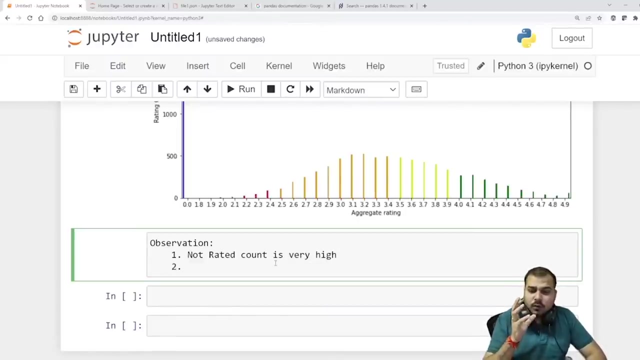 So observations, I'll write it down over here again. Observation: First observation that I would like to make: not rated basically means this blue color Count is very high. Then the second thing is that now, second observation- that you can see that maximum. 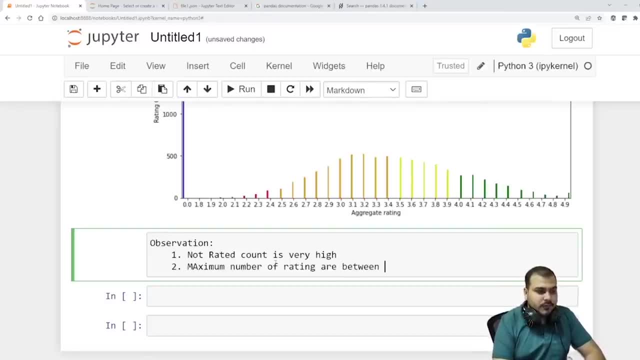 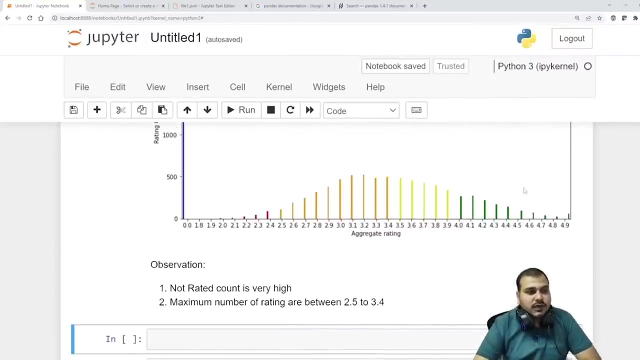 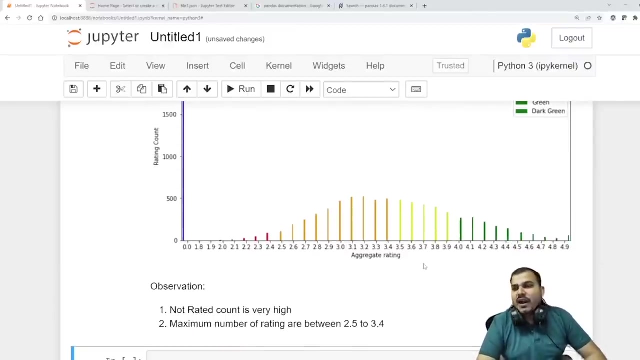 number of ratings are between 2.5 to 3.4.. Max number of ratings are between this. so definitely these two observations. you can basically find it out. this two observation you can definitely find it out. clear, everybody, these two observations, we can basically find it out. now, just imagine that if you have some ratings as missing, then what do? 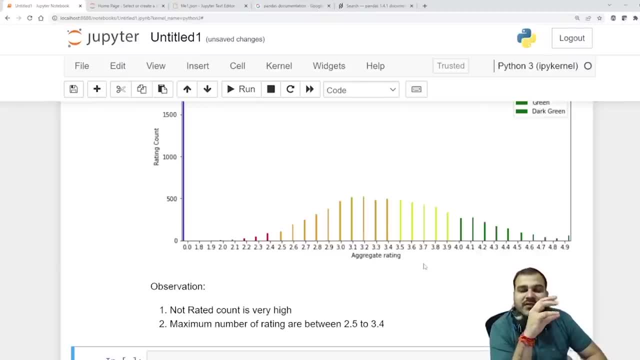 you do suppose, let's say, that a person has rated, but you have some missing values. now, can't you think that now, probably, you can use the values between 2.5 to 3.4 as an average, right? so this is what type of observations you can basically have. this is what? because maximum number of 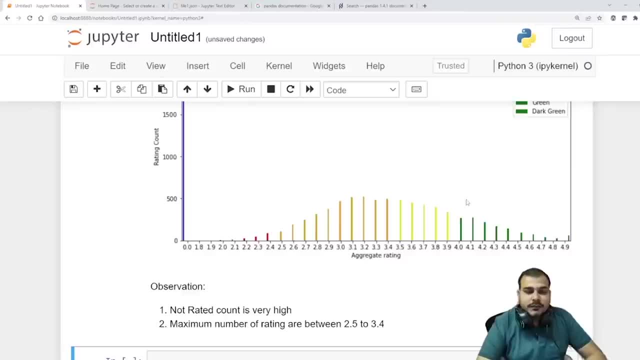 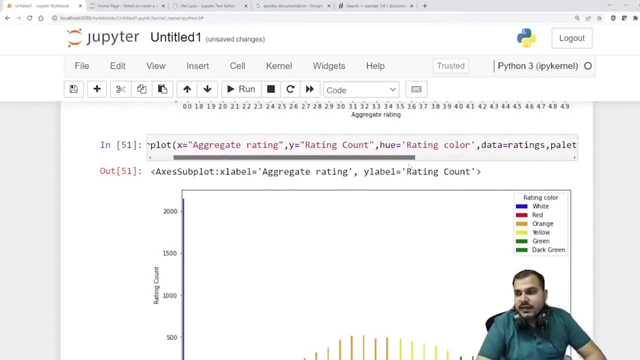 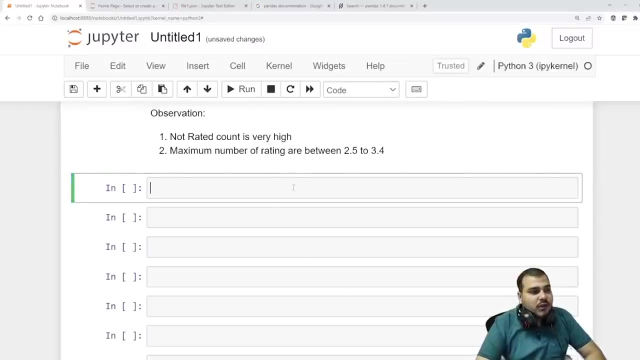 observations, or ratings, are between 2.5 to 3.4, so you will try to find out the average between them and then try to get it. so i hope you're having fun, guys. clearly you are able to understand now the next step we will also see. right now we have just seen with respect to aggregate rating. 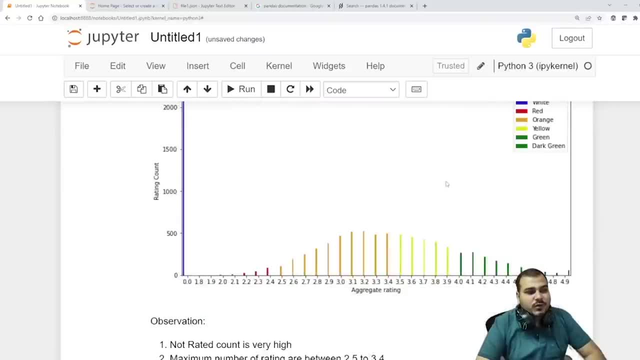 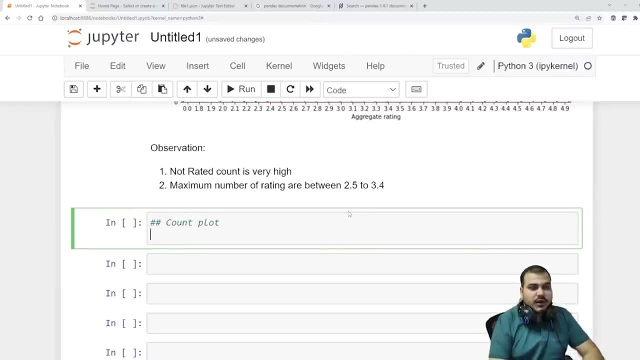 and rating count. i probably also want to use, with respect to just the coloring part, this rating color. i want to plot this as a count plot, so count plot, let's plot it. so i'm going to use snscount plot and here i'm basically going to use: x is equal to rating color, okay. 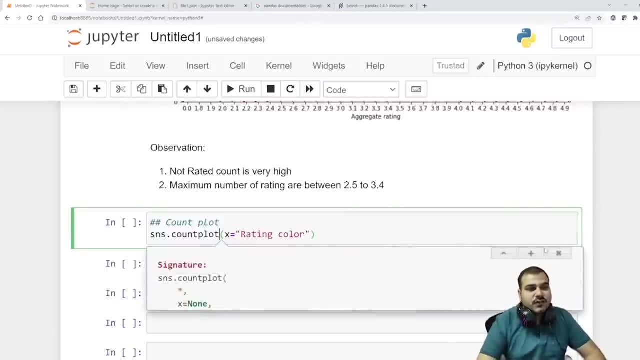 in count plot. we basically use this for plotting with respect to categorical variables. so here also you basically give an x and y value and v value. so here i'm giving x value and then i'm also going to give my data, which is my ratings, and then again i can give my palette over here. 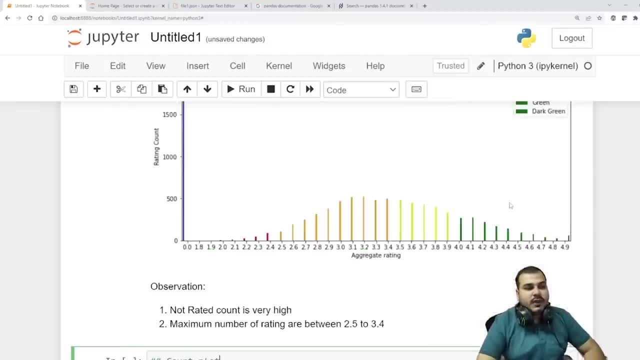 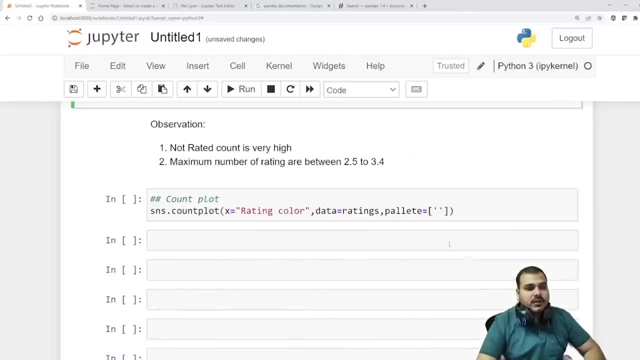 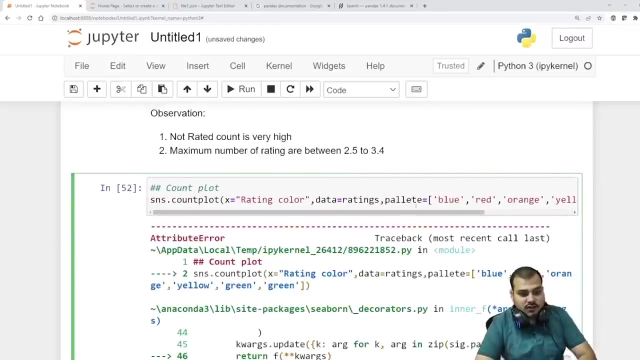 with the same list that i have actually defined over here. palette: the color should be same, right? so that is the reason i'm just going to copy this entirely and paste it over here, so once i execute it here, you'll be able to see i'm getting every time i write, the wrong spelling. 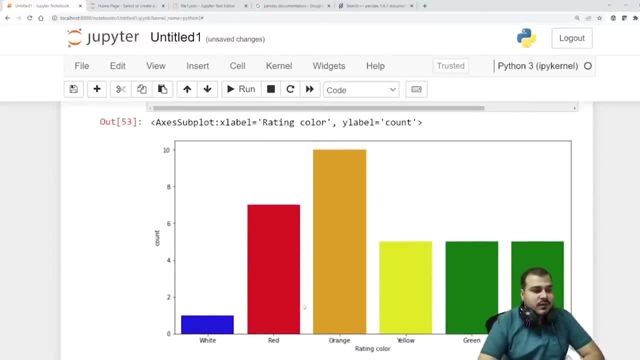 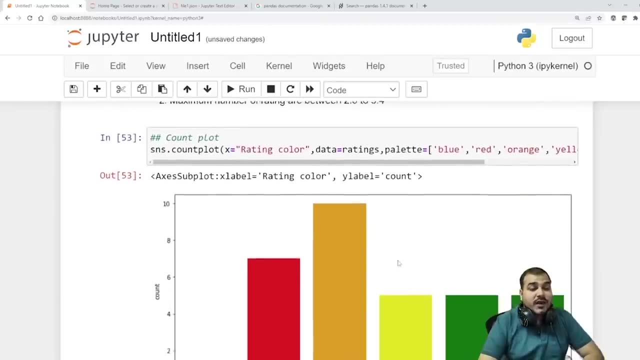 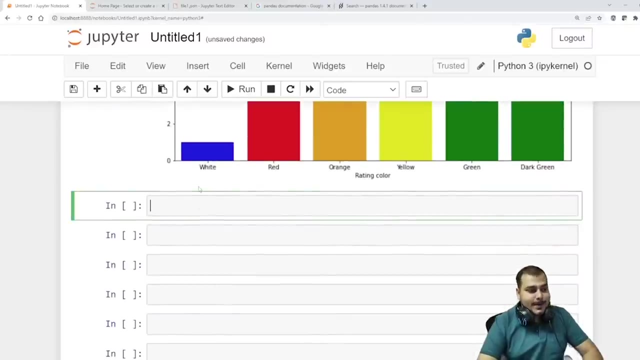 so here you can see white, red, orange, yellow green, dark green. this is with not respect to count guys, don't worry. okay, this y y axis here you are able to see over here. but understand, in rating what you have, what you have, you basically have something like this, right? so white is only. 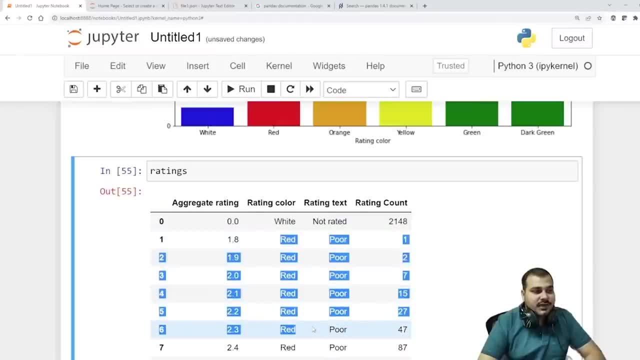 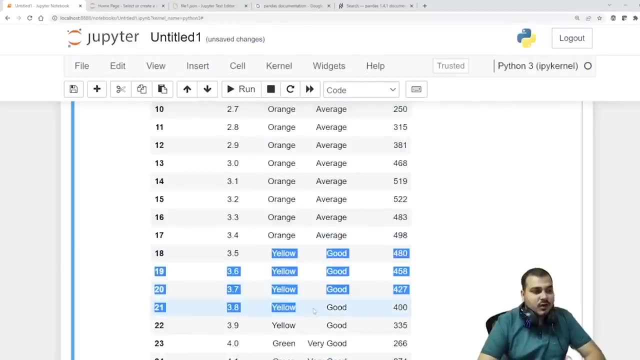 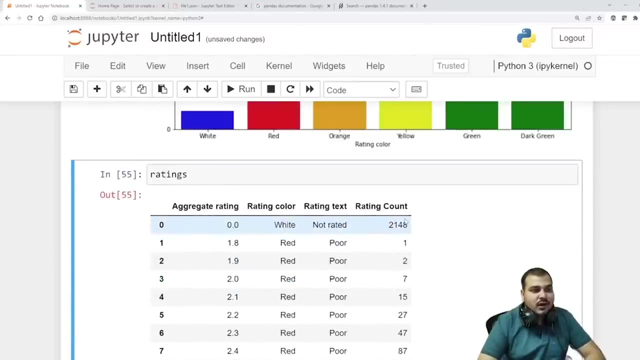 one record. red is so many records. right, this is my red, they are around five records. then orange: they are around seven to eight records right. yellow: there are around this many records. green, they are this many records. don't consider that this count is basically your rating count. no, this is the. 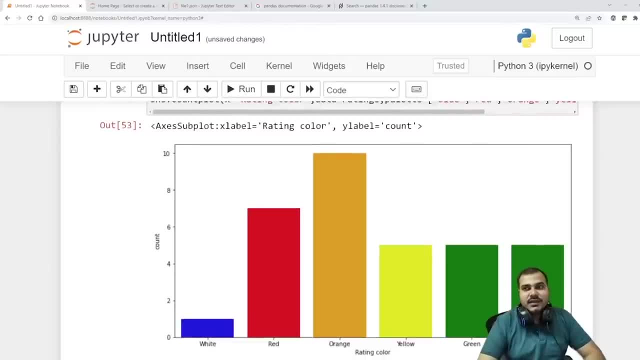 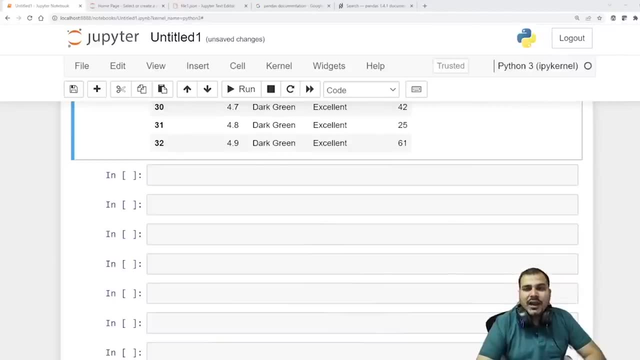 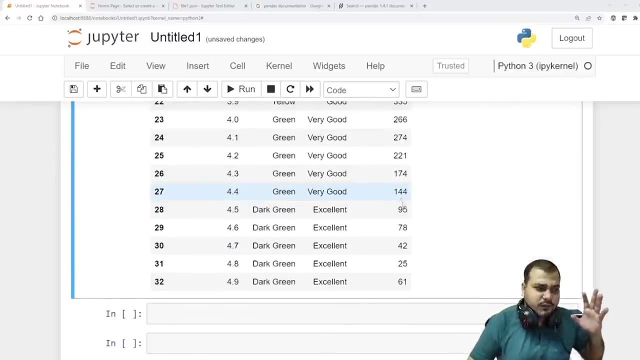 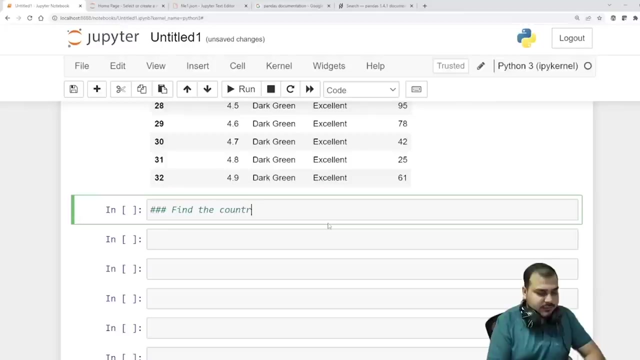 frequency, how frequently it is basically present in this uh data frame. now let's go ahead and do some more in-depth, in-depth analysis. in-depth now. you will get more confused. now i'll give you a question. please try it out from your side. okay, find the countries that has given. 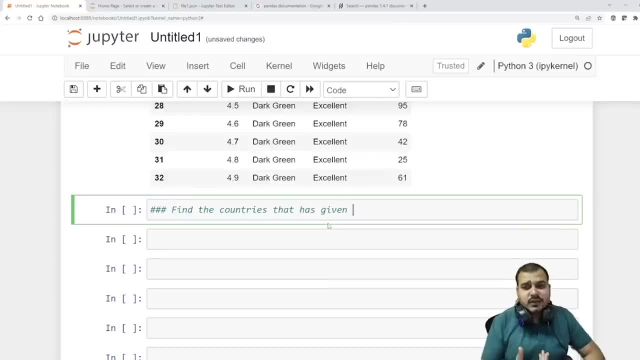 find the countries, a country name, a country's, country, country's name that has given zero rating. now this is my one of my query for you all. try to do it and i'll wait. i'll wait for you all. let's, let's try to do something. guys, you should be getting some queries at least. 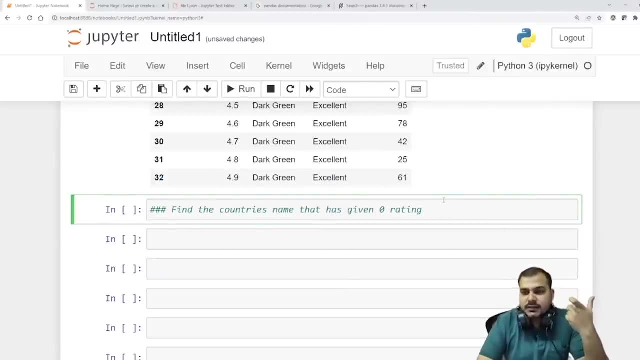 very important interview question. as a data analyst, find the country name, country's name that has that has given zero ratings. please do it everybody, i'll be waiting for you. that has given zero rating. how do you do it? you will definitely get more confused. that is where a data analyst will. 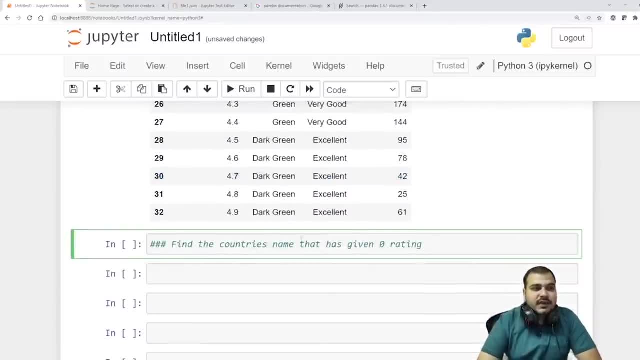 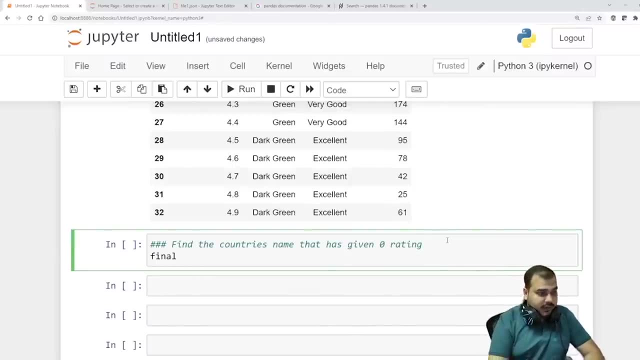 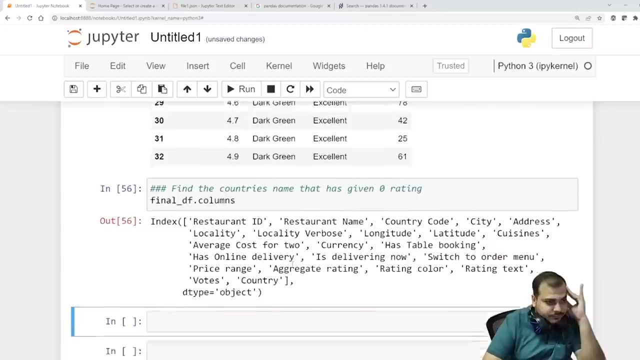 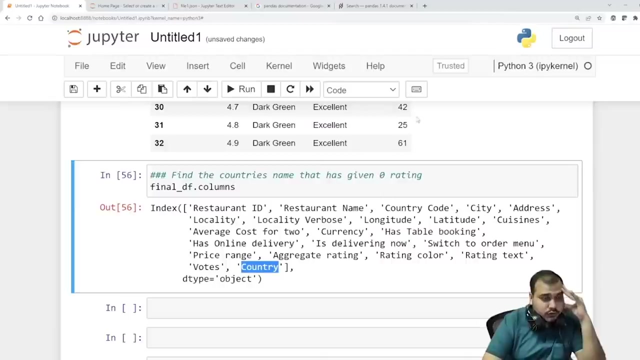 come find the country's names that has been given that has given zero rating. i'll also try till then. final underscore: df, dot columns. so i need to basically get all the country name. so country name is obviously there, okay, and those who are given zero ratings, if zero rating is there. 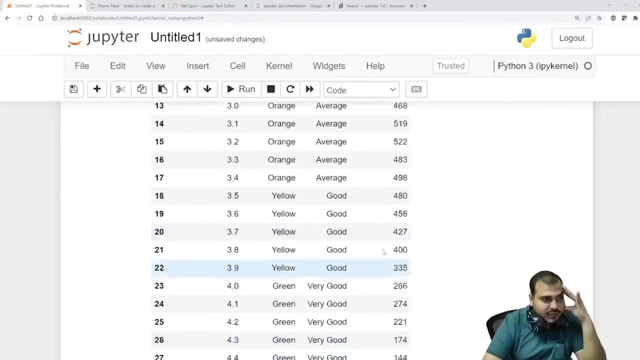 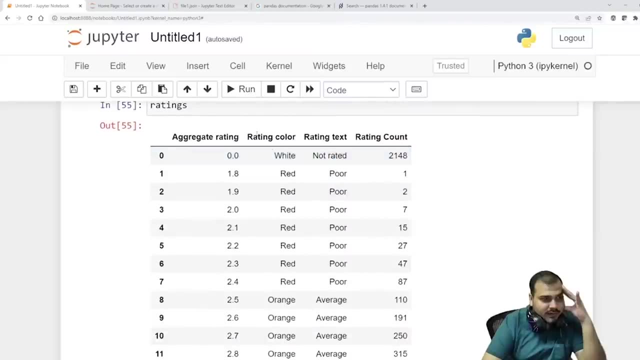 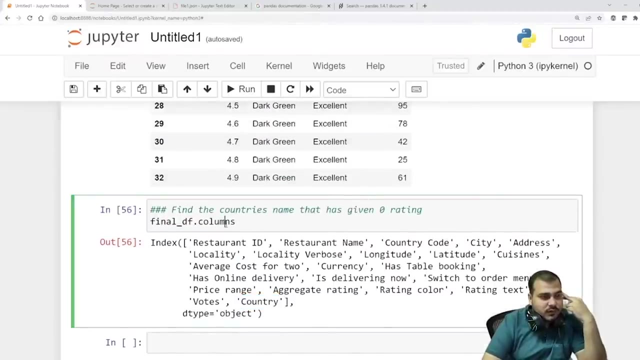 probably i can identify with zero ratings, i can identify with aggregate rating, or i can also identify with rating color. okay, so two parameters i can definitely find out with. so what i'm going to do over here is that i'm just going to say rating color. let's use rating color. rating color, if i say if the rating color is equal to white. 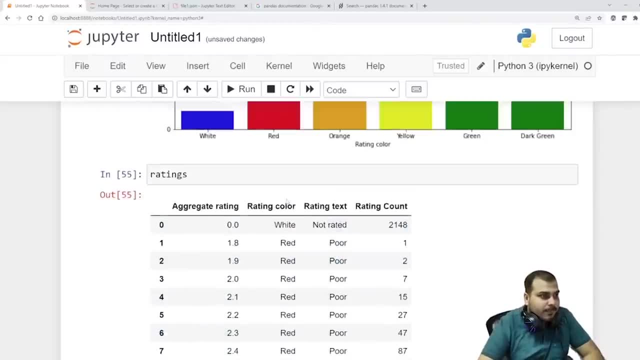 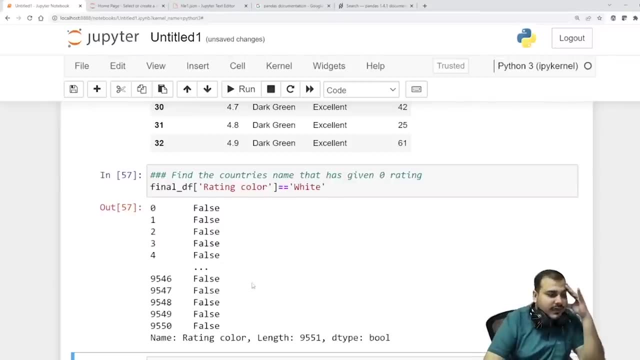 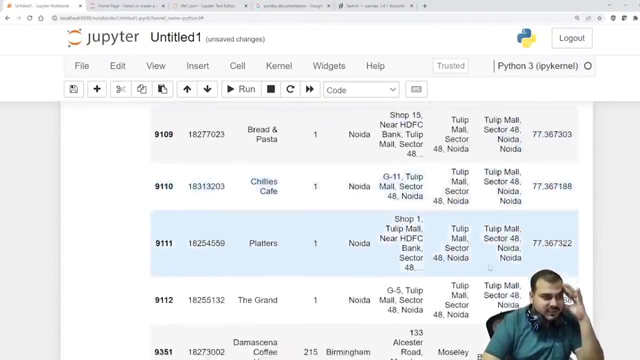 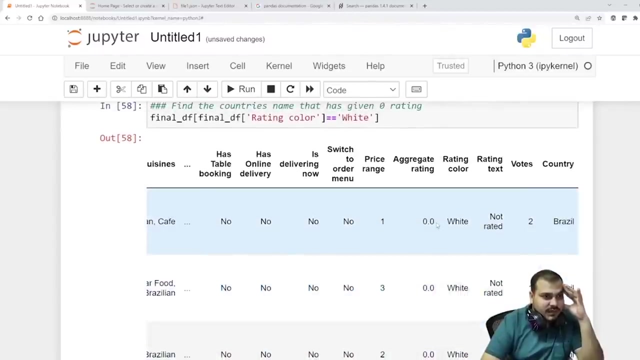 white is capital or small white is capital. so if i execute this here, i'll be getting like this: false, false, true, true. so i'll just write final underscore: df. so here, so many information i'm getting now. city, city, city. so many records are there. but i don't think so this is right, because here i may. 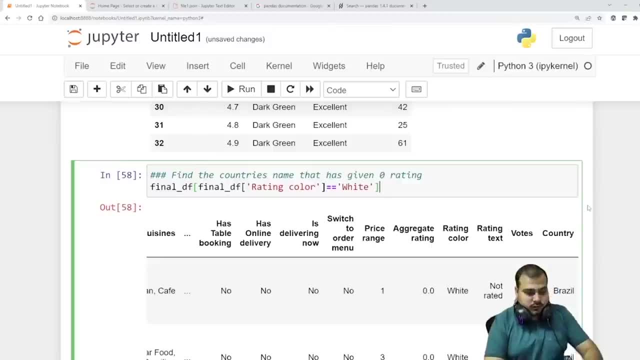 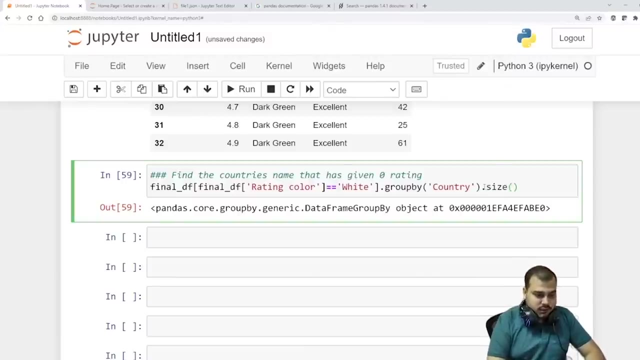 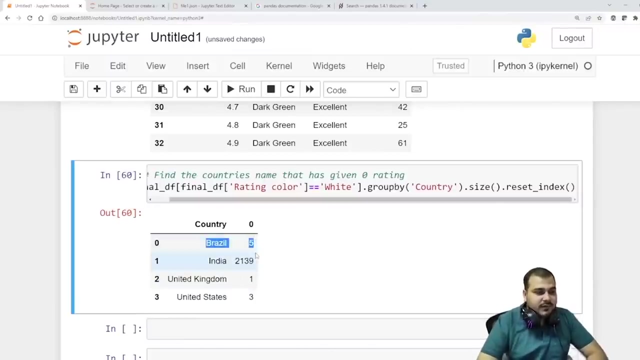 see different rating also. so here what i will do: i'll do group by and here i will specify my country. so if i execute this, this is my data frame. so here again i'll be doing dot size, dot reset index. so if i execute this now i'm able to get it. brazil: five different zero ratings is given. india. 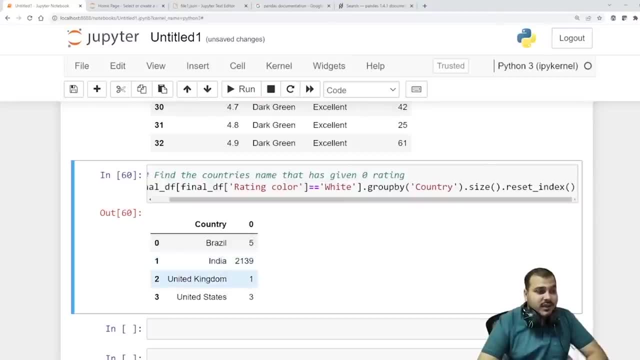 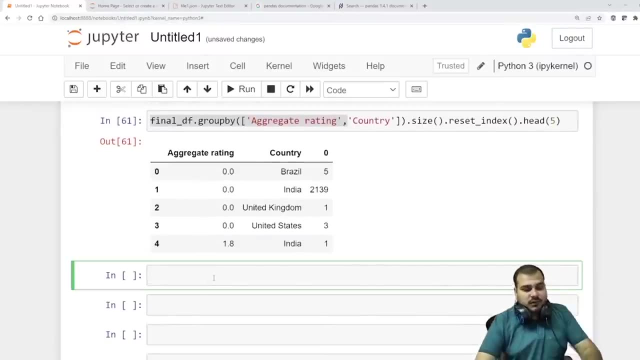 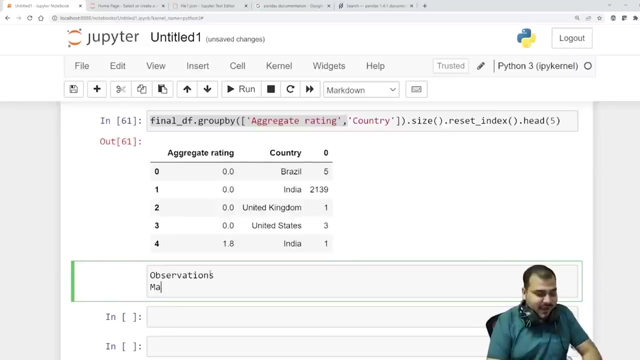 two, one, three, one, three, nine zero ratings has been given, united kingdom one, united states three. so again, what is observations that you can basically say? so here, write down the observations again now here, observations are what right? just just say observation. maximum number of zero ratings are from. 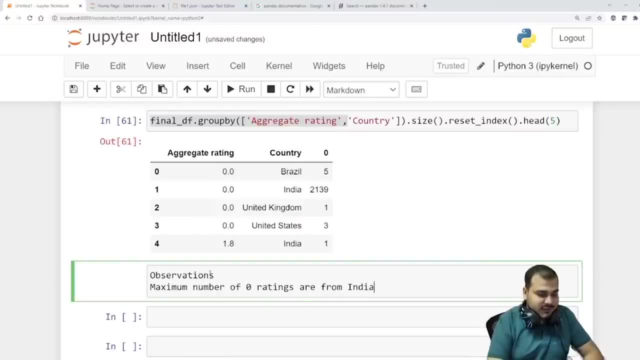 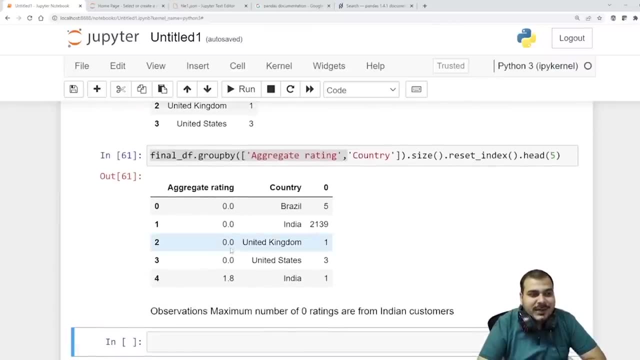 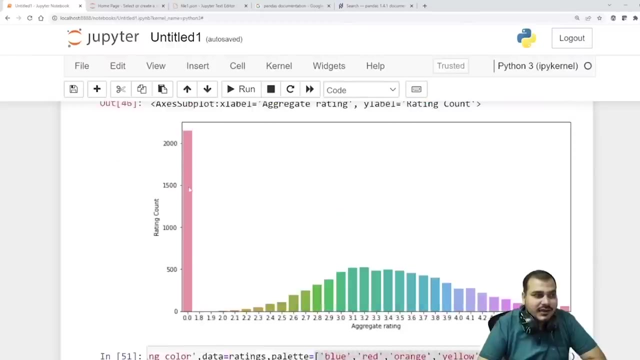 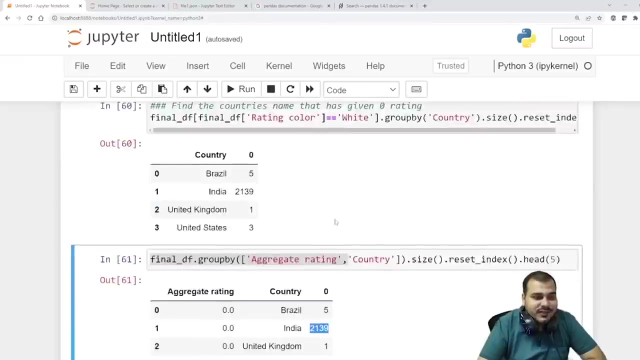 indian customers, right. so i guess you take that and think of it like: how is auditions going to work? is Zero rating equal to two, one, three, nine? no, it's not about imbalance data set in this case. uh, because if you see the data set right over here, two, one, three, eight, forty one. 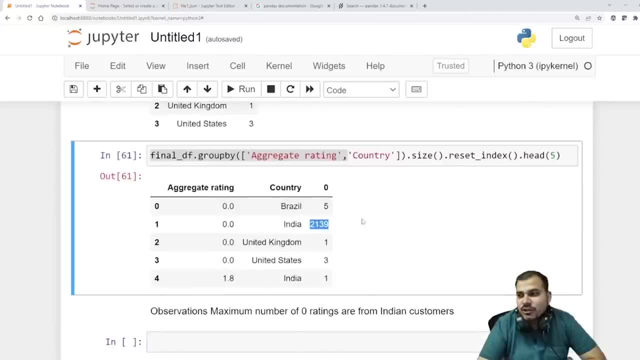 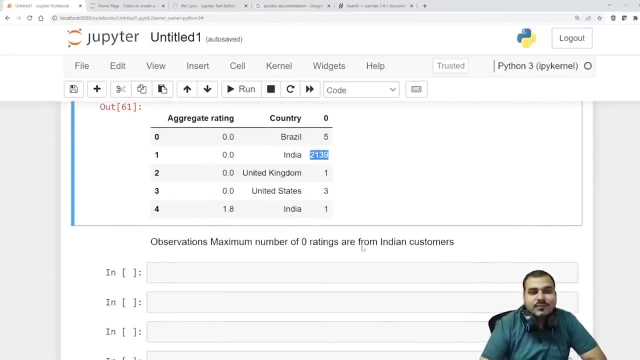 or four, eight, and from them, if you try to see two, one, three, nine, two huge number, because we don't know what we need to predict right now. we are just analyzing the data, taking out information from that data. okay, next question. next question to you: find out. 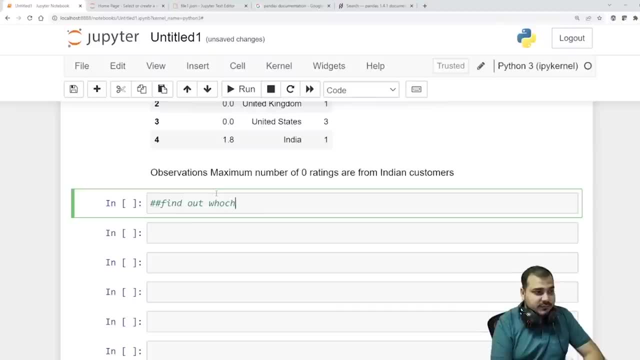 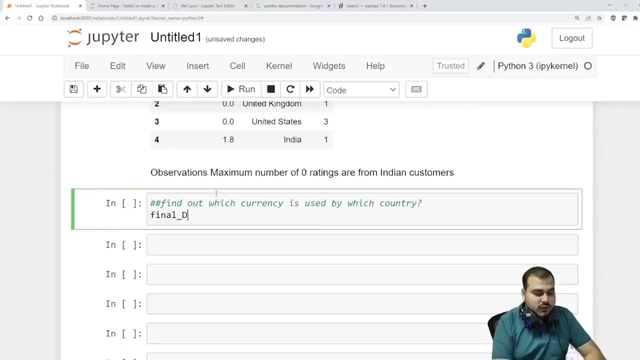 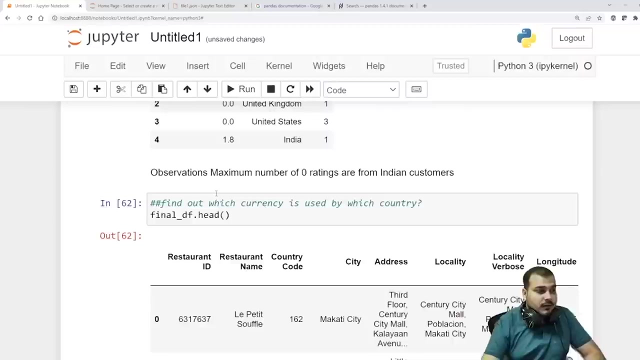 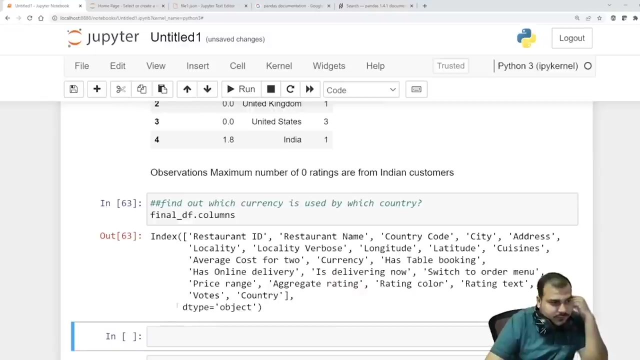 which currency? which currency is used by which country? so this is my next question to you all: if you probably go and see final underscore, df, dot head, you will be able to see this specific thing. so sorry, dot columns, i will just write it as dot columns. so here you have, let's say where it is, currency is there. 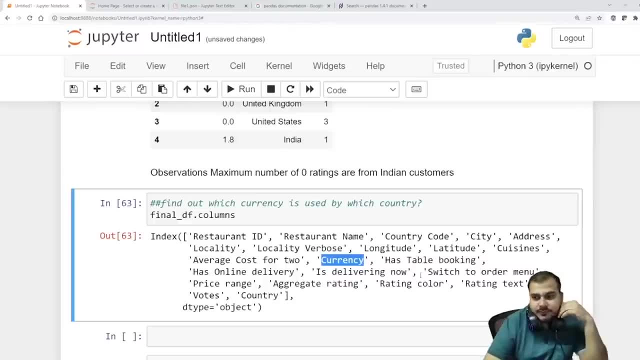 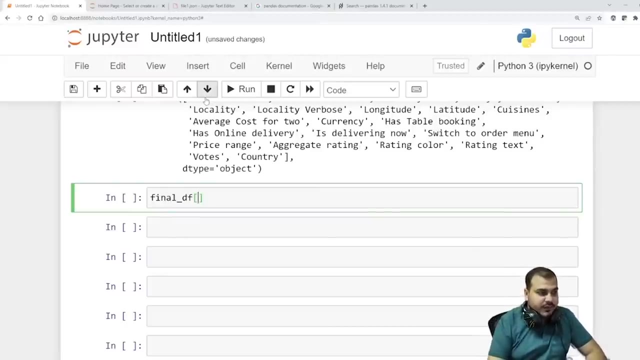 okay, currency is there, is there? so just try to do this: find out which currency is used by which country. if you want all the list of records, what you'll do. so what i am actually going to do now, i'm going to use final underscore df. there are two. i, i want basically country with respect to currency. so what i'm. 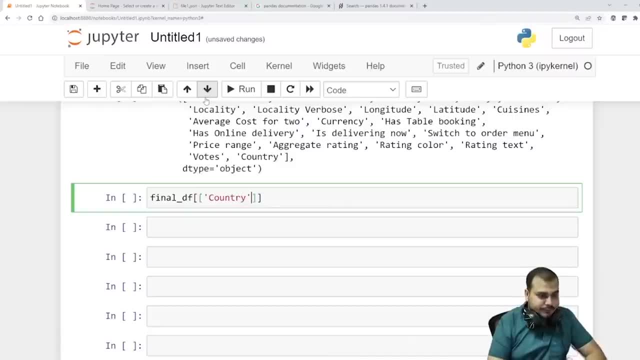 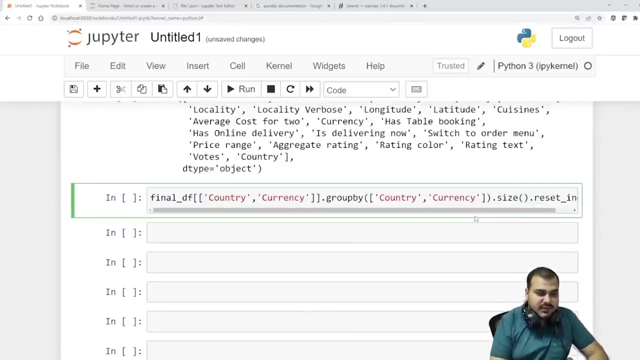 actually going to write over here. i'm going to basically say country, comma, currency and then i basically use group by again, and group by will again be based on these two groups, that is, country and currency. dot size, dot reset, reset index. reset index is used in many ways, so here you can see. 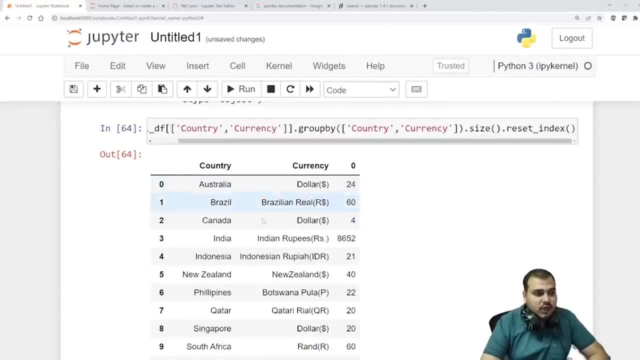 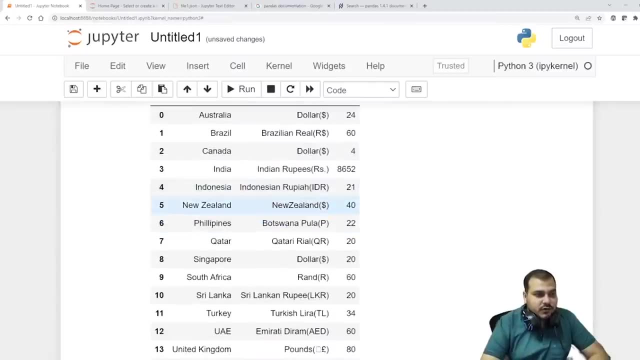 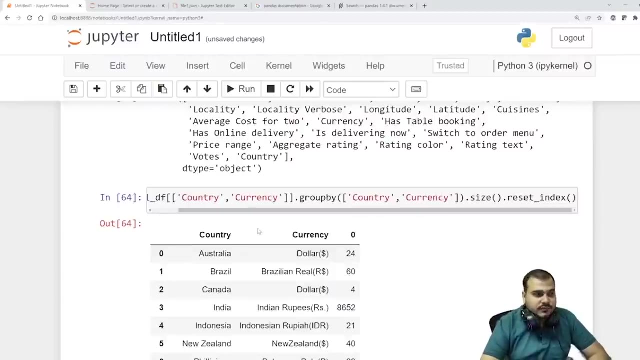 i'm actually getting australia dollar, brazil, brazilian real, canada dollars, indian indian rupees, indonesia rupiah, new zealand and all so two things: one is group by dot size, dot reset index, that's it. you don't have to do group by by everything, you have to just focus on two records. 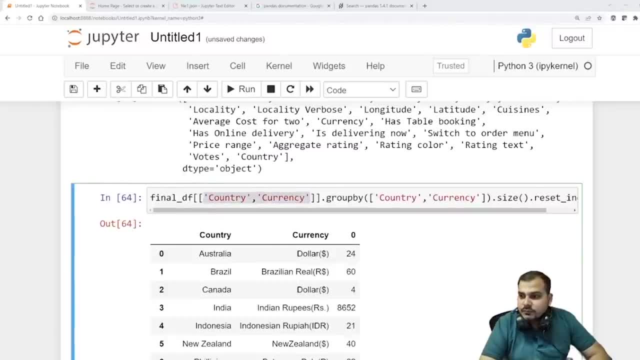 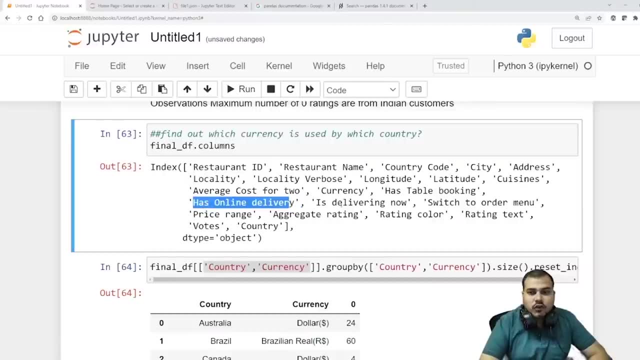 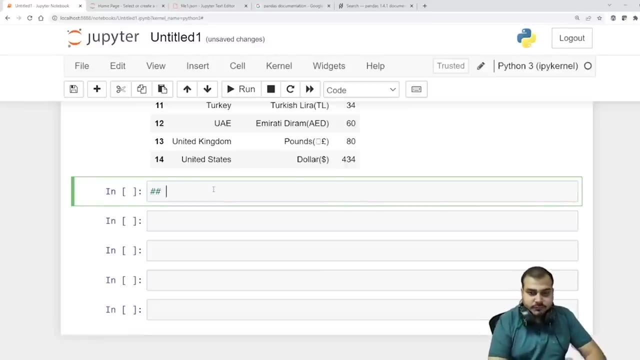 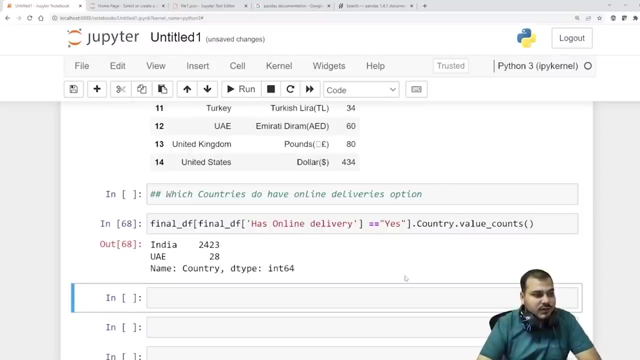 two features, that is, this and that. now here, one more feature is there. see, has online delivery or not. so my next question to you all, for those people who have done this, the next question is that which countries do have online deliveries, online deliveries option? so india has 2423, uae has 28- amazing, that's nice. that basically means: 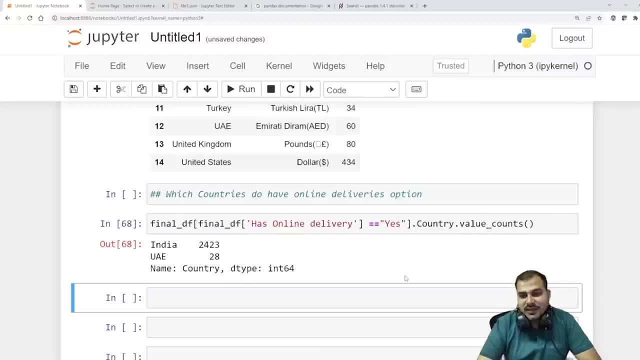 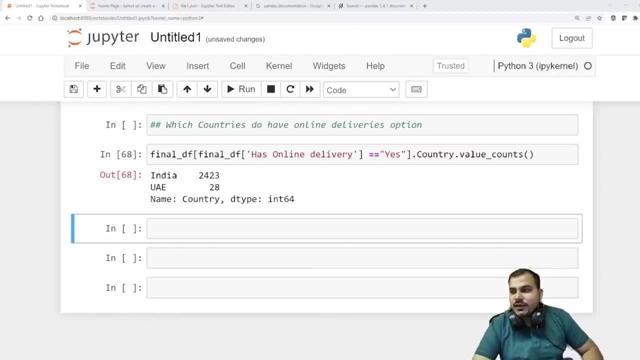 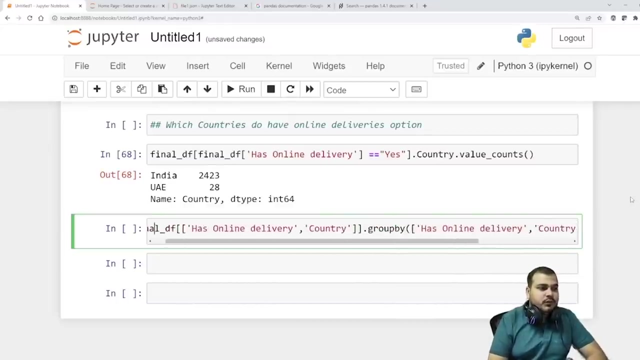 that the online delivery is only available in india and us. but let's say that i want to find out uh all the countries that has or has not. okay, i will just use this code. so reset index. that's it. so what he has done is that he's basically used uh two. 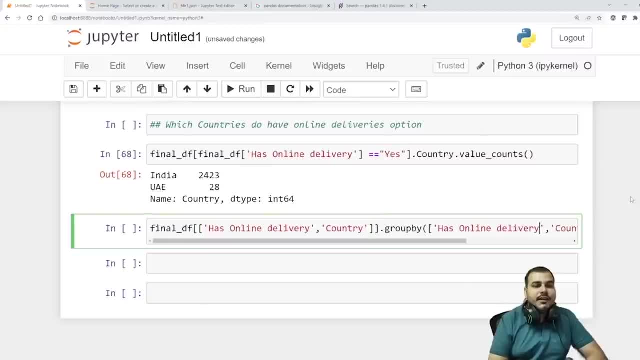 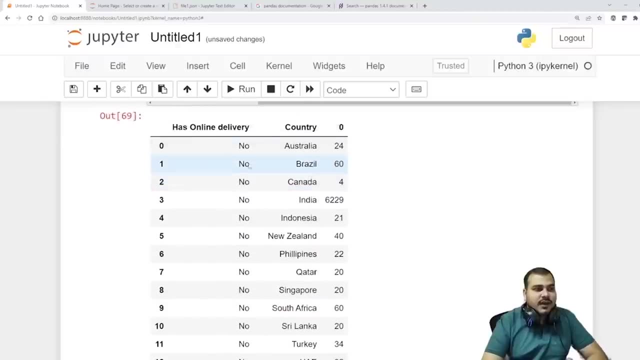 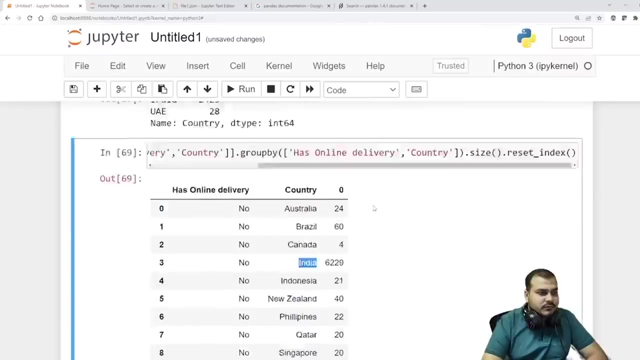 features: has online delivery country group by: has online delivery country and size dot reset index. so here you can basically see that australia: it does not have any. brazil: no online delivery. canada: no online delivery. why india? how come india is again coming over here? why india is getting repeated again? 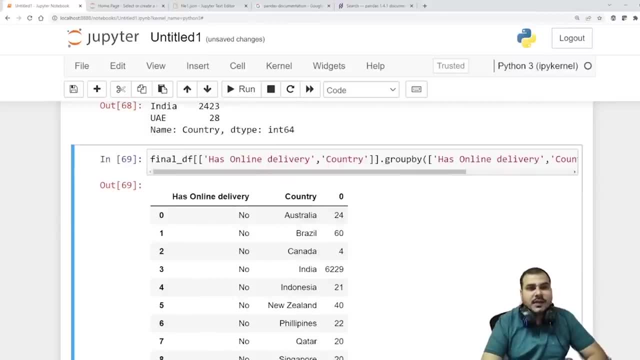 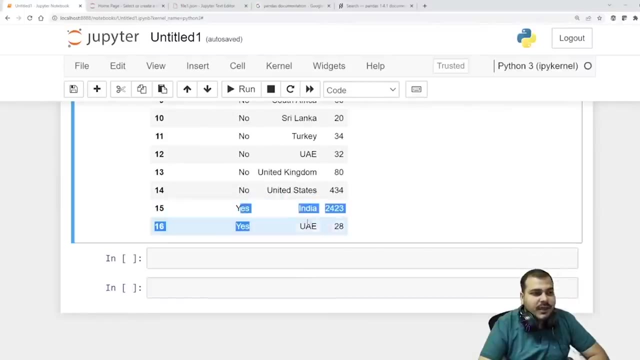 okay, in india also. probably in some of the reasons, online delivery may not be there. perfect, in india, in some of the regions you will not be finding online zomato delivery available. okay, so because of that, some records you will not be able to see, so but here you can see main. 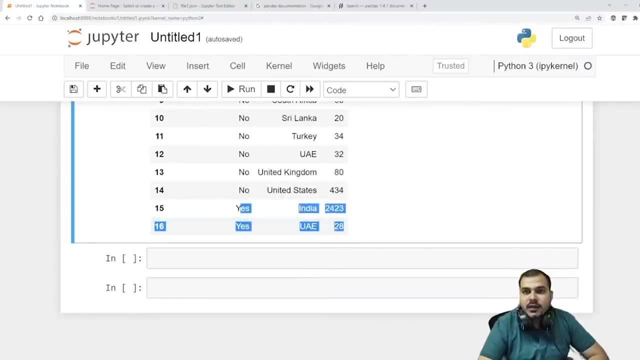 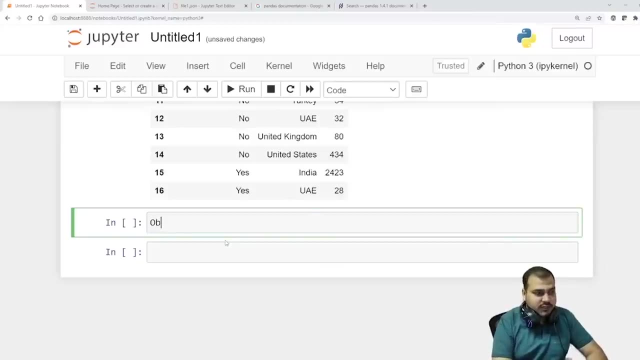 two countries that has online delivery is india and uae. so obviously make some observation from this and try to find out. so here i'm basically going to basically say observations again about what is my observations over here. i will basically say number: What are my observations over here? 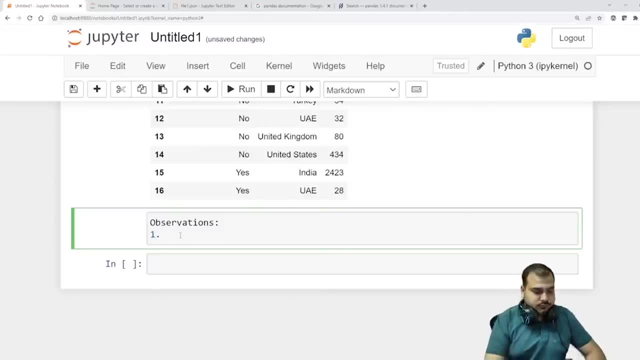 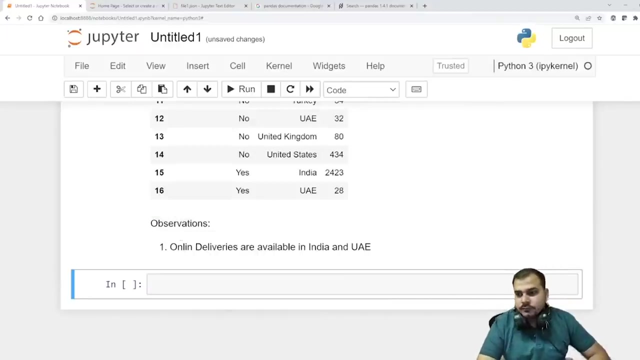 My first observation is that are available, since India and uae First online delivery is available to India and Uae. that internet delivery is available in india and uae. This may learning by the next question. So this is next question. Let's say numbers: uae that purchases, nevada that buys up. 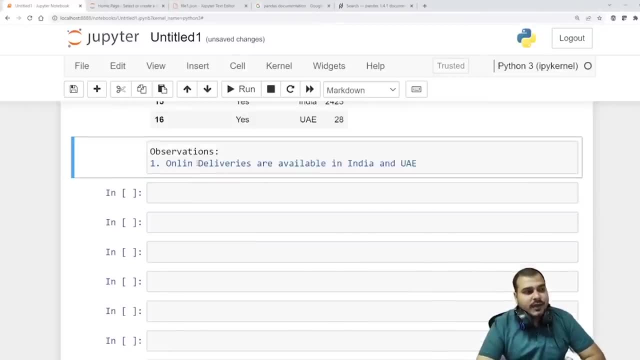 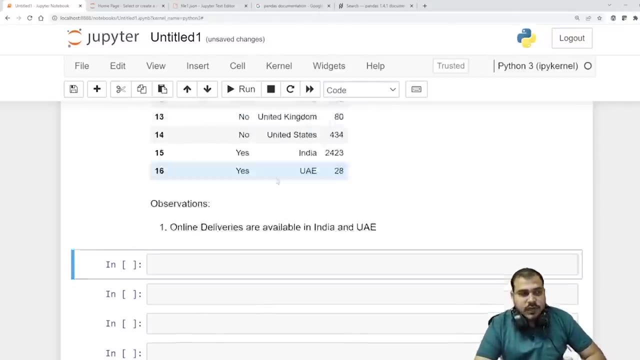 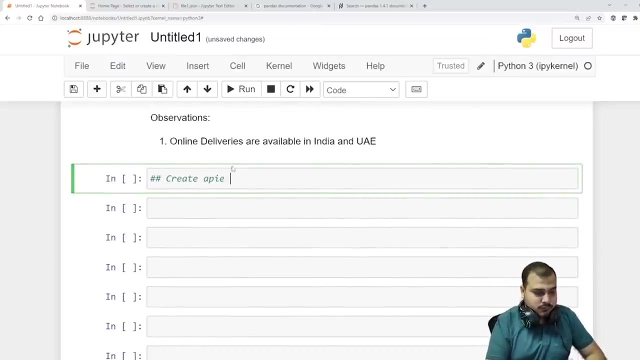 millions of dollars. Now, the next type that I am actually focusing on is that I'll give you one question, like how we did with respect to the countries, How we did with respect to the country. similarly, try to find out or create a pie chart for. 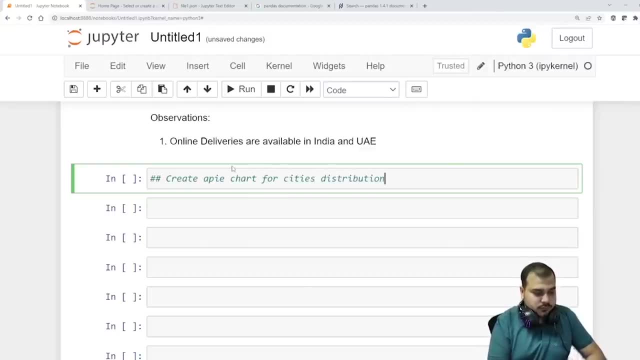 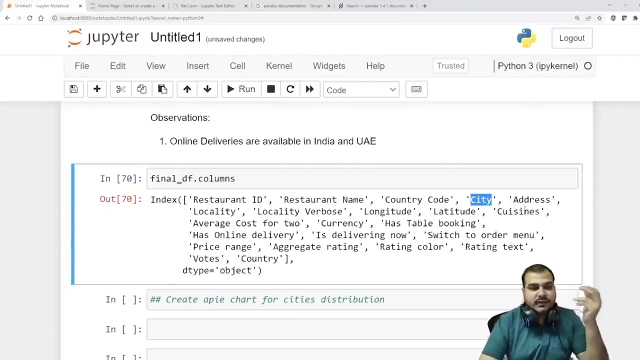 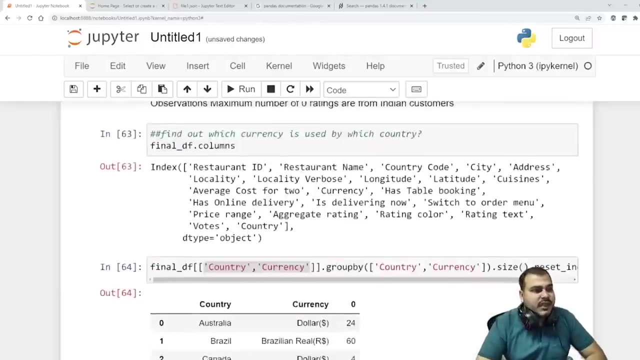 cities distribution. I hope everybody is understanding the question. So here, if I write final underscore df dot columns, you will be able to see there is also a city. Now I want to create a pie chart with respect to this specific cities. Again, the same thing like how we did it for country. 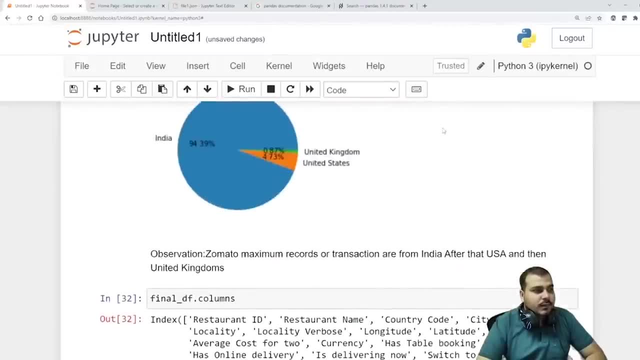 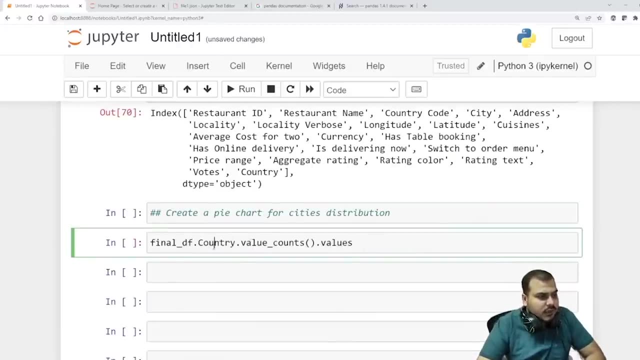 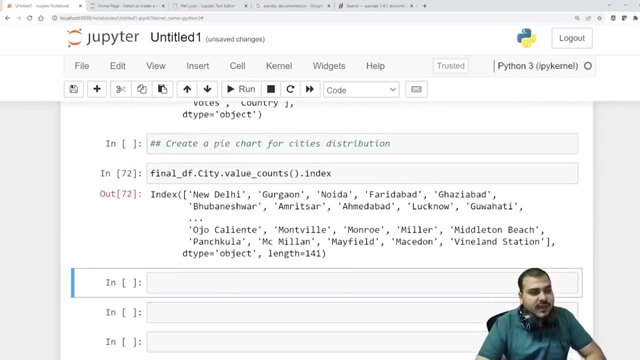 So I'll go up, I'll go up and I'll copy this two things, let's see. So here is one Here. instead of writing country, I'll write it as city. Then this is my values, this is my index. So this is my countries, cities from where the order has happened. 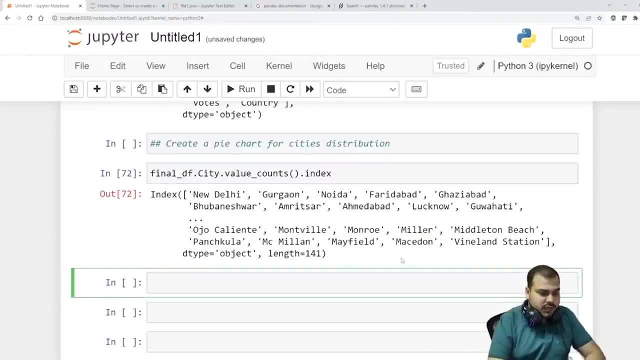 And I'll try to draw a plot, a pie plot, okay. So here I'll say plt, dot, pie. And here I'm going to give two things. One is with respect to values and then with respect to index. final underscore: df country. 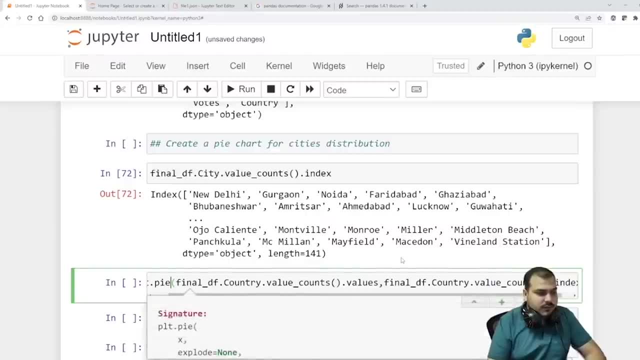 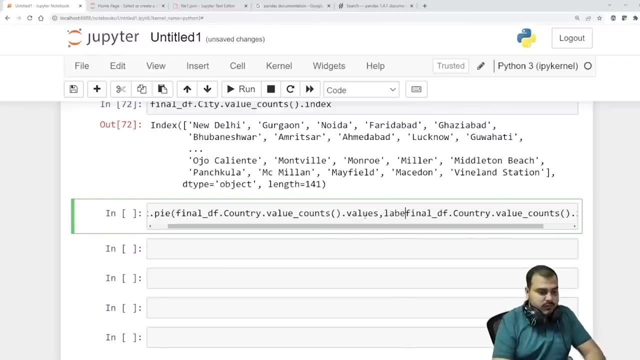 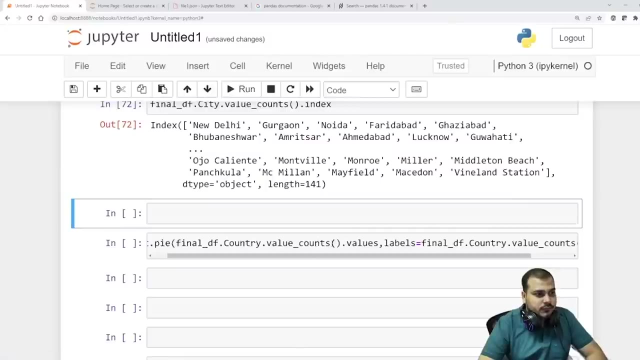 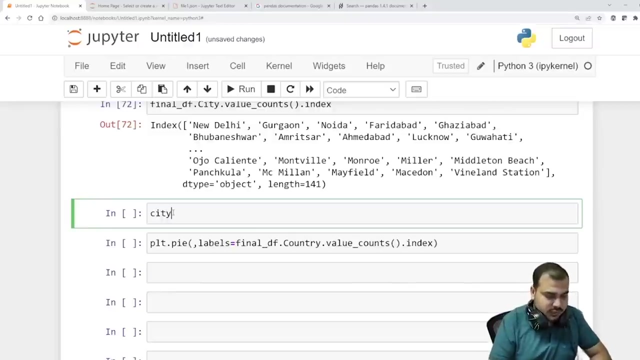 dot values. I hope this works Fine. Then x, x and y. I have to basically given this as labels: Okay, Labels. Or let me make it little bit easy for you, Let it make easy for you, Okay, City values. 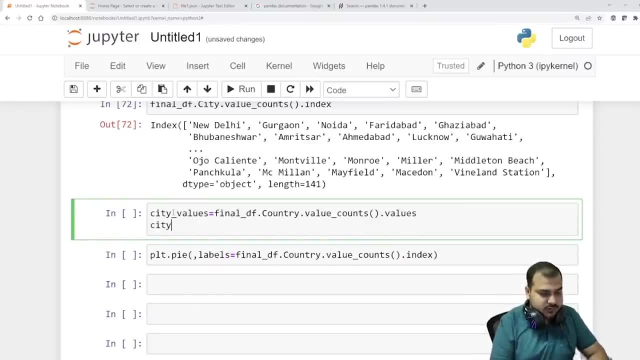 I'm going to save it in this City labels, I'm going to save it in this and this will basically be using index. so i have executed this. so this will go with city values and this entirely will go with respect to city labels. so i let's say that i want to. 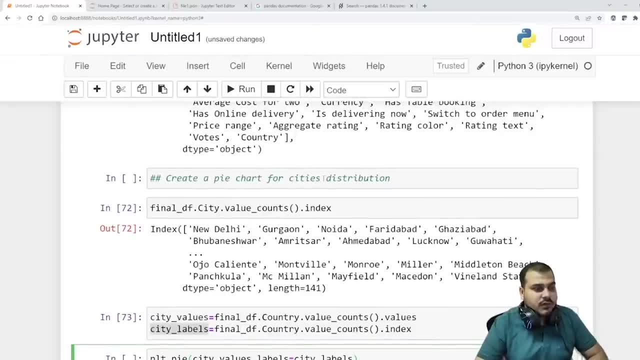 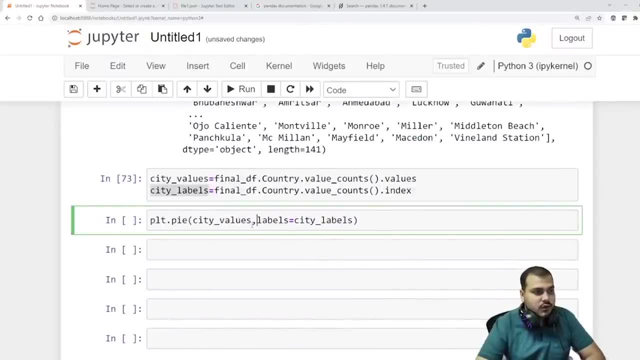 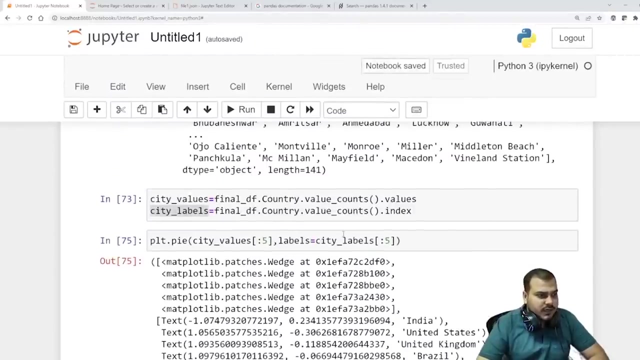 get the top five cities for cities. we should be for top five city distribution, top five city distribution. so here i will just use colon five and here also i will be using colon five. so once i execute this here, you will be able to see this the first. oh, it's coming as india. why city labels? 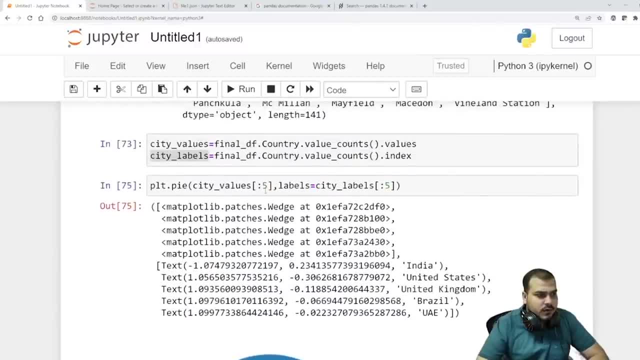 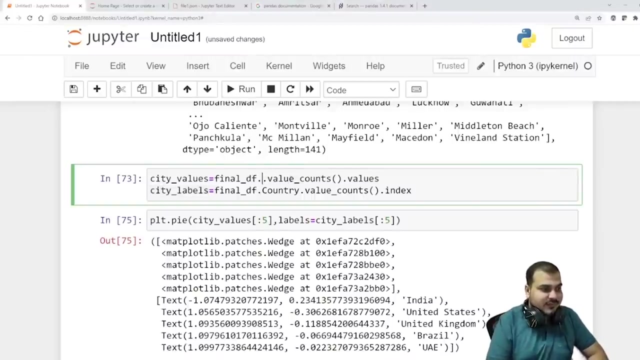 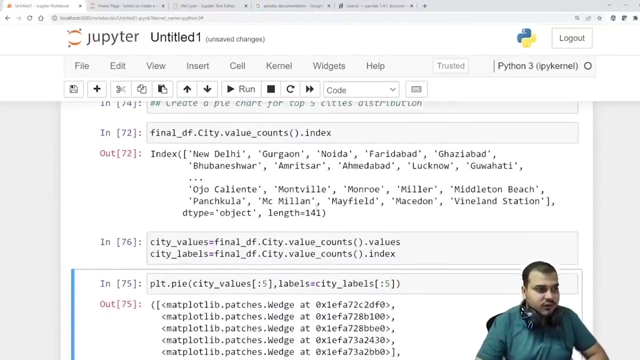 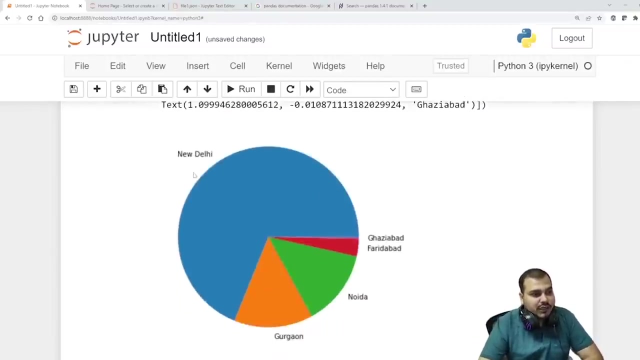 plot dot y city value city labels. why, why, why, why, why, why. i think there is some mistake. plot pi final and so you can. oh, i have to use city mistaken, mistaken, mistaken. i had copied right. so you should not do copy and paste a lot. don't do copy paste. so new delhi has the maximum number of transaction gurgaon, noida gaziabad. 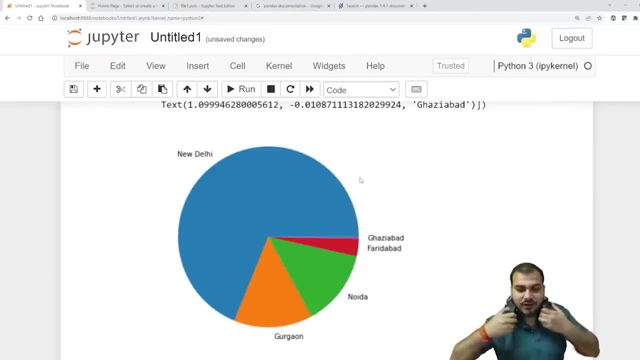 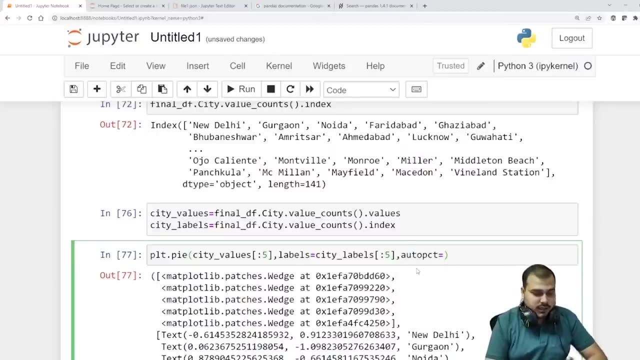 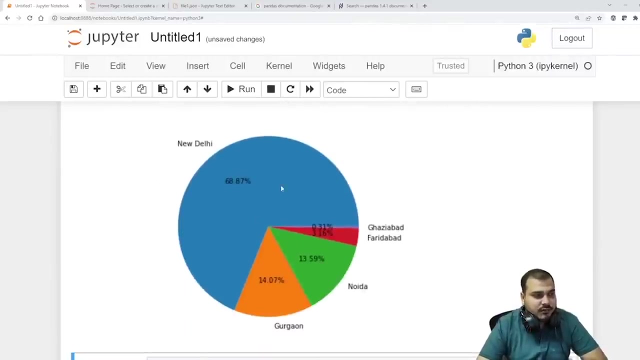 and faridabad. why not bangalore? i think in the data set bangalore is not given. after this i'll also add one auto percentage and here i can basically specify 1.2 f. so if i go and see this, here you'll be able to see percentage. so maximum number of transaction. 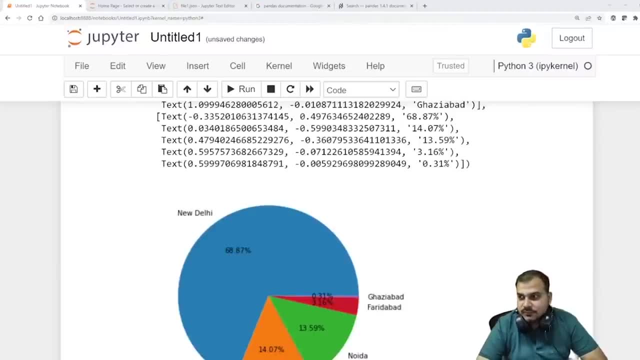 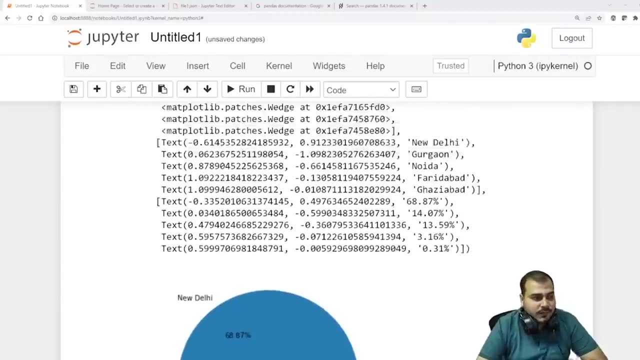 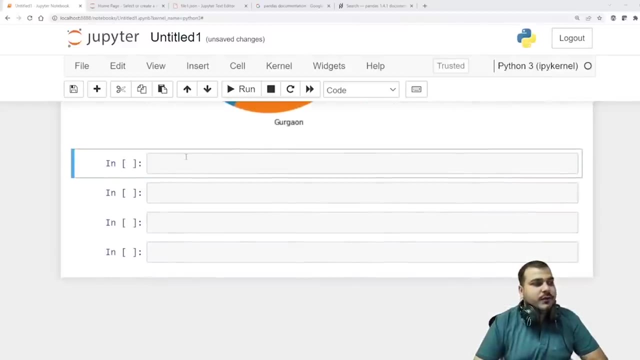 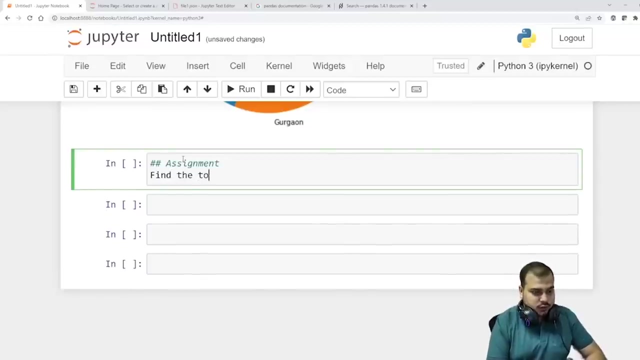 is basically happening from new delhi. so, guys, overall, how was the session? everybody? one assignment for you. so assignment: find the top ten cushines. cushines basically means food. okay, food item. so this will be for you. just do it: one assignment and remaining all items on the menu and you will get the last item now. good bye, bye, bye. 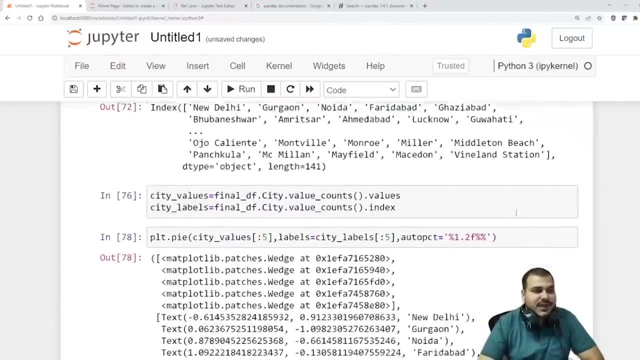 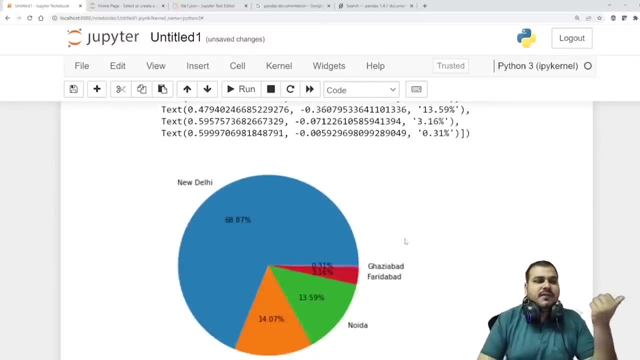 all. I think I have done it now in this data set. I had never used this data set for doing machine learning modeling. I needed this data set to find out what all information I can capture from it and finally I was able to do so many things right. I did not worry about. 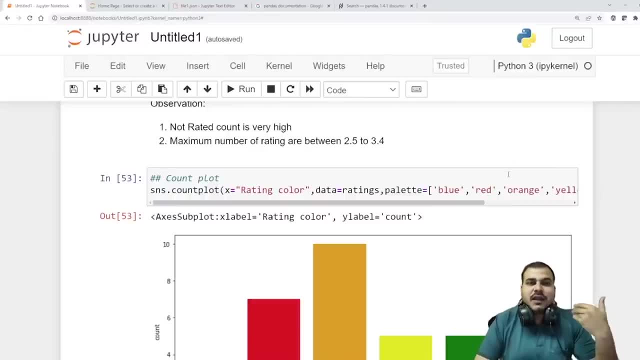 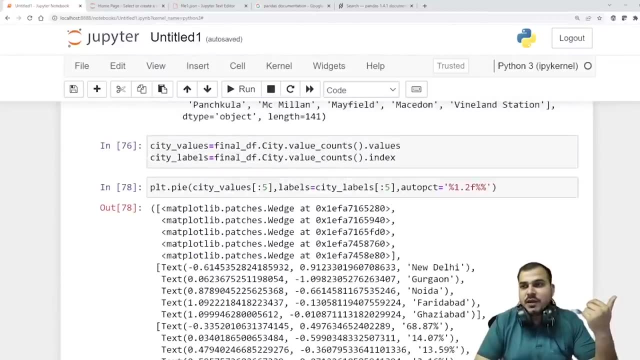 distribution and all that is the part when we actually create a model with respect to the data set. at that point of time we do. so I hope you like this particular session. it was fun, it was comedy, it was good. can we group the other cities under rest? yes, obviously. 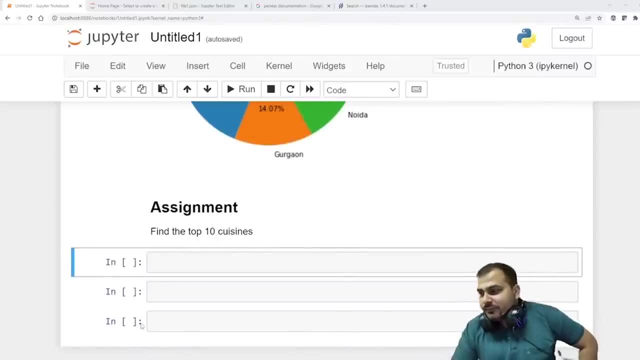 you can do it right tomorrow, another amazing day, another amazing data set, so that we will be working on it and definitely you will be able to learn a lot. as I said right. visit the website, guys, because here I am going to give the entire materials. have you seen the? 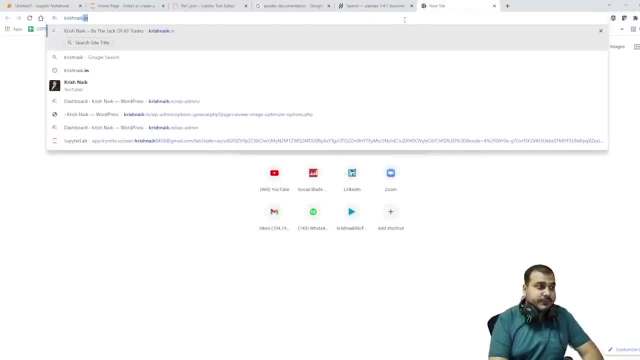 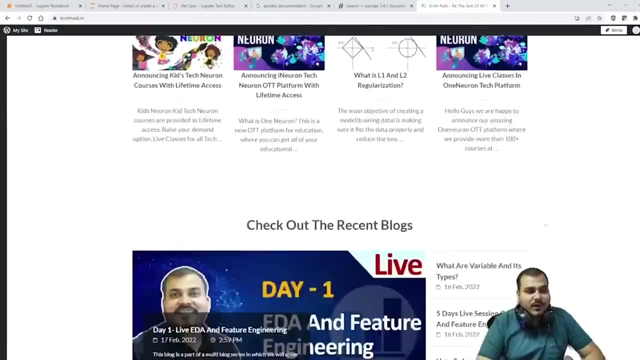 website guys. have you seen the website guys? have you seen the website guys? have you seen my website? how do you like to rate my website guys? so this I created in 3 to 4 hours probably, I'll also start showing you how to create websites. so this entirely I created 3 to 4. 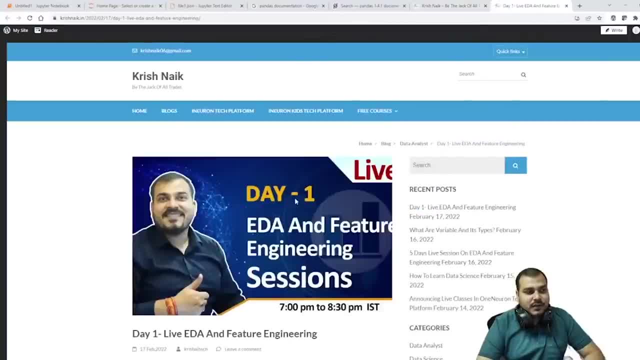 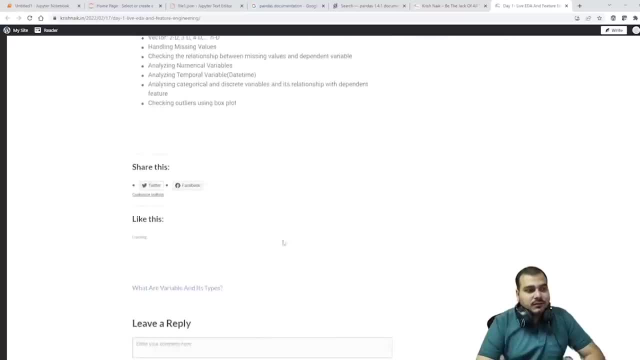 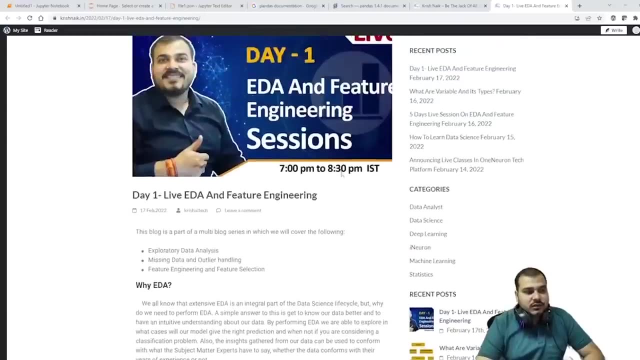 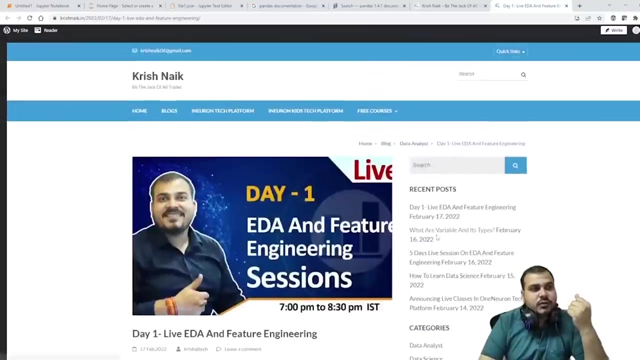 hours, so everything will get updated in this article. also, see this: this live session is going on right now currently. see, all the materials will get uploaded over here- data set materials. so please make sure you do this and, yeah, start exploring it, okay, guys? so thank you, keep on rocking. I'll see you all in tomorrow's video and, yes, I will see you in tomorrow's. 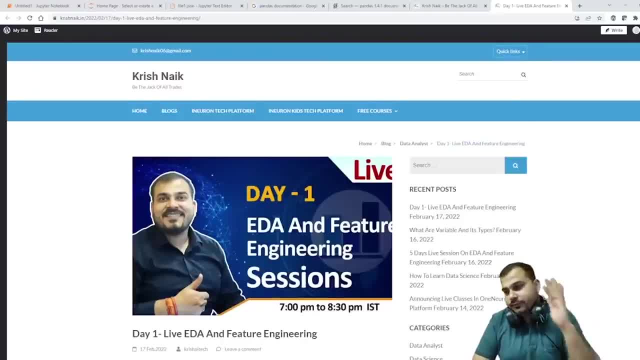 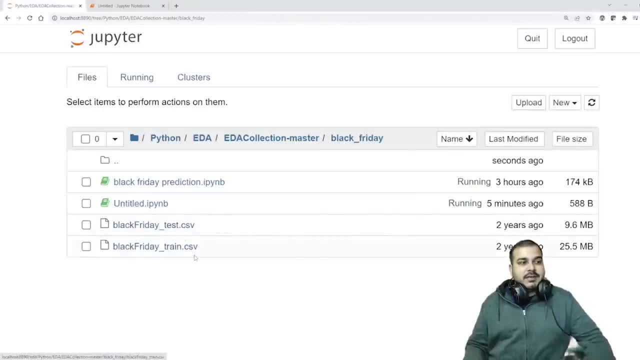 session. tomorrow we'll have more in-depth session. thank you everybody. bye, bye, take care. thank you guys, I hope everybody has downloaded the data set. you will have this two data set: one is test and train. right, I'll talk about the problem statement and today we are going. 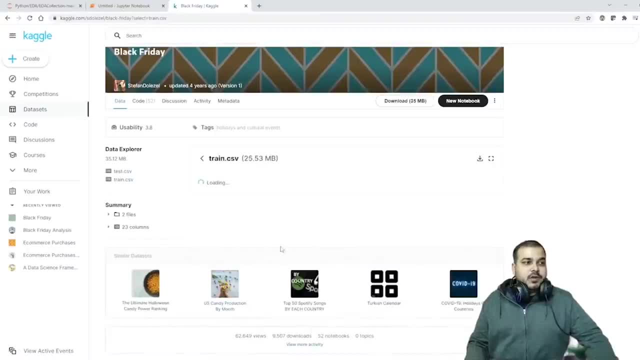 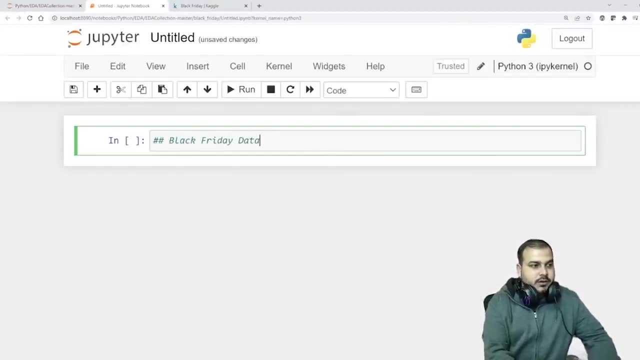 to do feature engineering and both these things right, as usual. today we are going to do black friday: data set. I'll talk about the agenda everything: EDA and feature engineering. we are going to do both of this and we will keep our model ready for model training, ready it's. 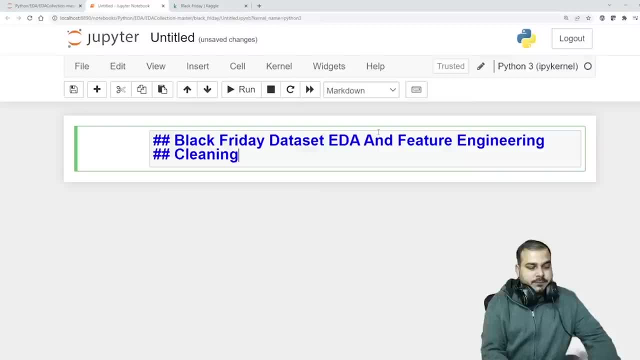 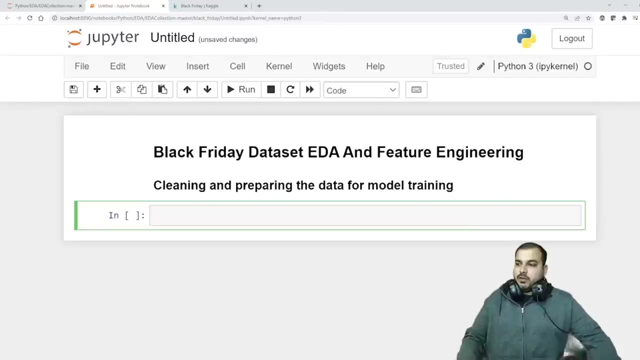 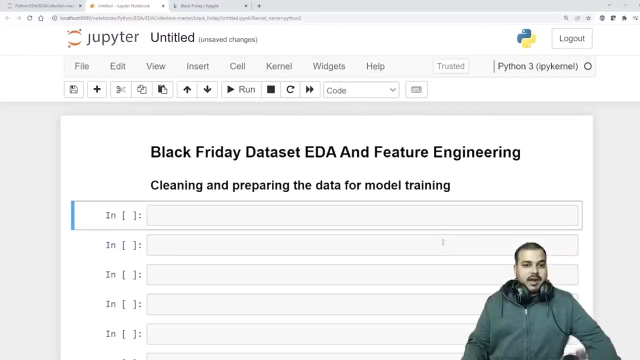 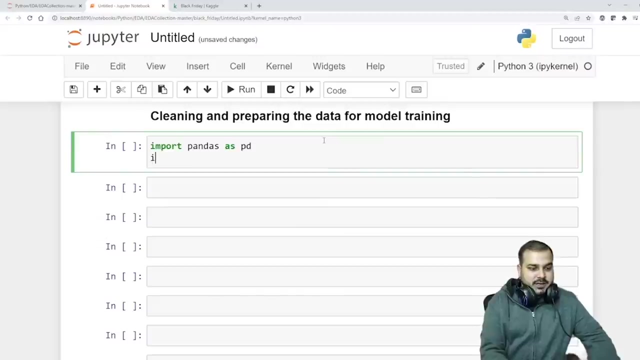 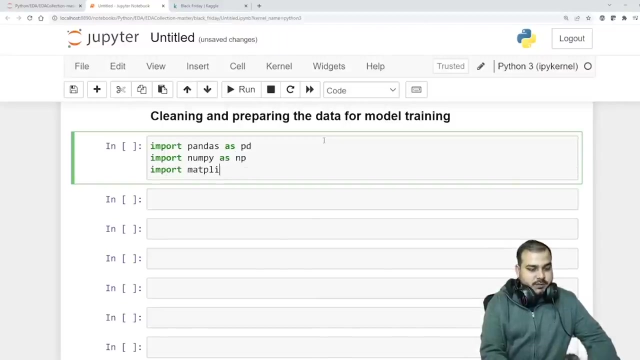 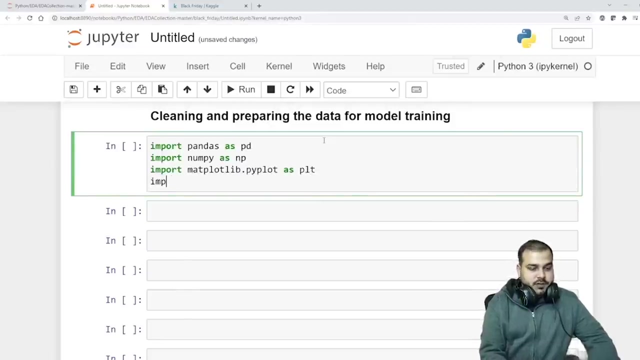 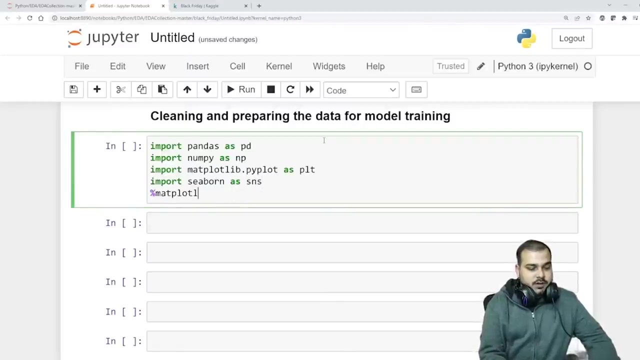 cleaning, doing everything cleaning. I'm preparing for the next session. I'll see you in the next session. so guys, take care, guys, and I'll see you in the next session. bye, bye. as np, import matplotlibpyplot as plt, import cbon as sns and then matplotlibpyplot as 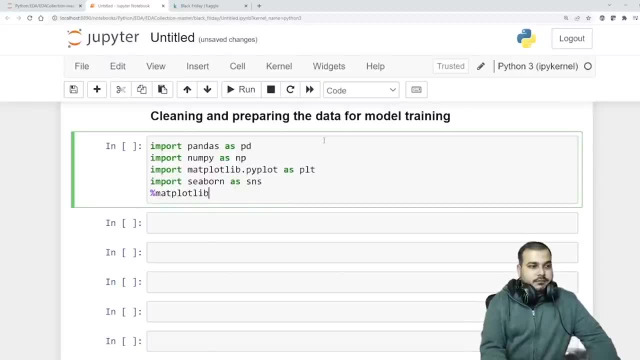 plt. ye, sorry, inline, so this is basically given in caggle. ok, so in caggle, whenever you get a specific data set, what do you have to do? train and test that. all steps i will show you so that you can also participate in caggle. so let's go ahead, and let's go ahead with 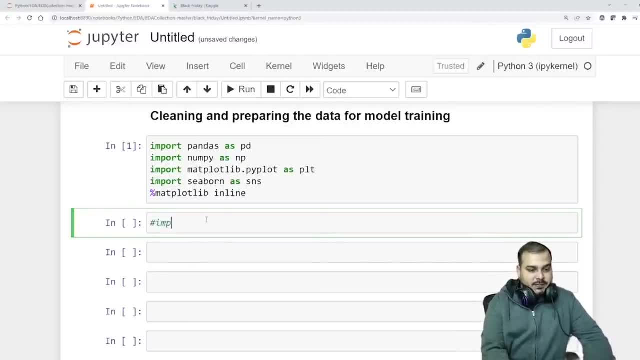 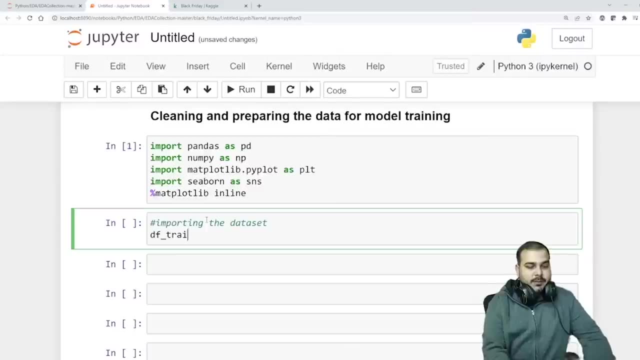 first of all, importing the data set. always make sure that you write the comment so importing the data set. the data set is already given to you. so let's say i am going to name it as dftrain because i have two data set: one is train and one is test data. so this dftrain- 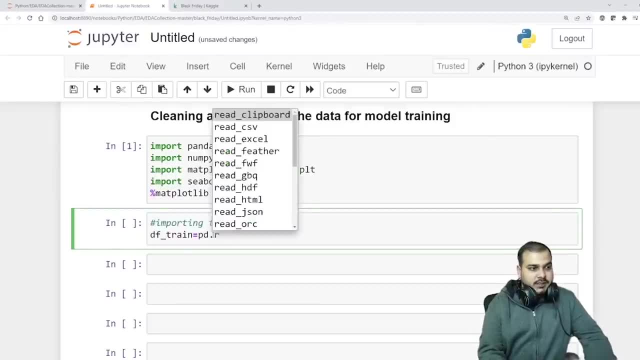 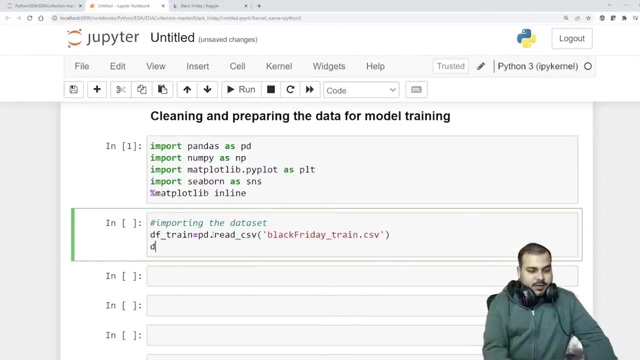 I'm just going to write pdreadcsv and I'm just going to give my dataset name blackfridaytraincsv. I have renamed the name, guys, For you it will be traincsv. okay, And then if I probably write dftrainshape, I will be able to see it, or if I write dfhead, I'll be able to see it. 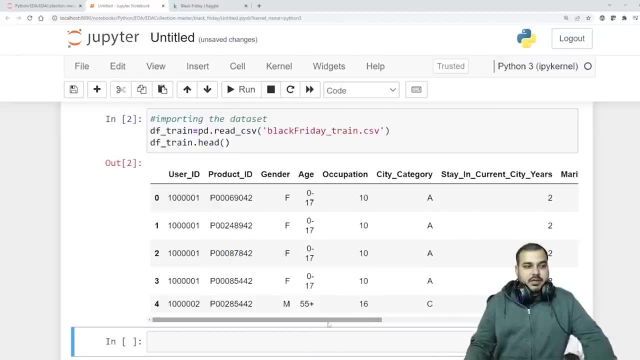 So I'll talk about the data, What this data is basically about. So this data is an e-commerce data, So people who have bought some kind of products and, based on that, we need to predict what is the purchase capacity. Again, understand? I'm just going to basically talk about the problem statement. 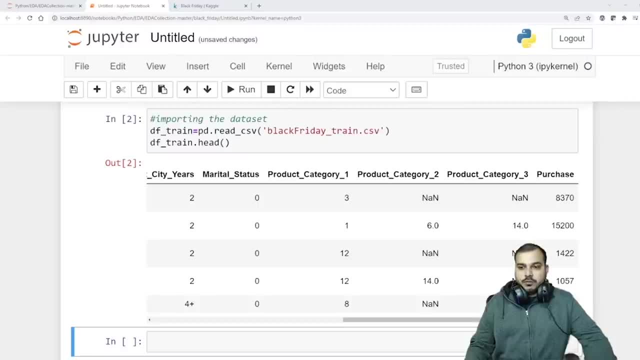 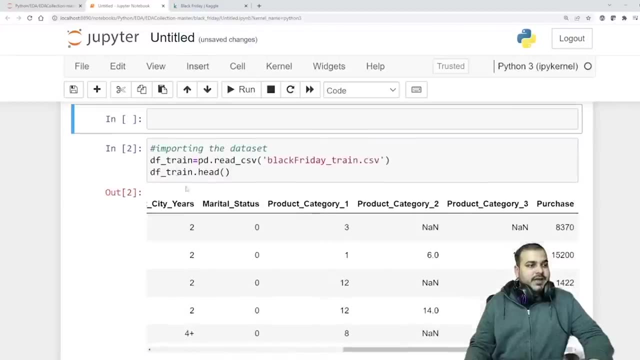 Here. we want to build a model. I'm just going to put the problem statement over here. Let's say, I'm going to put a problem statement over here. Everybody Read the problem statement. Anyhow, I will be giving you all these things, materials, everything in the GitHub. 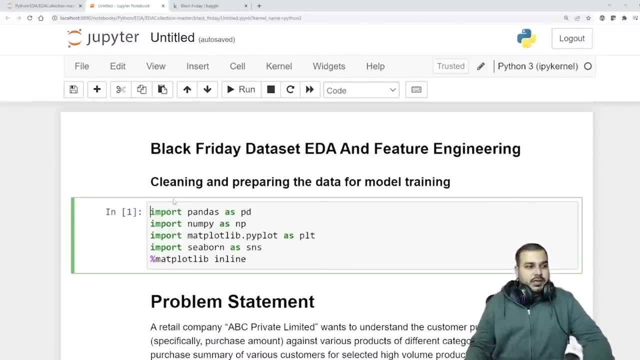 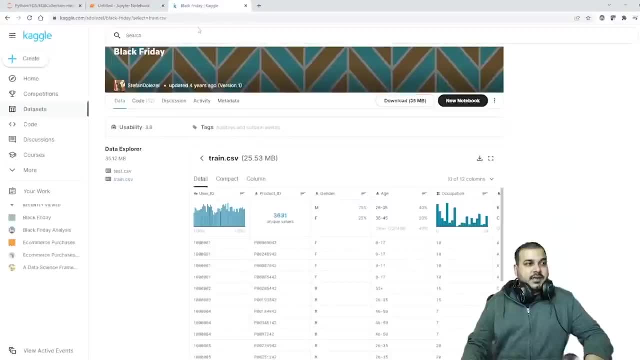 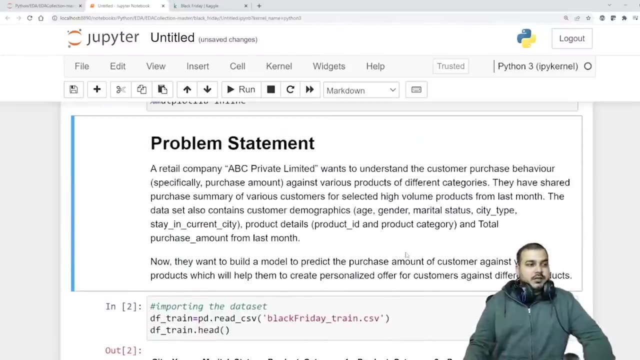 Don't worry. So I'll also put the dataset link over here: Dataset link. So dataset link is this Dataset link And this will get saved over here. So what is the problem statement? So this is the problem statement that we are going to focus on. 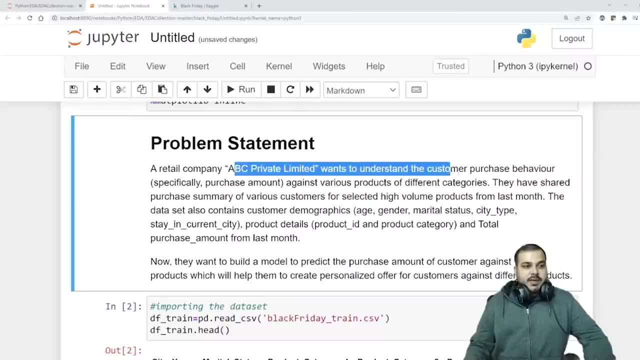 So the problem statement is at readcsvtraincsv. That page has multiple different categories. This is an event for evaluation. it's different from every other, So every article has got different categories. Again, it will provide a simple example for the research actions in this country. 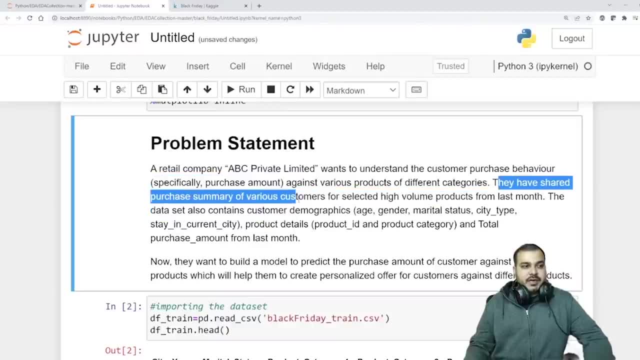 The detail company, ABC private limited, wants to understand the customer purchase behavior. There is an e-commerce data set. Dataset is also very huge So it will be very good to work on it against various products of different categories. they have shared purchase summary of various customers for selected high volume products. 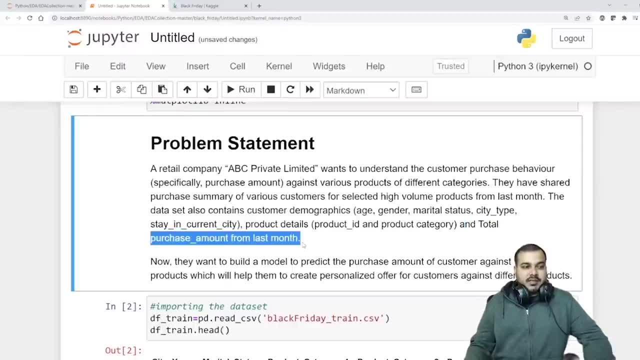 from last month and total purchase amount from last month. so over here now they want to build a. now they want to build a model to predict the purchase amount of customer against various product. that will help them to create a personalized offer for customer against different products. so this is the problem. 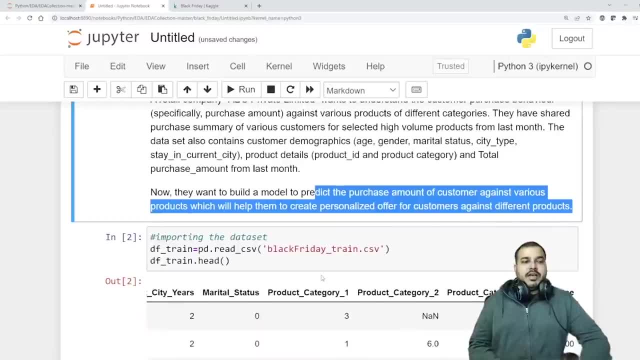 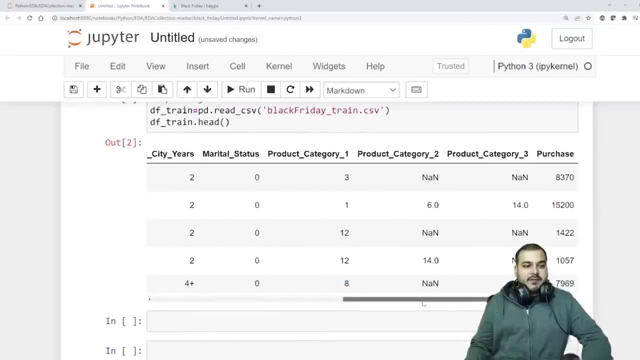 statement over here. the problem statement is very simple: you need to create a model to predict the purchase amount of a customer against various products, right? so suppose, if i have, if i give this information like this product, with this product information, these all things i give, then we should create a model that will be able to predict this purchasing capacity, right? so this is. 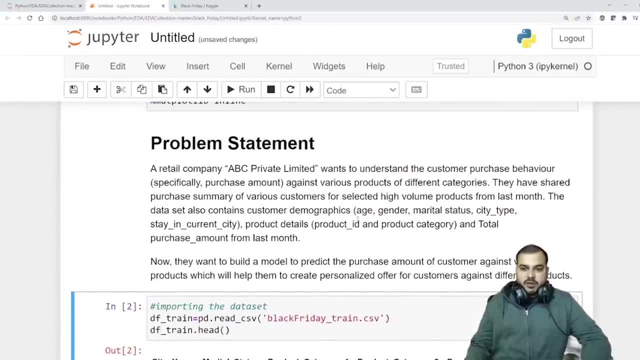 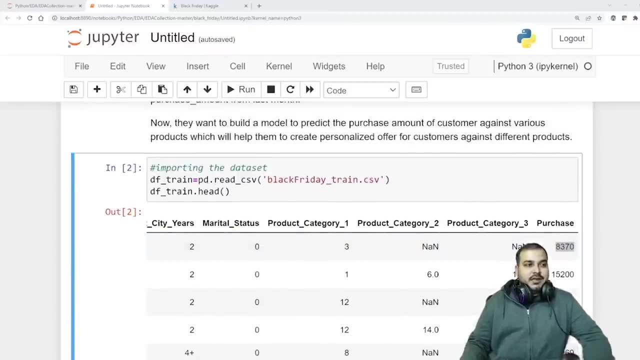 the entire information regarding the problem statement. okay, so this is what we are going to do. interesting, we'll solve the problem here only in front of you. so i have read the training data set. the next step is to create a model to predict the purchase amount of a customer against various 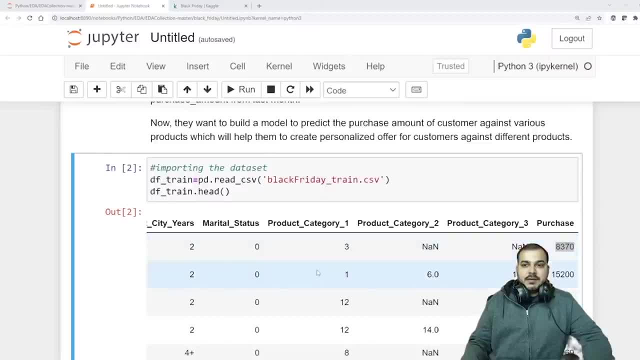 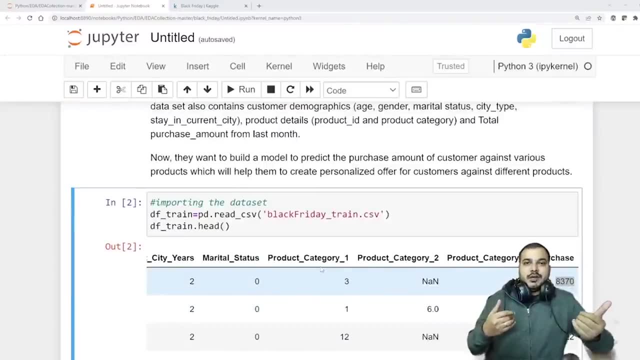 the next step that you have to do is basically start reading the test data set now. train data set, test data set. see, whenever you are given train and test obviously, what initially you have to do. you have to combine them in a kaggle competition. always remember to combine them so that all the 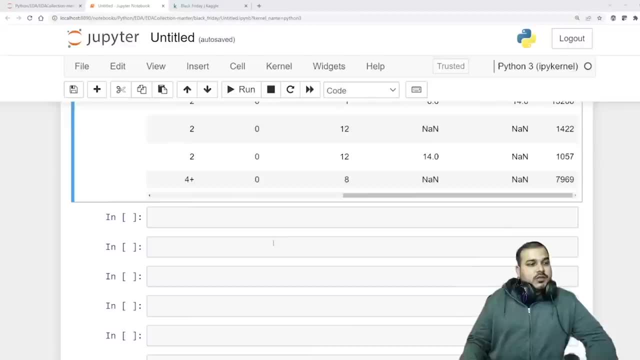 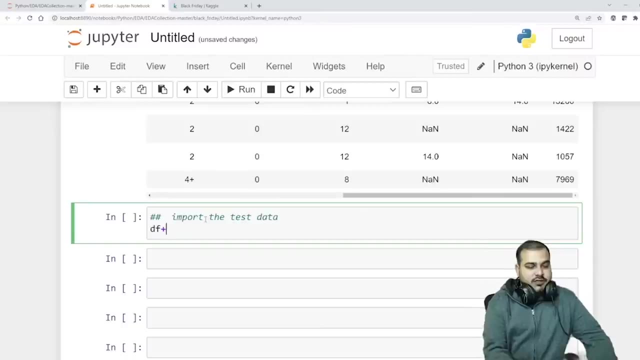 data pre-processing. that we can do, we can perform on both the data set. so here i am going to now import the test data right. so here i am going to say: df underscore test is equal to, is equal to, is equal to pd dot. read underscore csv. 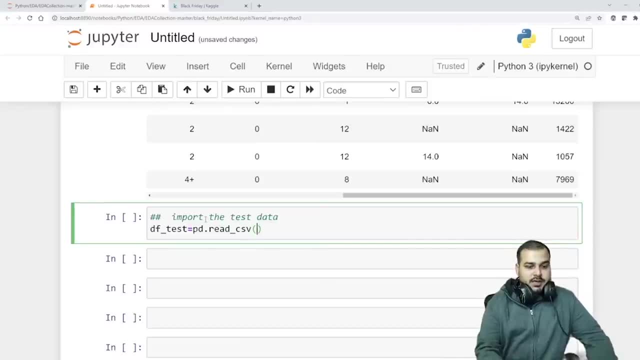 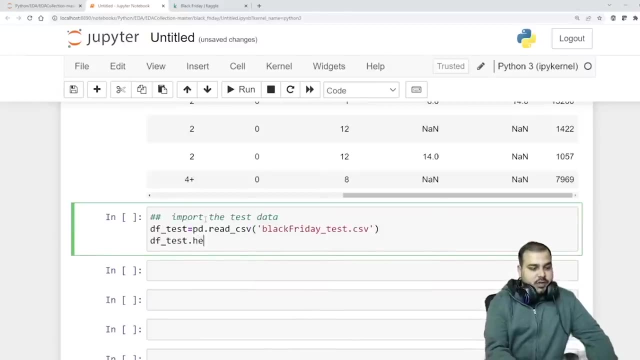 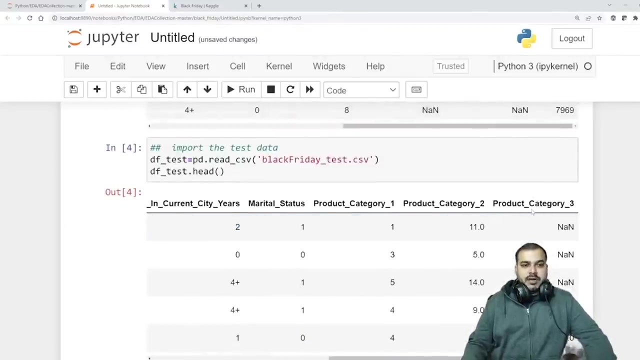 and here i am going to basically write black friday test dot csv df underscore test dot head. in the test data you will not be able to find the output variable. so here you can see analytic product. category three is there here. additional purchase column is there right. so now, if you want to combine the train and test data, how do you do? 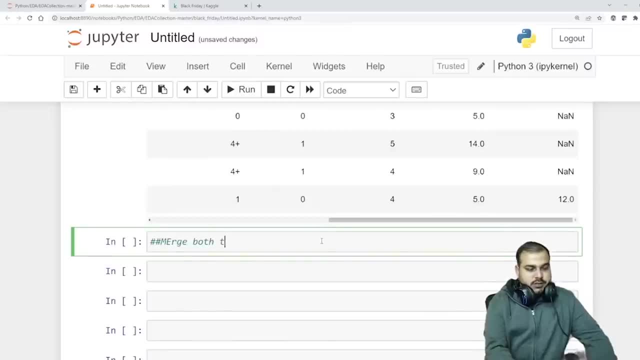 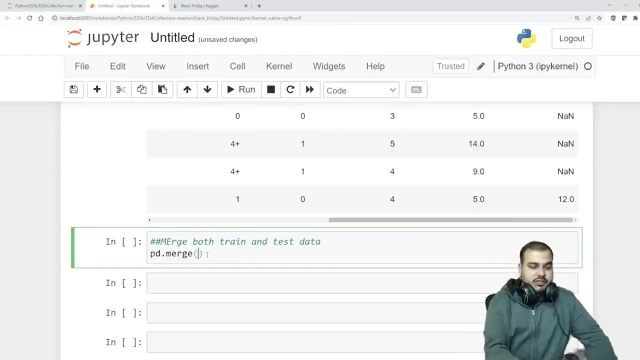 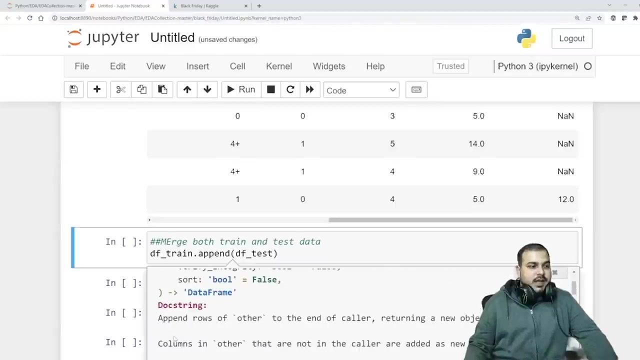 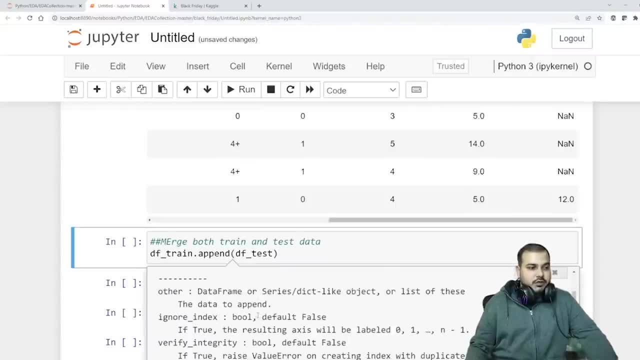 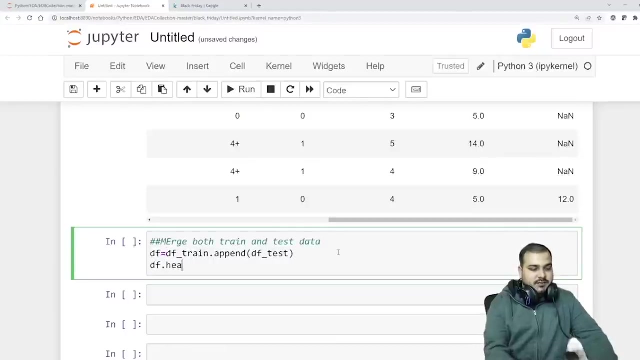 the end of the caller returning a new object, right? so i'm just going to do this. there is also one more parameter that i see with respect to sort. so sort by default is false, right? so i'm just going to execute this and then i'm basically going to store this inside my df. so this is my df dot head. 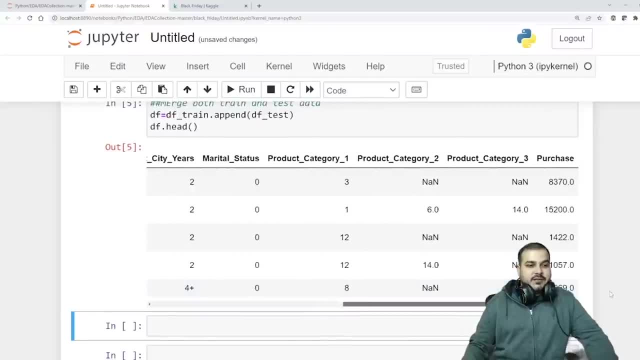 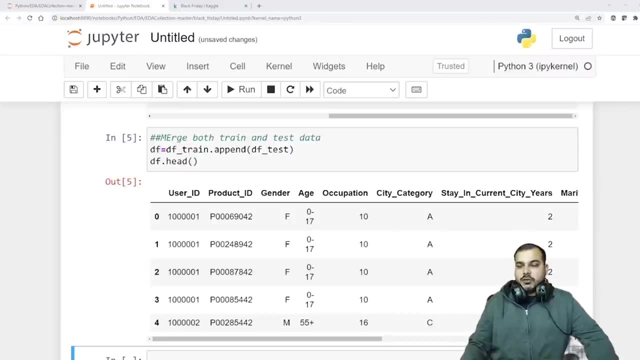 now you can also append it in different, different ways. i have no problem. okay, it is up to you. so this is the first step that we have. actually merge also, you can do, but again, understand, we have to append it at the bottom right. we are not merging it like this. so merge if you want to do with 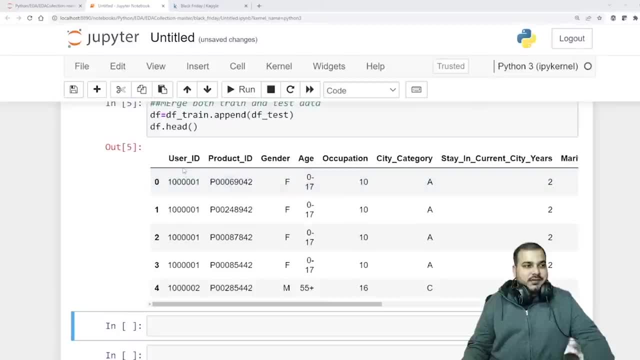 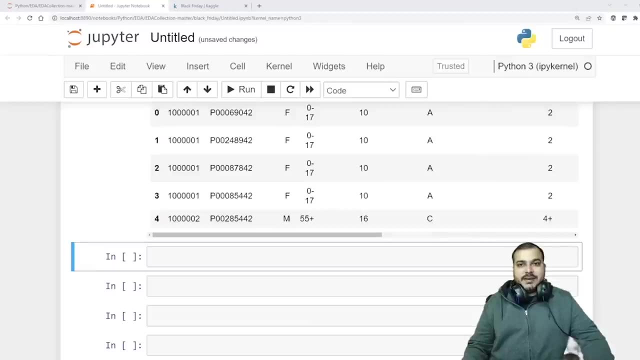 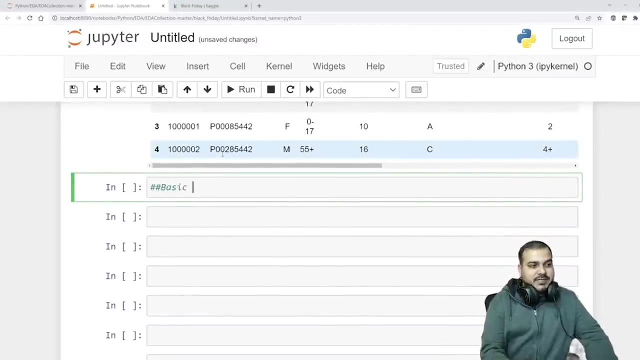 merge. if it is possible with merge, try to do it. instead of writing merge here, i could also add written append merge also. you can do it, it okay? so this was the next step. now let's go to the next step. everybody so basic, basic code that we have seen already right. one is dfinfo. we can check out this one. 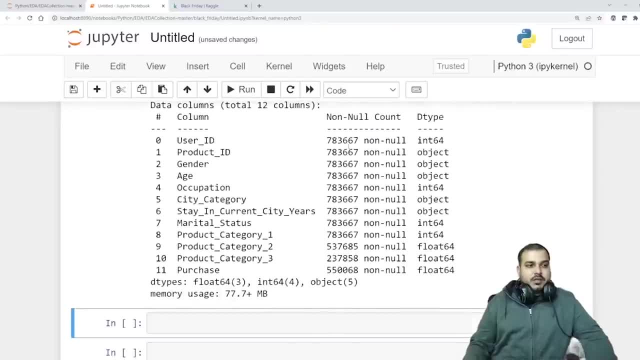 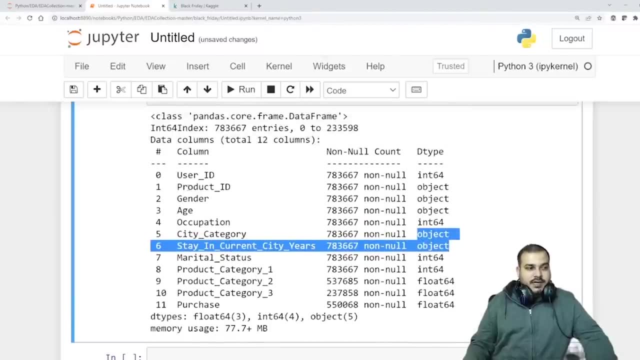 here. we can understand that. how many different types of features are here? so obviously, int is there, object is there. object is there, object is there. int is there. object, intent, float, float, float is there. so definitely, when you see product id, it will be a combination of both integer and 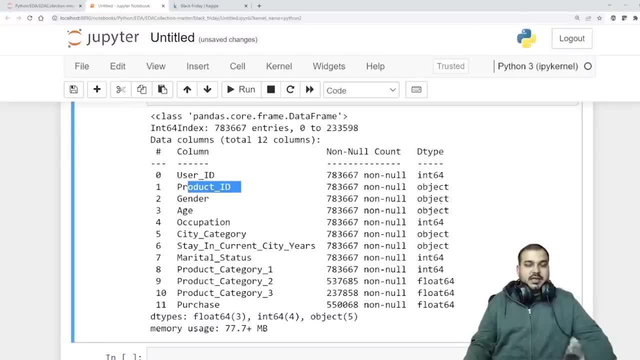 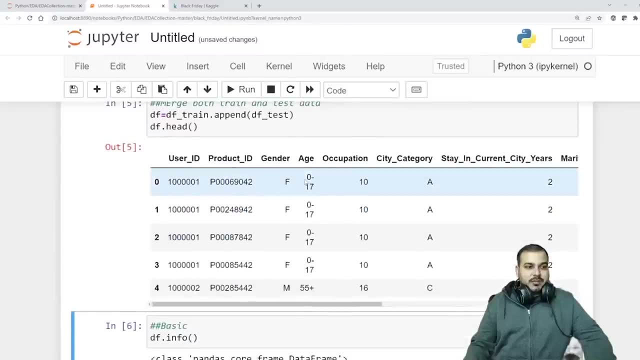 different values. so it is basically an object. then you have gender. obviously it has male and female, so categories, it is an object. age is basically an object. why age is an object? because here you will be able to see age is given in some range: 0 to 17, 0 to 17, 55 plus. so this i can. 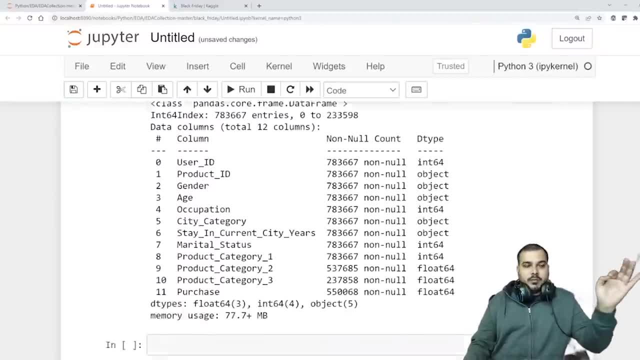 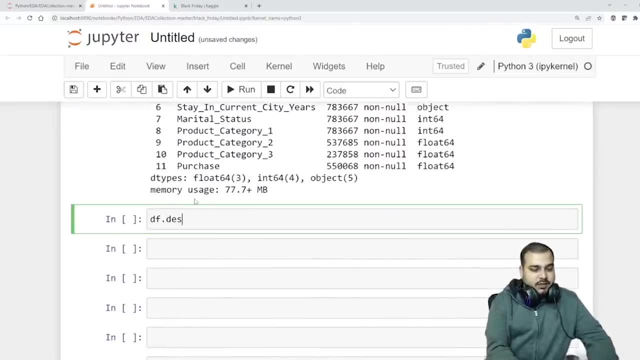 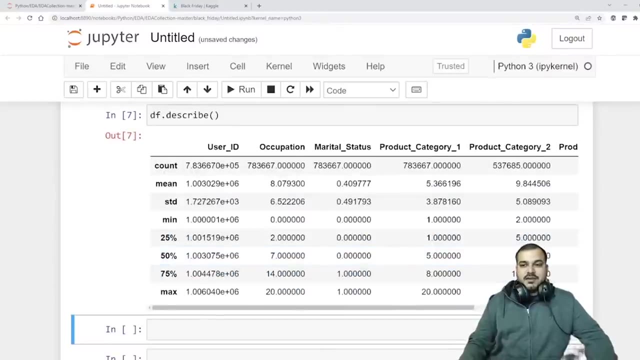 consider it as categorical variables. i'll also show you how to solve that particular problem also, but i hope everybody has got our understanding till here. the next statement that we are going to basically find out is something called dfdescribe, just to find out like what is the percentile values and all so here is just a basic information. 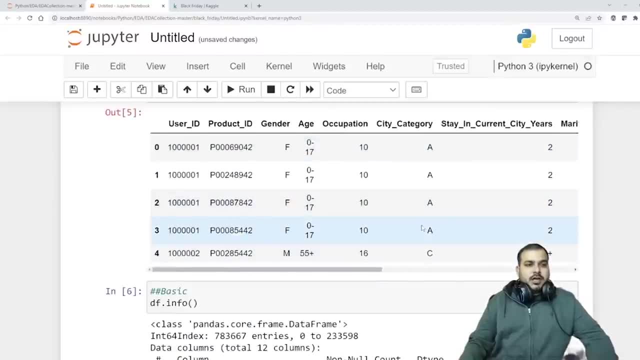 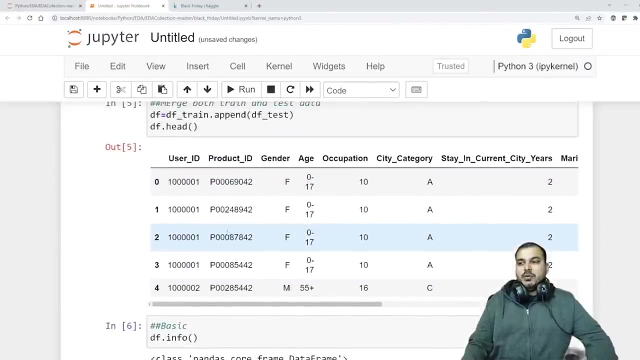 that we are going to differ. now tell me, um, which which column do you think out of? this is just waste. you can directly, blindly, you can, delete it. see, over here there is a column which is called as user id. user id is just a unique id over here, so you can definitely go ahead and 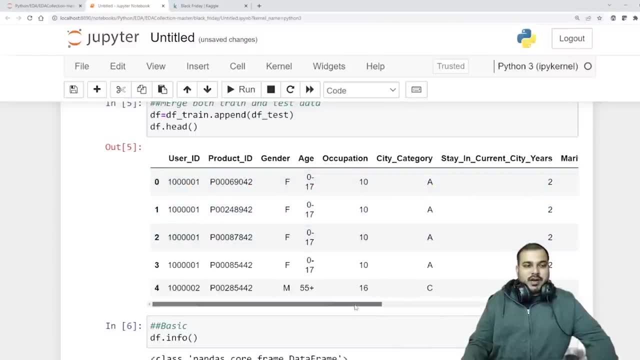 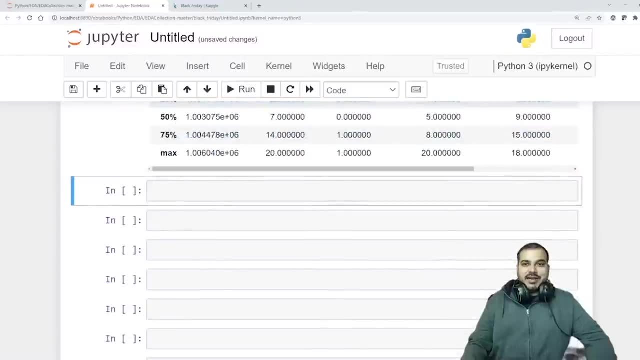 delete it. okay, user id will be of no use, so i'm going to delete it. so what i'm actually going to do? i'm going to basically write: dfdrop, um, dfdrop. this is a statement which will basically use to drop the feature. and here i can. 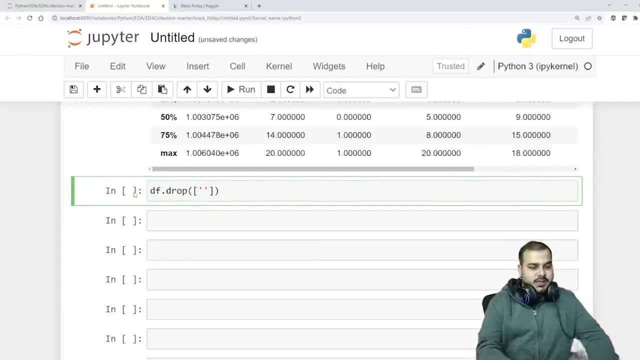 give any number of features, any number of features with respect to my feature name. so feature name is nothing but user underscore id. so i'm just going to copy this, paste it into my user underscore id and here one very much important parameter if i see in dfdrop is: 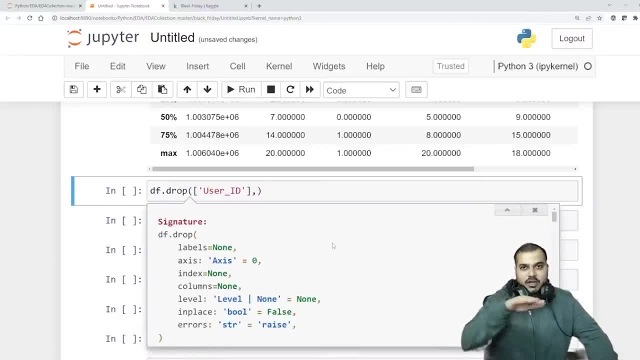 axis. axis is equal to zero basically means horizontally right row wise. axis is equal to one basically means vertically right, column wise. so we really need to drop it, column wise. so here i'm going to basically say it has, axis is equal to one, and here i'm going to specify. 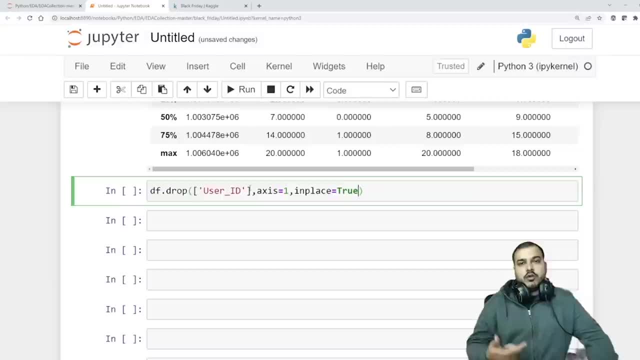 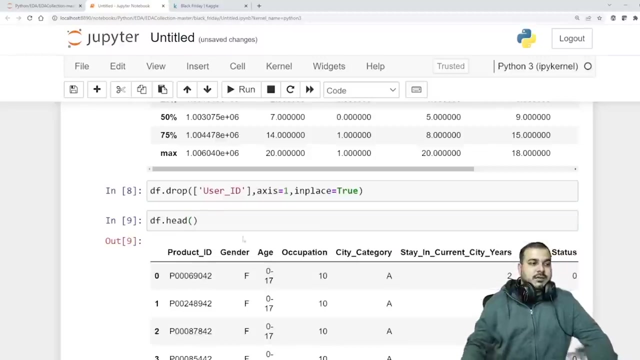 in place is equal to true. the in place is equal to true. what it will do is that it will remove the user id and it will update automatically into the df value. so if i go and probably execute it and now if i go ahead and see dfhead, you will be able to see that i'm actually able to see my 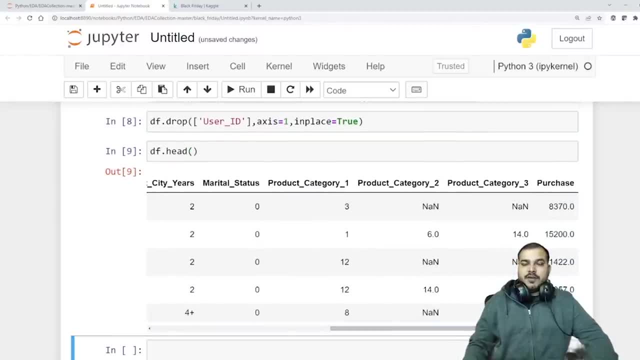 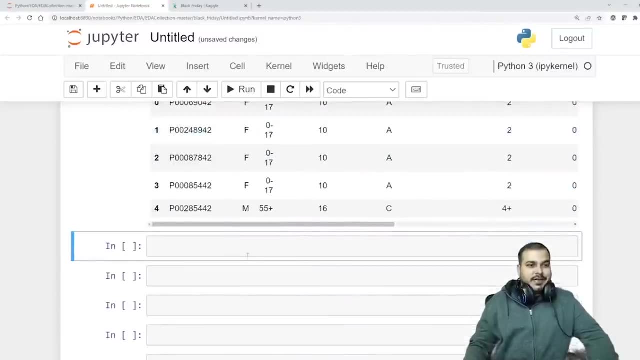 product id, gender, all the other information, perfect. so here we have basically done this. we have dropped the user id, we have dfhead, we have everything ready. now let's go ahead towards the data pre-processing side. now tell me, how many categorical variables are there? how many categorical variables are there? just by seeing this one, you have. gender, one, you have. 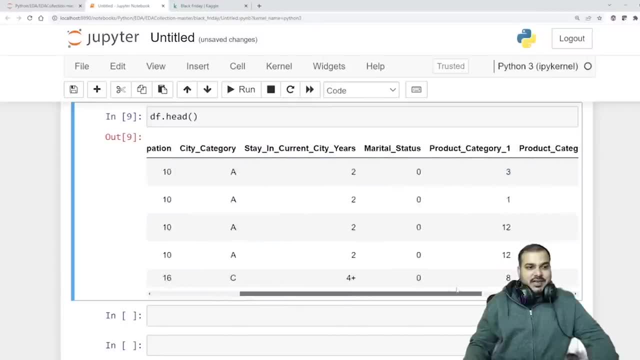 age one. you have occupation, city, stay in current city, this, this, this. but before that i also need to make sure that how many number of missing values are there. for the missing values, i may do something which i will show you in the later stages, but let's focus on fixing the categorical. 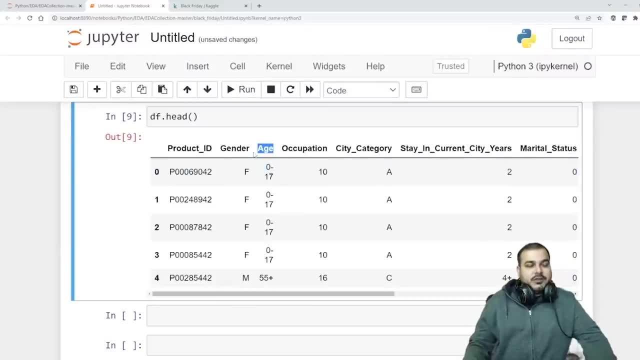 features right now. so how many category features are there? you see over here? gender is there, age is there, city category is also there. so we'll try to fix this category features, because our model will definitely not be able to understand, uh, how my categorical features will be there or not. 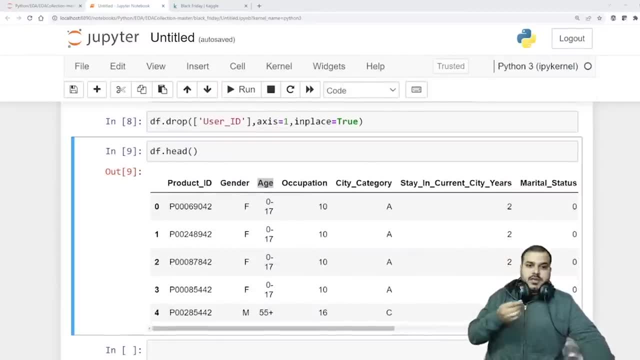 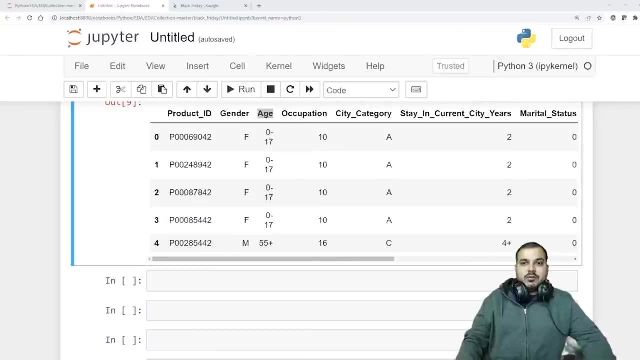 marital status is already in numbers, but let's see what all things will basically be there. so let's go ahead and take up age and try to solve this. convert this categorical into uh, uh, category into a numerical. we'll try to do that, okay. so first of all, let's focus on this and let's go ahead. now tell me, with respect, 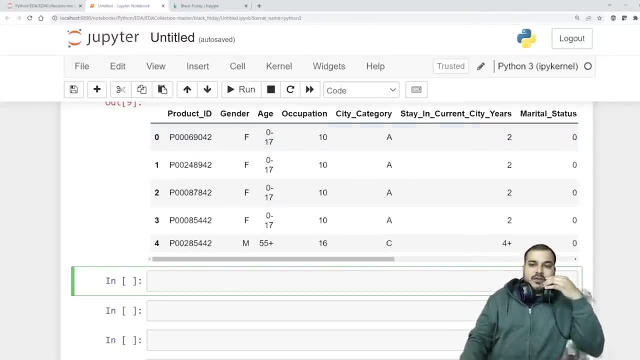 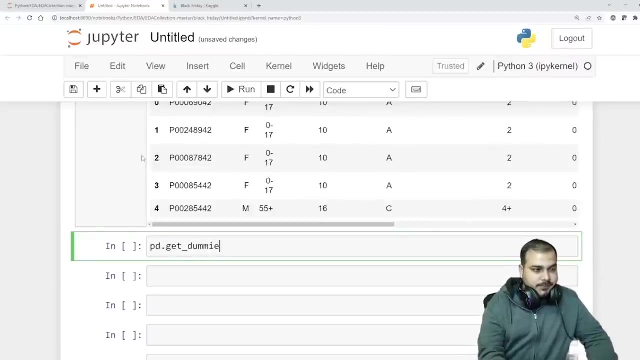 to gender. i have male and female right with respect to gender. i have male and female. now what should i do in order to probably in male and female? what kind of encoding i can definitely use so if i write pd dot, get underscore dummies and if i give my df of gender? 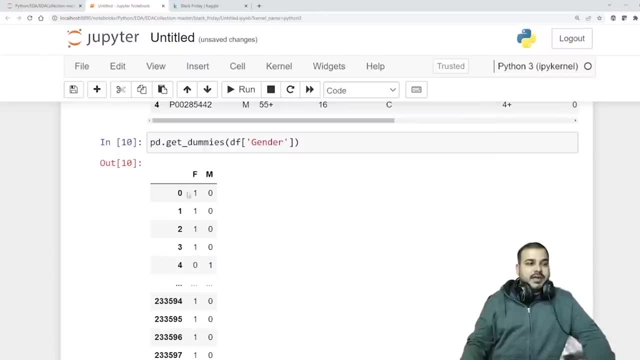 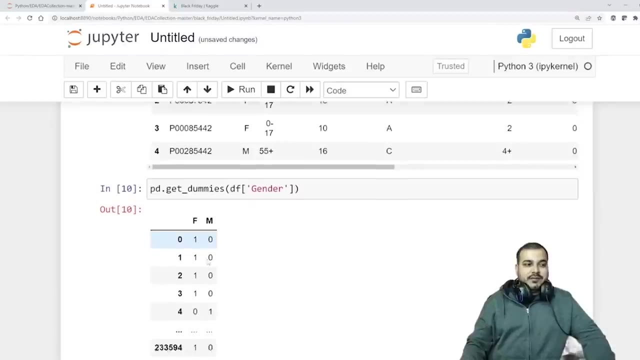 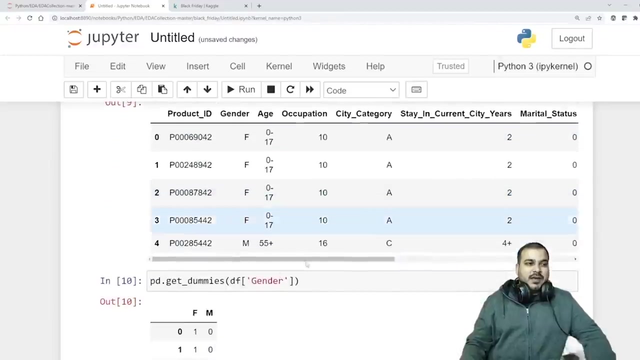 if i execute it here, i'll be able to get either male or female. so here i'm actually getting ones or zeros right. one is basically given to f, zero is basically given to male. okay, so either in this way you can do it, but again, see what is the problem here. if i convert in this way, then i have 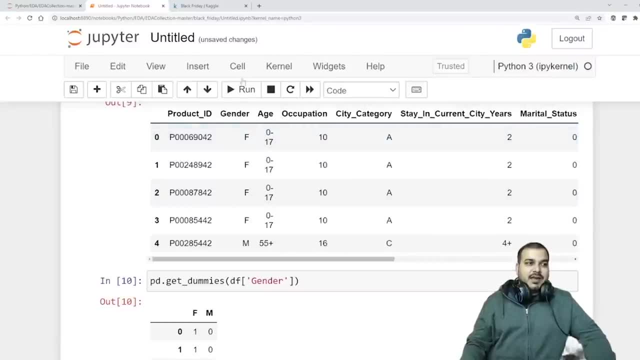 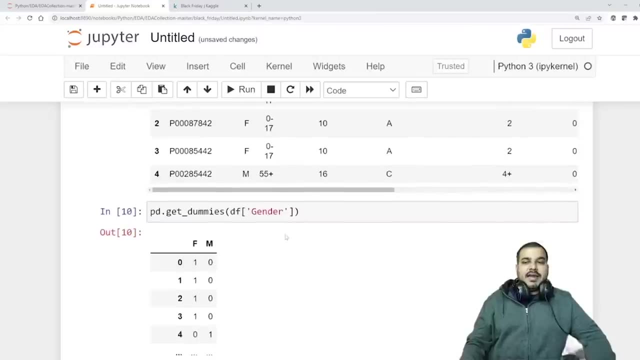 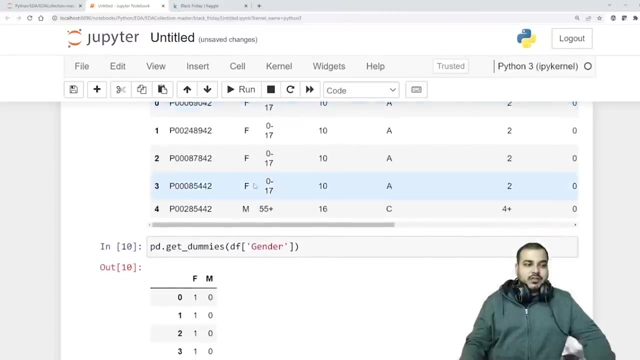 create another data frame, then i have to add this data frame over here, then delete this gender column. can i do something within the data set itself where probably i can directly convert this? wherever the f is zero, sorry, wherever the gender is f, i am going to convert this into zero or one. whether m, whether the gender is male, i am going to convert it to zero. 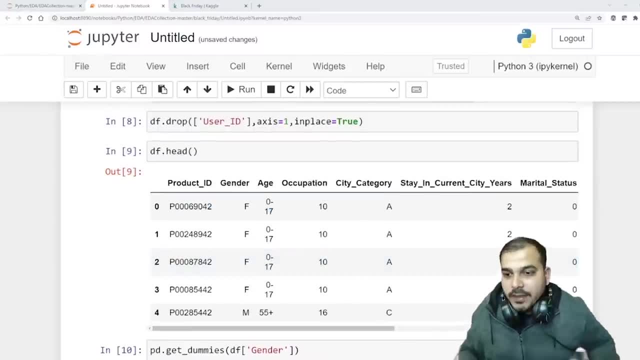 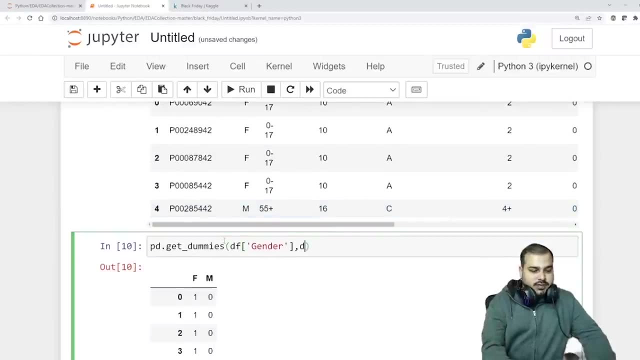 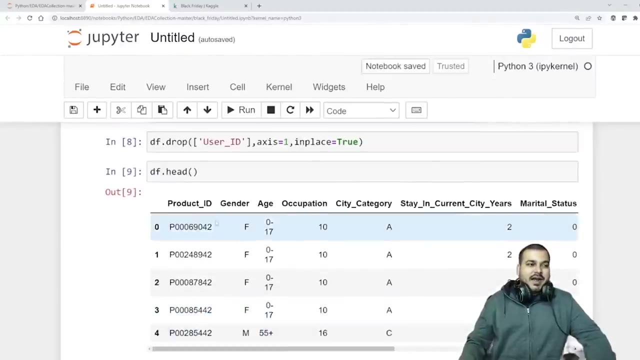 to one. so how we are going to do that, guys, how we are going to do that, yes, i can definitely use drop. drop underscore first is equal to one. i can definitely use over here. but understand, i don't want to do in this way because i have to save this somewhere. then i have to add a column over. 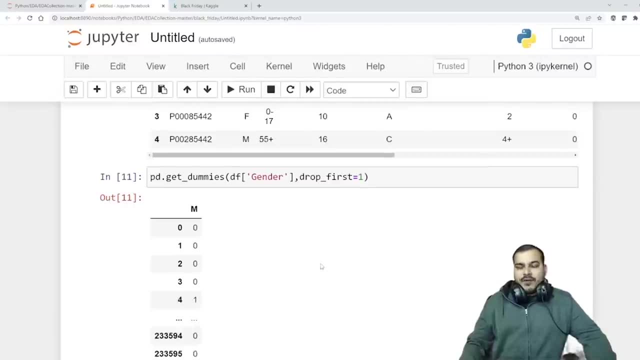 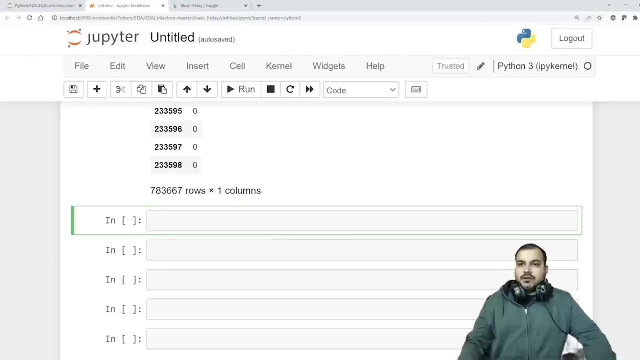 here. i don't want to do in that way. i want to find, i want to find out a way where directly i have to do it over here itself, in this particular data frame itself. so how do i do it? so for this i will be using a code, simple code. so i'll write df of gender and here i will say df of gender. 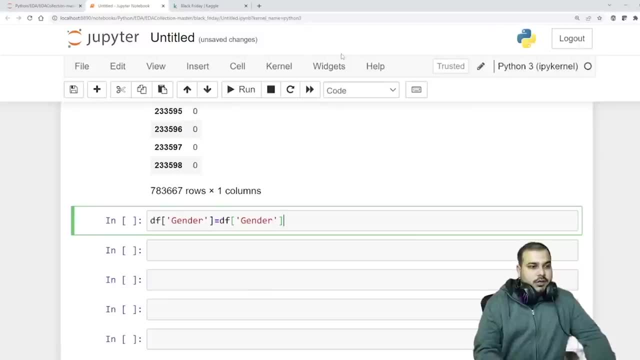 dot map, map method. what it does is that. see what does map method do? map method will basically map with respect to the conditions that i'm giving over here. so here, if i say my first condition is that wherever i get female, i'm going to convert it into zero, and wherever i get male, i'm just going, 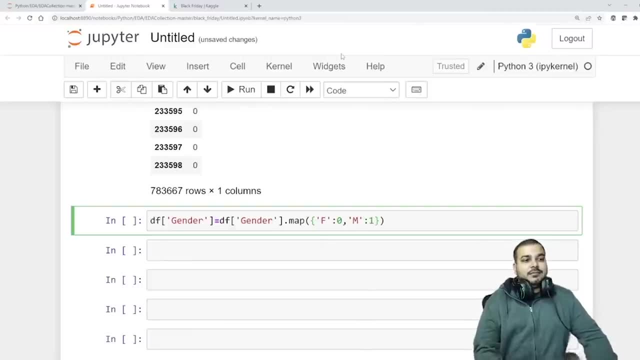 to convert it into one. many people ask me when i'm teaching what is the map functionality in python? so here you can see easily within this particular data set. you will be able to see it over here. now, if i write df dot head and if i probably see this: 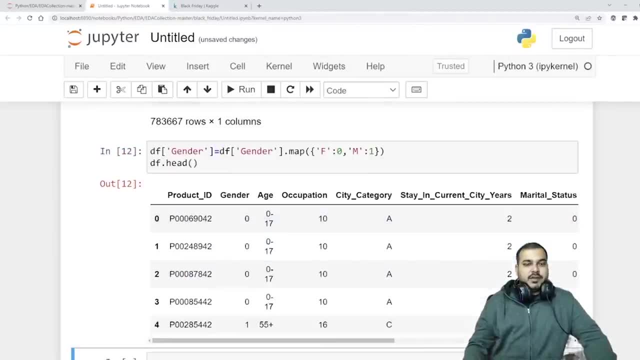 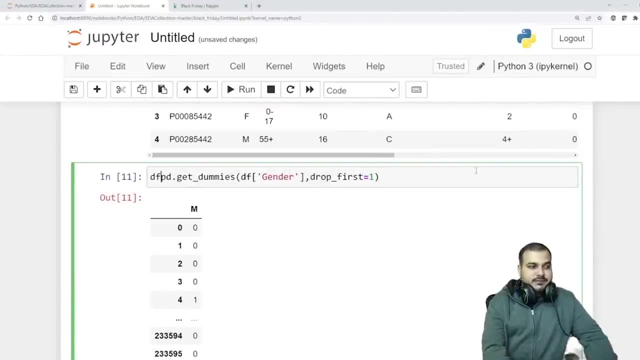 you will be able to see now, gender will be zeros and ones. so everybody write down this code, okay. one more way is that directly i assign this to df of df, of gender, right, so this way also you can do it. so both the ways, whichever way you feel you want to do it, just do it both the ways, it will work. 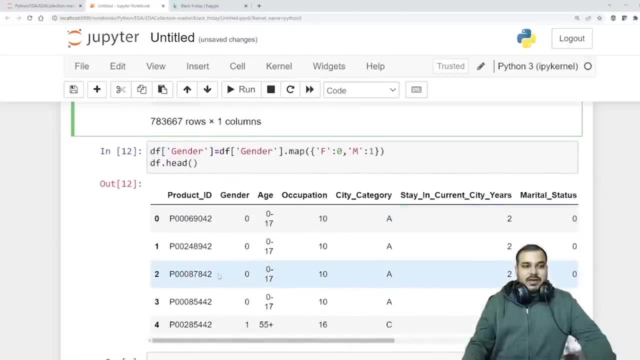 this is not ranking guys. zeros and ones are not ranking one, two, three, four, five, six is basically ranking. uh. zahid hassan says: do we have to apply feature engineering on training set only or test data? no, on both. on both you have to apply. i'll show you how you have to apply both. 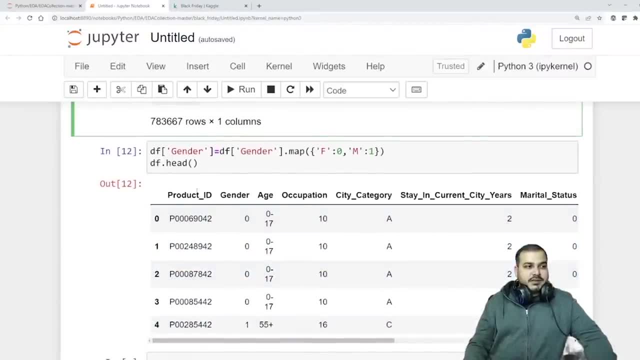 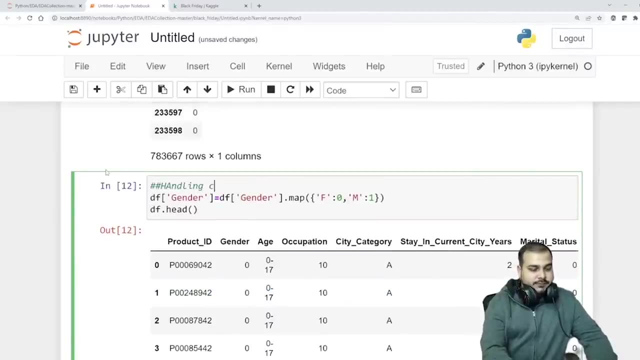 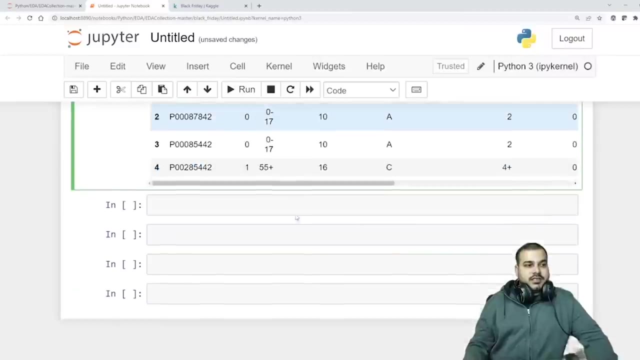 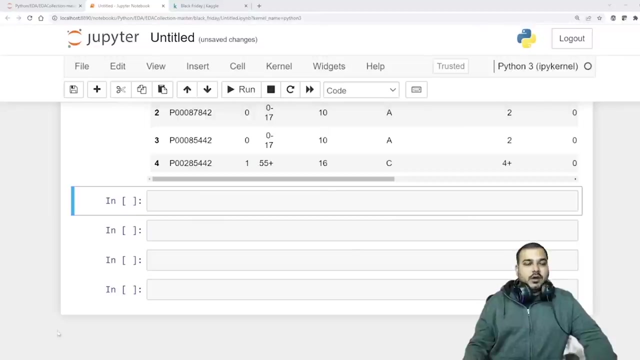 okay, perfect. so everybody has done this right. so this is with respect to handling the categorical feature. handling categorical feature: age, sorry, gender. so this is done now. let's go to the next step. now, the next step, what i'm actually going to do. gender is done. now we also need to handle age. 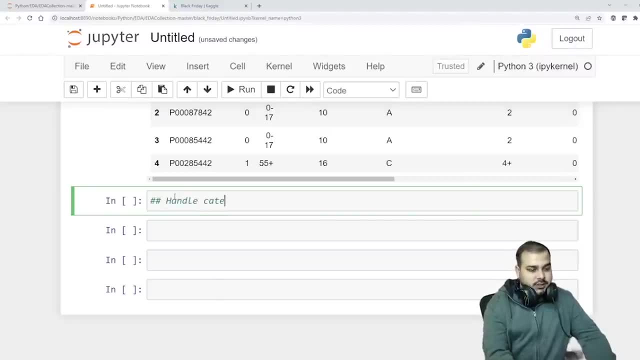 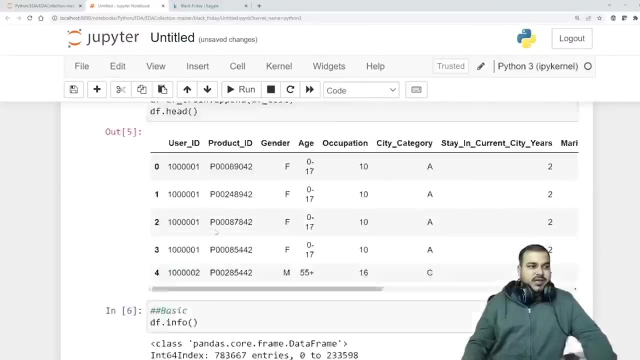 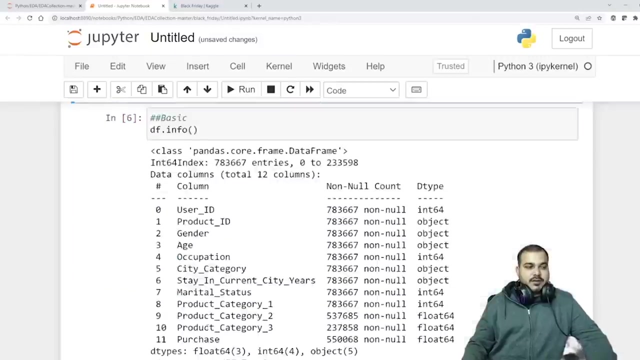 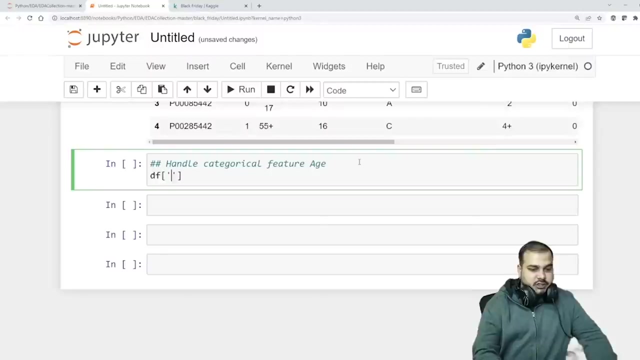 handle categorical feature age. now why i'm saying specifically saying age? because here you go and see age is what? age is also a categorical feature, see 0 to 17. 0 to 17- 55 plus. so first thing, i will try to execute something like this: i will write df of age. 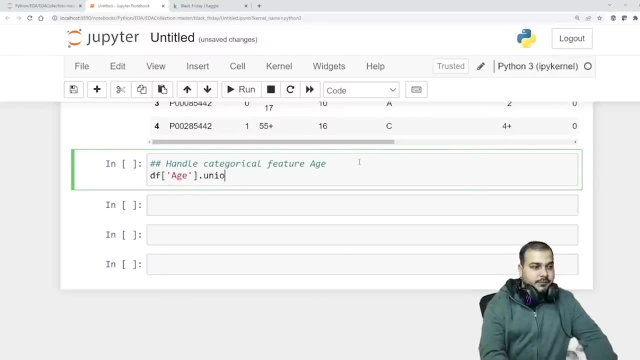 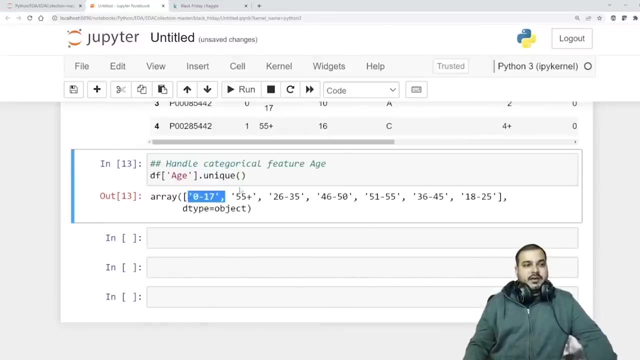 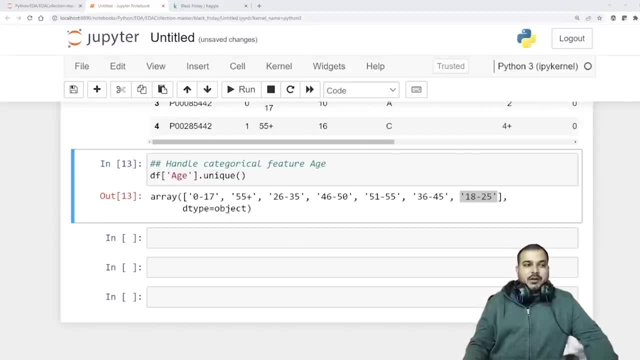 now, if i have, in this particular unique way, not tell me how should i convert this categorical feature into some numerical feature? so here also i can actually do encoding. so the type of encoding, what i will probably doing. many people will again get confused over here. so why, why you're doing like this? 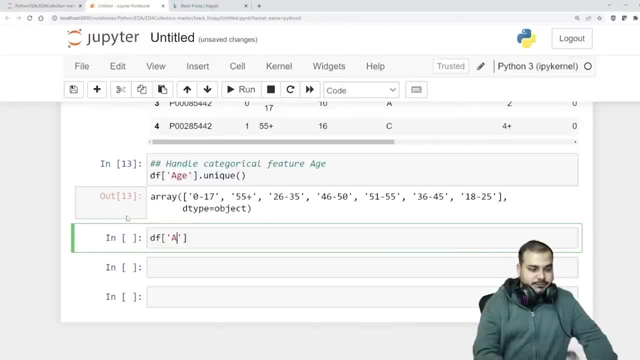 so i'll just tell you. so you're also. i'm going to use the f-dot page and i'll assign it to the f of age right. i can definitely do one is directly get dummies. you can directly do pd dot, get dummies. see this: if i write pd dot, get underscore dummies right, and if i give it for df of age, i will. 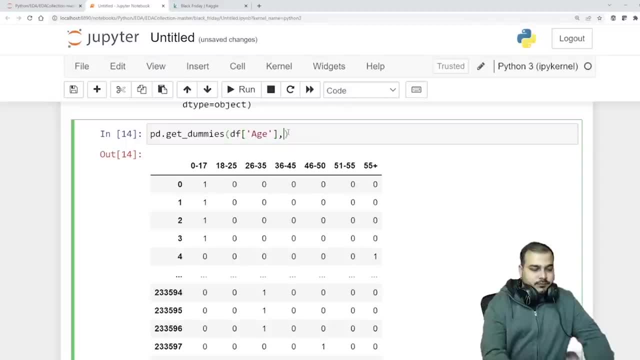 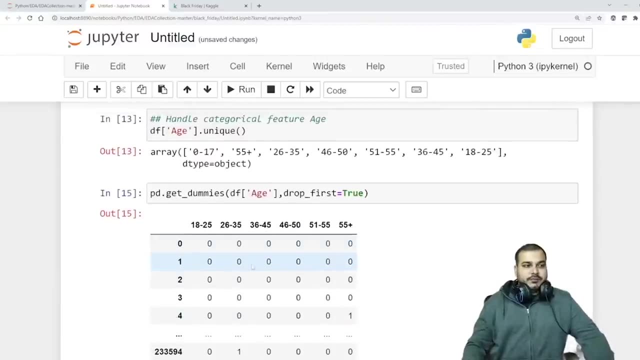 be able to get like this: right, and if i drop- drop first is equal to true- then i will be able to get like this. then what i can do, i can save with this column name and i can put it inside my data frame. i can do this, okay. but just imagine something, guys: here. a domain knowledge will 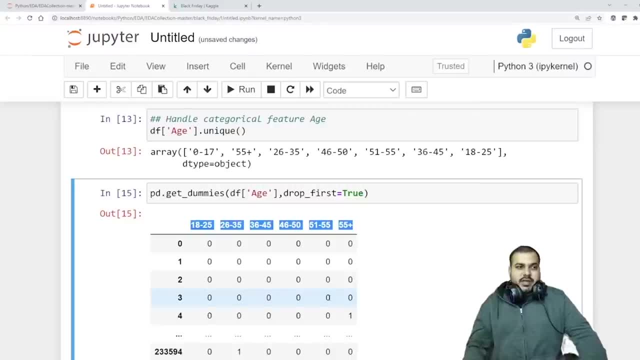 definitely come. one very important thing: do you think like shopping 0 to 17 years, it will be very less right in an e-commerce website. it will be very, very less right, whereas if i say 26 to 35, you can get like this. then what i can do, i can save with this column name and i can put it inside. 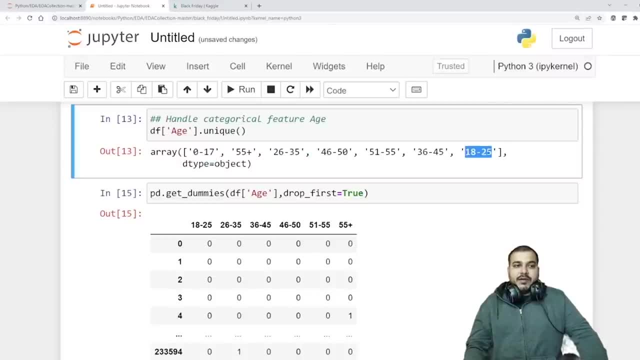 it may be more. and where i say 18 to 25, it may be more, 15 to 55, it may be more, 55 plus, it may be very less right. or 46 to 50, it may be also very, very less. so here, what we will do is that we'll. 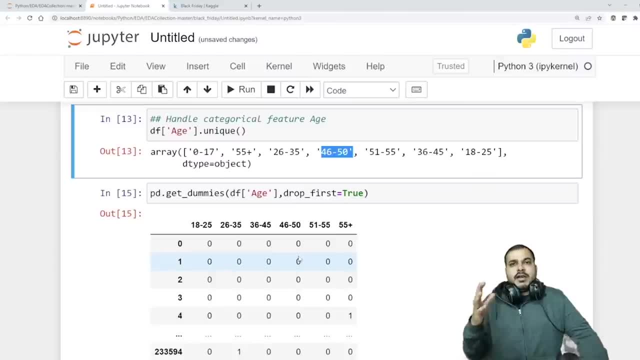 just not try to convert this into dummies. let's do some ordinal encoding only. let's let's give some rank to it. okay, let's let's give some directly some values like 0, 1, 2, 3, 4, 5. why i am saying to: 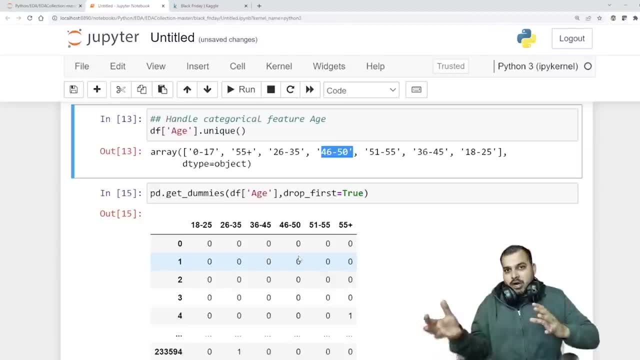 give 0, 1, 2, 3, 4, 5, because if i'm training the model, my model maths will definitely be able to understand right. my model maths will definitely be able to understand with respect to the values that we are given, like 0, 1, 2, 3, 4, 5, whatever values i'm actually given with respect to the other. 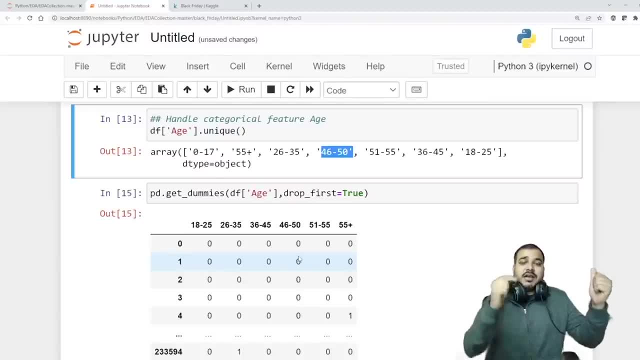 features my model will definitely be able to understand. this is also called as target guiding. so we will do something like this, okay, but this, this will definitely not work. this is not a very good practice also. so here i'm just going to comment it and then i'm going to give 0, 1, 2, 3, 4, 5, because if i'm training the model, my model maths will. 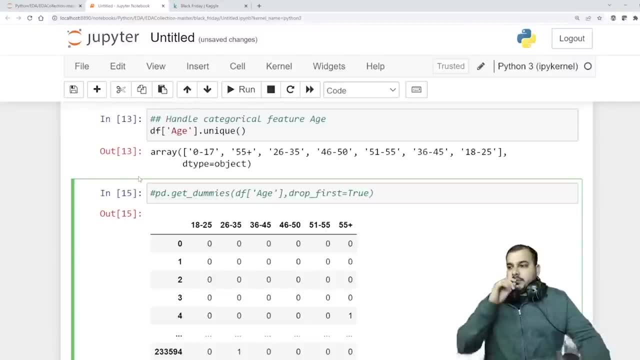 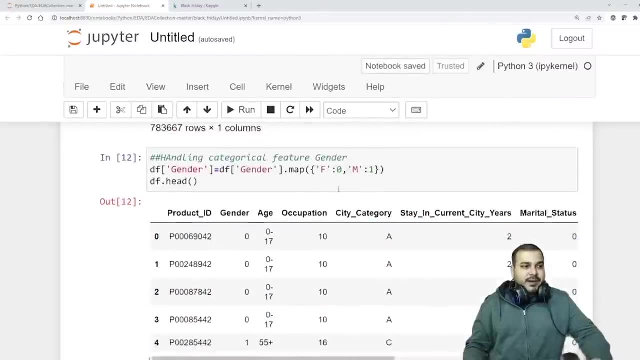 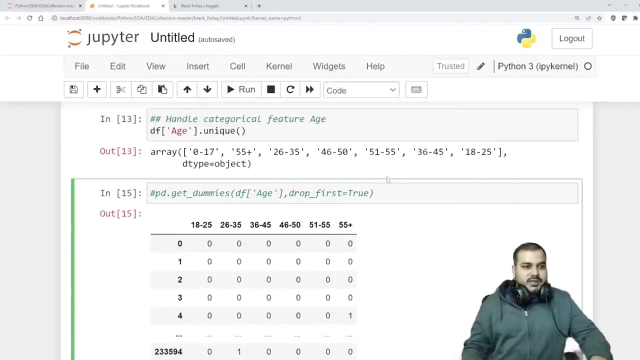 it out, and this will definitely not work. instead, what i will actually give is that i will say: let's apply the same map function which i had applied over here. so here i'm going to basically give in this way map function and i'm just going to basically put it inside this here. 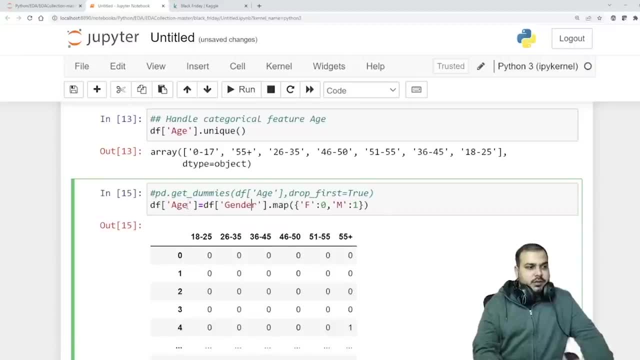 definitely. i'll say age. this age and mapping i will do for 0 to 17. first. let's say for 0 to 17 i am actually giving some numbers. let's say i'm giving it over here as 1 because at least some value should be there. then 18 to 25 in the sorted order i'll try to give. 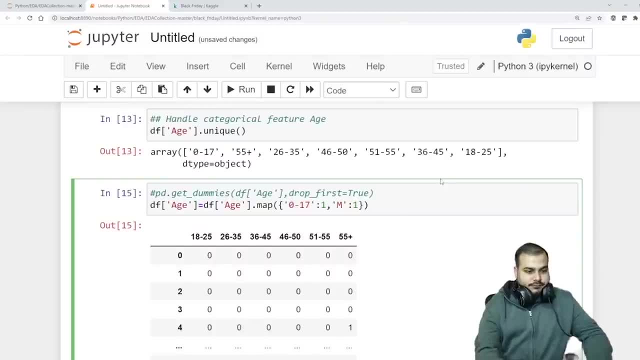 18 to 25. my second one, and here i will give it as 2, then third one, again in the sorted order, 26 to 35. i will give it over here because see my model. maths will definitely be able to understand this. when i'm training my model, it will be able to understand. this is called as target guiding. 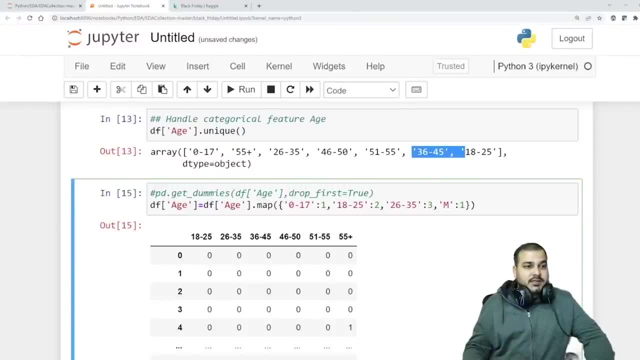 target ordinal encoding. then, uh what, we have 36 to 45. i hope i'm doing it right colon here. i'm actually going to give it as 4, and then, after 36 to 45, i have 46 to 50. 46 to 50, i have 5, and then i'm going to give it as 4. 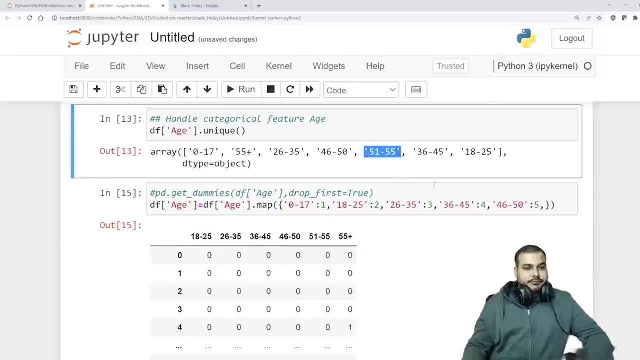 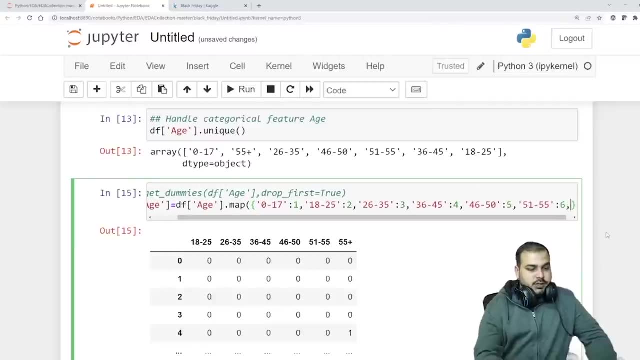 i will be writing 51 to 55 and i will say it as 6 and then 55 plus i'll say it as 7. label encoding can also be done. label encoding will also work. perfect label encoding will also work. but again, understand for this, again you have to. for label encoding, you have to import a library and 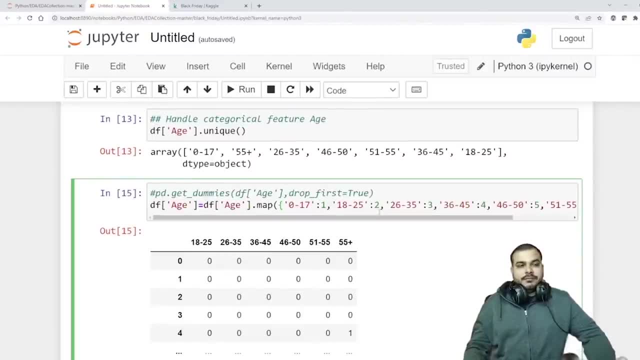 then perform it here also. you can do. this way, you will become good at maths. don't put zero, guys. see, as i said, i, as i'm saying right, there will be some mathematical equations that will be happening. so if you want to do label encoding, how you'll do, 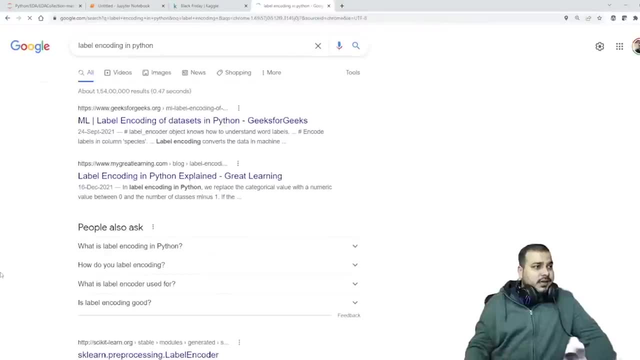 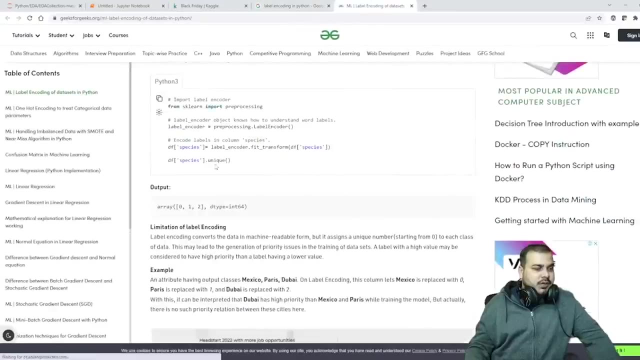 label encoding in python. let's see some articles. uh, i have some article from geeks for gig, so let's see. so i have to basically upload this entire thing, right, this entire code- see entire code- by using pre-processing label and all. but i don't want to do it because as i get a new data set, 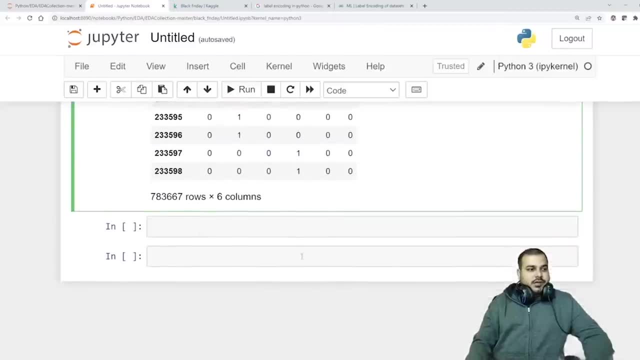 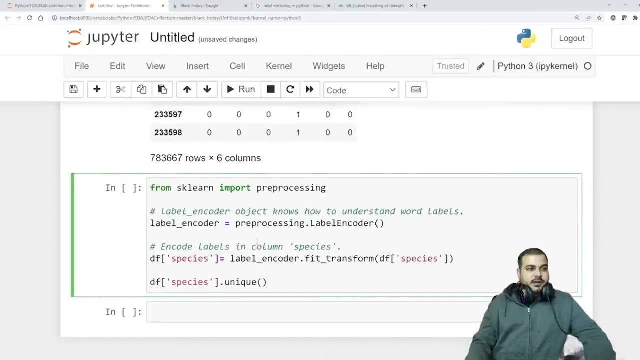 over there also. i should be able to apply all these things, right. so here i'll just copy this from sklearn you can see over here, right, and then you can basically do it with respect to df dot age and df dot age, so you can execute this and all. 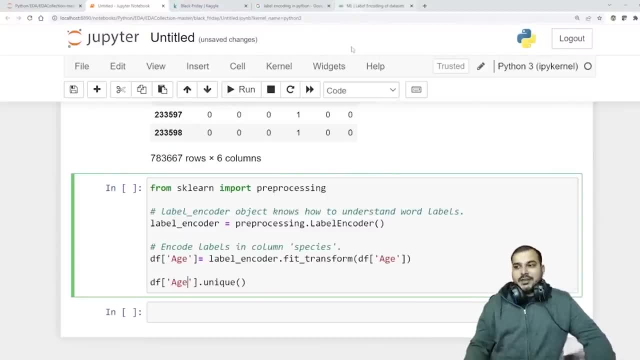 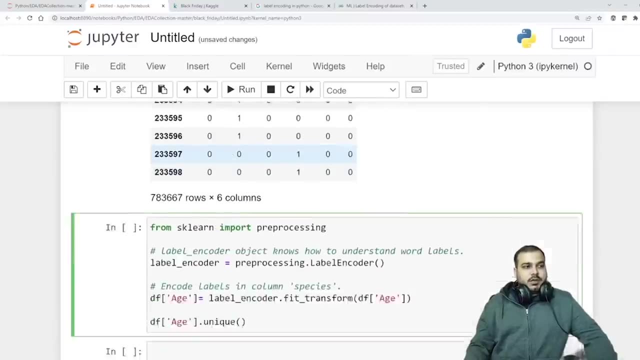 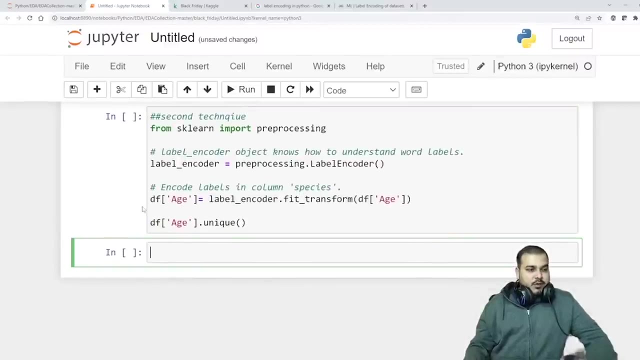 automatically. it will work. do not hesitate to google. it is up to you, right, it is up to you, so you can also do this in this way. this is the second technique, so i have already done this. now, if i probably go and see my df dot head, you will be able to see in. 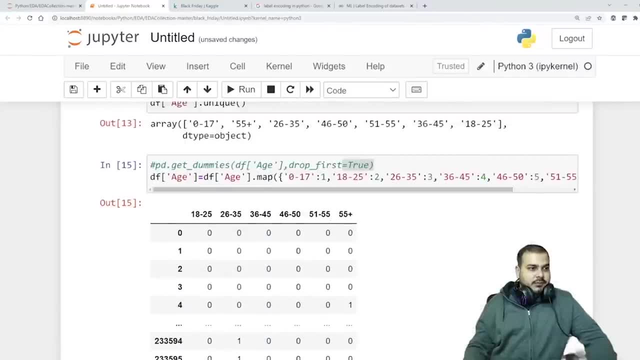 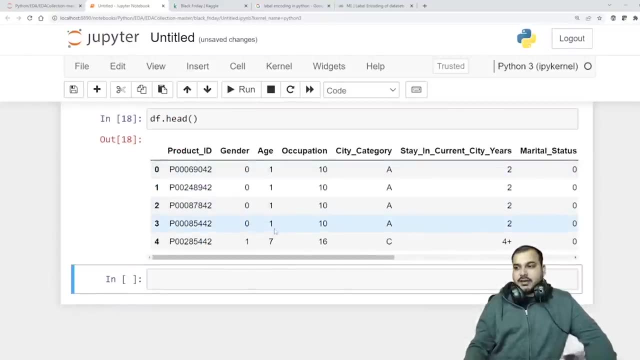 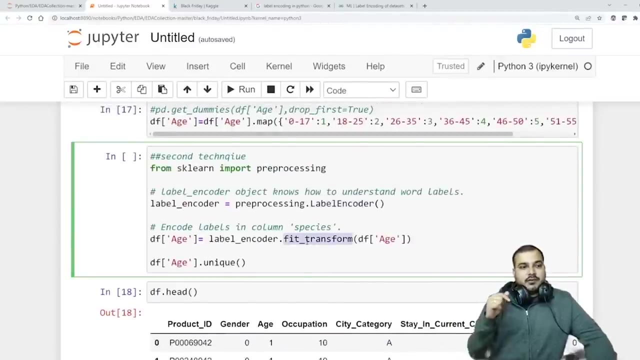 age also, i'll be okay. i have not executed it, so i have executed it now. if i go and see my df dot head, you will be able to see one, two, three, four like that you will be able to see. see, there will be hundred of ways: label encoder, fit, transform for the test data. you have to do transform. 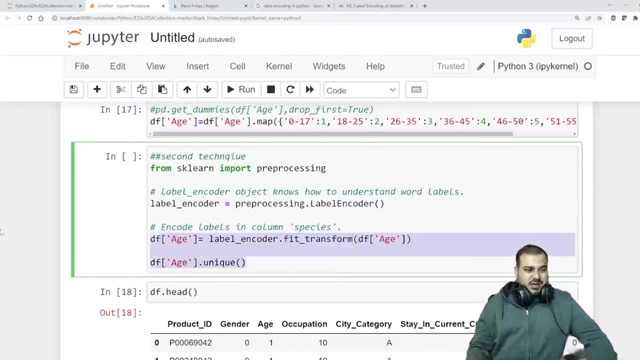 but here i've actually combined it, so this is not a good practice for this case. suppose. if i'm doing for train data, for test data, i will just transform it. no need to give any any any weightage, guys see, our machine learning model will automatically understand. 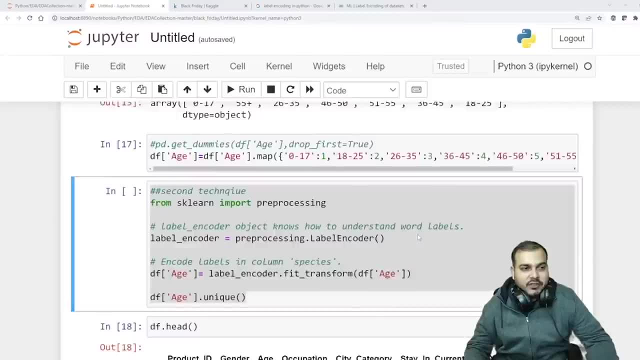 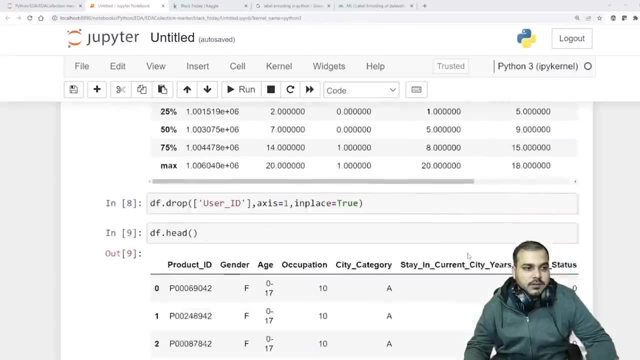 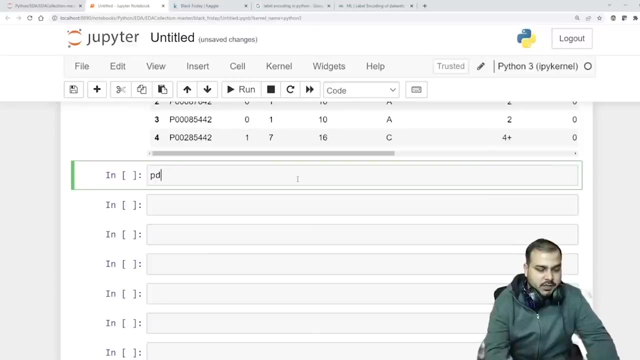 so one more thing, category that i have actually, we have actually seen, is something called a city categories see. oh yeah, city categories also there. so for this i will just use pd dot get dummies, if you want pd dot get dummies, and then you can basically combine them. 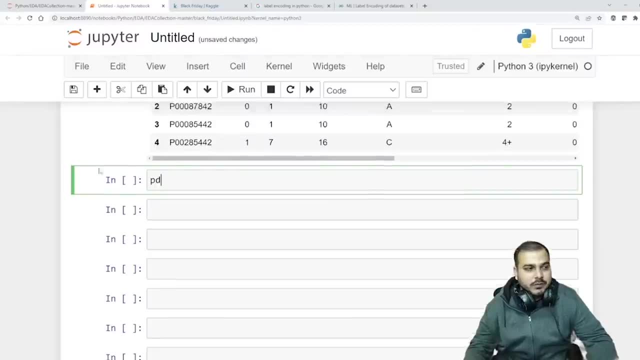 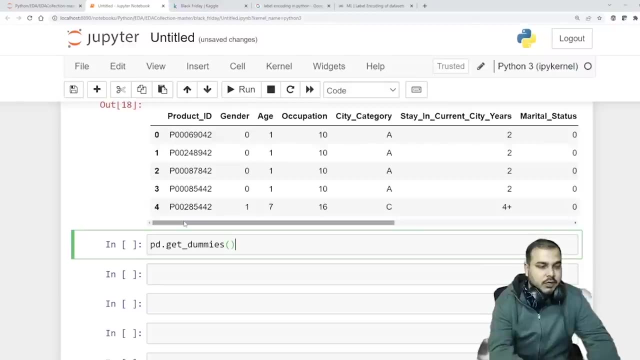 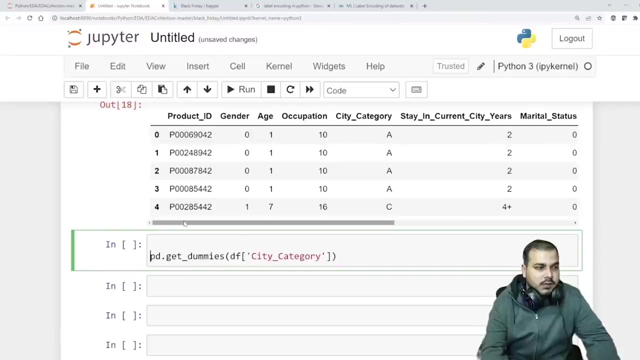 but in order to do that also, uh, what you will do. so here i can basically say that pd dot get dummies. and then i'm basically going to give my df of city name is city category. so fixing categorical, categorical city underscore category: pd dot get dummies. df of city category. and here i'm going to basically say, uh, 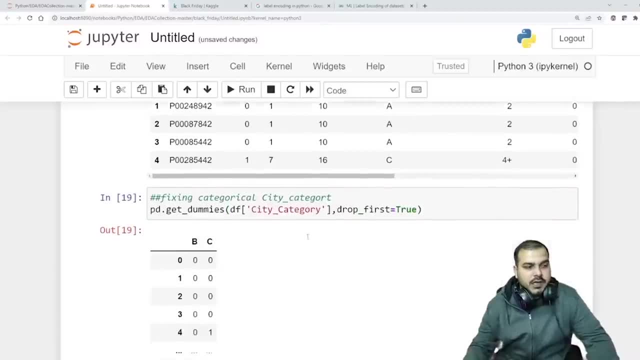 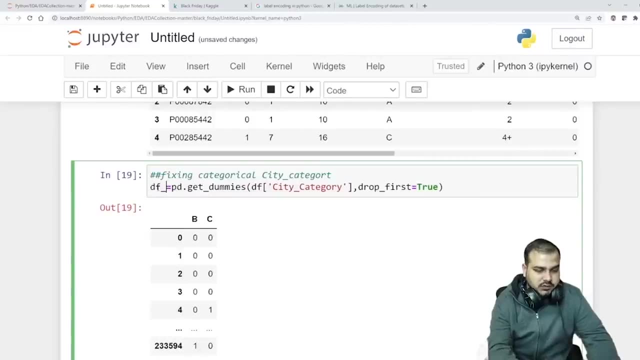 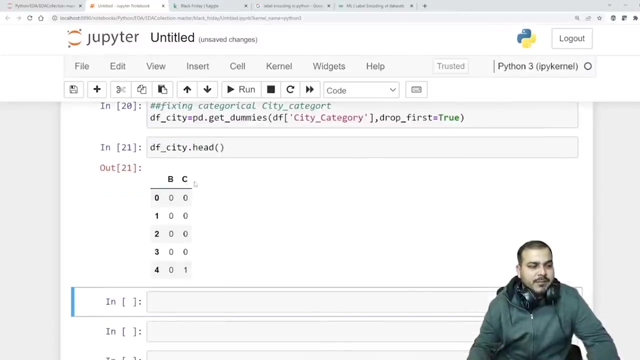 drop first is equal to true. so here i have all my values. so i have. I'm just going to save this. in one variable where I'm going to say df underscore city, Let's say so. df underscore city is this one dot head. Now I have to combine this entire cities with this df okay, which I have actually shown. 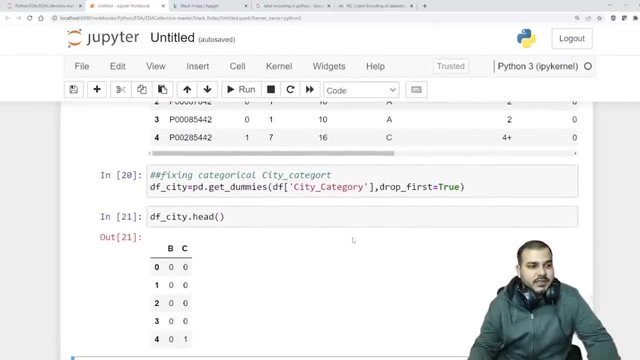 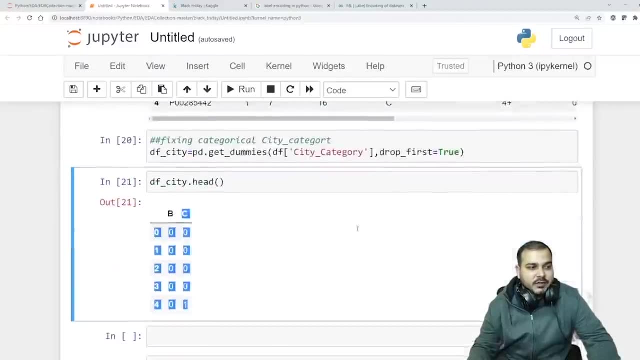 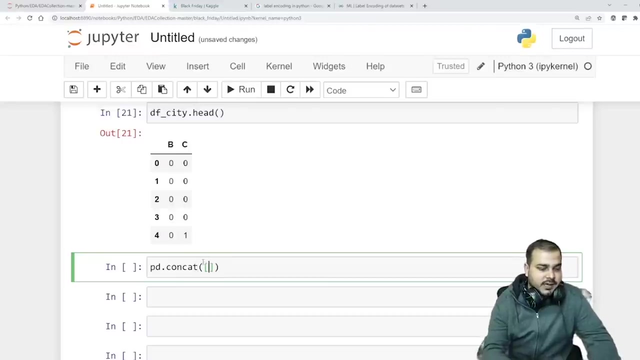 you before and now I hope everybody is done till here. So this two features will now get combined to this data set. Now, in order to get combined into this particular data set, what I will write is that I will say pd dot, concat, and then here I'm basically going to give df and df underscore city. 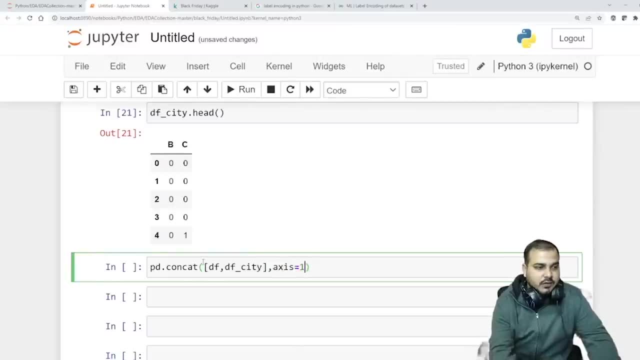 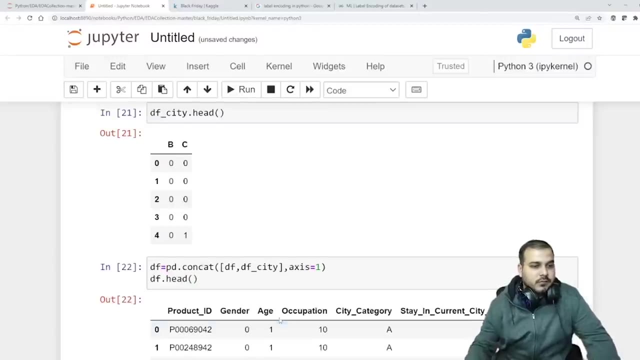 And when I'm doing concatenation I also have to give my axis value as one. So this I will save it in my df and this will basically be my df dot head. So if I go, probably in the last here, you'll be able to see b and c. 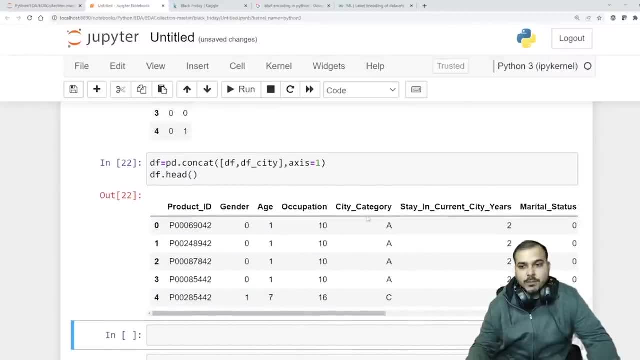 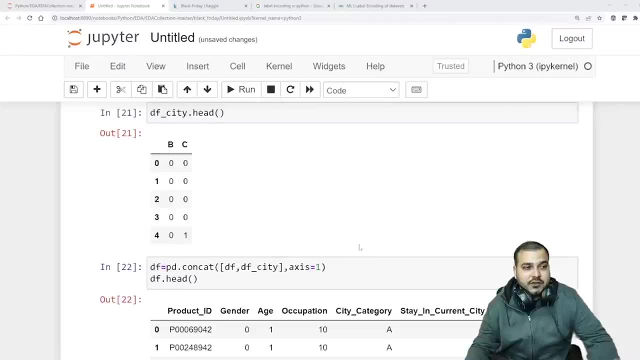 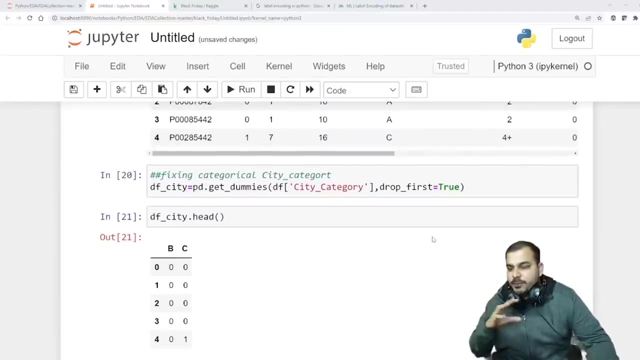 Now, Now I don't require this city category. I can drop the city category, but I hope everybody is able to understand. So why drop underscore first is equal to true, because always understand if I have three categories, two categories is sufficient to represent all the three categories. 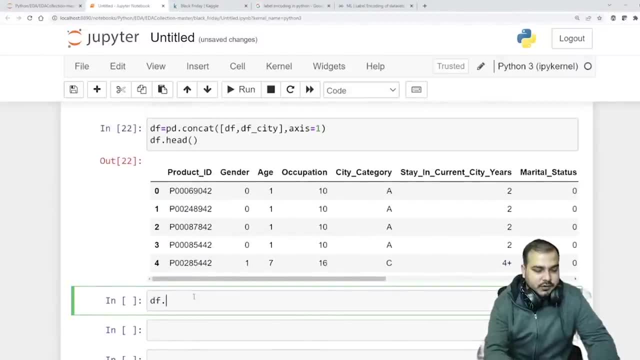 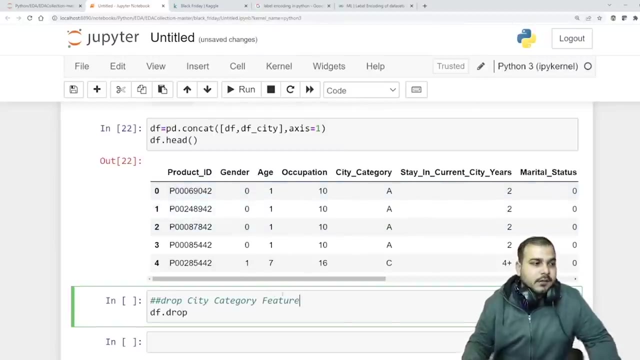 Now let me go to the next step. Let me quickly drop, So drop. I'm just going to write drop city category, Because I don't require this feature. now, right, I don't require this feature, city category, right? So I'm just going to do df, dot, drop. 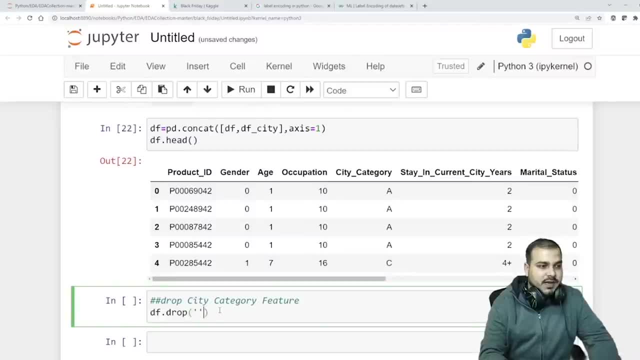 And here I'm just going to basically say my category name, which is city category. But again, I understand, here your axis will be one. So what is the error? Not found in axis Why? Why, Okay, It is city underscore category. 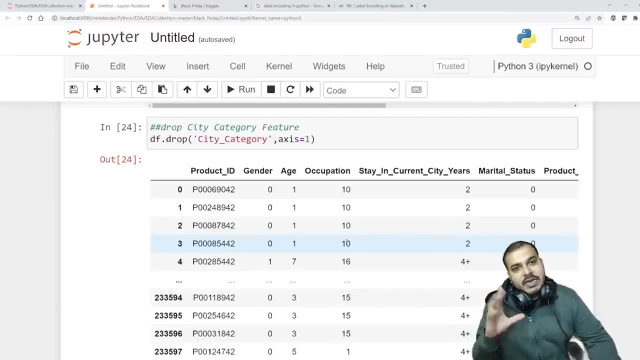 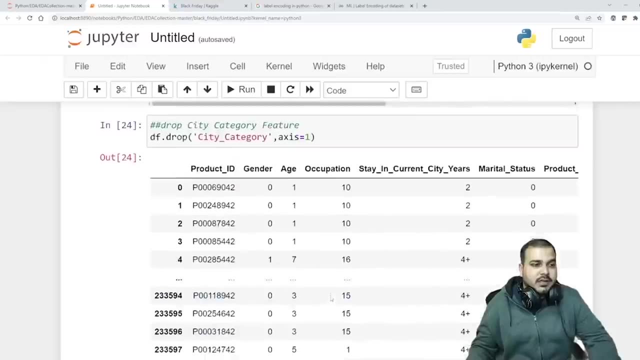 Guys understand why we are doing this: because any new data will come. We have to again follow this entire thing. Okay, This is entire steps. We have to follow whatever things we have actually done. This encoding everything will be done. 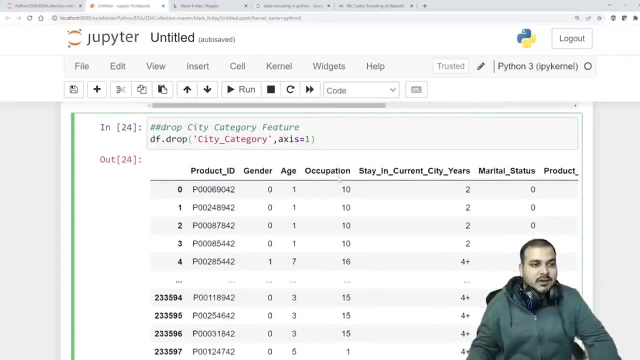 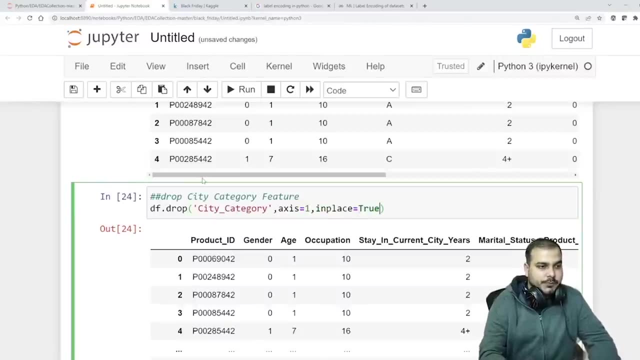 So here you can see df dot drop city category axis is equal to one. That particular feature is gone. So what I'm actually going to do to make this operation permanently I'm going to use in place is equal to true. So if I now go and probably check df dot head, 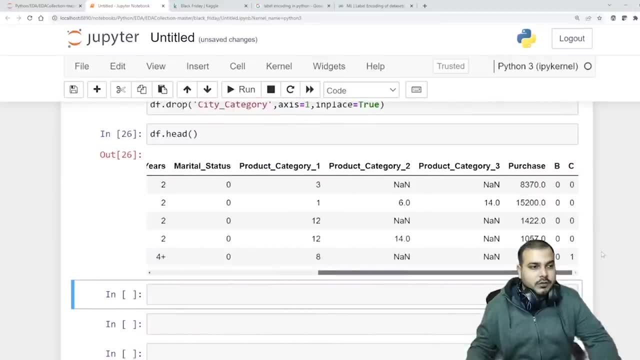 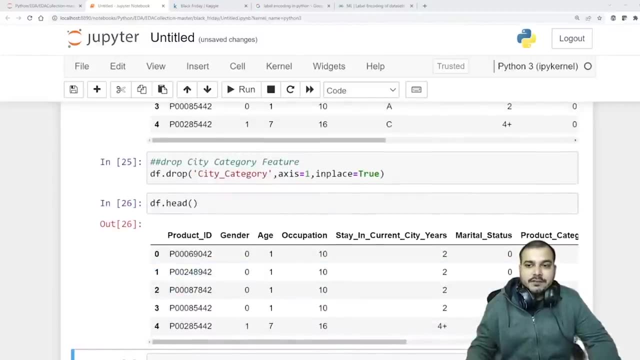 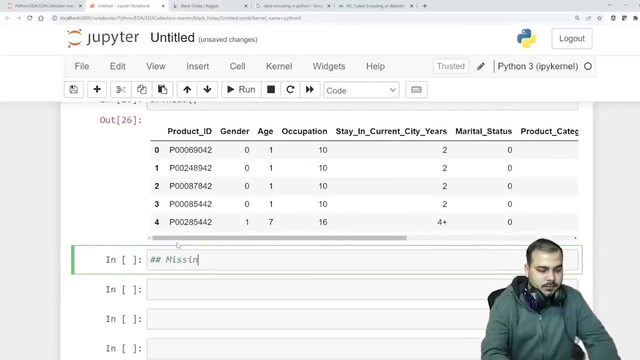 Here it is entirely So. BC is there, This is there. So we have fixed all these things still here. We have done a better work till here. Now let's go ahead and check the missing values. Missing values: City category is a category feature. 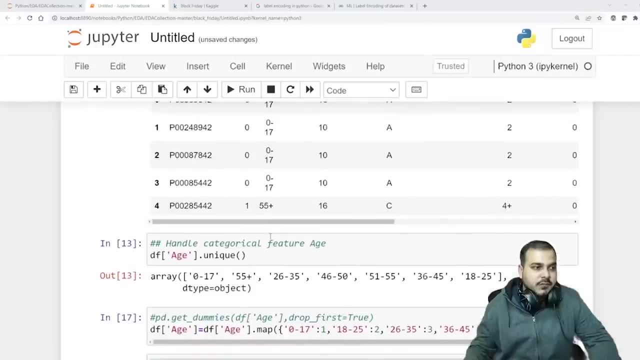 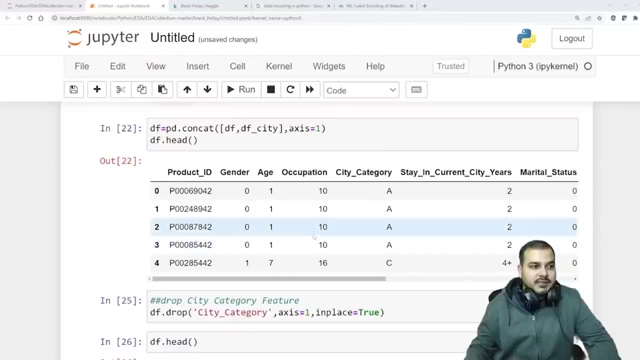 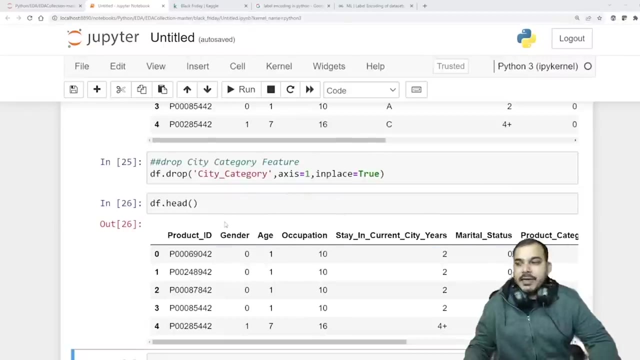 City category, one is another is age and one is gender. So three categories We have Spent Fixed up. Axis is equal to one basically means column wise We are adding or we are appending that specific data frame In this axis is equal to one basically means we are deleting the column. 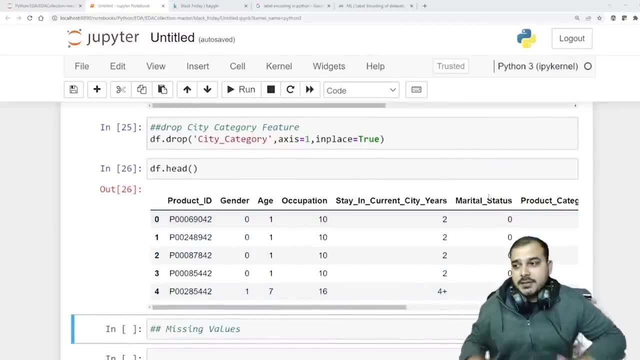 Guys, again I've told you EDA basics. The prerequisite is that you need to know Python. You need to know some basic things. If you are not knowing, it Difficult. Now, with respect to df, dot is null Missing value. 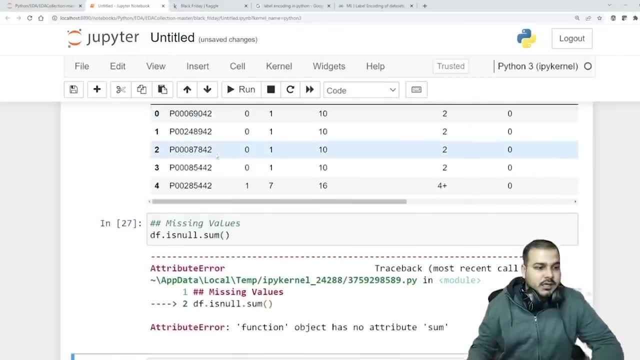 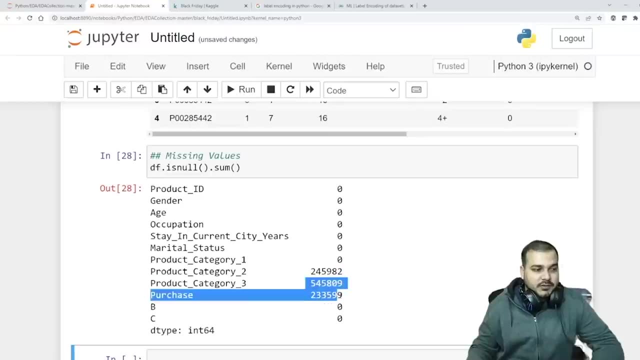 What I'm actually going to do. I'm just going to do some df dot is null dot sum. This is also a function. Now, here you can see: product category has so many null values. Purchase also has so many null values. Product category two has so many null values. 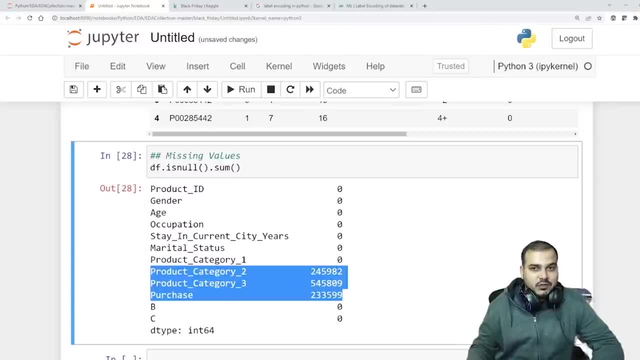 Product category three has so many null values. Purchase has so many null values. Amazing. Now, whenever null values are there, people will get shocked. what to do now? Everybody will get shocked. what to do now? Okay, categories are there. Should we replace categories with something? 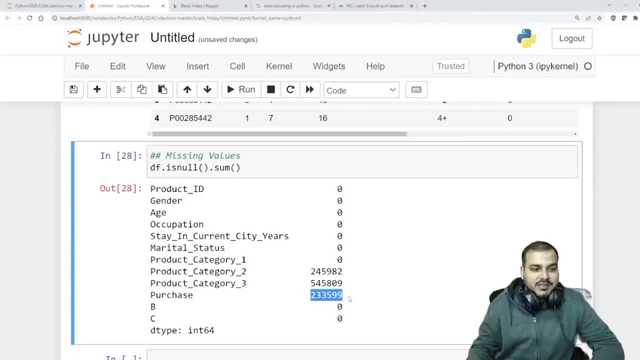 Just tell me, Purchase, why null are there? Because this is the test data, The null values that are present, that is the test data. That should be null only. But this two, we should definitely fix it up. right, This two, we should definitely fix it up. 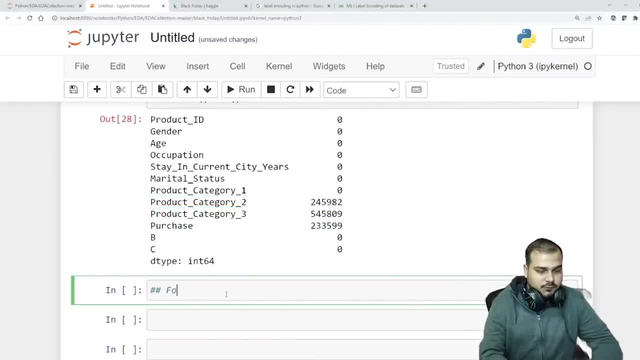 So what I'm actually going to do, we'll focus on focus on replacing missing values. Focus on replacing missing values. Now, when I focus on replacing the missing values, what I'm going to do, I'm going to basically replace the missing values for this two features. 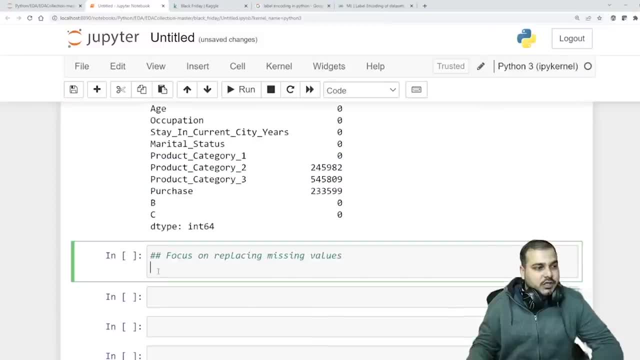 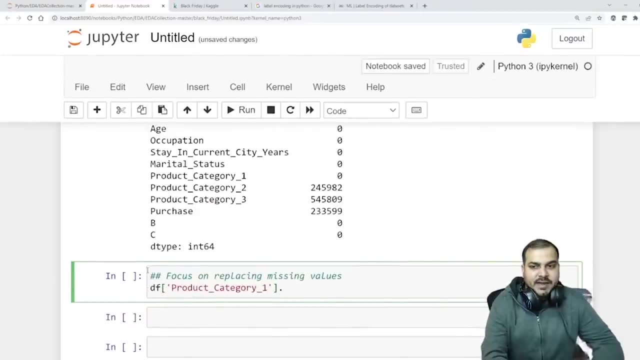 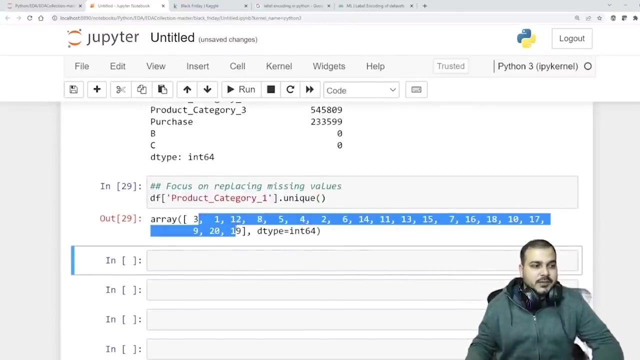 So we have to do some kind of data exploration for these two features. So what I'm actually going to do, I'm going to basically write dfproductcategory. Now tell me, guys, if I write unique, tell me what kind of feature this becomes. 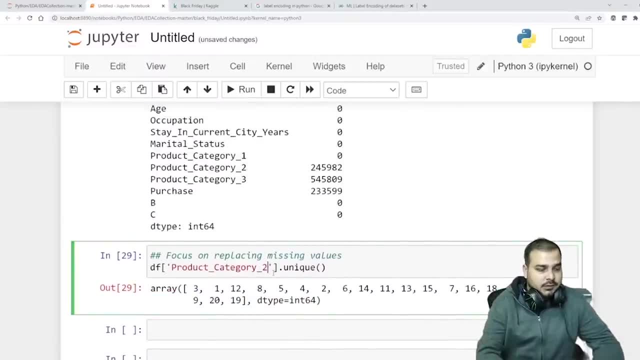 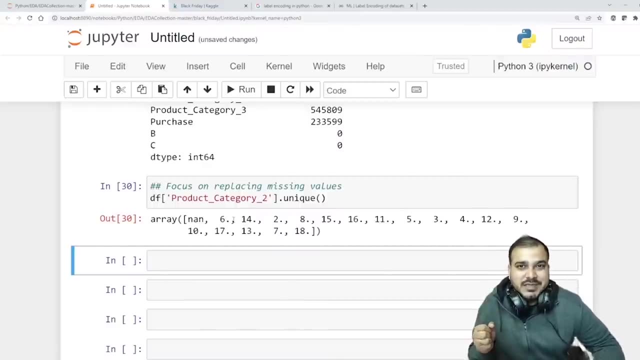 What kind of features, Or, if I write unique, what kind of features this will become. Will this become a discrete feature, Discrete, categorical, discrete, continuous feature, Or whether this will become a continuous feature. This will become a discrete feature, guys. 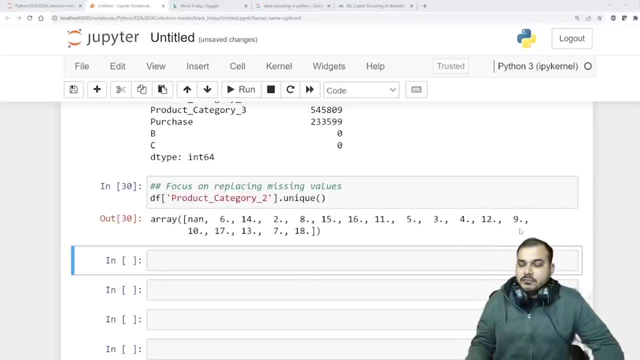 See, discrete, because this is only getting repeated. This will only get repeated. So, for the people who have attended my stat session will definitely know this right. So they will be definitely focusing on and they'll be knowing this. They'll be knowing this entire thing, okay. 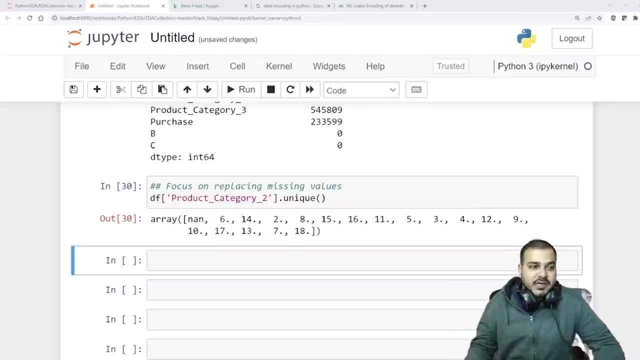 So over here you can specifically see that this will be a discrete feature. okay, This will entirely be a discrete feature. Now, in a discrete feature, if I have a NAND value, what is the best way to replace the missing values? 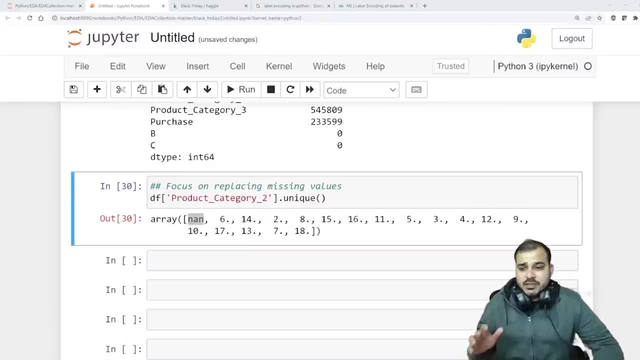 Tell me Quickly Now- this should be a lot of discussions that needs to be done on this, So tell me what should be a better way to replace the missing values. What I will also do is that I'll make your work a little bit easy. 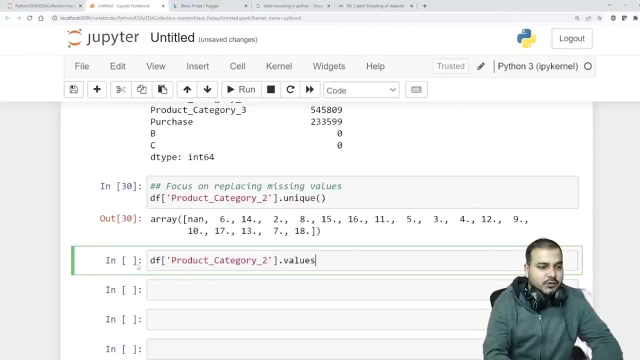 I will also. I will also write product category 2 and I will say: value counts. Value counts basically will give me all the values that are present with respect to this. okay, Value underscore counts. So here you can see, 8 is basically having this many values. 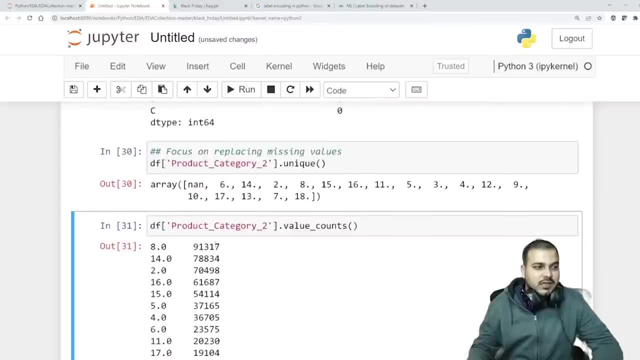 4 is basically having this many records. 6 is having this many records. What do you think? If I want to replace the NAND values, what is the best way to replace in this feature? So here what we'll do with respect to any categorical features. 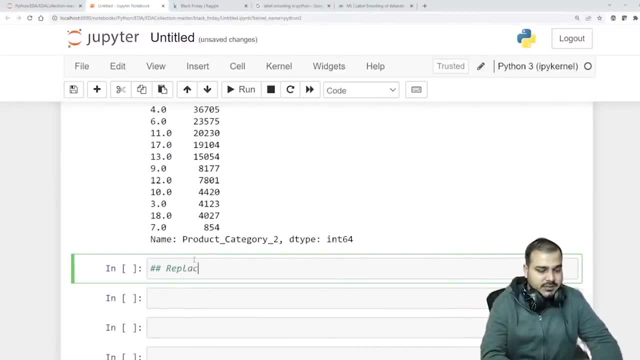 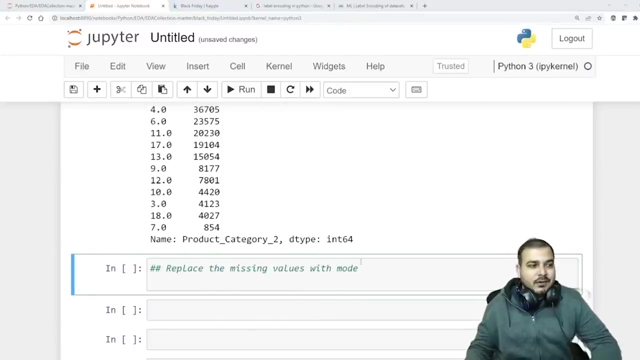 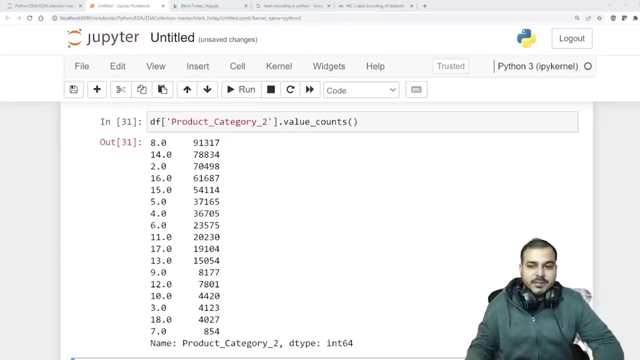 or discrete feature, the best way is to replace the missing value with mode. So, in order to replace the missing value with mode- okay, Mean, don't use mean guys, Because mean will create a new category altogether. So, in order to replace the mode, that is very much simple. 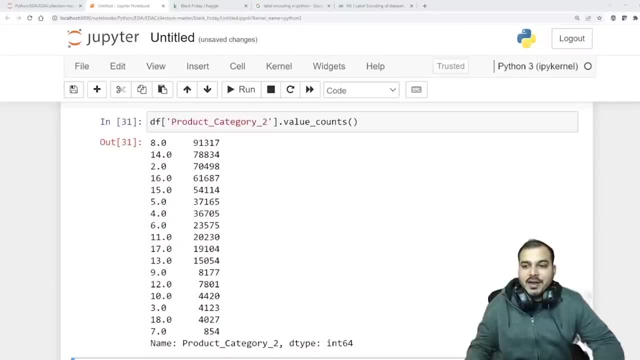 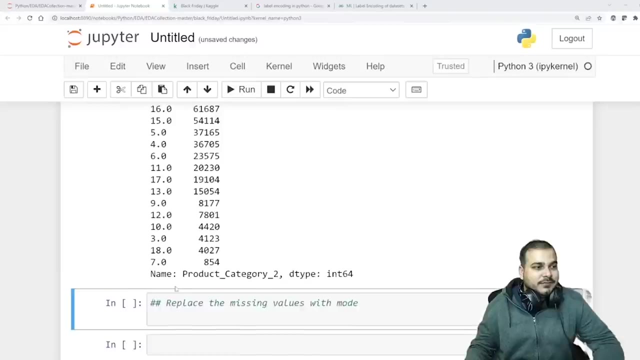 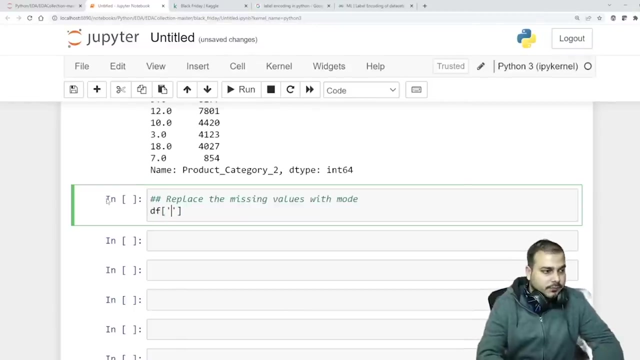 And how do you do it? Just let me know. How do you replace that With mode? Tell me guys. So first of all, I'll write a simple code for you. I will say: DF of product, product, product category 2, okay. 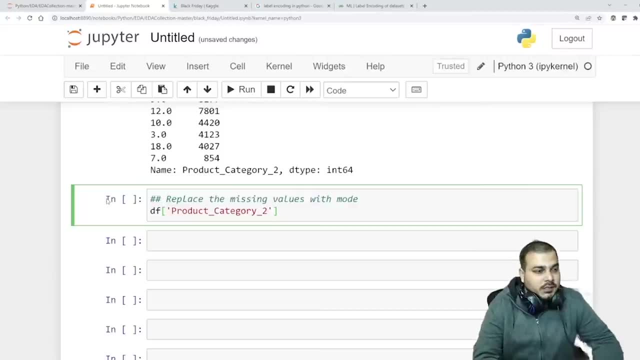 Please think over it. Try to write the code, guys, okay, Okay. So here I will definitely use something called as fillna. Fillna function is already there, which I have also mentioned or explained in my lot of lectures, So I'll say: dot fillna. 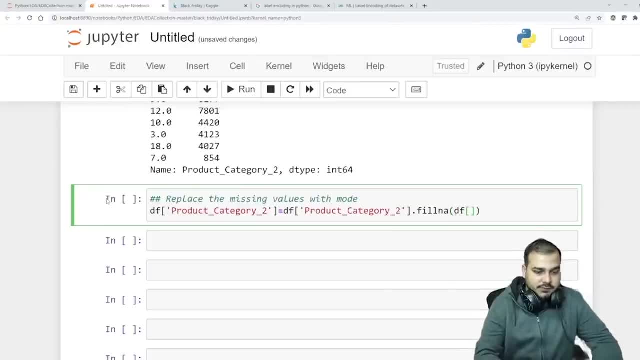 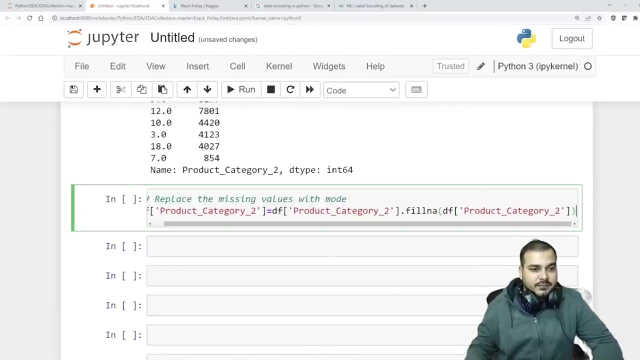 And here I'm basically going to say: DF of product category 2- dot mode- right. See, if I basically just copy this entire thing, okay, And if I write DF of product category- dot mode- right, What will be the output that I will get? 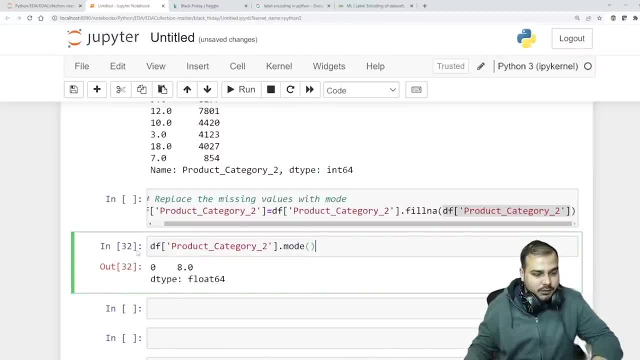 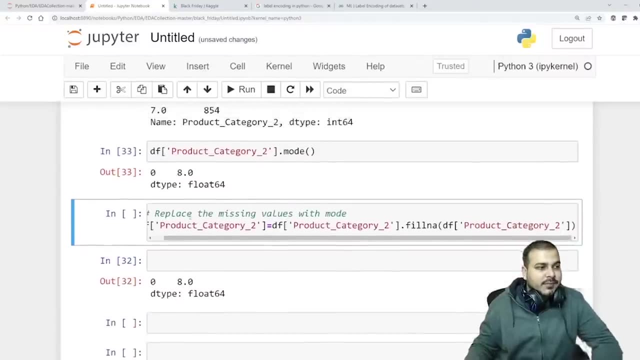 I will get this two output: 8.0.. So if I want to find out the mode, what I have to do, I have to basically write something like this For this: right Now: here I'm getting two values. 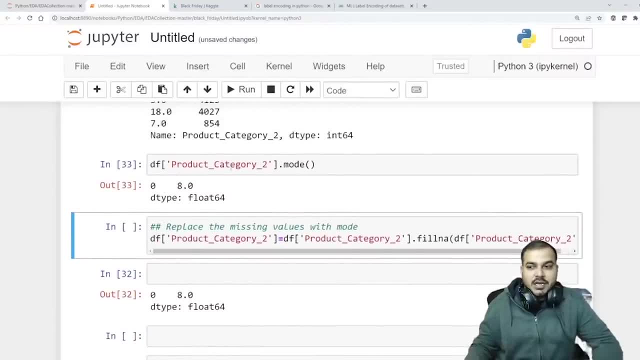 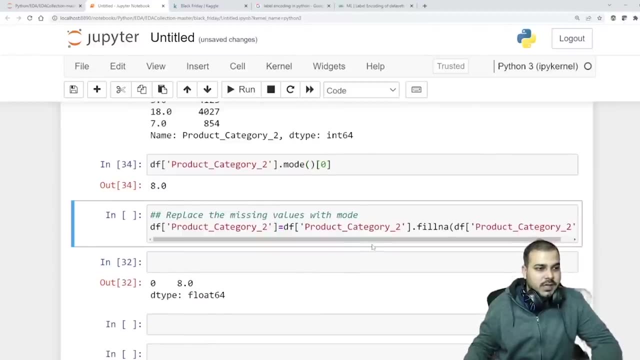 One is 0 and one is 8.0.. So this becomes a series. Now, in order to pick up this value, I can basically use indexing. So if I use this, then I'll be getting 8.0, okay. 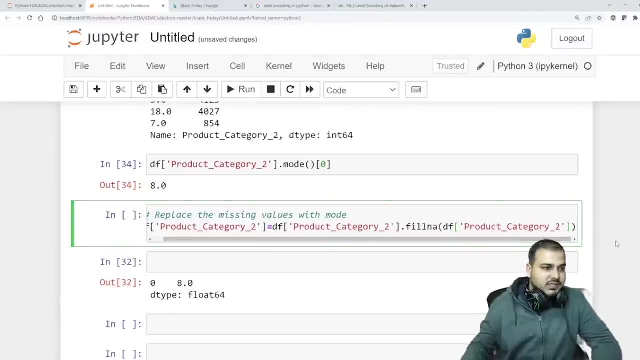 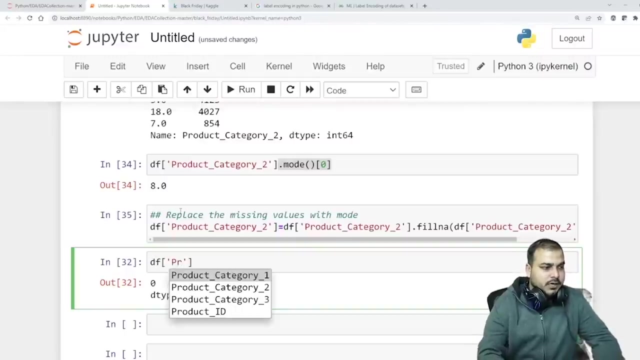 So here what I'm going to do after this. I'm going to basically just copy this entire thing Over here: dot mode. So once I do this, this will get reflected over here. And now, if I probably write DF of product category 2, dot is null, dot sum. 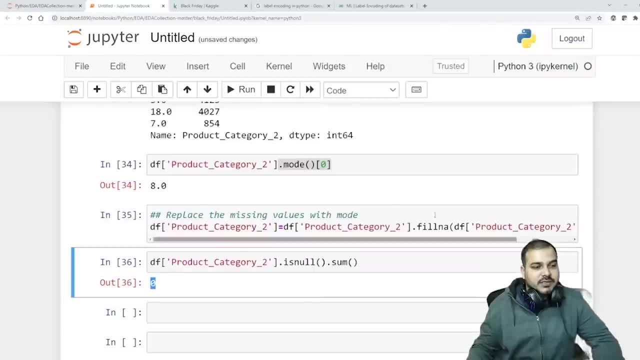 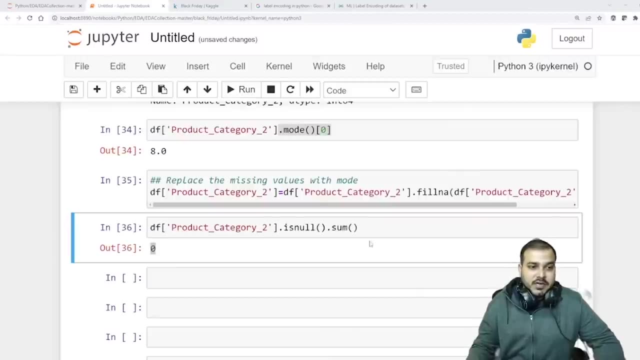 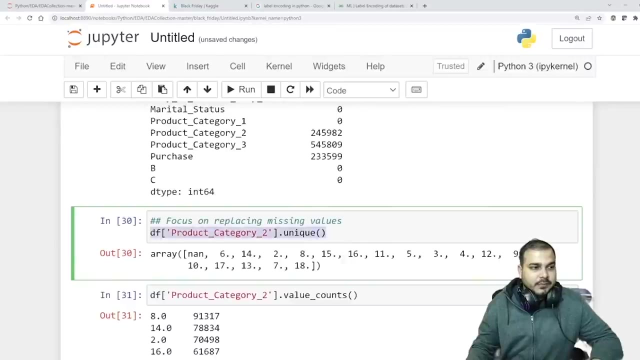 So here you can see that now my values are 0.. That basically means the replacement has happened. Clear, Yeah, Interesting. The data set is also quite huge. Now, similarly what I'll do for product category 3, because there are 54,000. 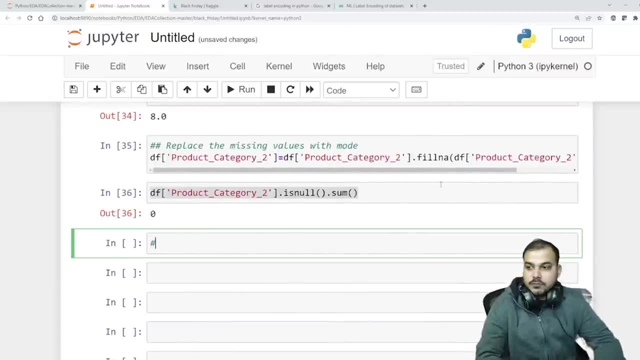 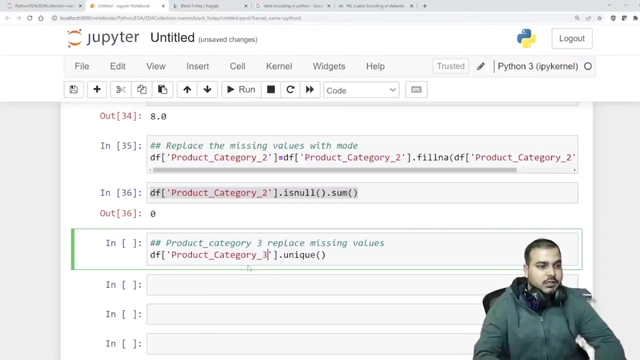 Okay, So we will also do it for product category 3.. Okay, Product product category 3.. Category 3, replace missing values. Again, I'm going to paste it over here. I'm just going to write dot 3, underscore 3: dot unique. 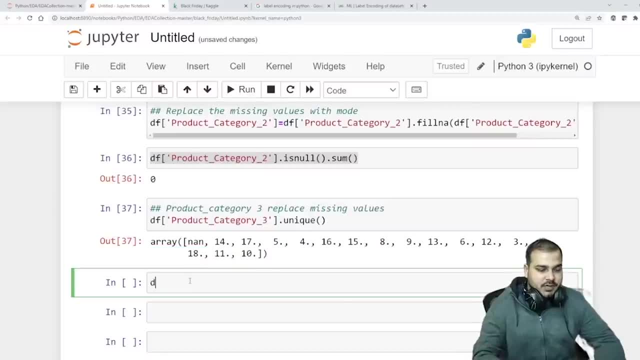 So here also I see 14,, 17,, this, this, this is there. If I want to also want to see what is the value counts, I can basically write: dot value counts, Dot value counts. So here it is all my values with respect to this particular value counts. 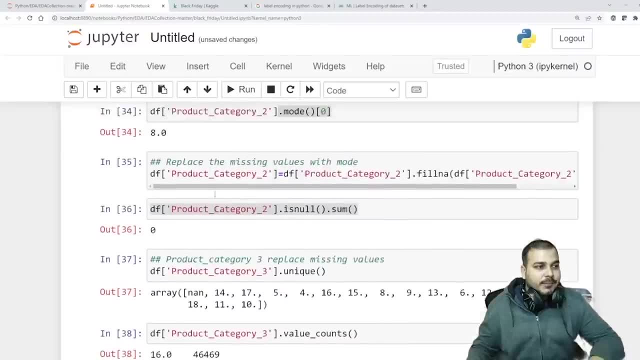 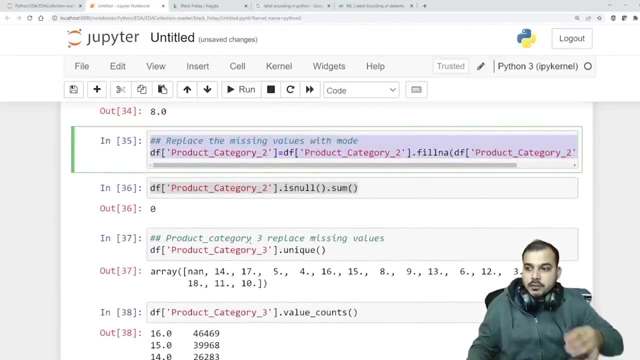 Okay, So let's go ahead and replace this. Okay, So, let's go ahead and replace this. Okay, So, let's go ahead and replace it. replace with missing values, with modes. I'm to again, I'm going to going to copy: please bring the missing value. 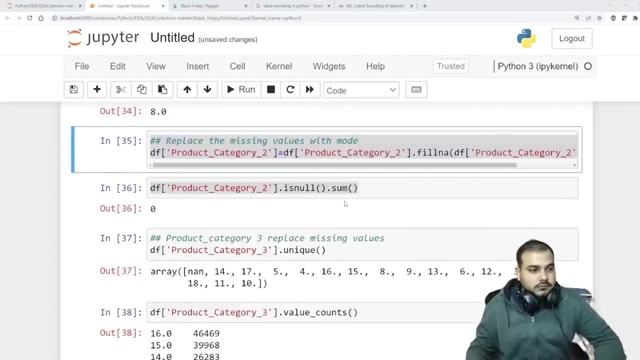 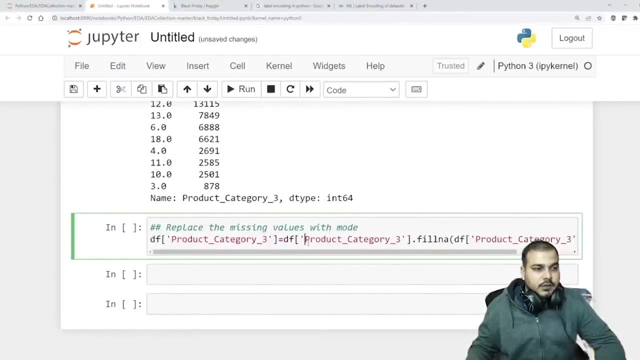 So here it is. Okay, I'm going to just use it with product category 3.. So now, if I execute it, now if I go and probably see my df dot head, Okay, So here it is everything. 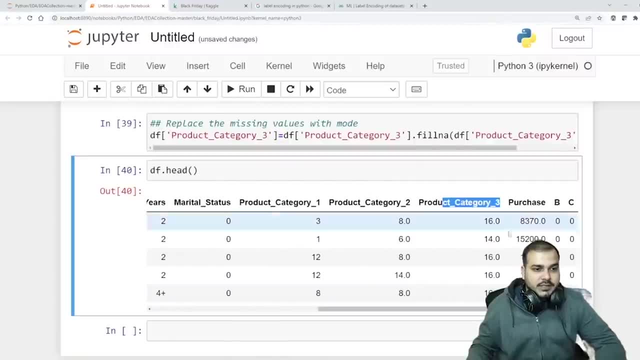 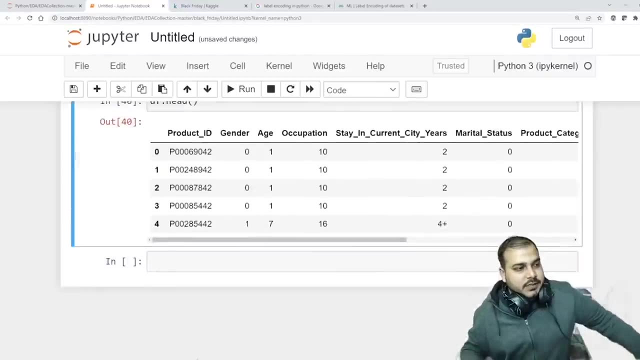 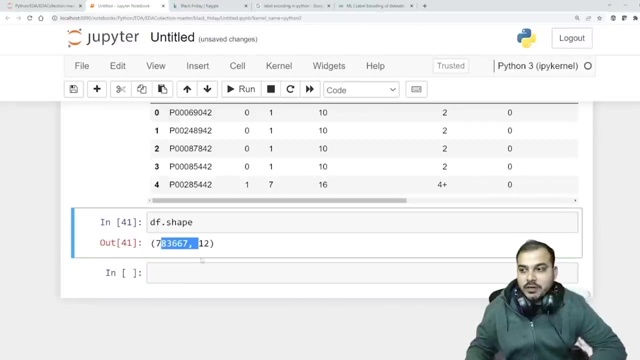 So product categories 3, this, this, this is fixed. Why shouldn't we just remove product categories? The reason is that because if I go and see df dot shape here, you have around 7,83,000 records and around 5,00,000 records are basically missing. 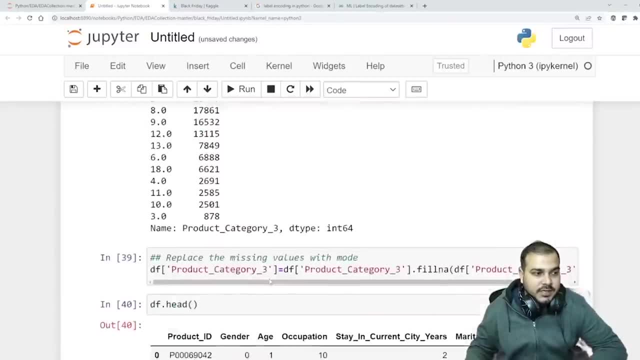 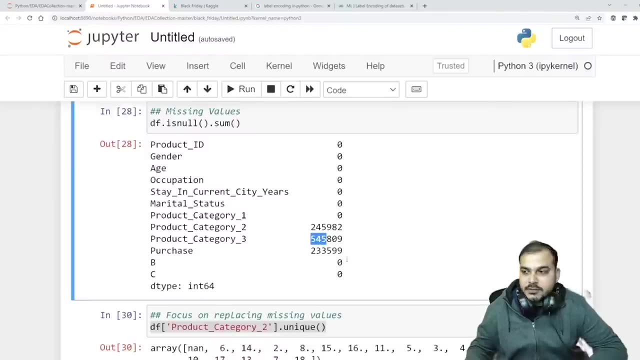 If you see over here, 5,00,000 records are missing. So why shouldn't we remove product categories? Okay, So here it is everything. Okay, 5 lakhs. 2 lakhs are there. you cannot just drop it. okay, probably that may be an important information. 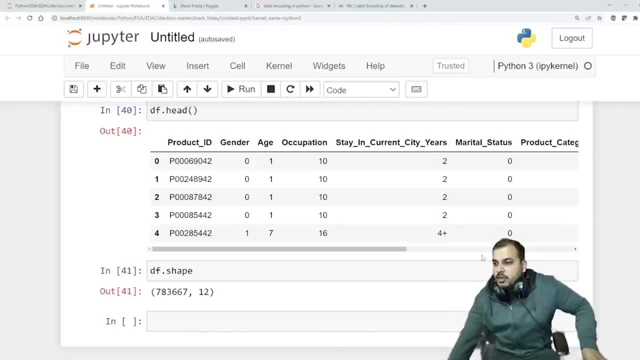 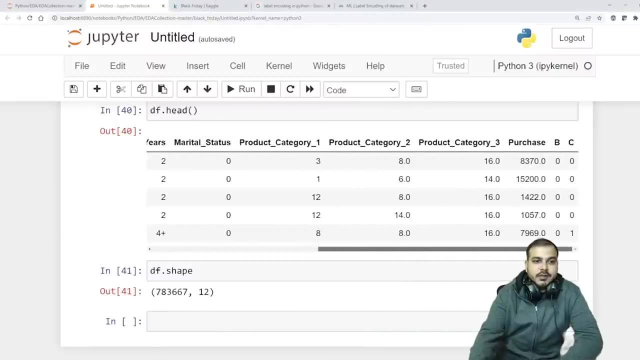 sir, you said for purchase column, then missing values are fine because it is for test data, but train test split is random. no, tritraj, we don't just do random, we do cross validation. let's go to the next step. anything that is left, one more category, is this one right? stay in current. 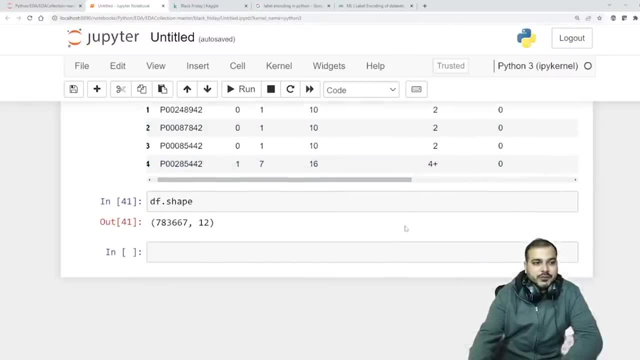 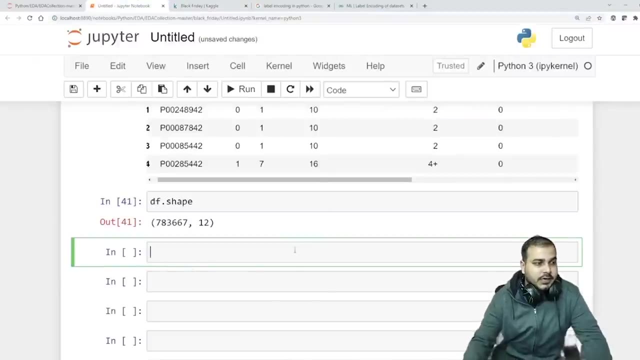 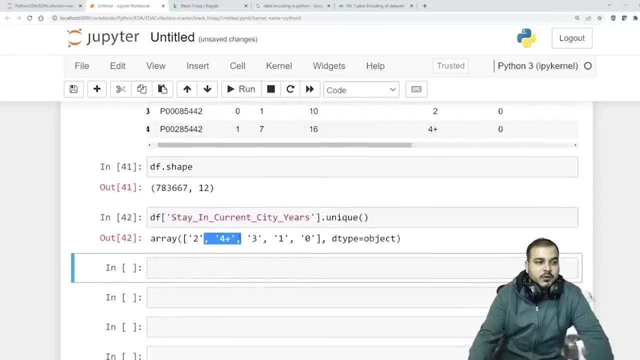 years. so what do you think we should do for this? so here, if i say hashtag stay for current years, right, stay in current city years. so if i write df of state- current city years- and if i write dot unique, so here i am having 2, 4 plus 3, 1, 0. okay, so what we can actually do. 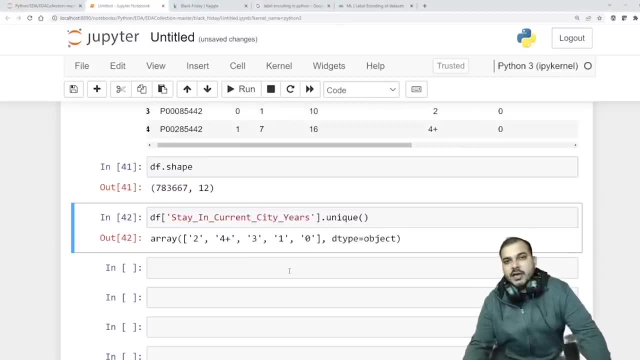 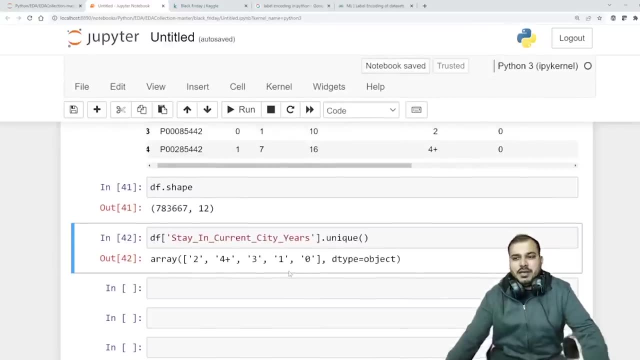 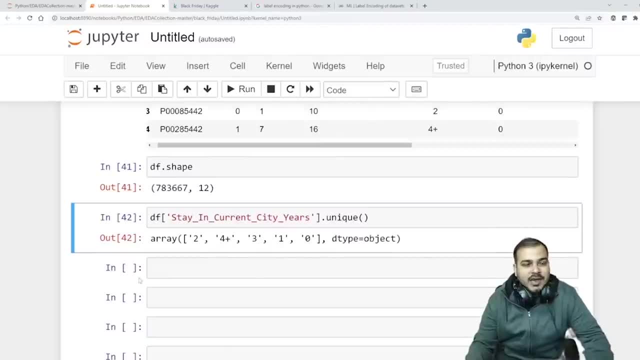 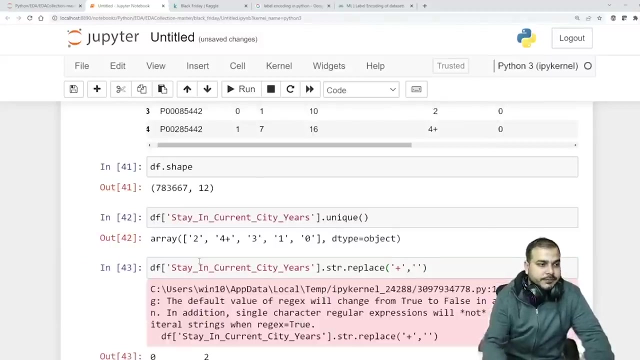 is that we can replace this 4 plus with 4. now tell me how to do it. so i will write tf of stay in current years, dot, str, dot, replace, and then i'm actually going to replace plus with with blank right. so if i do this i will probably be able to find out all these things right. so this, entirely, i can. 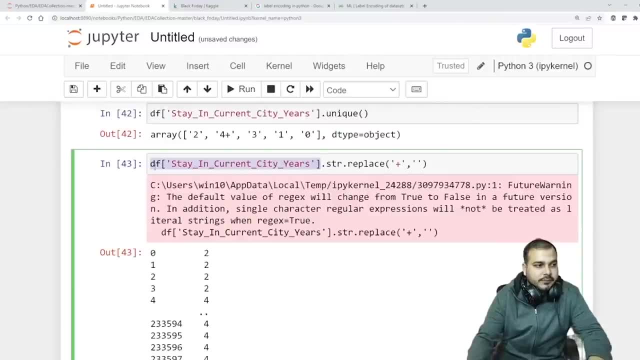 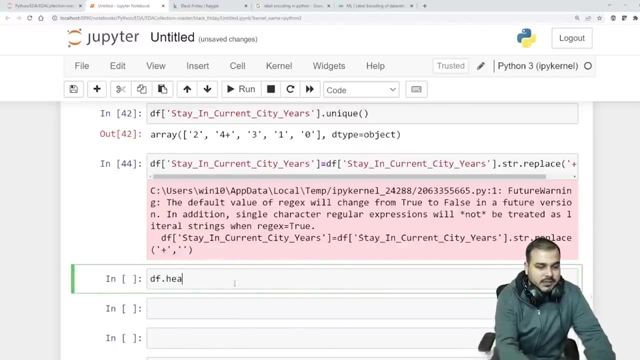 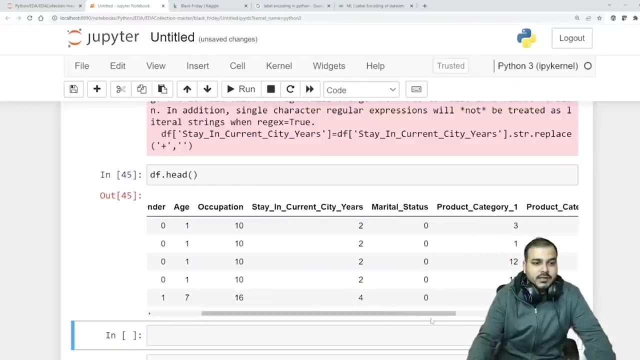 save it inside my df dot, stay in current. so if i execute over here, done some warning is there, but it's okay. so here you can see this now. i don't know how to do it, so i'm going to do this. i don't have 4 plus. i have fixed it. another category. any more categories today, we are just 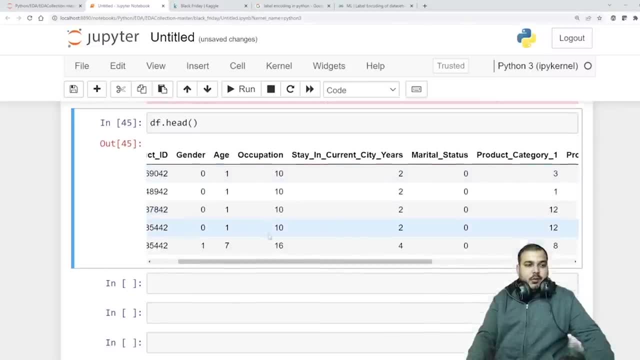 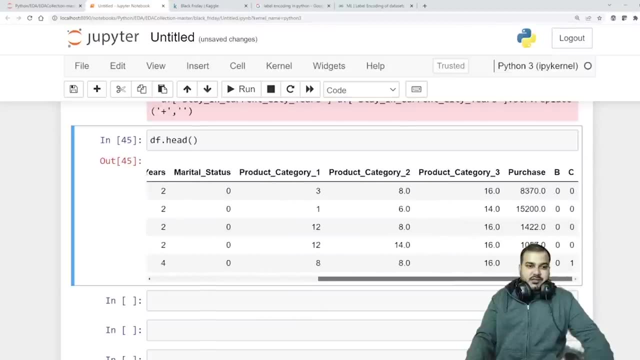 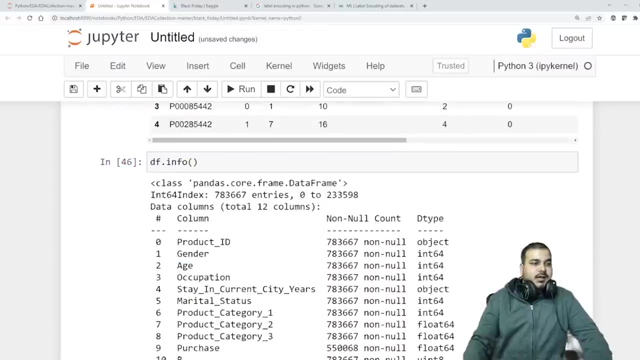 focusing on solving categories. now let's do one thing. okay. now, even though we are basically checking categories, we are we are basically checking other other things over here. right, if i probably just go and write df dot info. so here we are seeing that product id is an object, that 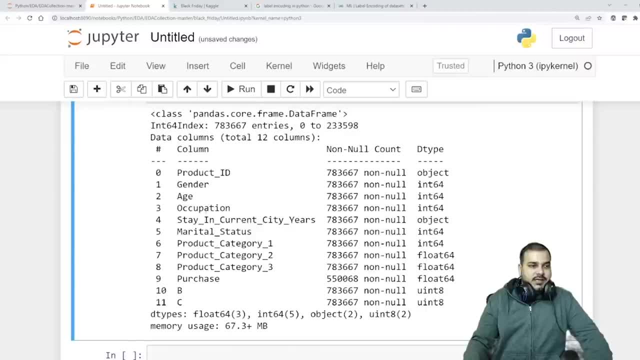 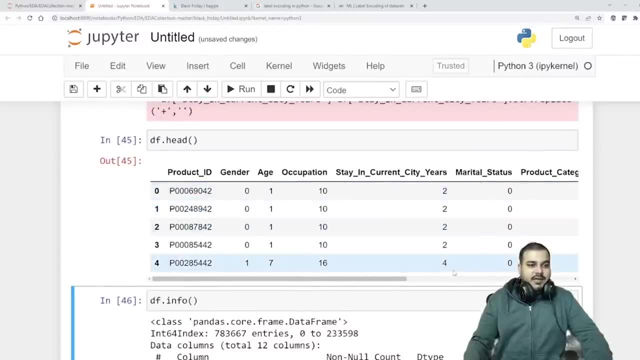 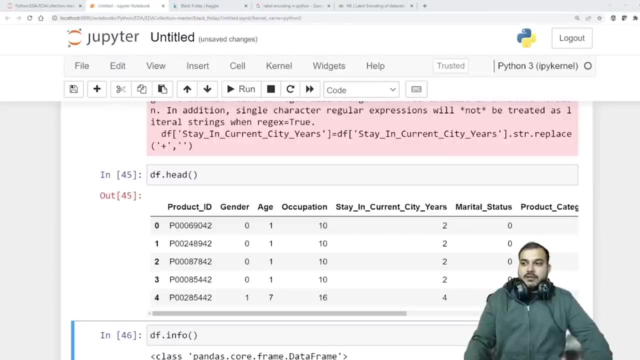 is fine. gender. it has an integer. that is fine. age is an integer, occupation is an integer. stay in current city years is also an object. but here you can see that i'm having values like two, two, four, four, four. so we need to convert this object into integers. that is a major step that we have to actually do. so what we are. 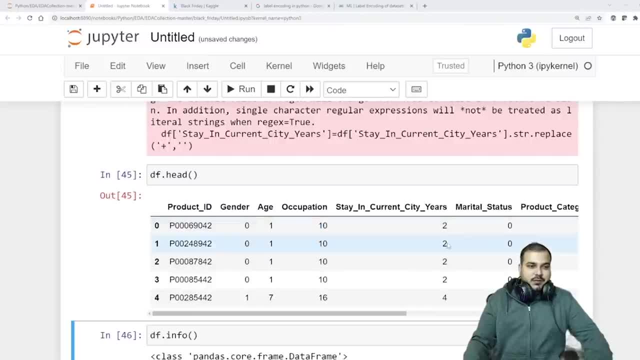 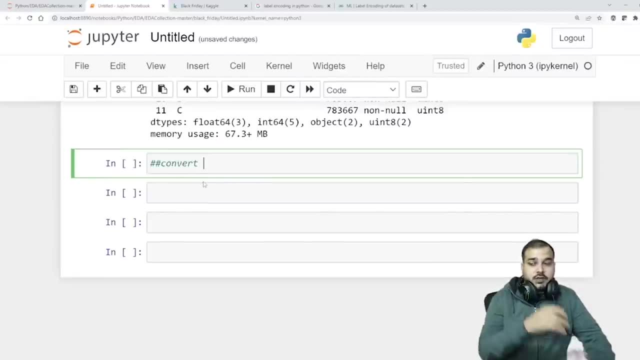 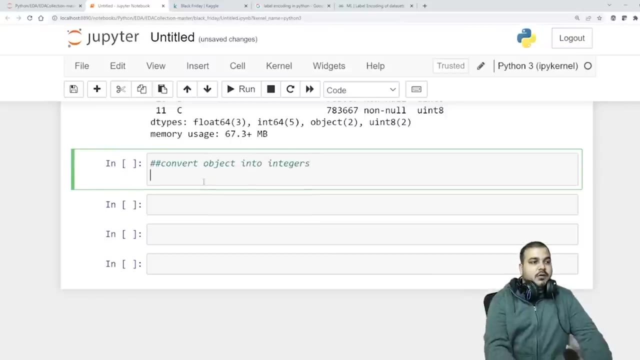 actually going to do over here is that we have to convert this, which is an object, into integers. so how to do that? so convert, because this kind of task also you may be getting- convert object into integers. can anybody tell me how to do it? very simple here. i'm just going to 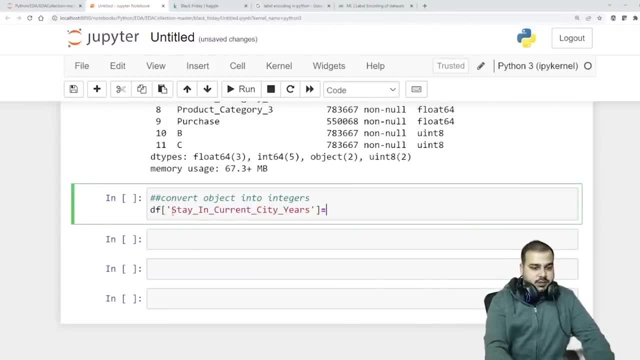 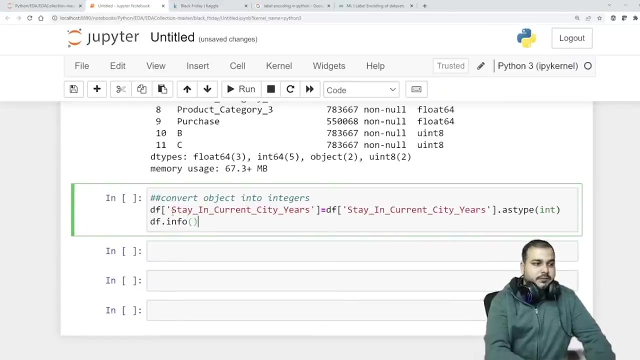 write df of stay in current city years is equal to df of stay in current city years. dot as type, as type integer. if i do this, done so now, if i write df, dot head or dfinfo, you will be able to see this. so here you can see, stain current is basically: 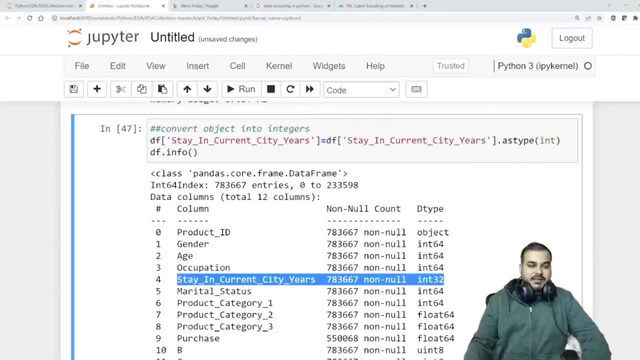 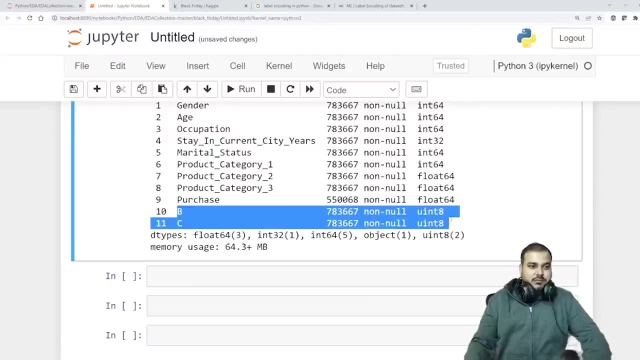 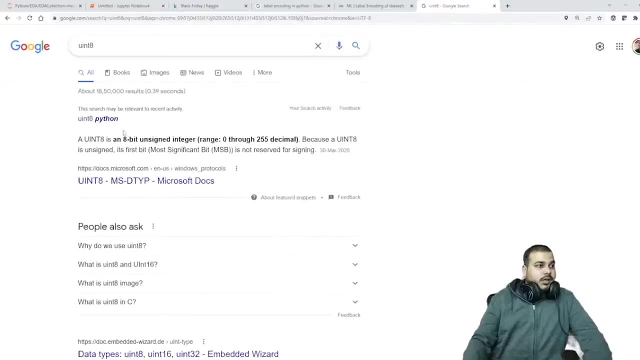 assigned a int32. you can also assign int64 by providing int64 directly over here. ok, there are two more columns: which has b and c as uint8, uint8. what is uint8 uint8? it is an 8 assigned integer ranging between 0 to 255 decimals. it's ok, you can also convert that. 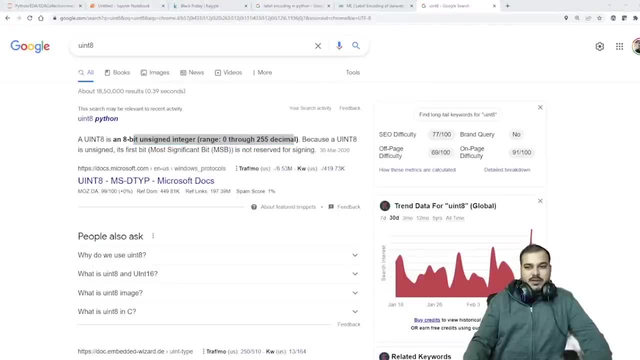 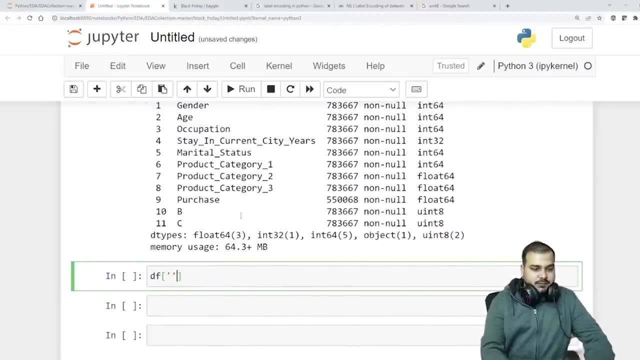 into int type. so if you want to convert that into int type, i will just use this: two codes. so what i will do here. i will say b and c, right, so df of b is equal to df of b, dot as type int. and same thing i can copy and paste here. 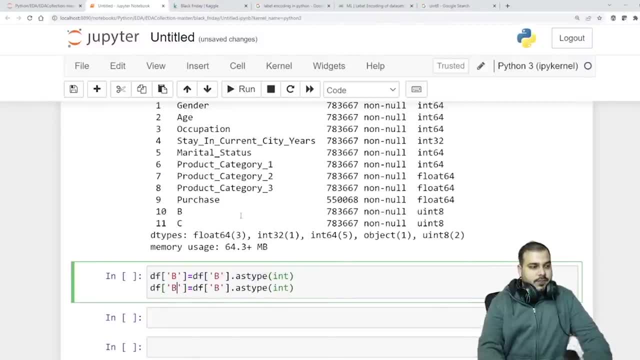 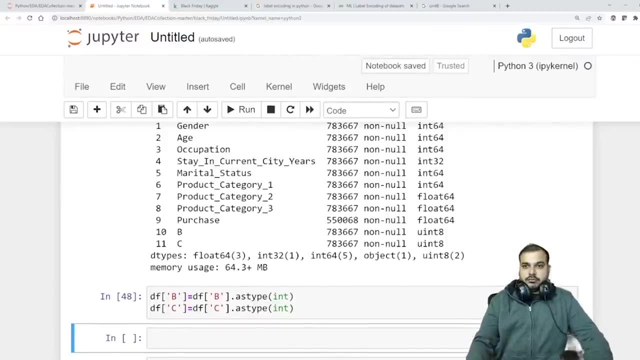 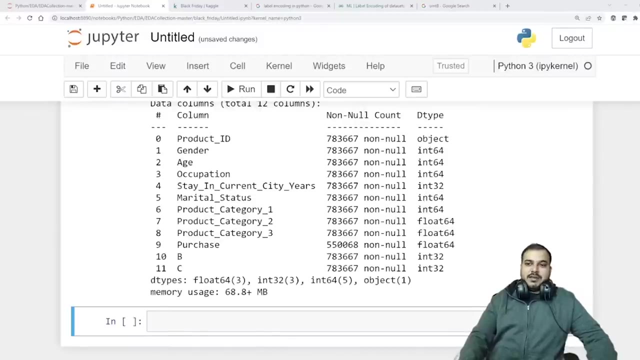 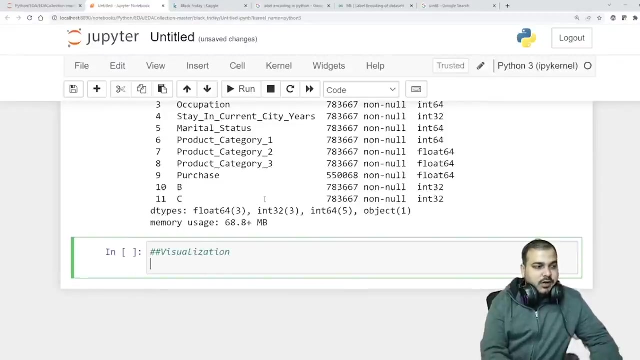 paste it for df of c. hello, execute it now. if i go and probably see my dfinfo, you will be able to see this now. once we have done this, the best visualization, what i feel visualization is present in cbot, which is called as dfinfo. 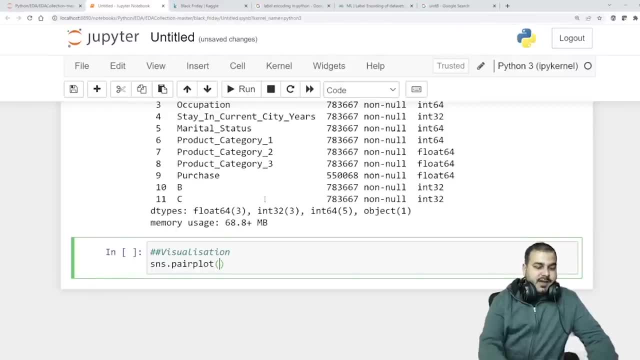 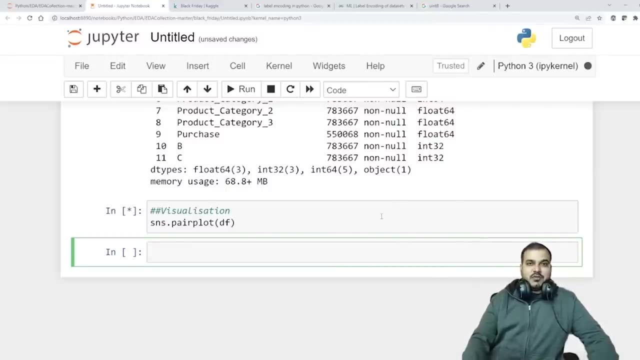 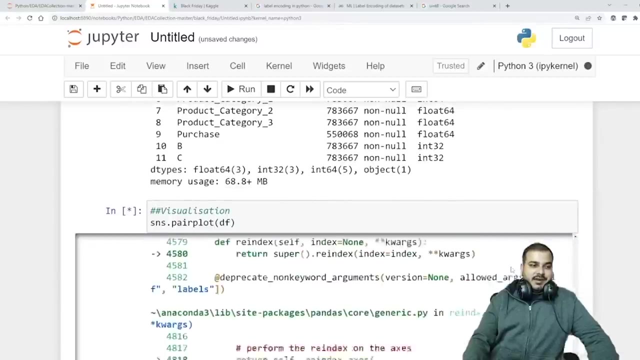 snspairplot. if i give pairplot and just give df, see what is the amazing diagram. but it will take lot of time because there are so many data points along with that, so many data sets. ok, it is giving me an error. let's say what is the error. cannot reindex from. 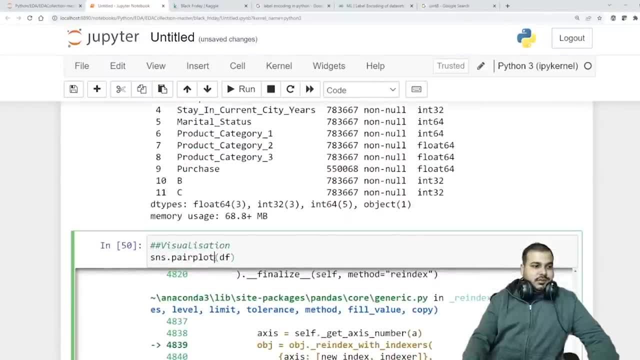 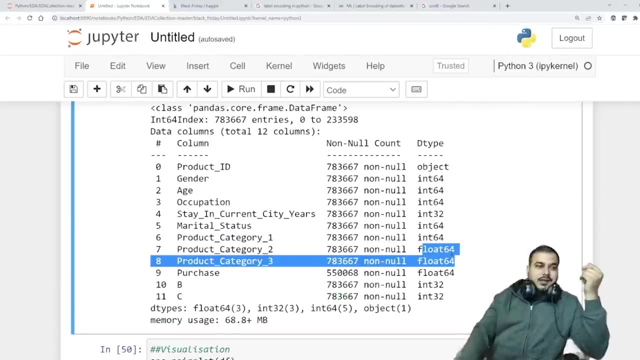 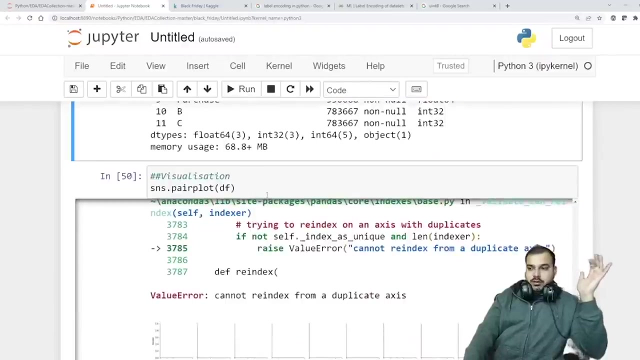 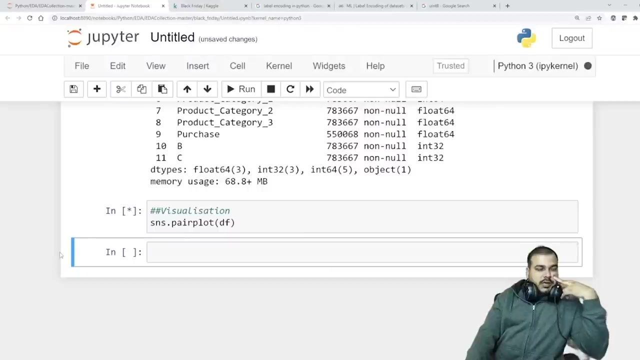 a duplicate access, duplicate points, why this error has come. it's ok, see, if there is something like a product type, right, that will actually get removed in the pairplot. that is the reason why do we use this. it will give an error. i will have a look on to this. ok, don't worry till then. 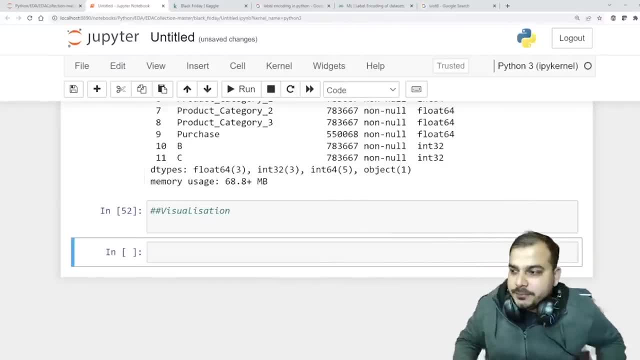 let's see some other visualizations. ok, till then, let's see other visualization diagrams. so i will just have a look why that probably is not coming, but i can definitely use another plot like barplot. let's say that i am using barplot and i want to basically compare age with respect to purchase. so this: 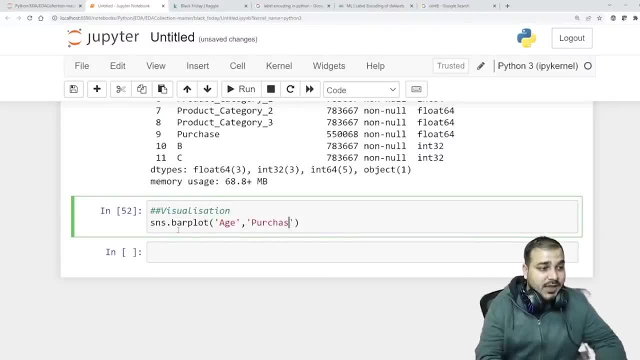 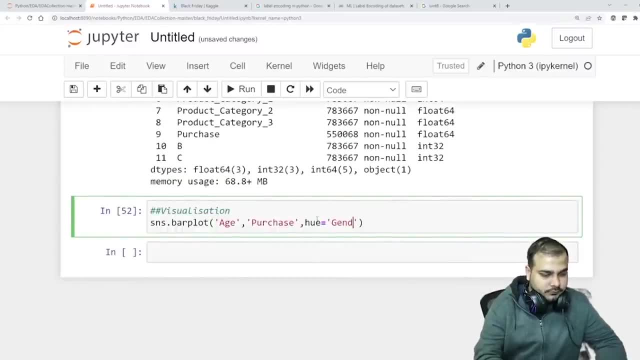 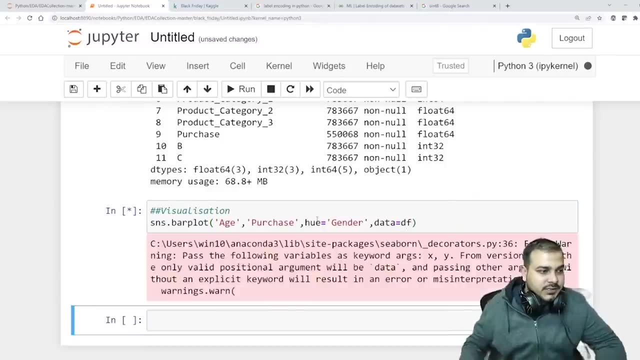 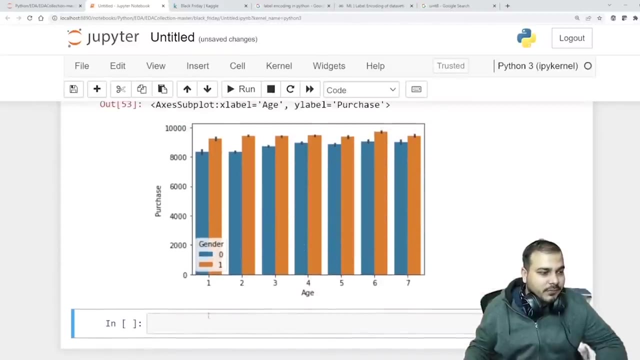 going to use that we as gender. ok, i have done some observation over here and data is equal to DF. ok, so let's execute this. so this is the diagram that you're getting, so date: 1, 2, 3, 4, 5, so which you can basically map with it, but definitely you can see that even. 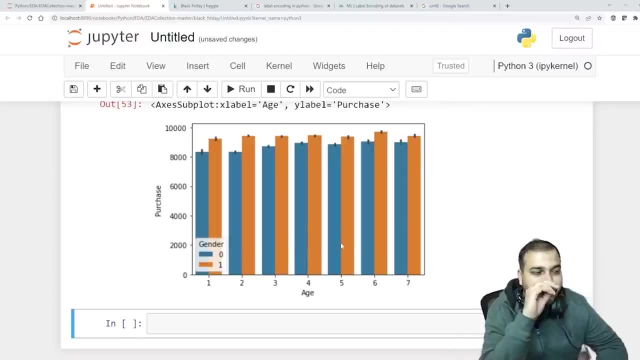 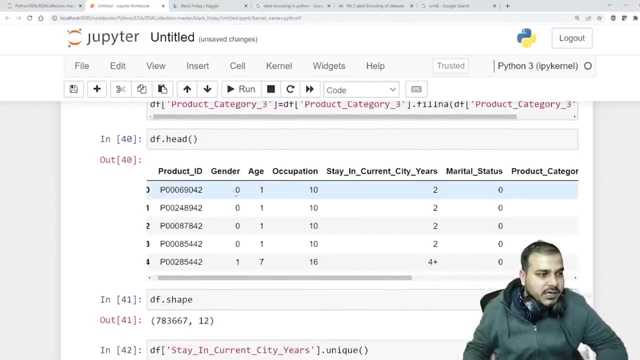 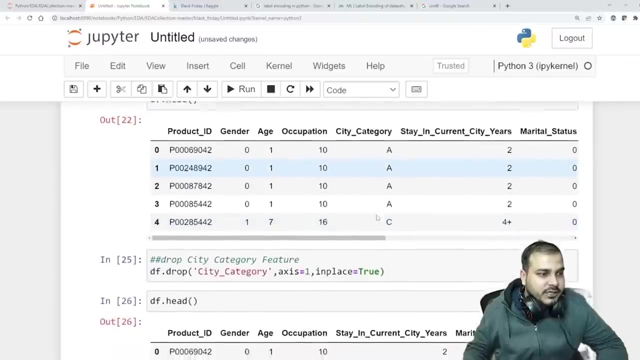 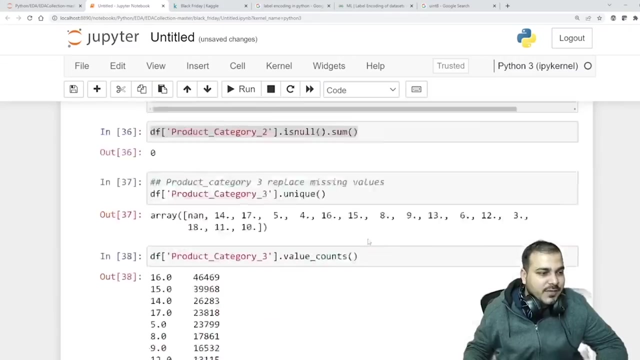 55 plus. Yes, Which observation. if gender 0: 0, what we have replaced with male right gender, uh, 0, we had replaced with female or male, very gender, very gender, i think, for male, for female, we had made it is 0, yeah, so from this definitely you can come up with some conclusion. 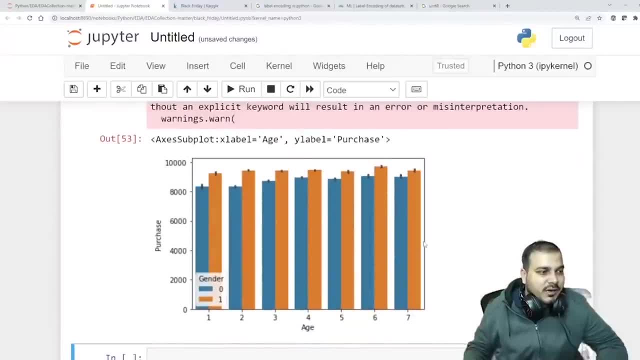 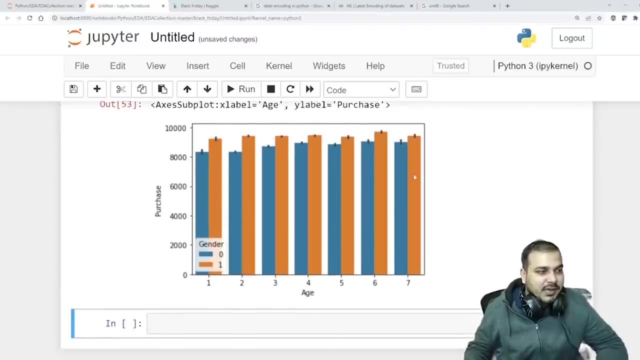 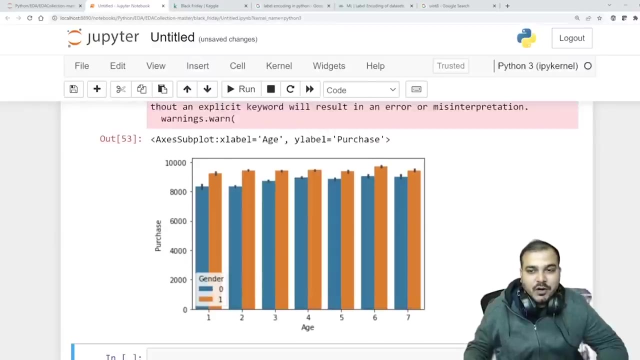 that, whether female has bought more or male has bought more, but over here, with respect to the purchases- maximum amount of purchases- you can see that uh, male has a huge purchase. uh, with respect to the orders: also, we'll try to see with respect to different different orders. 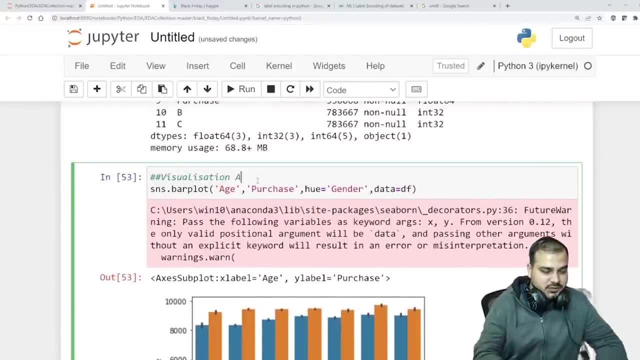 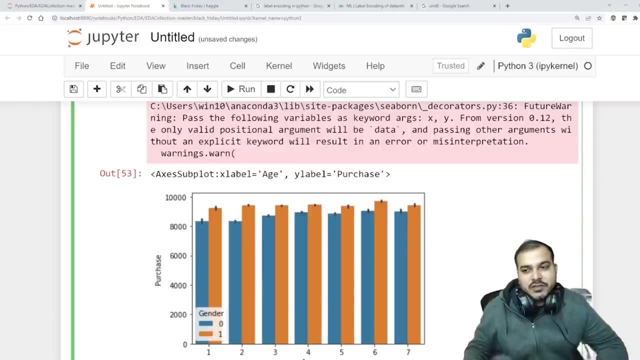 this is nothing but visualization of age versus purchase, so please write down your observations. what do you feel with respect to this kind of things? purchasing of goods of each range of age are almost equal, but we can conclude definitely that the purchasing percentage of purchasing services is very high. so we can conclude that the percentage of purchases is very high. 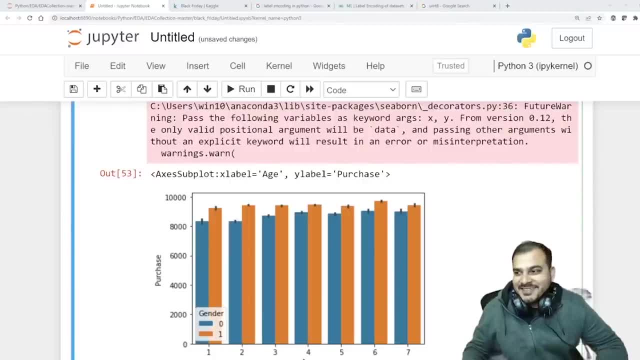 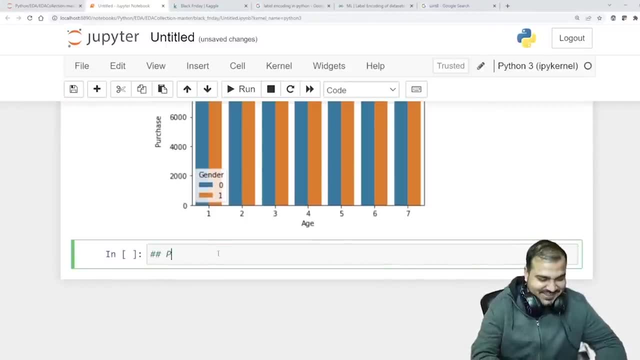 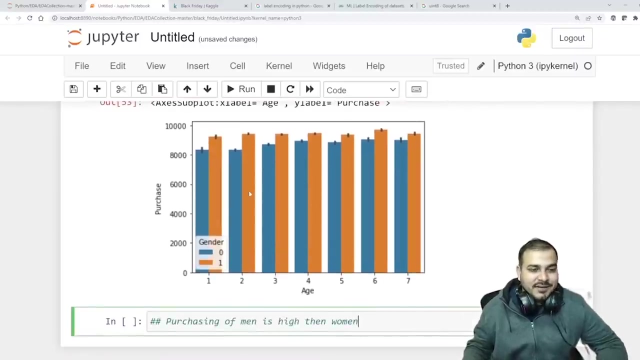 goods of men over women is high, right, is this possible? no, purchasing of men over men is high, then women. so this is the observation that i have done, which is not at all possible. right, but data does not lie right. right, so definitely, all the other purchases with respect to the ages are uniform. but 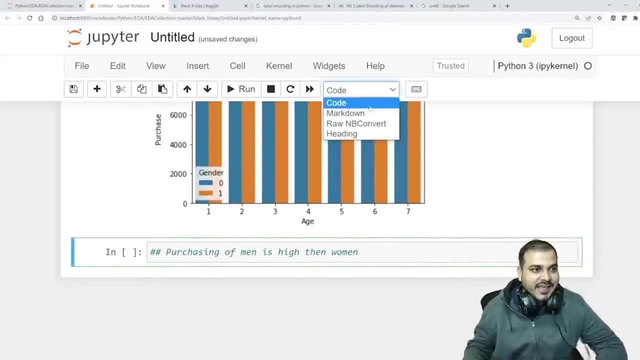 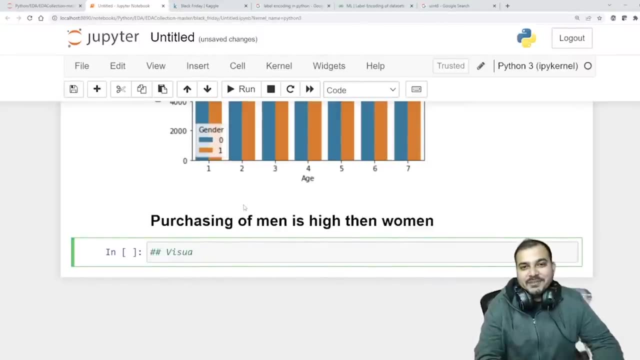 purchasing of men is higher than women. yeah, nice, i like it. so this is my first observation, let's say, with respect to purchase. we'll try to visualize the occupation, okay, so visualization of purchase with occupation. so i'm just going to copy this same thing. so, i'm just going to copy this same thing. 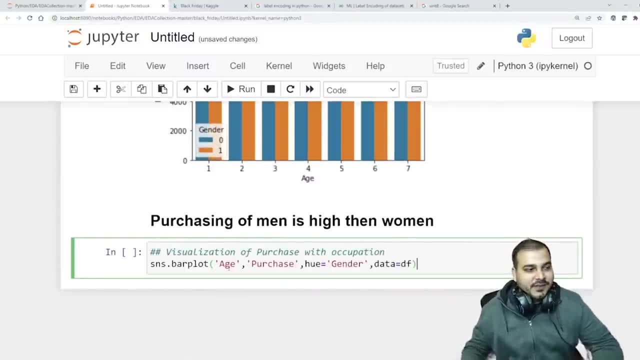 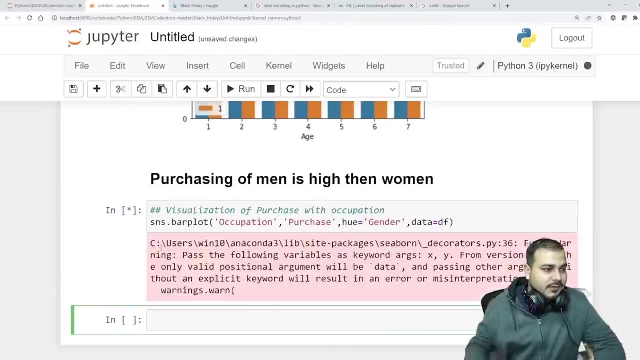 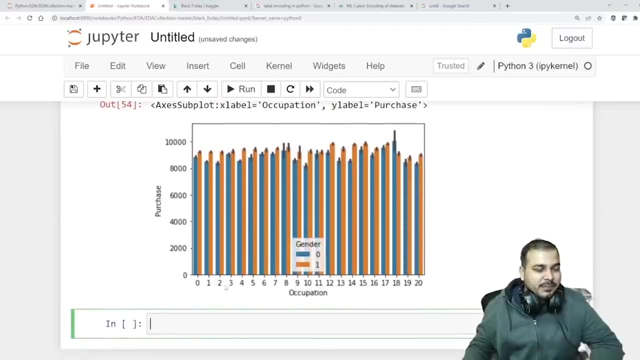 and i'm going to paste it over here. so here i'm just going to say it as occupation. uh, let's see the diagram. this will be quite huge because it will be stuffed. right occupations are many. right occupations are many. so you can just go and check out which all occupations are there. 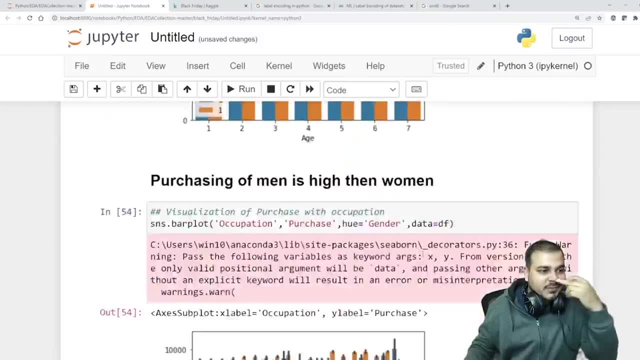 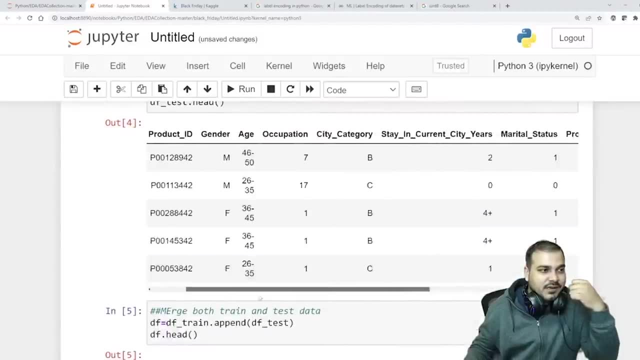 are 20 different occupations. so from this data set you will be able to find it out, the initial data set, and you can see that the occupation is big and the occupations are many. so this will be quite huge. you can make some observations from this. let's see where is occupation occupation with this. 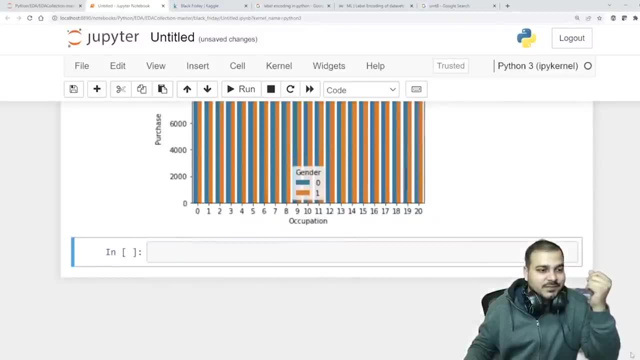 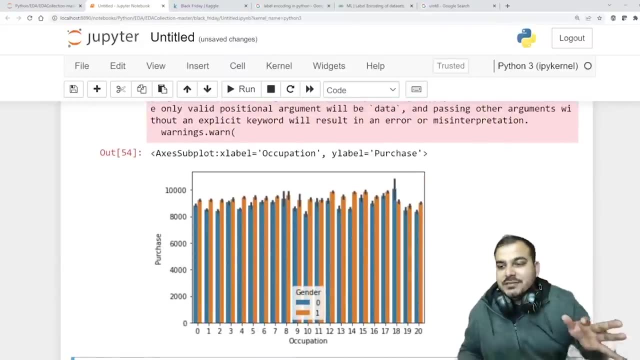 some categories are mapped okay. so with respect to this, i'll i'd suggest that this is also uniform. it won't affect a lot. let's compare, uh, whether product category one, product category one, versus purchase. like many people have bought product category one because if you go and see the data set then we'll be able to see it over there. 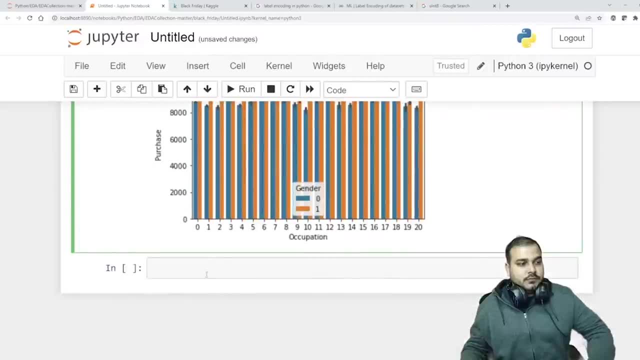 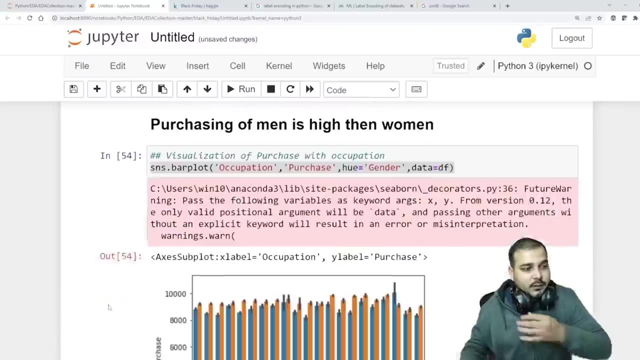 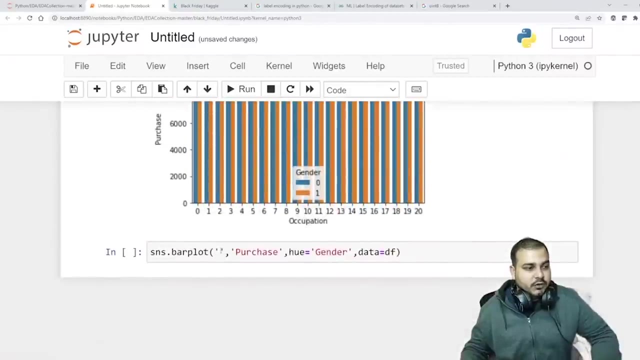 so i'm just going to copy this with the bar plot, i'm going to write it over here and i'm going to basically write product category one product. so let's see product category one: how many people have bought with respect to the purchases, so that amount will be shown. 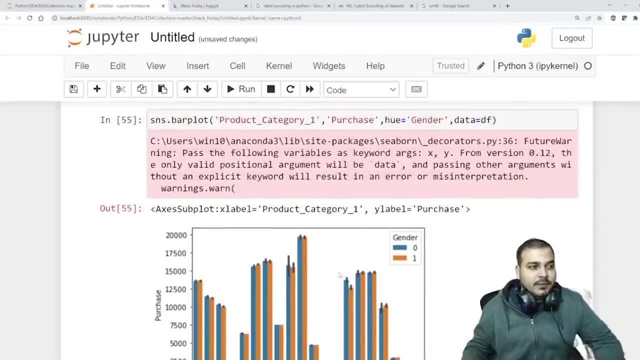 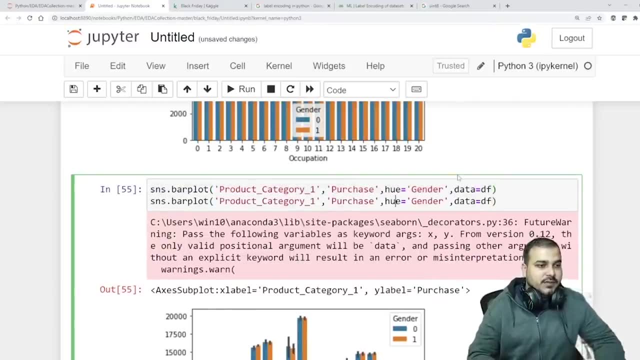 so here you can see. this is the graph with respect to product category one. similarly, let's see with respect to product category two. i don't know whether we'll be able to see it or not. in the same thing we can see two graphs. two graphs will not be able to see it. i. 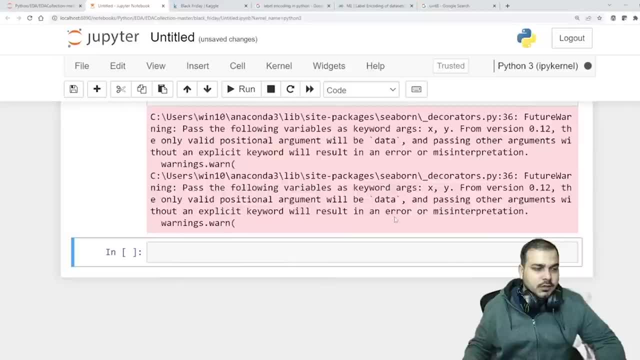 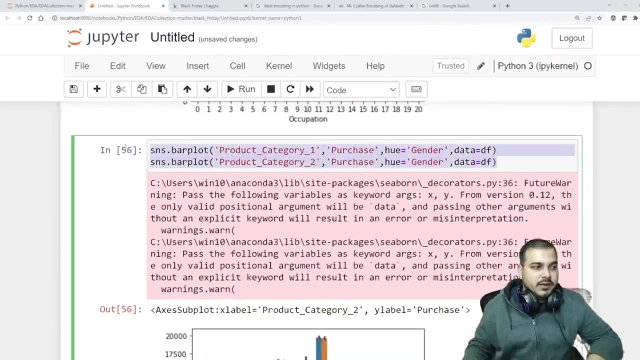 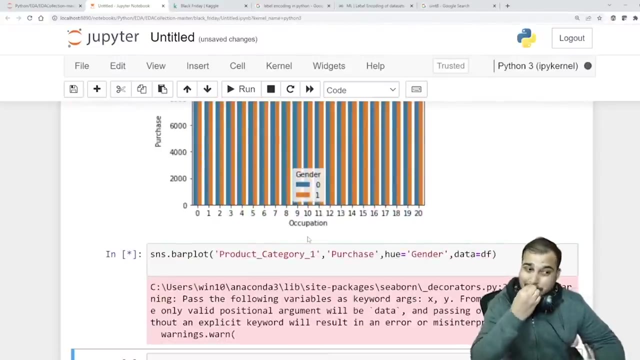 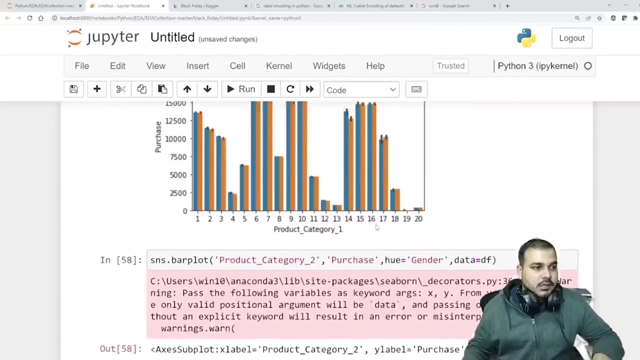 guess what is coming? no, only one is coming. okay, i will remove this. i think it will replace in that same order. okay, so i will just execute this product category one, and then this will be my product category two, and the next one is my product category three. 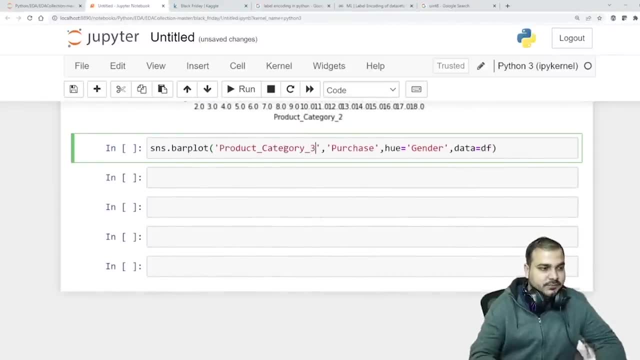 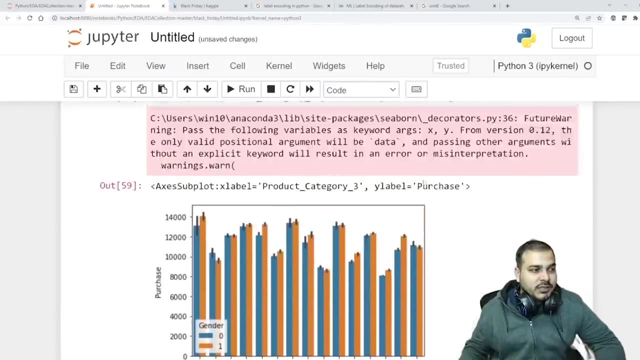 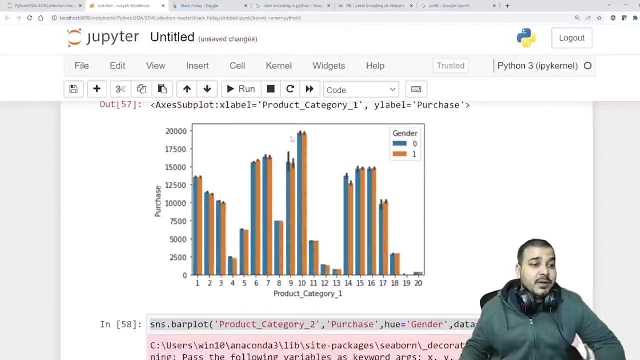 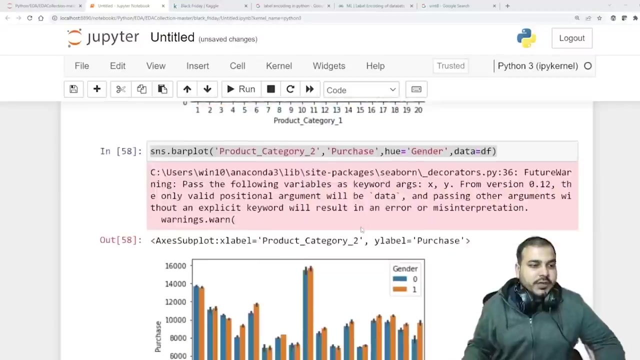 but observe this and come up with some conclusion. guys, here you can see, with respect to 12 000 is there here till 14 to 16 000, product category two is sold, bought more, whereas product category one is bought the most right. it is still 20 000 right. so definitely that information you can take it out from. 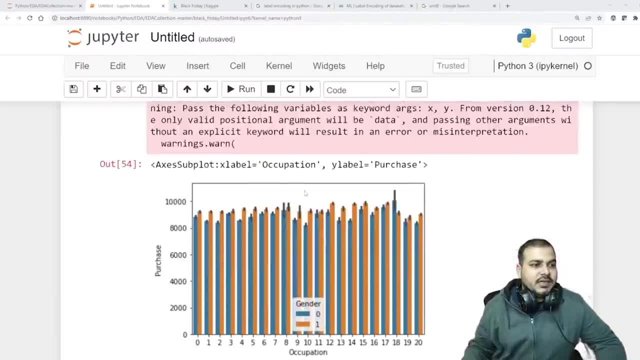 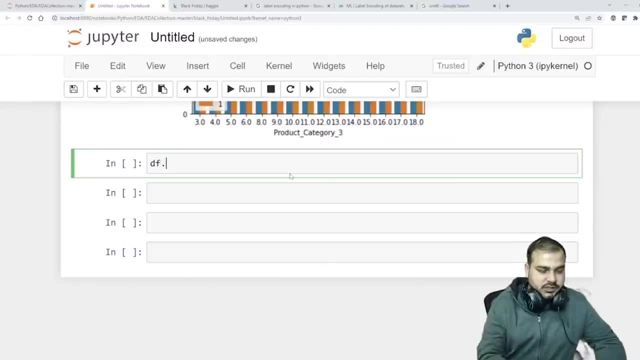 this particular graph, any other graphs that you want to propose, but you can definitely use this. tell me, guys, is this more? is this data set good for the model or not? now, because the type of data pre-processing we have done, i think we are good to do it right. 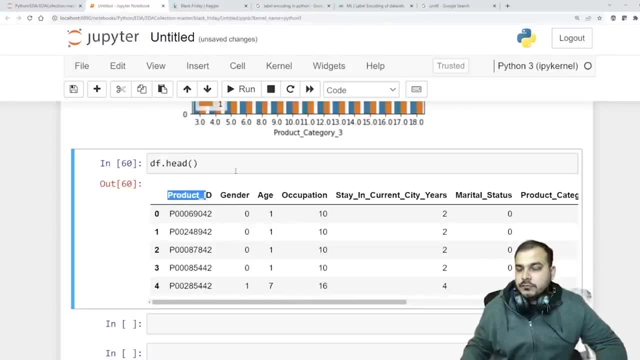 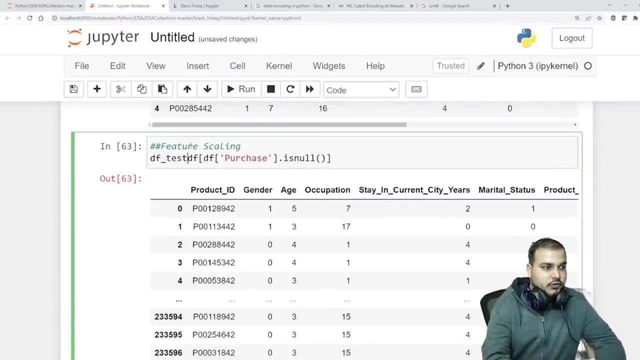 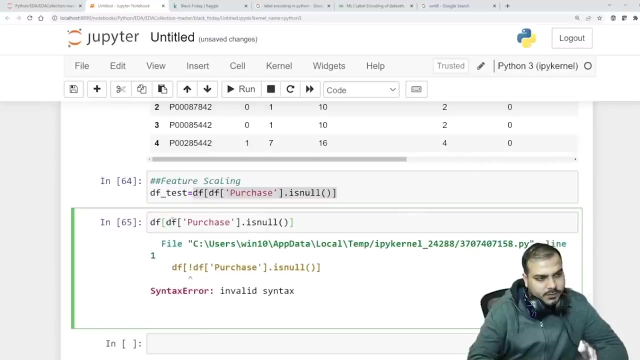 we are good to do it. we can also drop product id. Now let's probably do the one last thing, that is, feature scaling. This will now become my df underscore test, and then I can remove dfpurchaseisNull, See wherever the purchase in the purchase column. it is null. that all belongs to the. 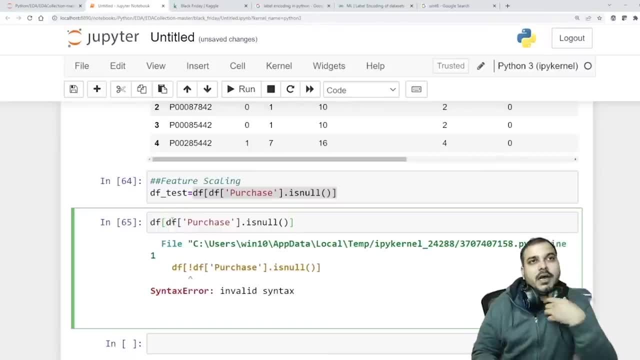 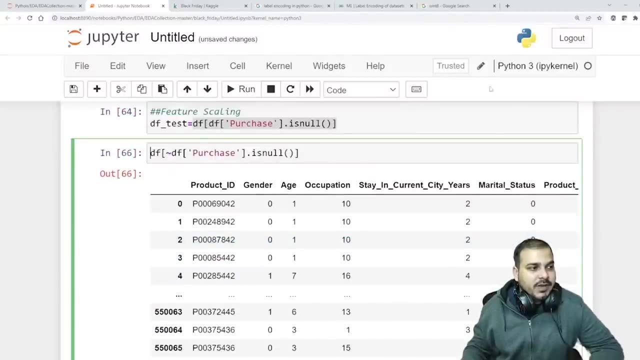 test data. So I'm just trying to find out, apart from isNull, how do I find out if it is not null? So if you use like this, so here, by this you will be able to see this and here you can basically write dftrain. 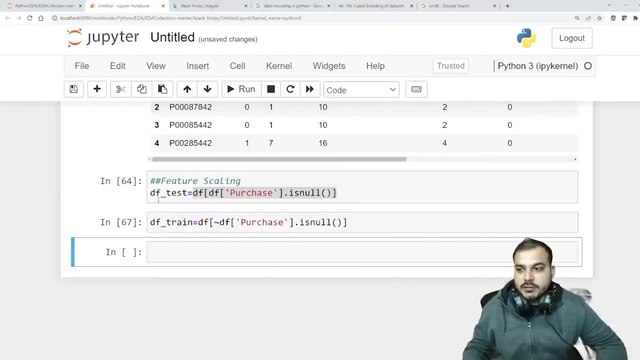 So now you have your dftrain and df underscore test. So df underscore, train and test you have Now. let's go to the feature scaling In the feature scaling. how do you do it? We basically apply standards, Standard scalar, as the feature scaling. 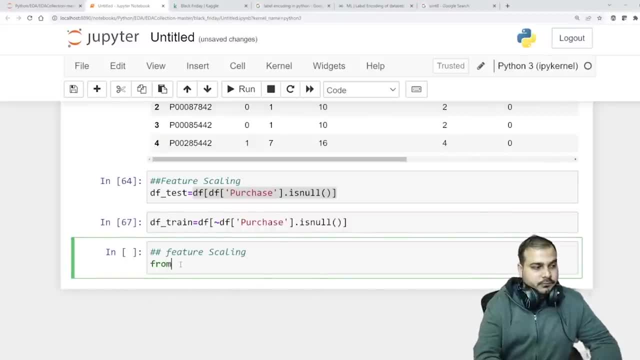 So for that it's very much simple. from sklearnreprocessing I'm going to import standard scalar and then I'm going to write: sc is equal to standard scalar. and on my train data set always remember df underscore test. Okay, Before that, if you want to do train test, split. 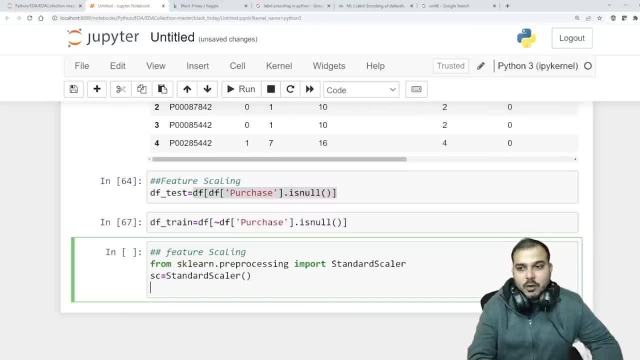 Define train test split. Okay. Okay, I can definitely go ahead and do it. I don't have any problem. So I can definitely write df underscore train. You can do that. x train, x test, y train, y test, It's up to you. 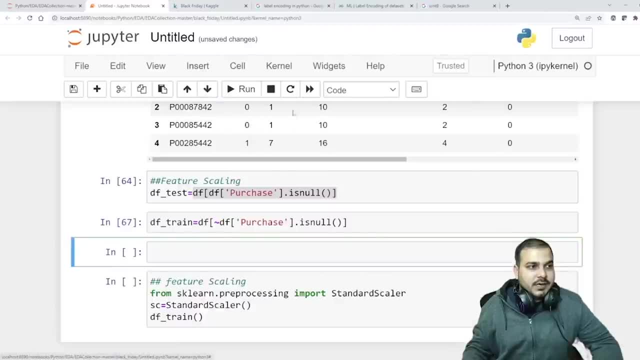 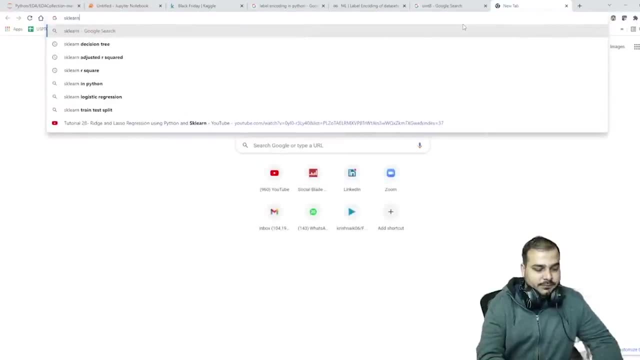 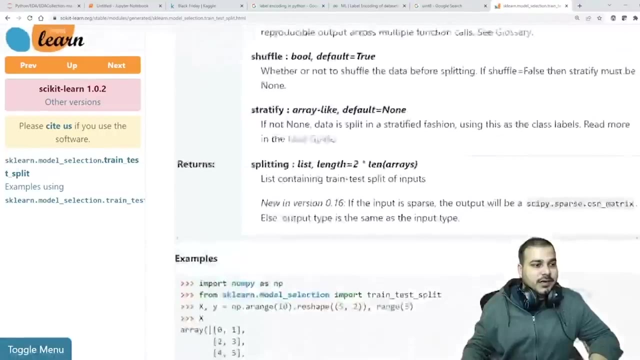 Okay. So before this, let me write one code where we will do the train test split for the training data. So here what I'm going to do: sklearn train test split. Okay, It is always good to Google it and copy and paste and do it instead of writing it. 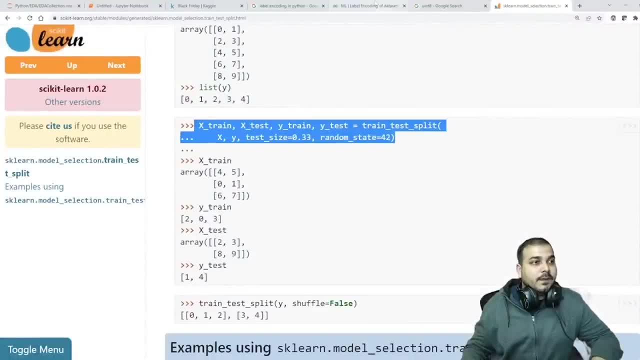 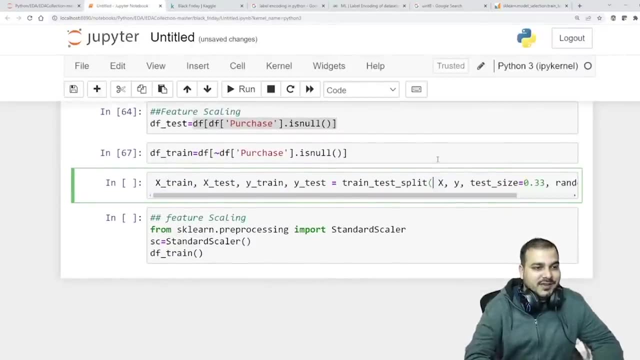 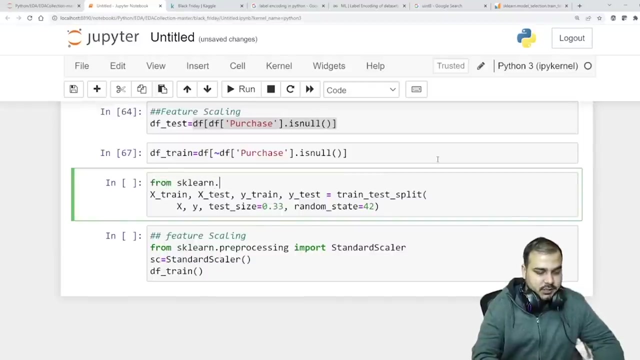 Okay, So I'm just going to copy this and paste it over here. You also do that same thing. Don't tell me, Chris, ping me the queries or answer. So here I'm just going to change it, But before that let me write from sklearn dot: model selection: import train test split. 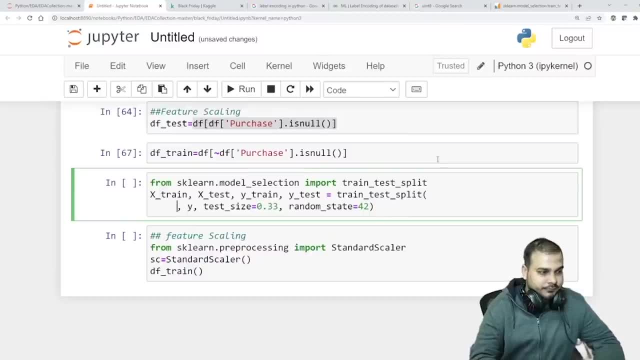 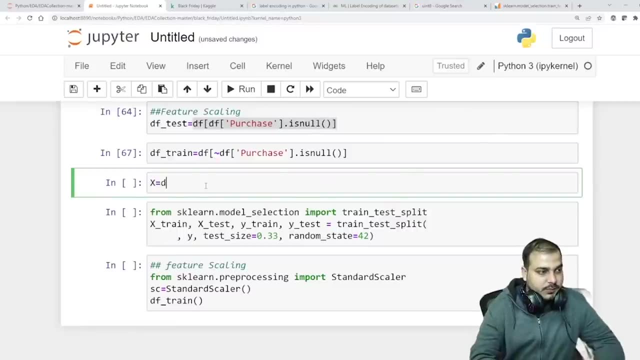 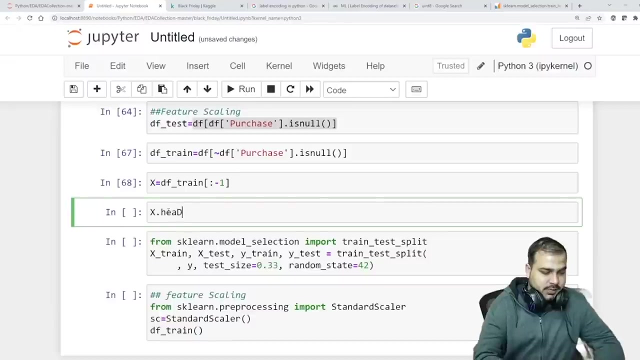 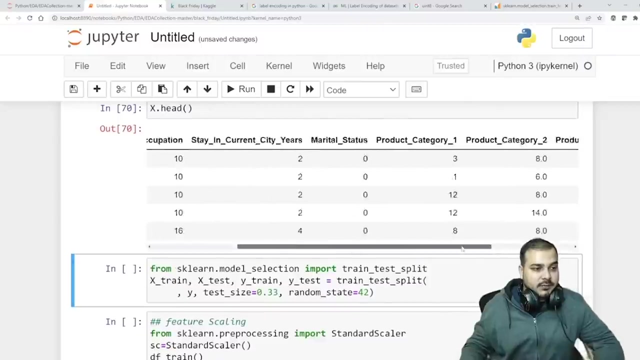 Okay, So here will basically be my df underscore test. Okay, My x. so my x will basically be df underscore train colon minus one. I hope so it works. So x dot head, just make our x and y axis so that it will get our independent and dependent. 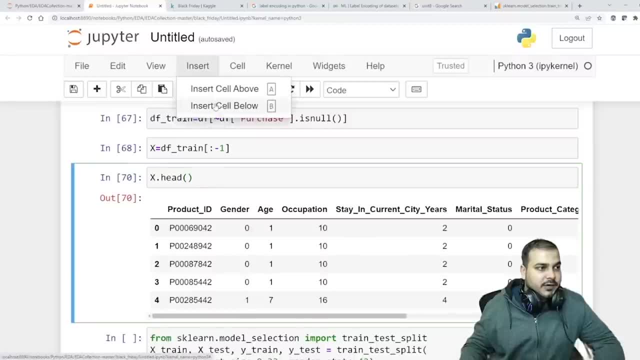 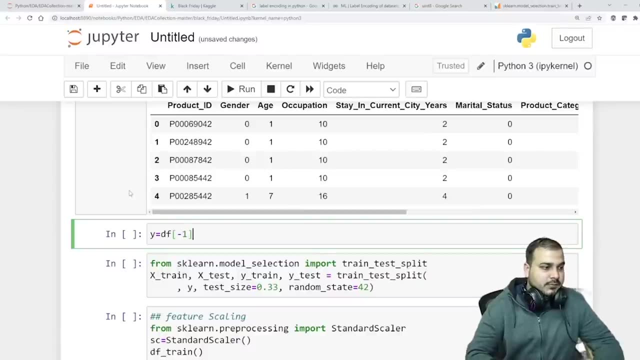 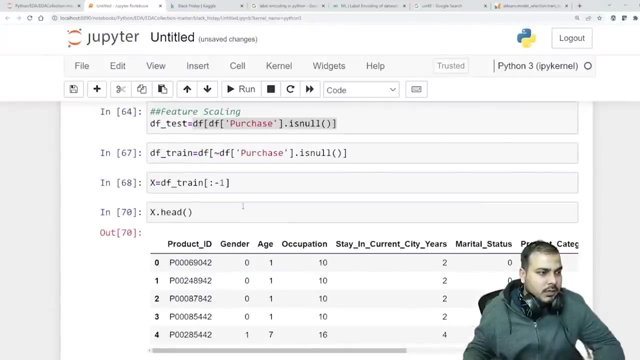 feature. So this is my x. Similarly for my y, what I will do, I will also create my y where I'll write df of colon No minus one. will basically give my okay Minus one is not there. Okay, Colon minus one, colon, colon. 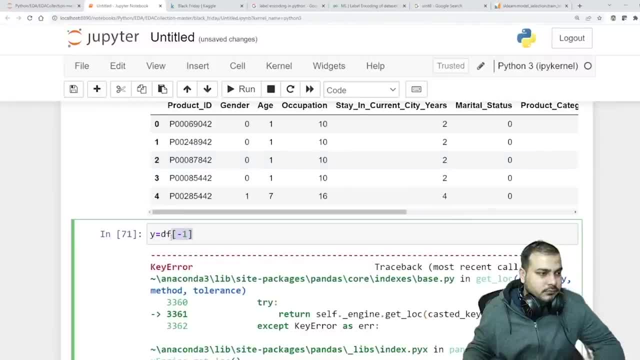 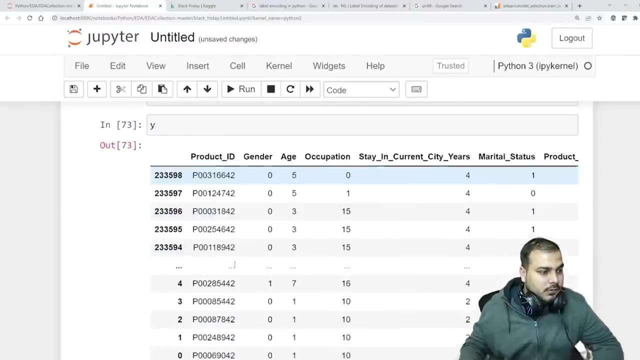 How do we get the last column? No df of colon minus one will give you the entire thing, double colon minus one. So So this will basically give your last value. No, it is not giving double colon No, just a second. 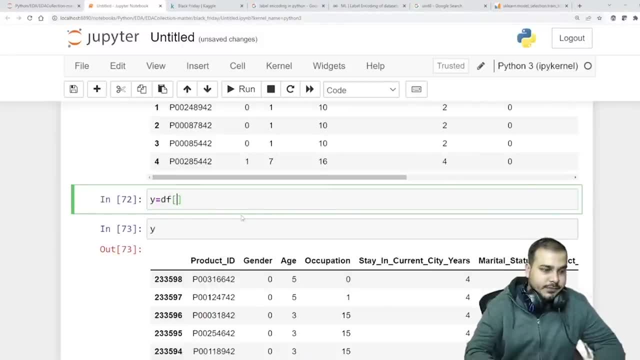 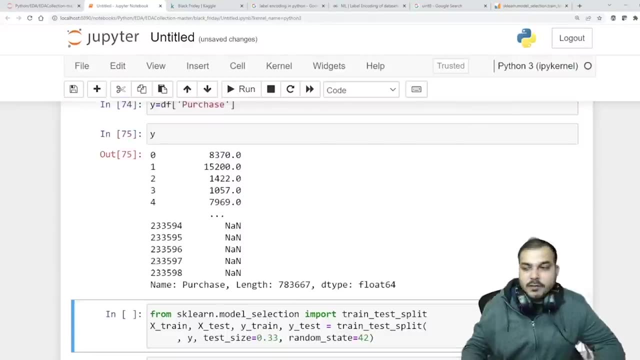 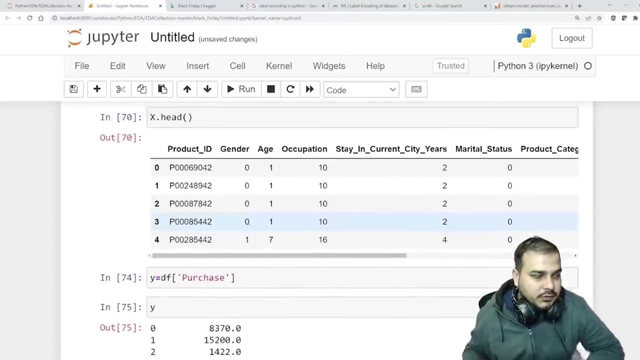 I can basically say it as df of purchase: right? So this is my y value. colon comma minus one will also work. colon comma minus one will also work. Just give me a second, guys. Yeah, So this is my x and y. 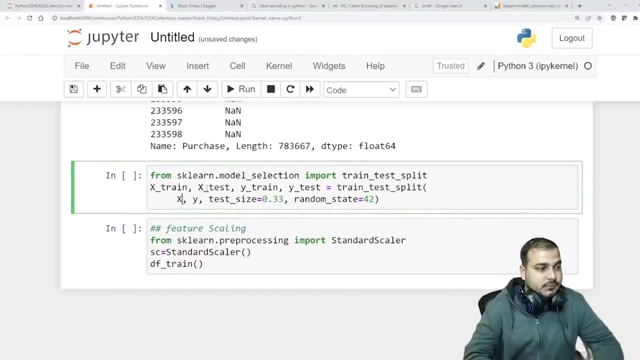 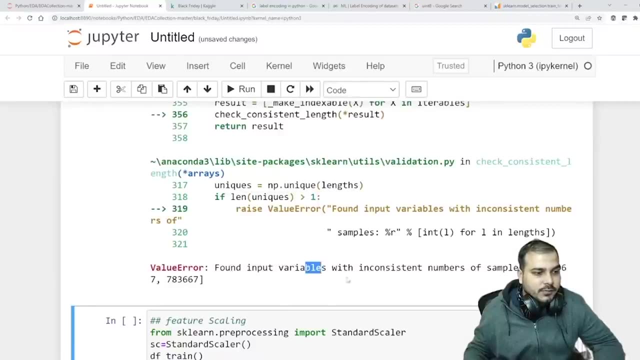 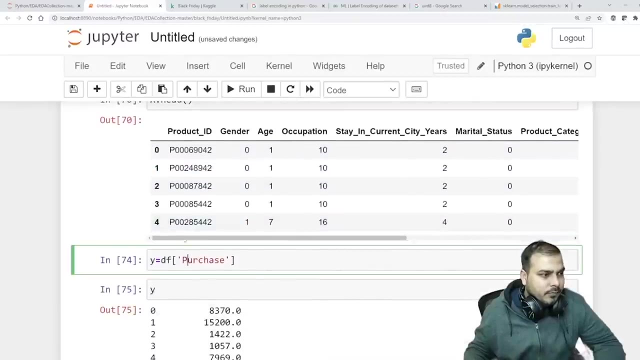 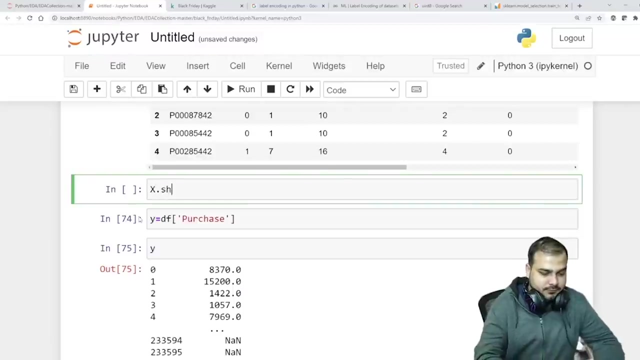 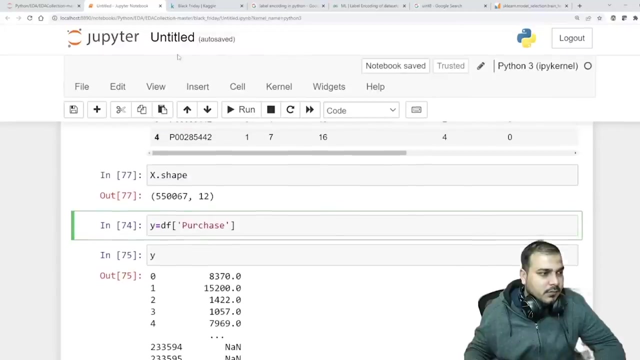 Now what I'm going to do? give it to my x and y here And here I will get a error. y upon input variable: the inconstant number of samples, comma 36y. I made some mistake. X dot shape. Let's see, this is basically having 12 rows. that is fine. 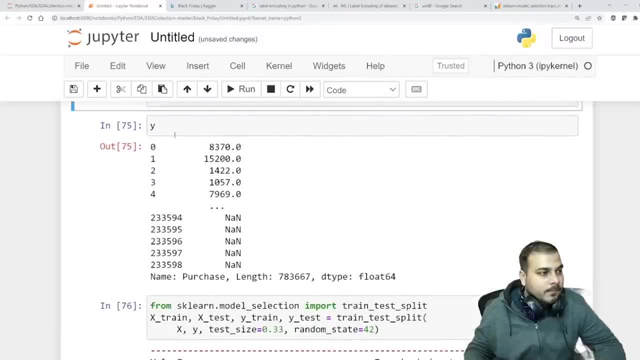 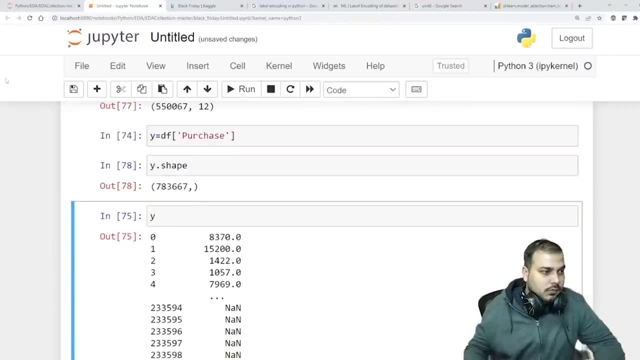 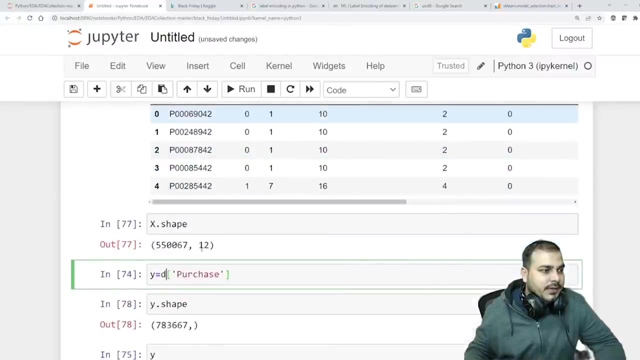 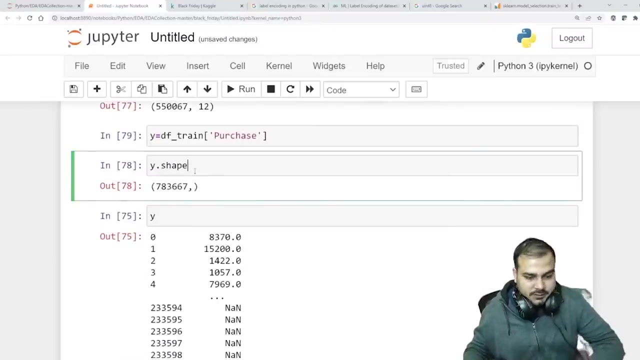 What is this? having Y dot shape? Hey, how come difference is there? My mistake, It should be df underscore train. Okay, That was a mistake that I made. Fine, Now it will work. Now I've got the same answer. 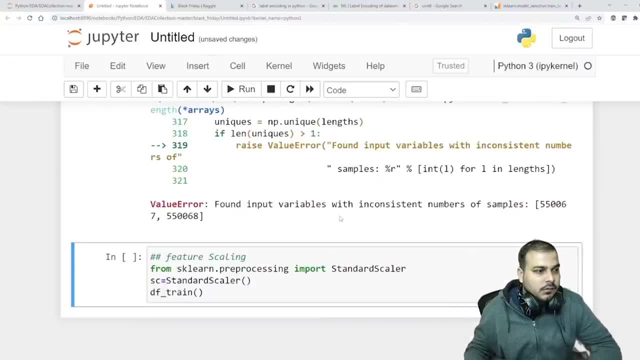 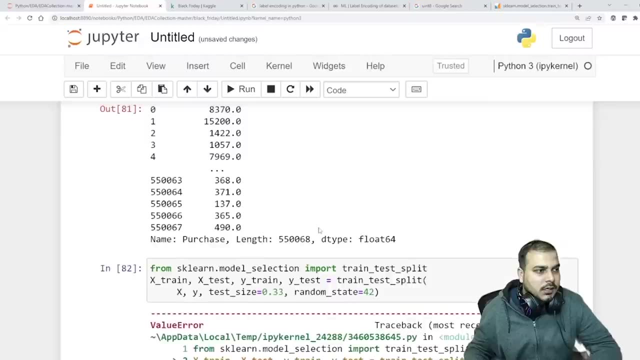 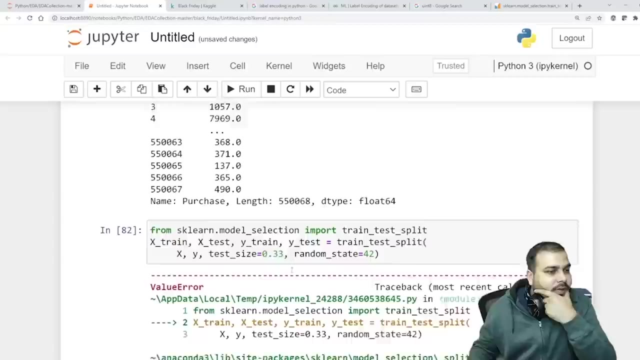 Here I will basically go and execute it: X train x test x comma y. df underscore train that I have written, but still I'm getting this error. Why A scalar normal model import train test? split this, this, this, this x comma y is there. 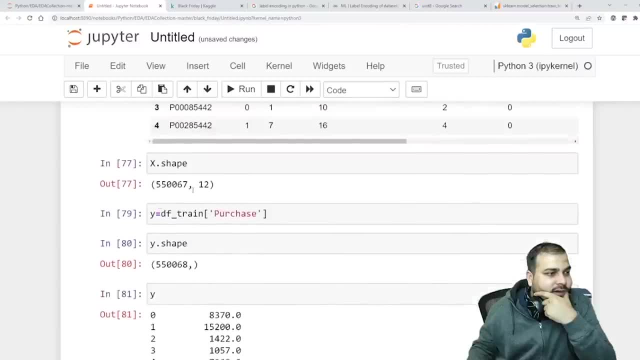 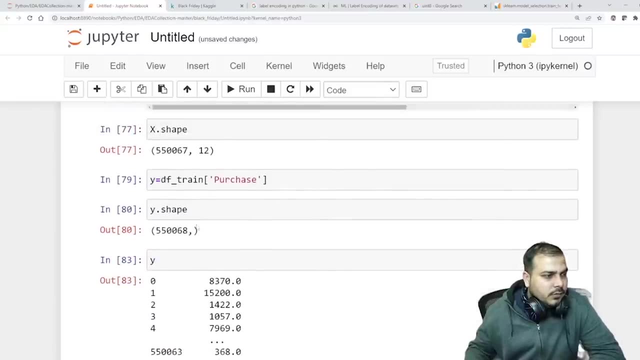 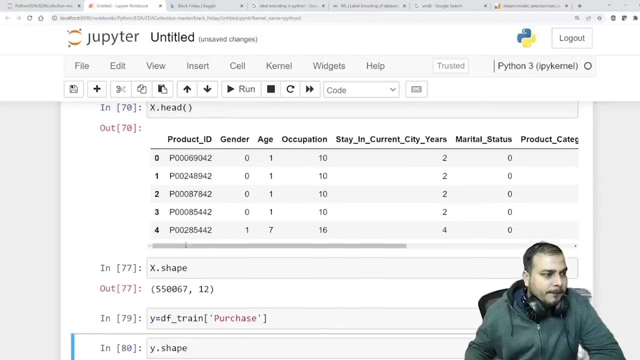 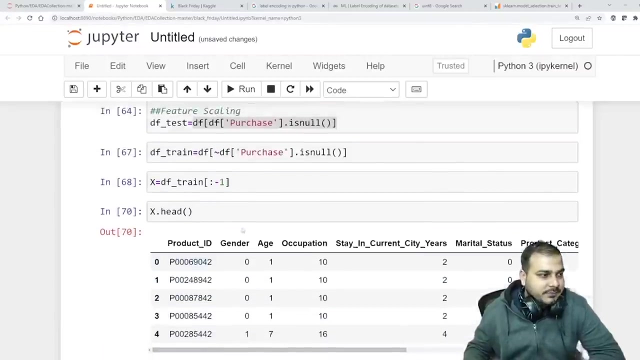 Y is also here, Y dot shape also. I'm able to get it Same. One extra record is there? How come? One extra record? How come Purchase is not the last column? Your screen is not visible properly, looking hazy. then please reload it. 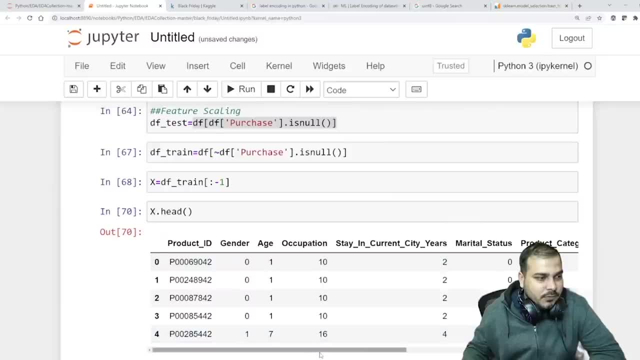 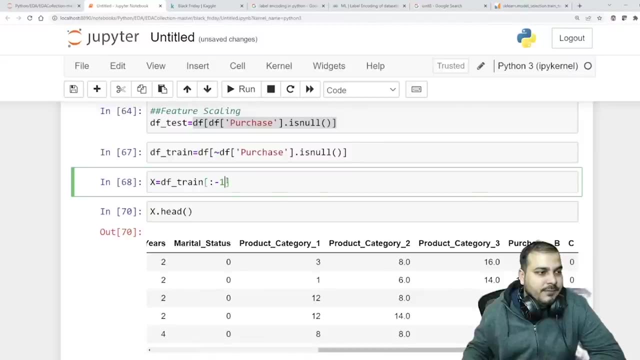 Okay, Purchase is not the last column. Your screen is not visible properly, looking hazy. Then please reload it. Okay, last column. that is a problem. so i made one mistake over here, so what i will do is that i can basically say: df, dot, train, dot. drop of purchase with axis is equal to one. now this: 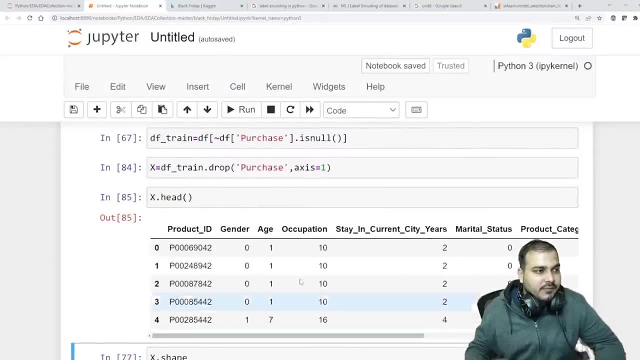 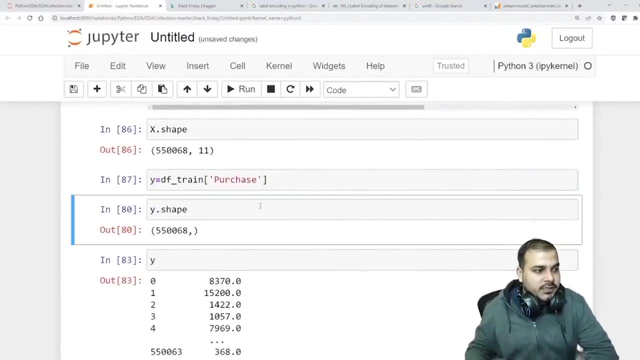 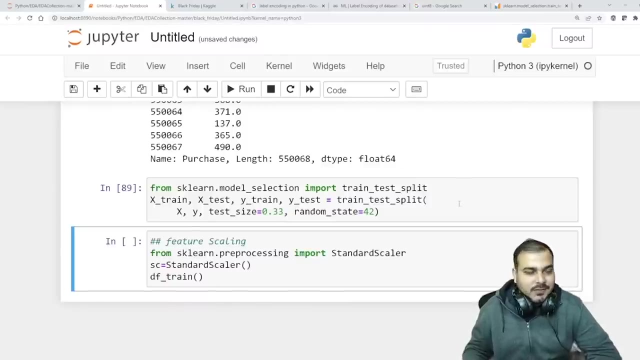 will definitely work. this is done. so i have all my features over here. if i do x dot shape, now i have 11 columns. then df underscore train. this is there. this is there. perfect, perfect, perfect café. it happens. i will google it. it happens now. it is fixed. see now df underscore train instead of 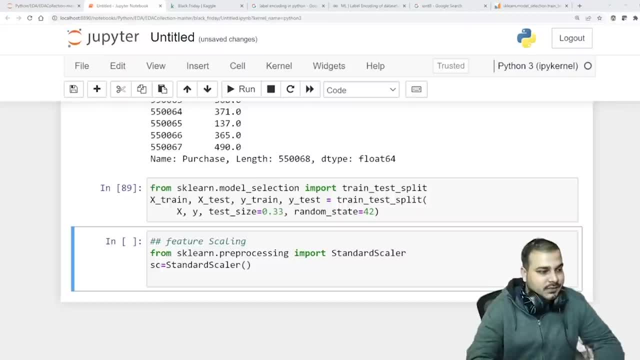 writing like this. now i'm going to do fit and fit, transform on extreme. so finally i will write sc dot, fit, fit, underscore transform. and here i'm basically going to write extremex kind of the genre will be this one, the google top, right into the top of the column, that's. 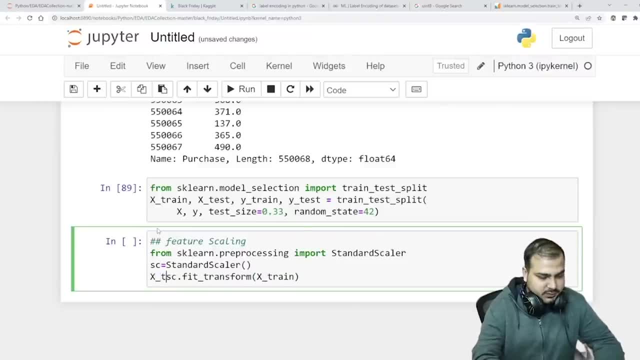 the form of our model, and now we will see that we al Bizhoped. then we changed it and we will just x underscore train, which will basically give me x underscore train is equal to this one. x underscore test is equal to sc. dot transform on x underscore test, y transform. think over it. 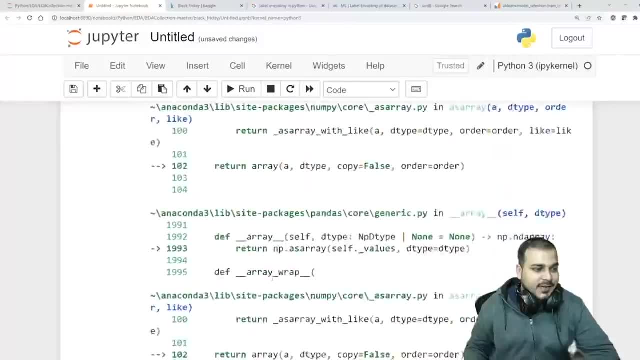 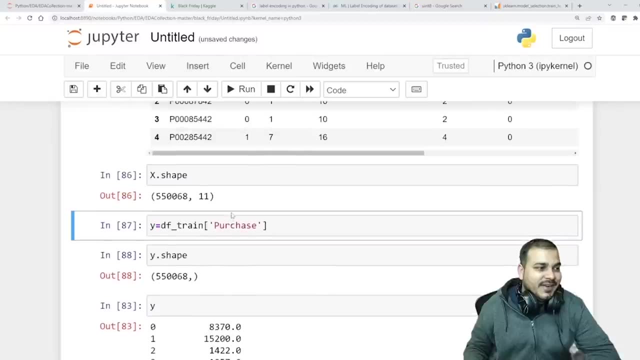 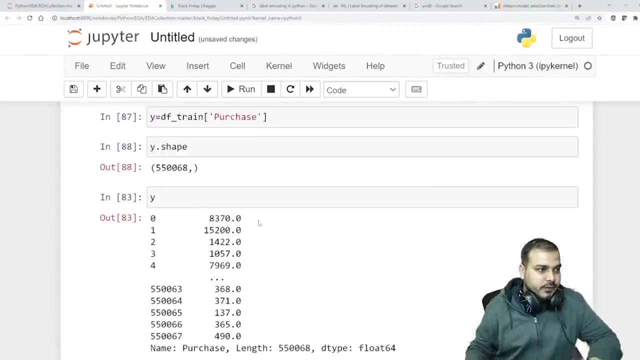 so let's execute this, and again it gives me an error. why could not? okay, let's drop one last thing from this. i think i could add: dropped in df dot train only and df dot test only. so just drop it. that will be an assignment to you all. i'm going to drop. the product id in place is equal to. 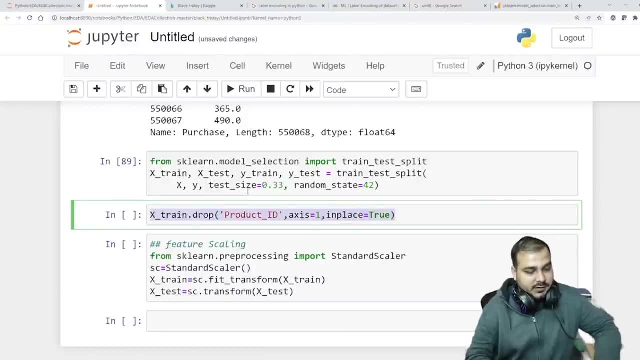 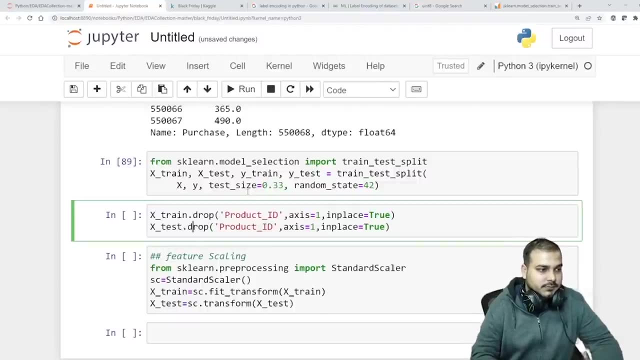 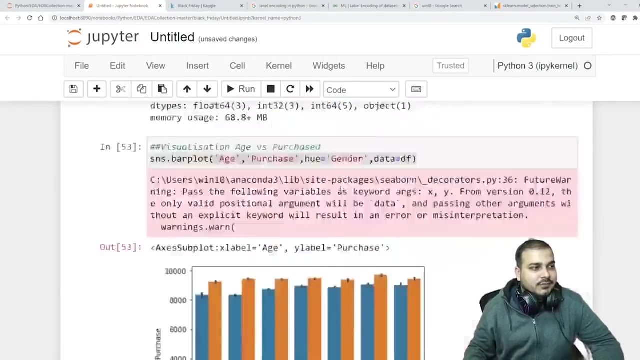 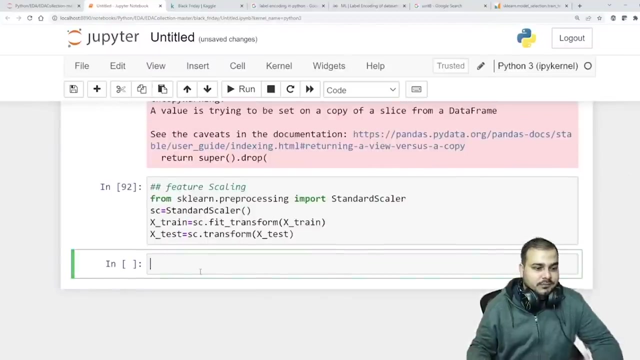 true, i don't want to get killed right now. x underscore test product id. this is done, finished. so 92 lines of code, more than 100 lines of code. i've written in front of you, did the complete analysis. now this is your data set. go and train your model. the next step is basically train your model. that's it. if 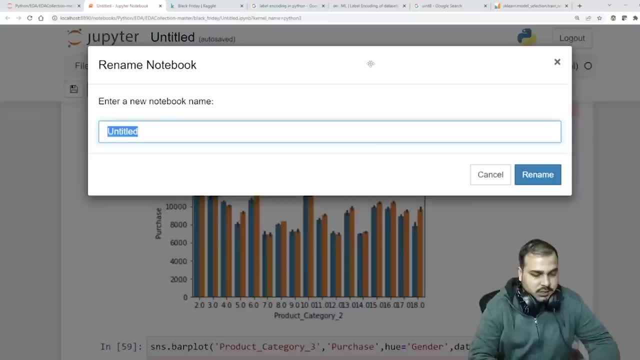 you want to see correlation, and all okay. so here i will just name this file as black friday eda and feature engineer everything i'll be giving you. i will be uploading this in my github. so that's it for today's video. thank you for watching and i'll see you in the next one. bye, bye. 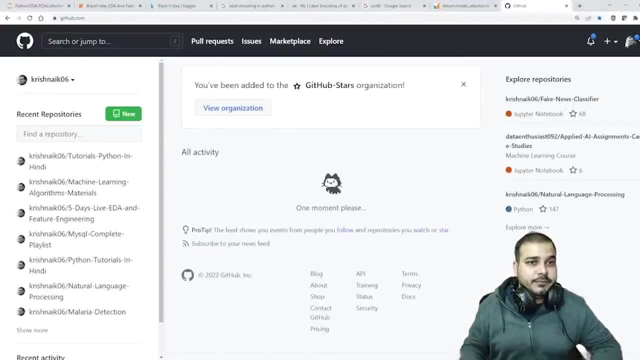 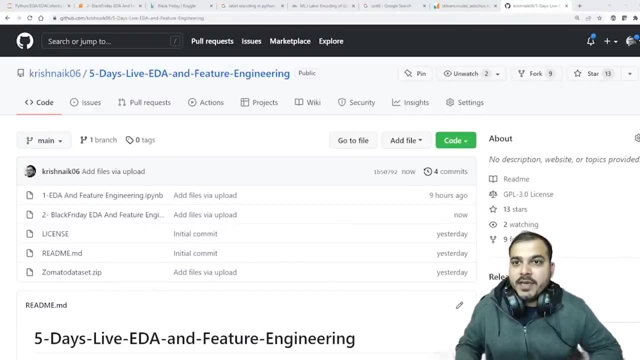 that you will be able to find it out. just a second, i'm doing it, i'm uploading it, okay, guys? so just uh, reload the page and uh, yes, you will be able to see the file in the description. so tomorrow also, we are going to take up any other different data set and then we are trying to see that how things. 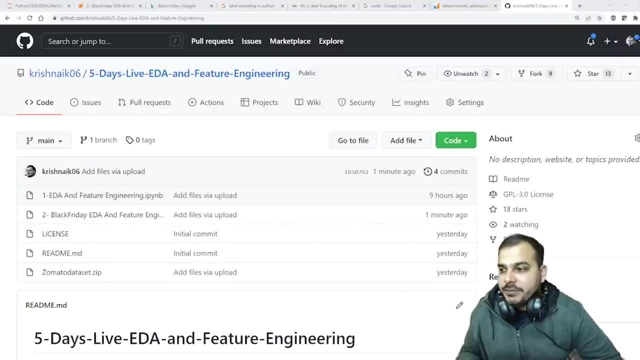 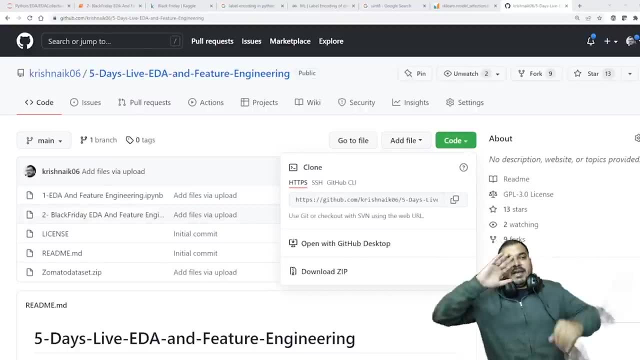 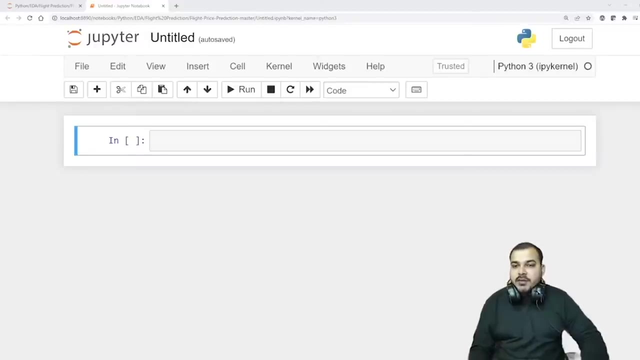 are going just reload the data set and tomorrow we'll continue the session. uh, thank you everyone for joining and, yes, i hope you liked it. so, thank you, have a great day. bye, bye, guys, keep on rocking. we'll see you tomorrow. hello, guys. i hope everybody is able to hear me out. so, from that, today we are basically going to solve flight price prediction. 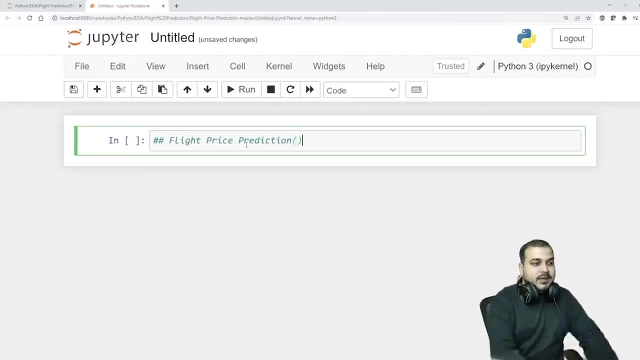 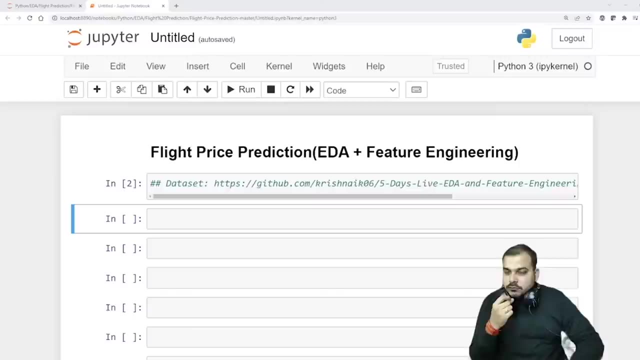 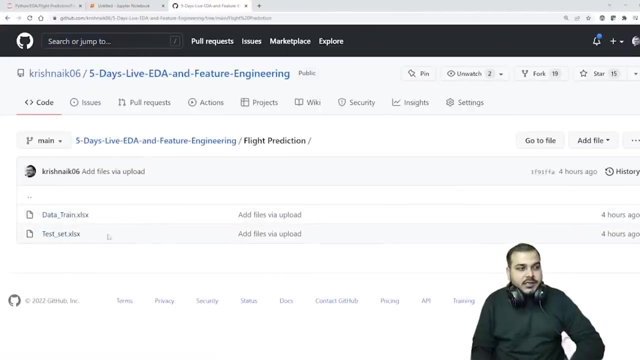 and here we are basically going to do eda, eda plus feature engineering. so data set. here i'm actually giving you the data set. so if you go and see the data set, the data set looks something like this: data train test set. okay, two xls file. 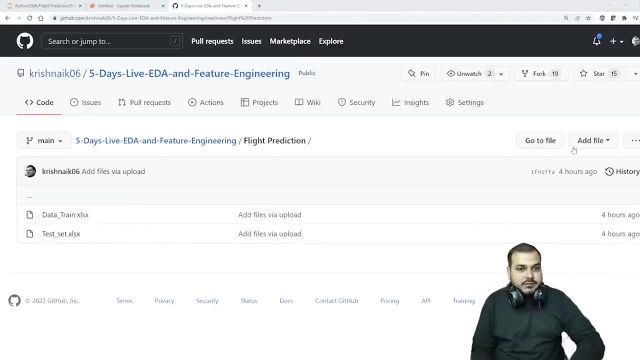 will be there, so you have to download these two files. if you want to download, make sure that go to this. download it right as a zip file. and inside flight prediction we have this specific data set, this two data set. we are going to take it up. data train and test underscore set. 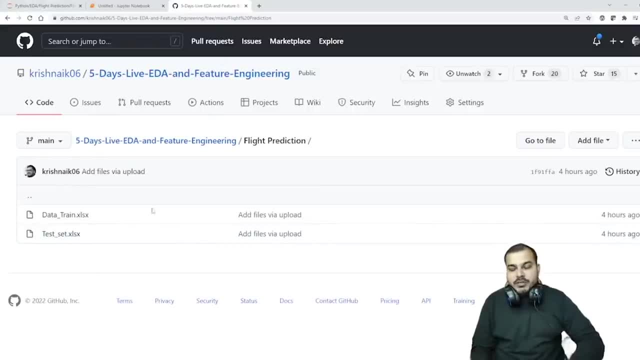 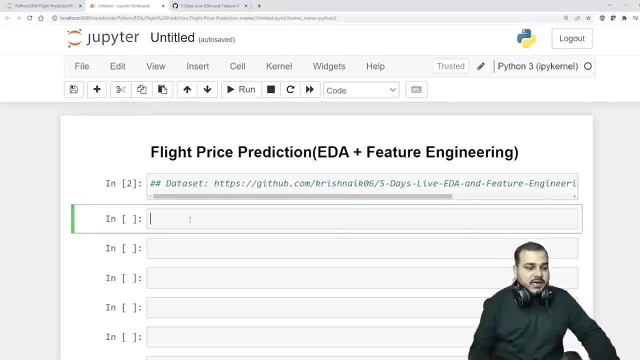 and this problem statement was given. this flight price prediction problem statement was given in a hackathon that we are going to basically solve over here and let's start. so initially we'll start with importing some basic libraries. importing basic libraries quickly, do it, which all libraries we require already. we have done yesterday. extension: i'll write: import pandas: spd. 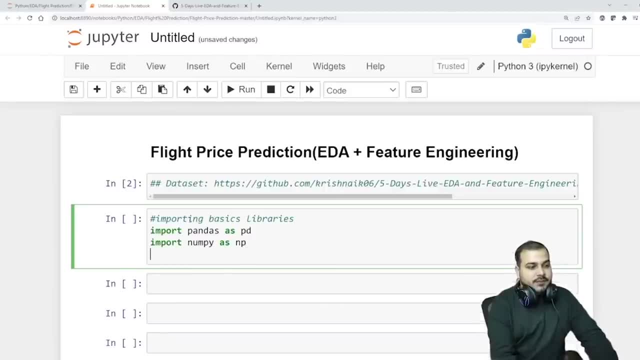 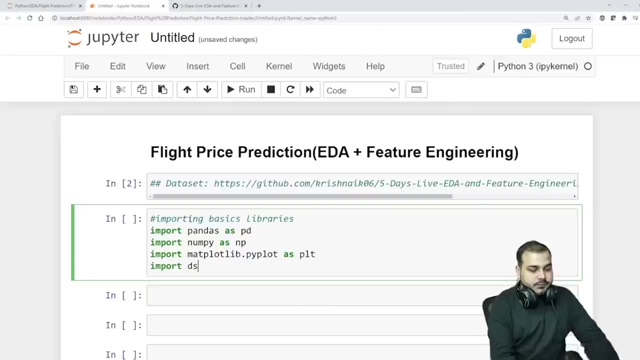 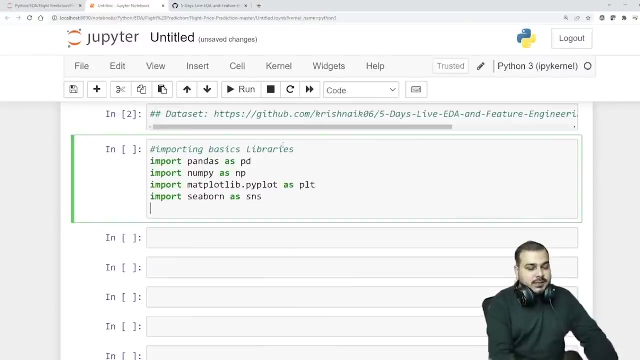 import numpy as np, then import matplotlib, matplotlib dot, pyplot as plt and then import seaborn as sns. import seaborn as sns and then probably we will also be importing. we'll write matplotlib inline. now, guys, many people usually ask me: what is this used for, matplotlib inline? see, suppose, if you want to probably show the diagram. 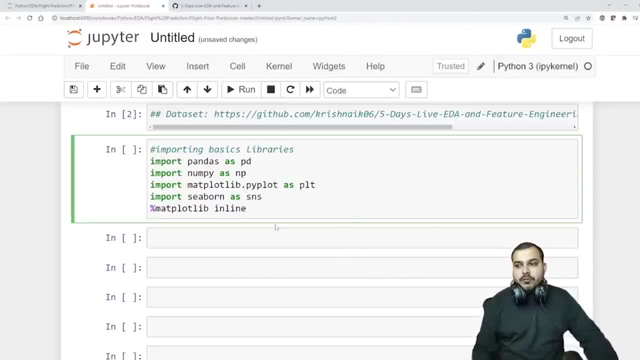 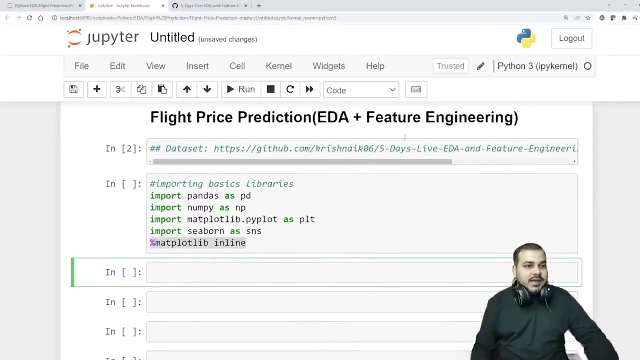 the diagram within this without writing plot dot show. so you can basically go, with respect to this one, matplotlib inline, so as soon as you plot anything you don't have to write plot dot show and automatically it will get shown over here itself. so, uh, now why i have specifically 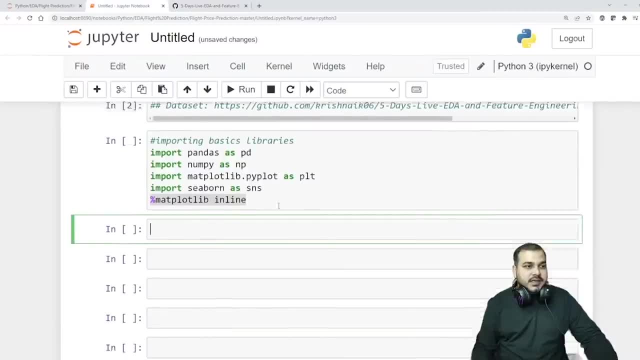 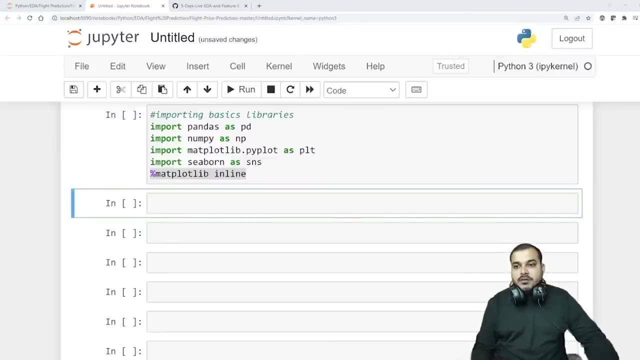 taken this data set because if we go and see this data set, there is something very amazing about this datastat because it also has date time information. okay, so date time information: you can have to really be careful whenever you are working at it. so that is the reason why i've specifically 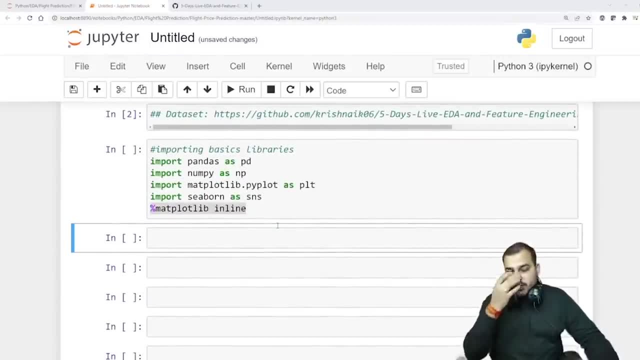 taken this because i wanted to show you different, different domain, problem statements, kind of data, so that you will be able to see, okay, what all challenges you may probably face into it. so, as usual, what i'm actually going to do, first of all, i'm going to just import the training. 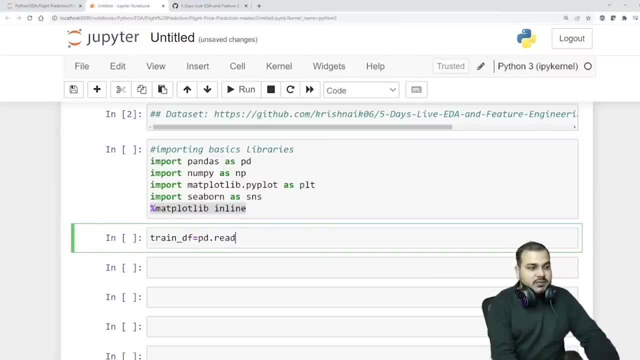 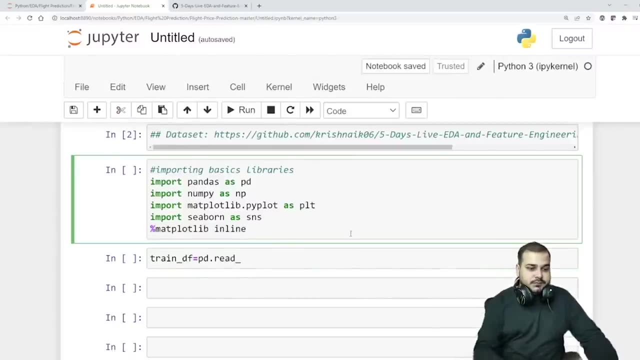 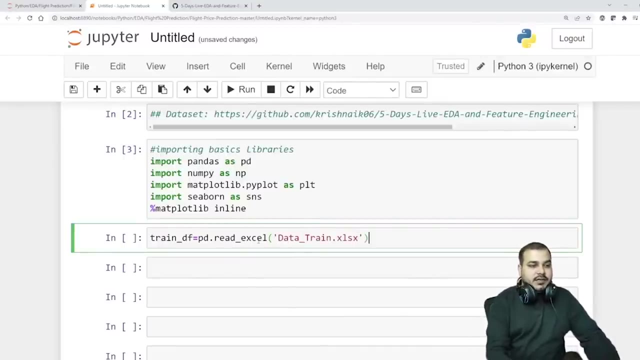 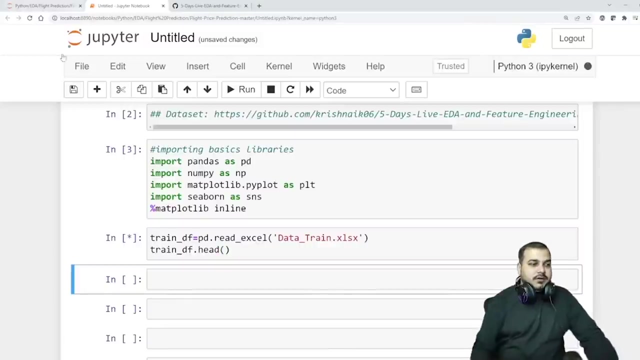 data set which i will write: pd dot. read underscore csb. read underscore excel. so let me just execute this one first. so read the data set like this: and here i'm basically going to give my data train dot xls, and if i go and probably see my train underscore df dot head, you will be able to see. 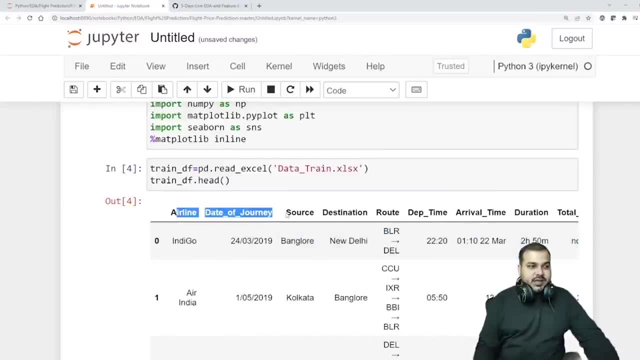 this specific data set. so here you have airline date of journey, source data set and i'm going to basically give my data, train dot xls and if i go and probably see my destination route, if it is given like this, bangalore to delhi, departure time, arrival time: 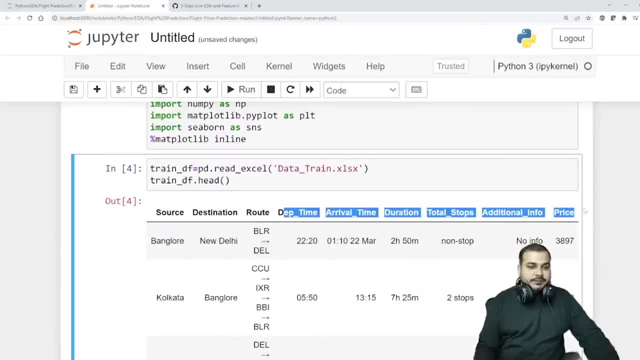 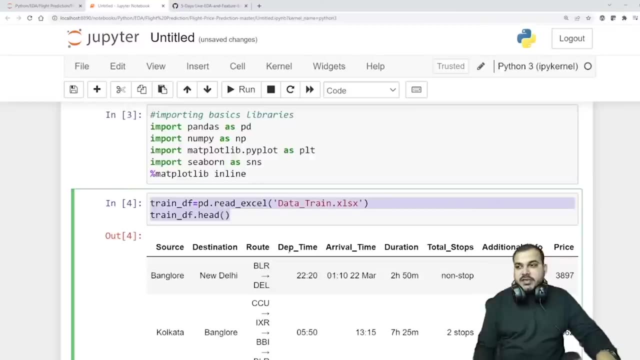 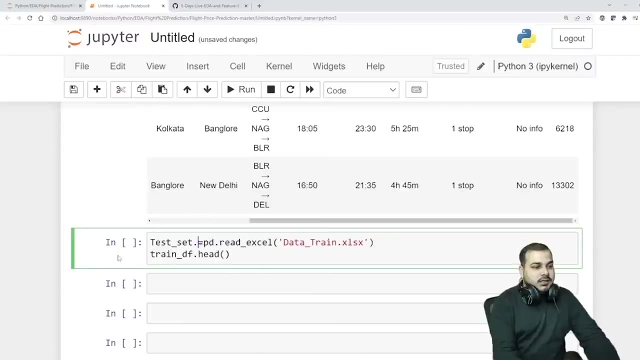 duration: total stops, additional info price. so after this, what we have to probably do is that same thing. i'll do it for the test data set. so here i'm going to basically do it for test data set. so test test underscore df, and specifically here i will write test xls. this is the file name. 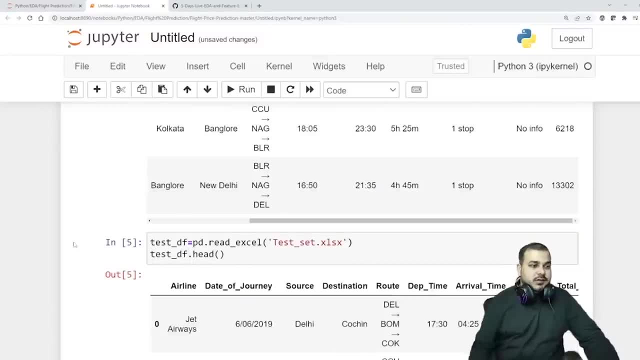 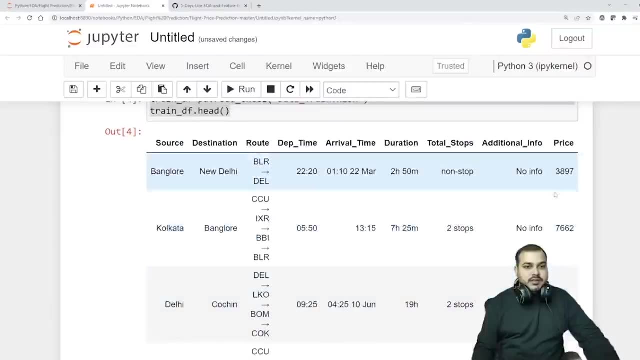 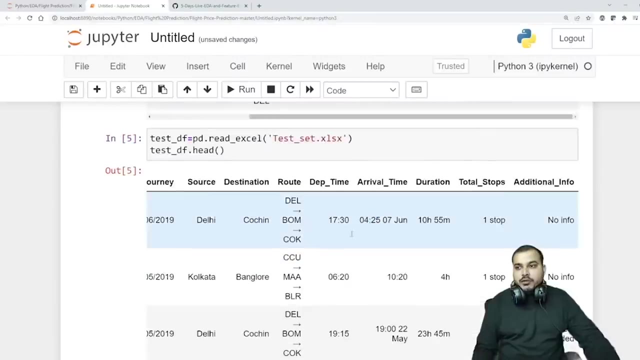 and if i want to display test df dot head. so here in my test data only one column will not be there, which is this last column that you can see. that is price. so this, both are done. you hope everybody is done now, as usual after importing. i did not try. 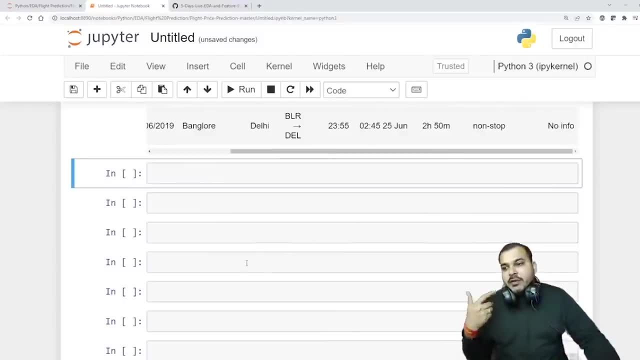 training the model. see if you are getting model score bad, like 12 percent, 13 percent, with the help of linear regression or other algorithms. try different algorithms. right, like other algorithms are also there, like decision tree regressor, random forest regressor. right, you have xg boost regressor. no one tried that, i don't know. we are just saying 12 and 13. 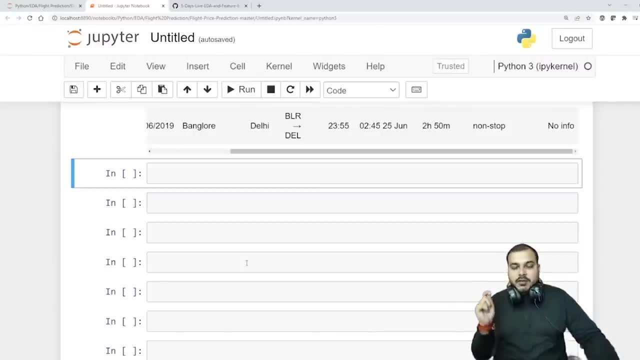 percent of the model score is bad, so i hope everybody is done now as usual, after importing all the 105 percent values. that was is above the reference meter is exactly. ah, oh, that is not. five percent. linear is actually not so negative. you will try 10 percent or 11 required. i'm just 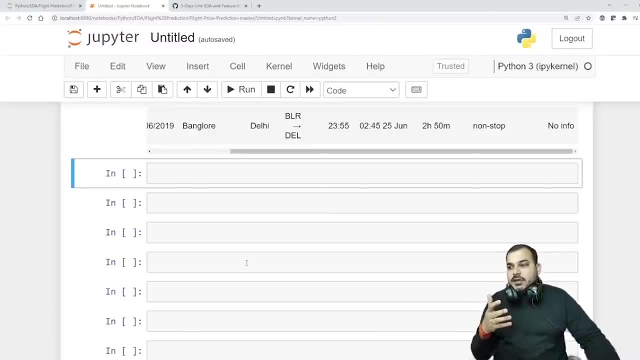 keeping hieroglyphics sick. and the third and fourth percent for linear and law hybrid. you will try up the technique ofadı, nothing else like u two. no one needs anyone's help. you stand up, just focus on thinking. so where i've taught all the machine learning algorithms previously. 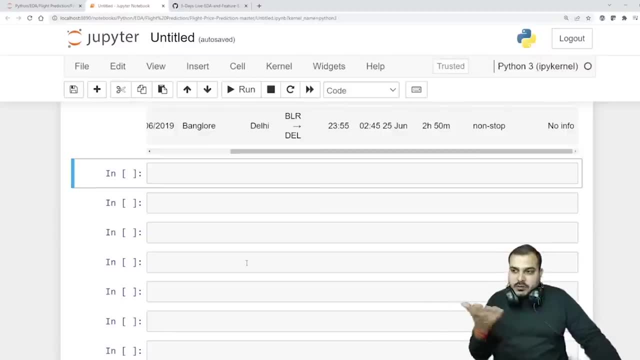 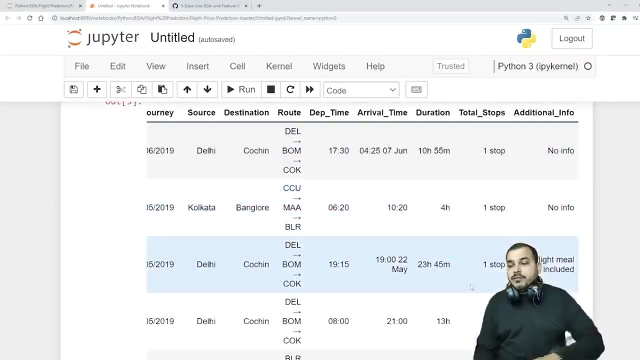 why don't you want to try with other machine learningvs? why you don't want to try with other arcades using visual discretization? you won't get this much common sense. it will be bad. if you don't get this much common sense, then i think, trust me for cracking interviews become 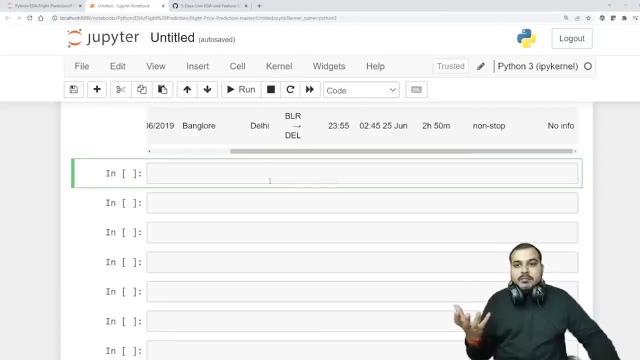 use different, different algorithms. so i i always tell you, do hyper parameter tuning on top of it. i, i just did linear regression, sir ridge, sir raso, sir, i got 12 percent. now tell me what to do. i don't want to do anything like that. you'll learn tomorrow- you'll give a no problem statement- how. 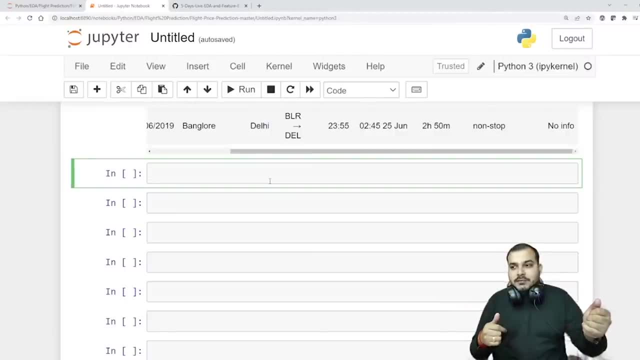 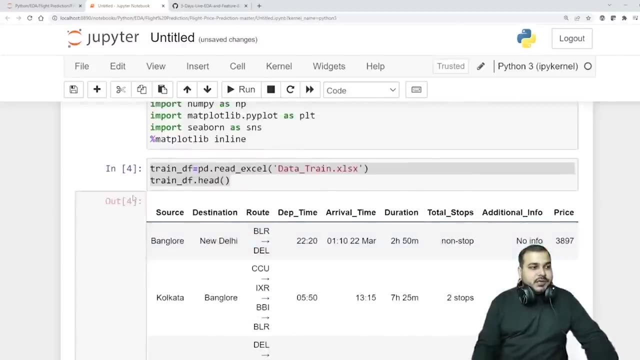 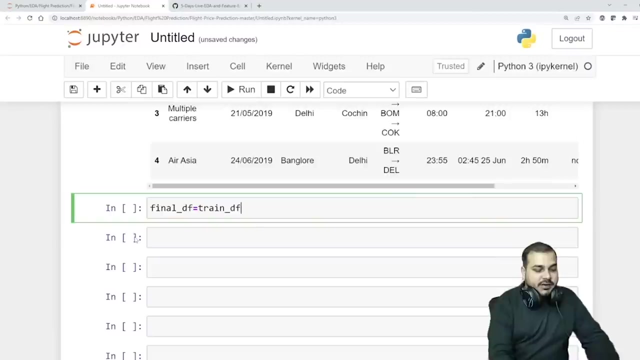 you'll do that. at that time krishnayak will not come right. so let's do one thing. first of all, i'm just going to combine this train df and test df into another variable called as final df. so what i'm going to do in order to combine, i'll just write train df, dot append, and then i'll write test df. 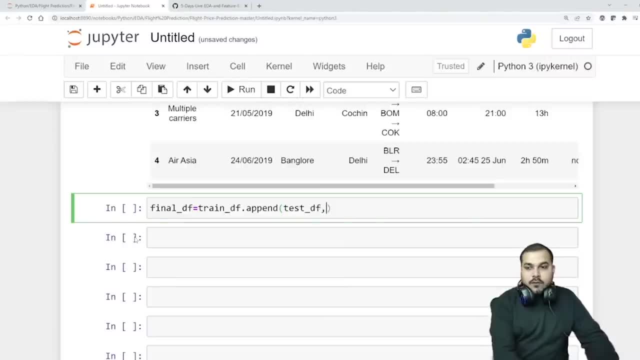 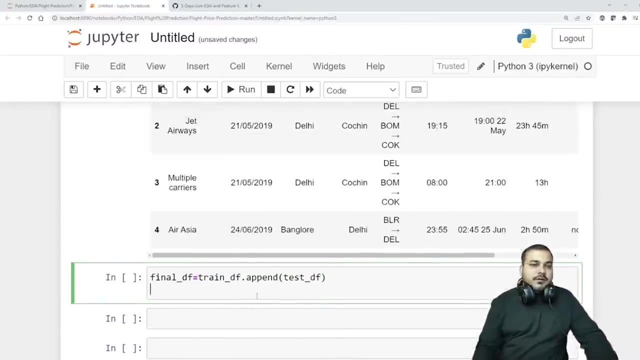 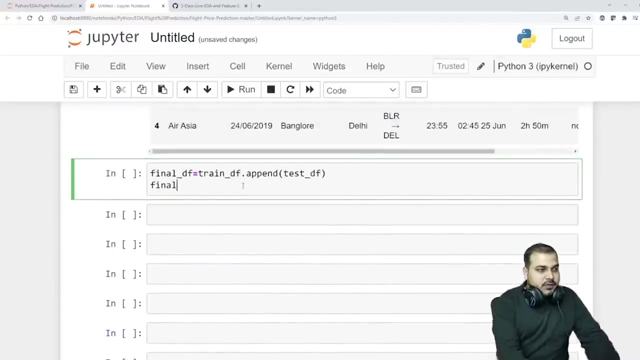 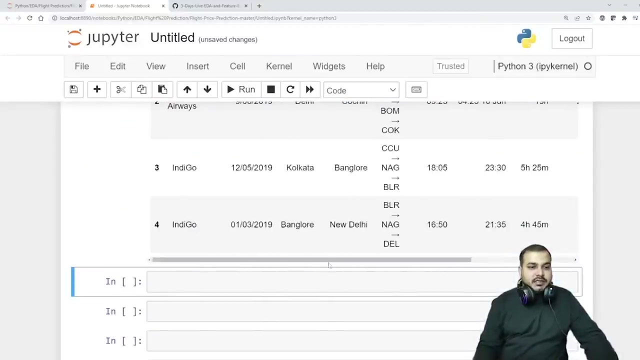 comma and train df dot append of test df. so test df is my this data set and train df is this data set. so once i will do this, i can go and finally write final underscore: df dot head. so this what i'm doing: i'm combining both the train and test. 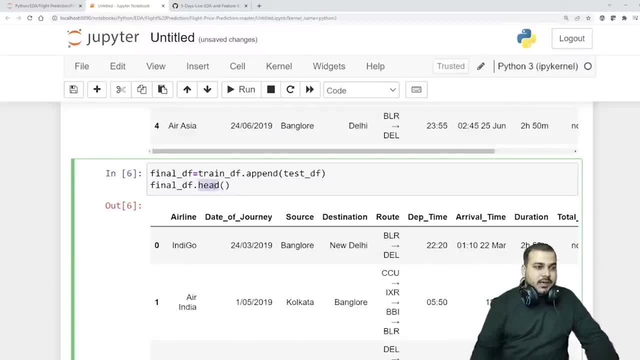 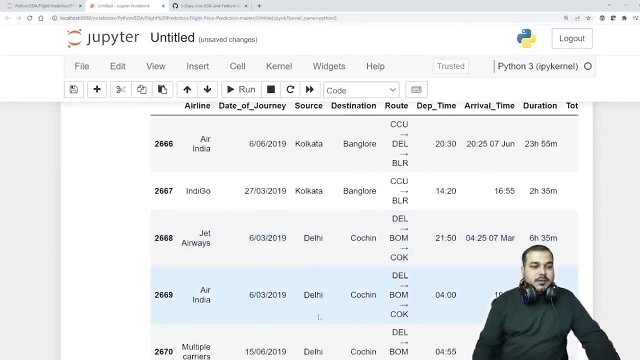 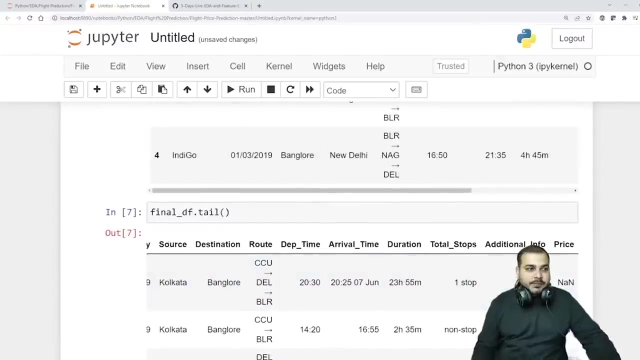 remember if i go and see the tail path. if i go and see the tail path, then you will be able to see that you'll have some nan values in the prices. this is because of the test data set. okay, so this much. i think you will be able to see that you will have some nan values in the prices. this is because of the test. 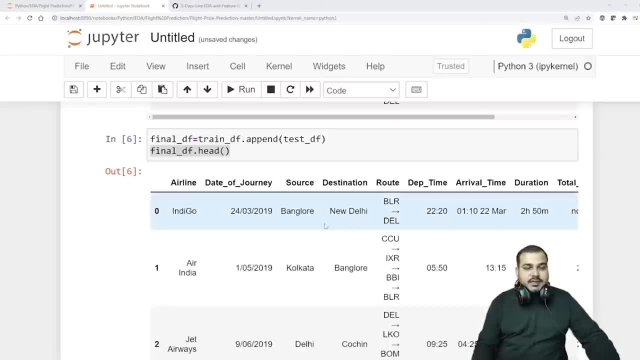 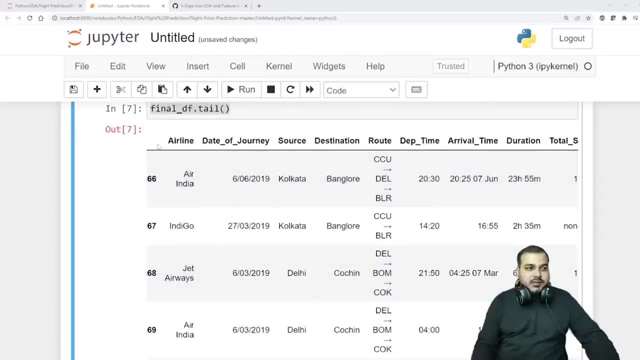 data set. okay, so this much. i think you will be able to see that you will be able to see that you will be able to see that you will be able to do it appending the data set which is getting converted into this one. now see, the features looks quite complex over here because the feature that you 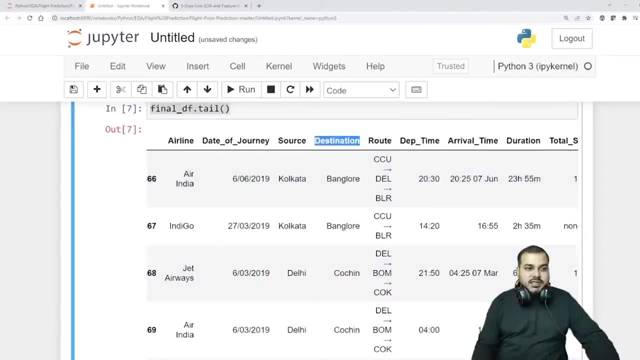 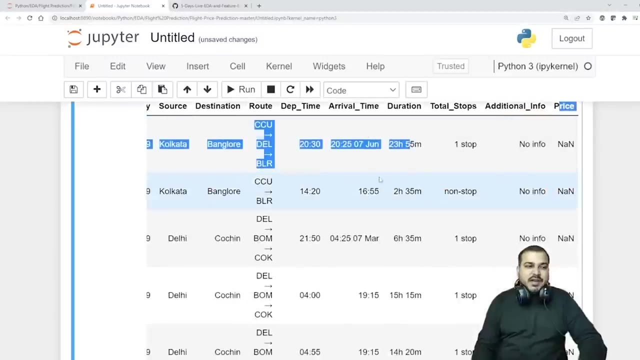 have is like airlines: you have date of journey, source, destination, route, then departure time, then arrival time. you know arrival time, then you have duration, then you have total stops, then you have additional info. very you different, different types of columns are there there. so a lot of feature engineering is basically required, and here i'm just going to focus more on. 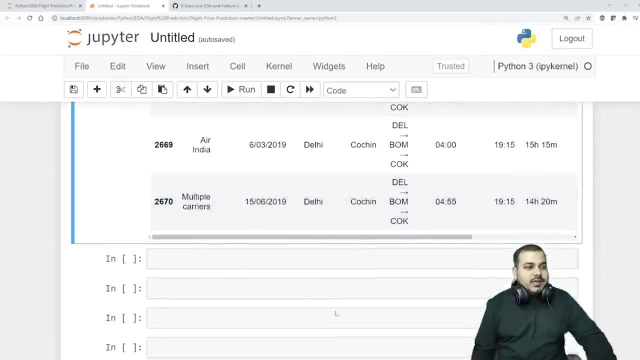 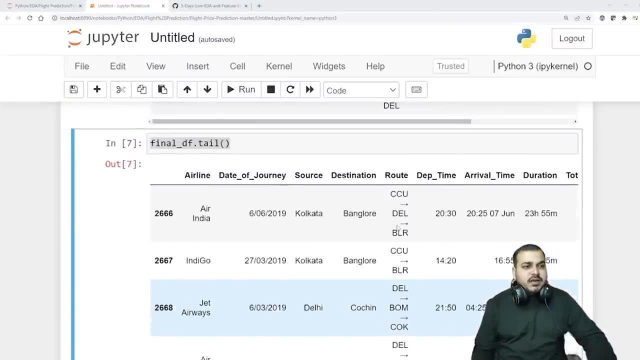 feature engineering, because we have done extensive eda, now let's go ahead and try to do feature engineering on each and every field. okay, now, the first field that you may probably see over here is something called a date of journey. now, in this date of journey, you have, obviously you have a day. 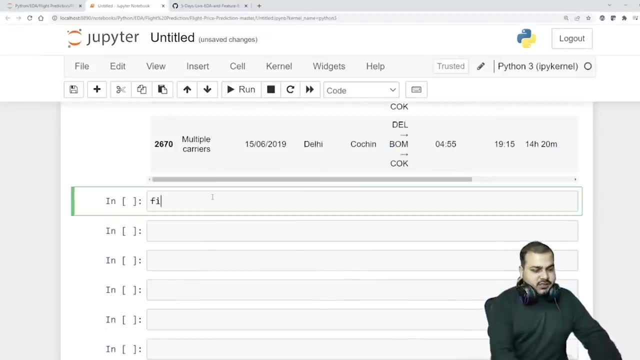 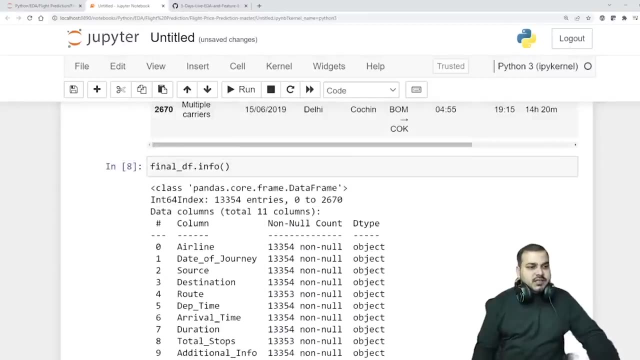 you have months and you have year and probably just let me just write final underscore: df dot info. so here you can basically see that date of journey is also an object. so date of journey is an object. that basically means it is in a string format. so we have to convert that into a date time format. 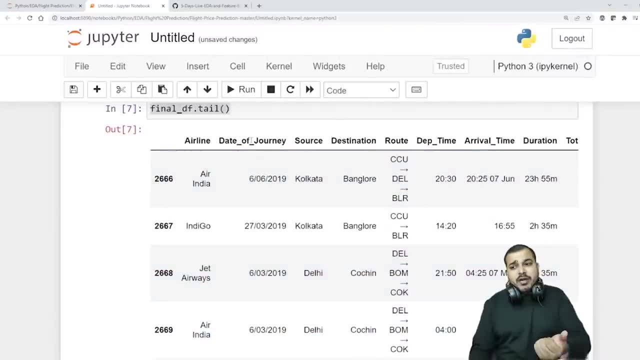 now this, after converting probably into a date time format. what i will do is that i i need to pick up this specific information like day. this will basically be my month and this may probably be my year. so this technique, from this particular field, i have to create three more fields which will 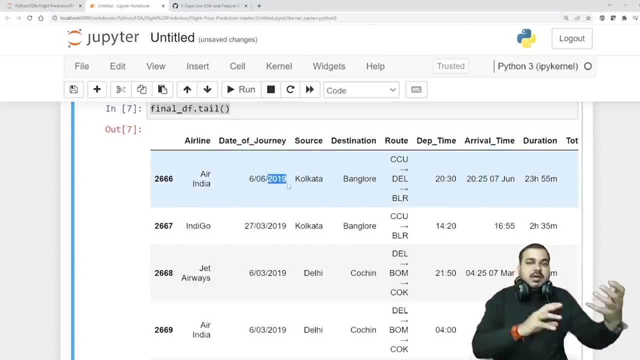 specify my day, month and year. so here, what do we say to this is that we are trying to create a derived feature. now tell me, guys, from date of journey. how do i create this? three fields, anyone, you can actually try it out and you can basically let me know. you can try it out, you can say some. 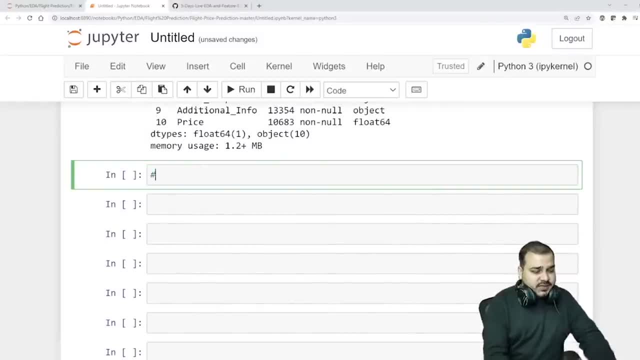 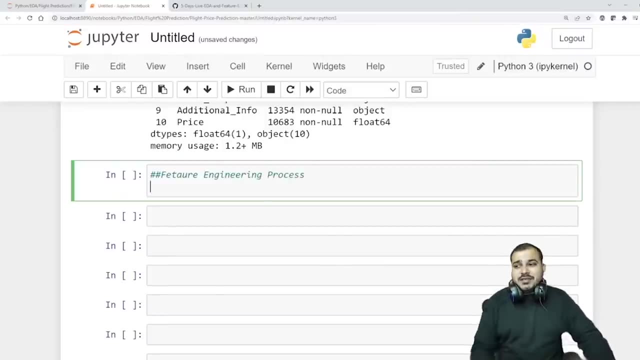 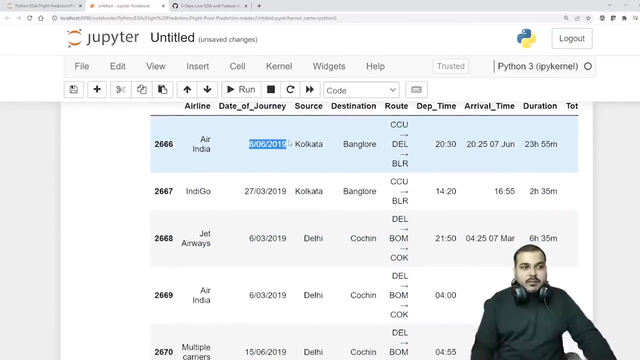 code how we should go ahead with doing so here. basically, i'm starting my feature engineering process and what i told that first i will try to take out or derive some features like from this: i will definitely be able to take out day, month and year. how do we do it? so for that, what i am, 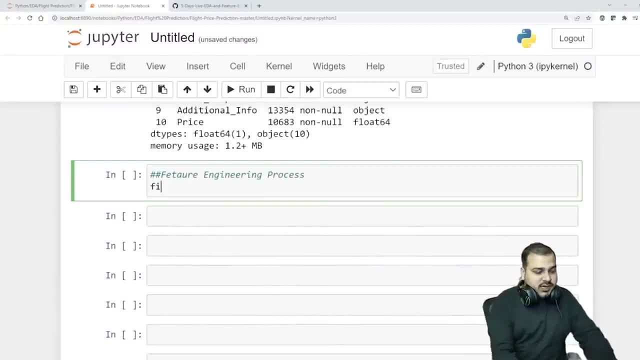 actually going to do it in a very simple way. i'm basically going to say that final underscore, df, and i will try to create three features. as i said, one feature will basically be my month or date. first i'll start with date, so one feature will be this, the next feature that i'm actually going to create. 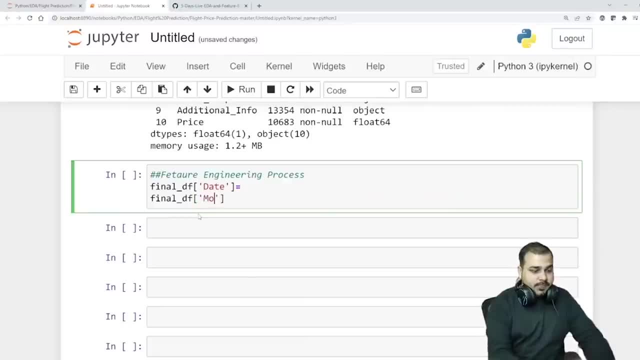 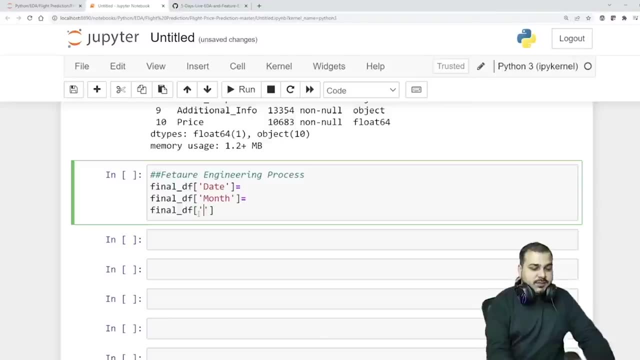 is with respect to month and the third feature that we are probably going to create is with respect to year. so this three feature we need to derive and we need to create. and how do we do it? we already know that i have a feature which is called as date of journey. right now, from this, 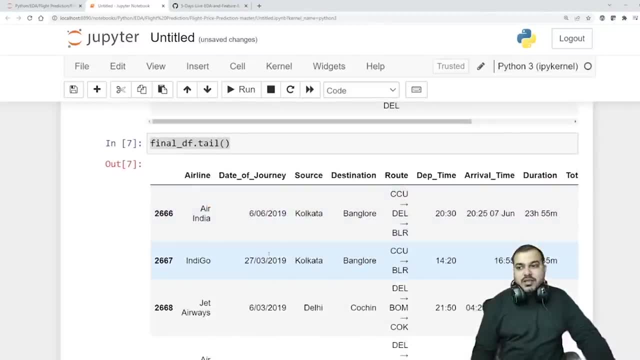 i basically have to split. okay, split by using what character? split by using this specific character, that is, this forward slash. if i do probably split, then i will basically be able to get three important information. one is this: 606 and 2019. now, in the case of date, i need to focus. 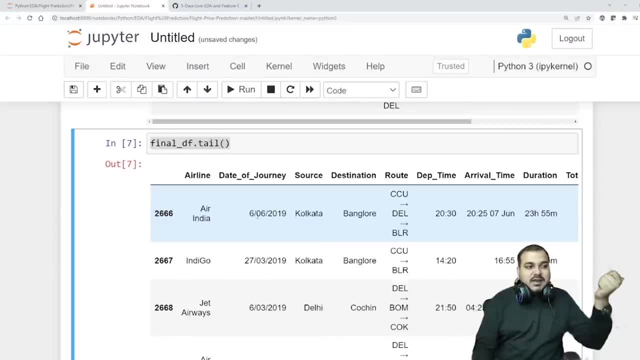 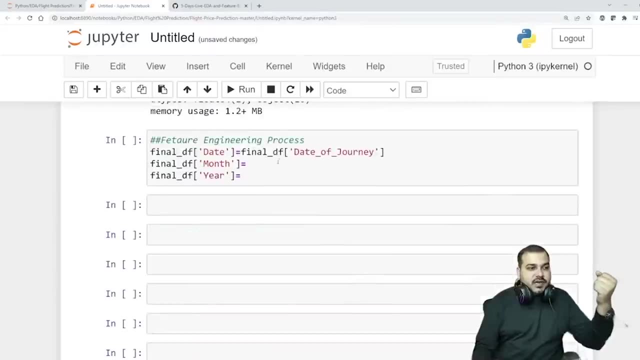 on the first index, that is, in the zeroth index. then in: in the case of month, i need to focus on the first index and in case of 2019, i need to focus on the second index. so that is what i'm actually going to do over here. so i'm basically going to write over here: dot, str, dot split, because 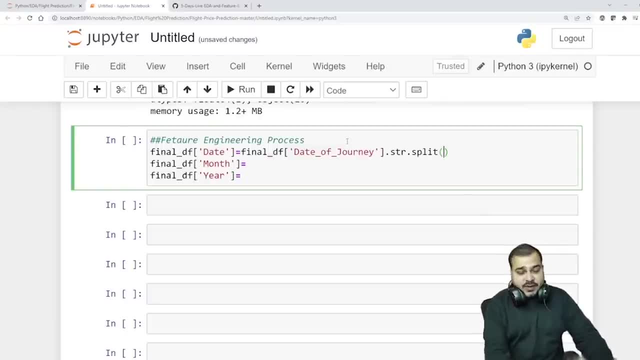 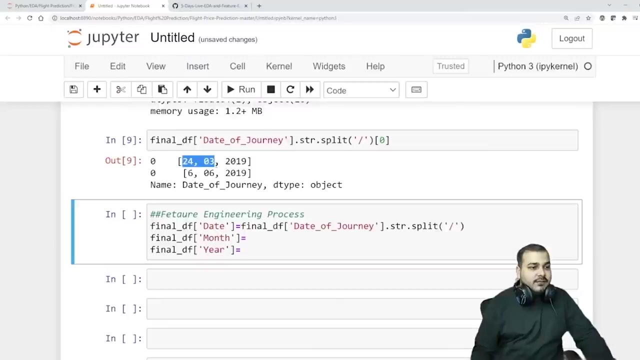 i have to convert that into an str. uh, if i need to basically do the split and after doing the split, if i copy this and if i run this code, let's see what will happen. you will be able to see over here. if i write zero, that basically means i will be able to get this all entire information. okay, so 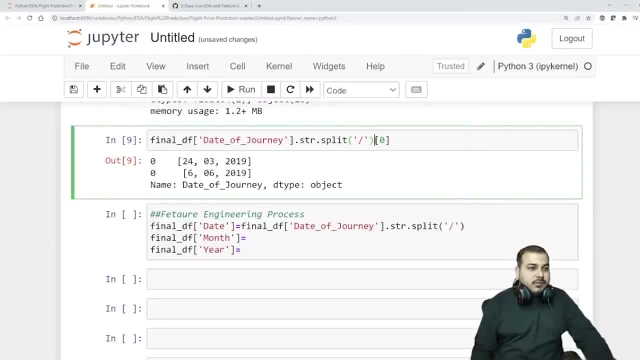 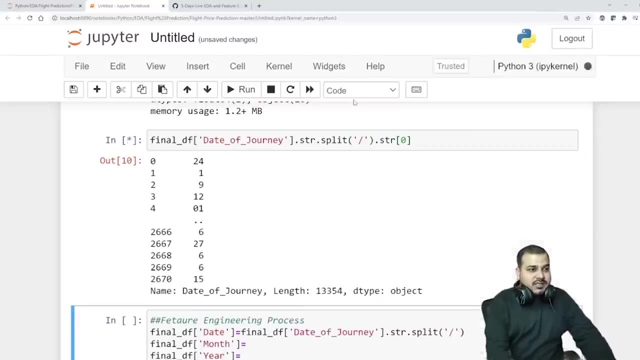 here you can see that if i write string- sorry, here i've written zero- then also i'm getting this specific information. what i will do: i'll also use one keyword called dot str of zero. so here you can see that i'm able to get all the dates. okay, so this is. 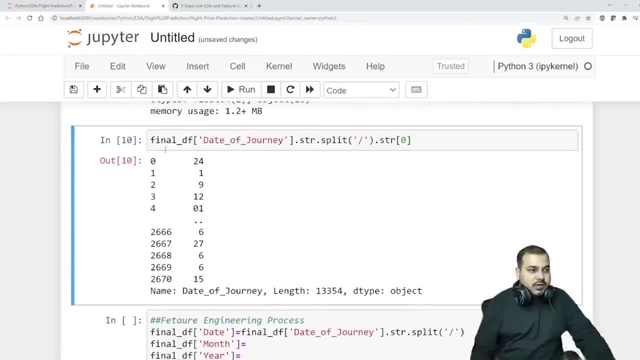 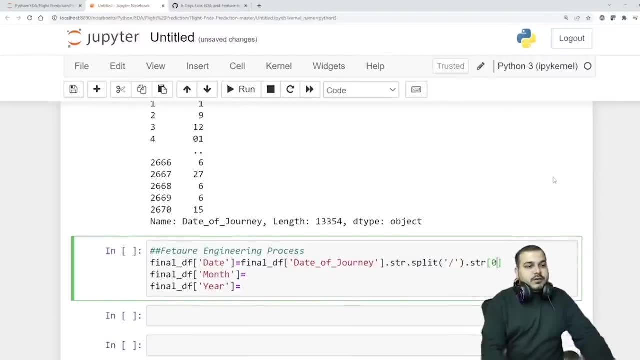 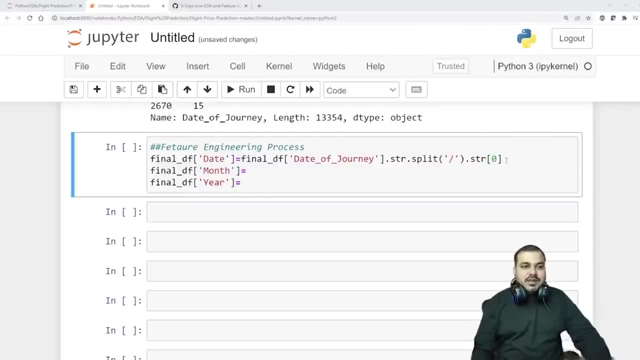 all my dates that i'm actually able to get. so, in order to get the dates, i'm just going to use this and in forward, i'm just going to write dot, str of zero. so this is the. this is the process that we can basically use to take out the date. no need to convert into date or time. also because once we get, 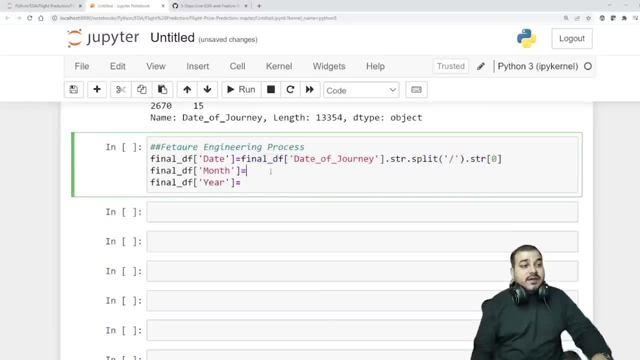 to an integer, then if i'm doing for forecasting kind of task at that point of time, i may use it. then for the month i need to just change the index to one, and for this i need to change the index to two. so here i will be able to get date, month and year. now, if i execute, you will be able to see this. 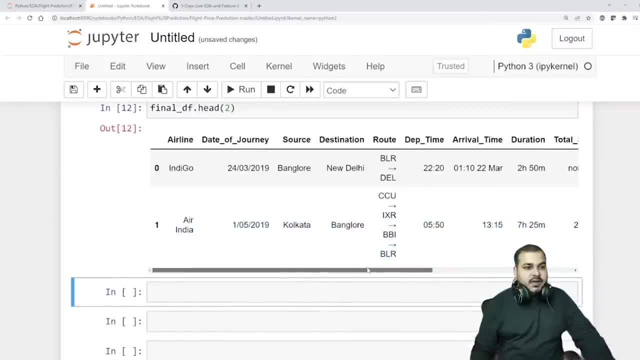 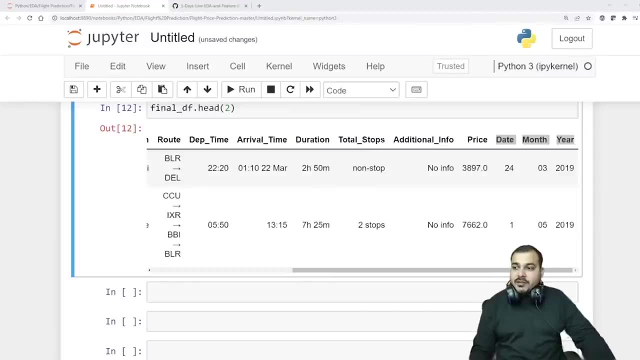 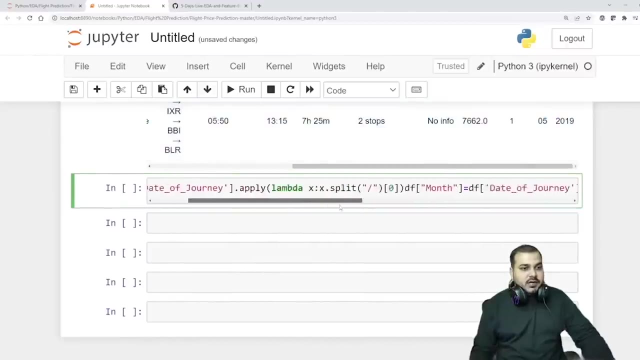 and head. i'll just see the top two records here somewhere at the end you will be able to see date, month and year is created. this also works well. you can apply a lambda function, which is very, very good, so i'm just going to ping or copy paste this code over here. this is also a very good technique. how? 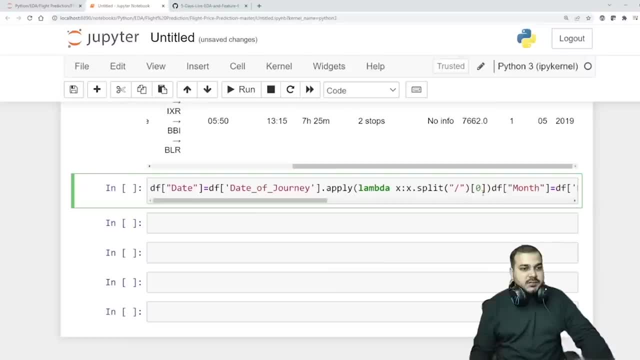 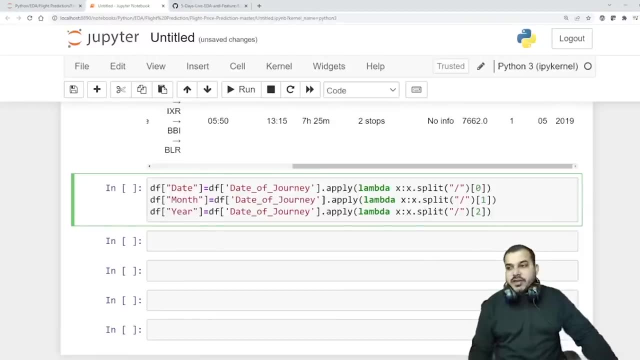 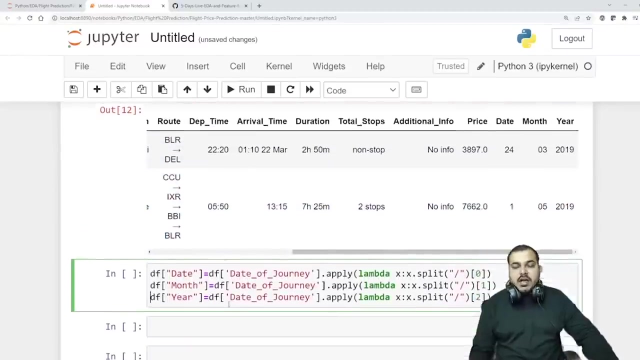 to do it. definitely, you can also do it with using this. so he has given this specific technique where he has specifically used lambda function. this will also definitely work. i hope everybody is able to understand till here. okay, so either of this code you can basically use and you can actually go ahead and do it, but this is a very good technique of applying a lambda. 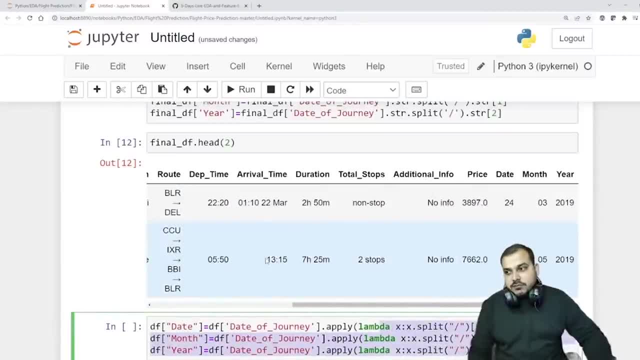 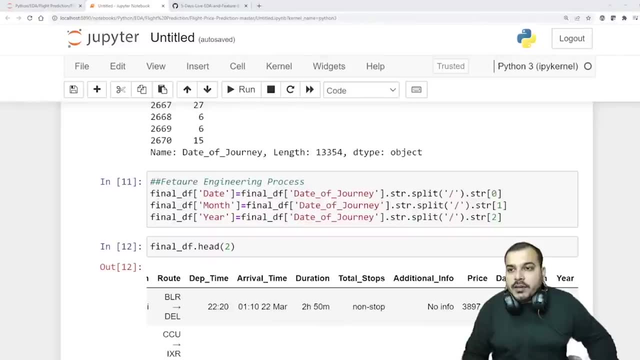 function very nice with efficient coding. okay, it's all about googling and trying to find out a better way. that will definitely work. okay. now let's see in the next step what we have to do. simple, it is that we have to basically also make sure that we convert that into an integer. 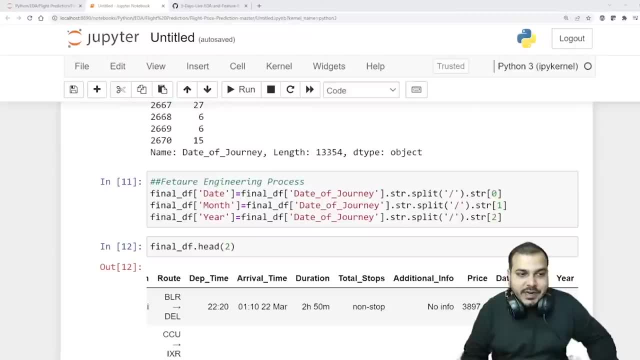 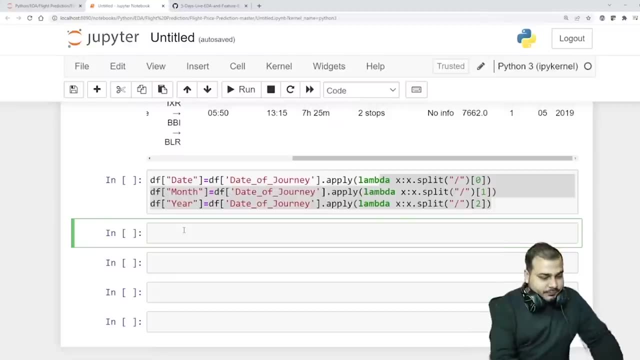 right, so integer also, we need to convert that date, month, date, month and year. so, in order to do this- uh, it's very simple. how do i do it? i will just write final underscore df. okay, is equal to final underscore df of date, and i'm actually going to convert this into as type. 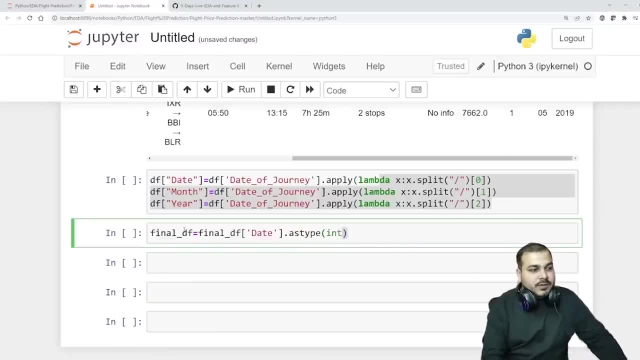 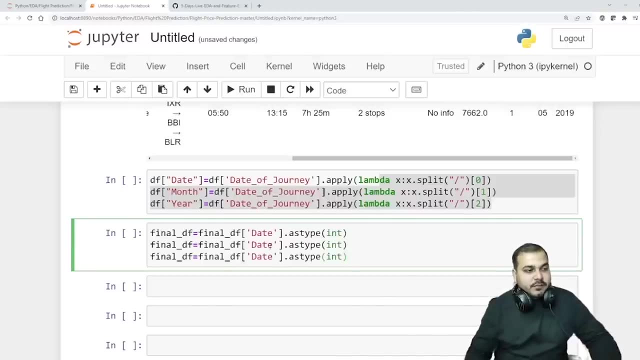 int. okay, then i'll copy this. probably i'll paste it. i'll paste it. i'll do it for month and year. but one mistake i'm definitely making over here: i have to apply this to the same feature, right? so i'm just going to copy this here. 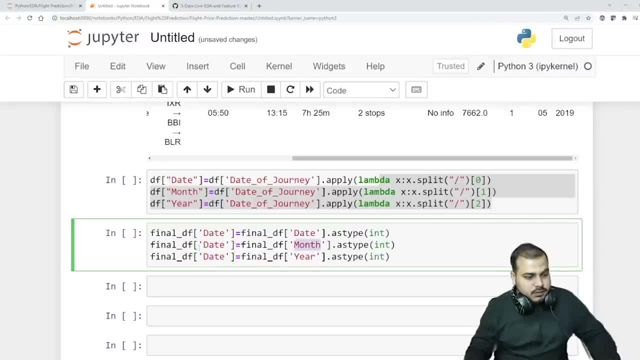 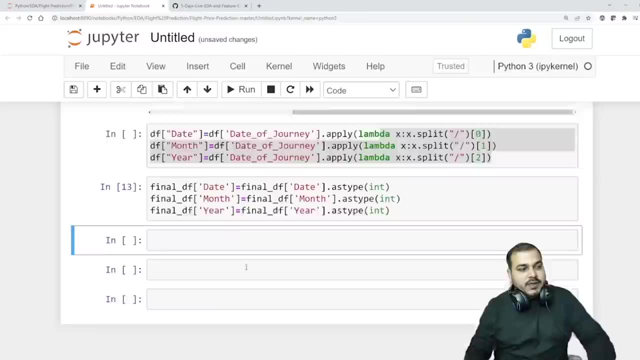 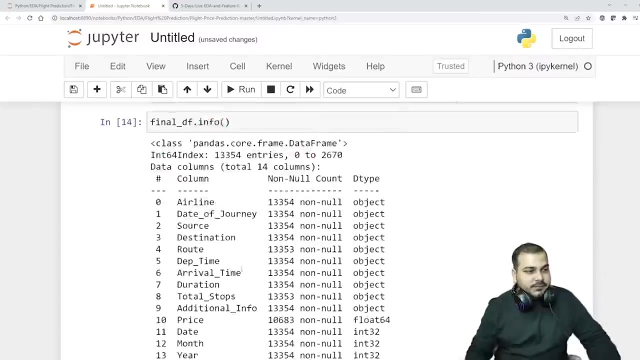 here, here i'll just make this to month and i'll just make this to here. so once we do this and once we execute, this is got executed. now, if i write final underscore dfinfo and if i see so, here you can see date, month and year is now in 32 in 32 – price is: 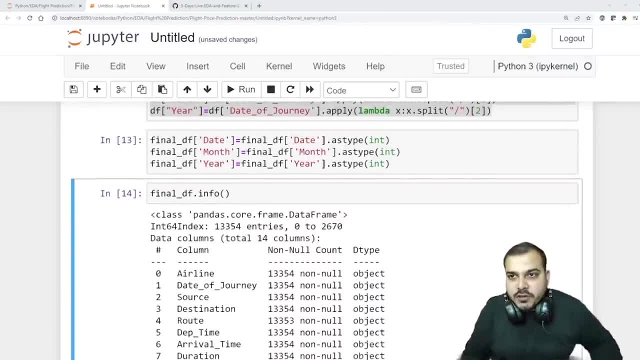 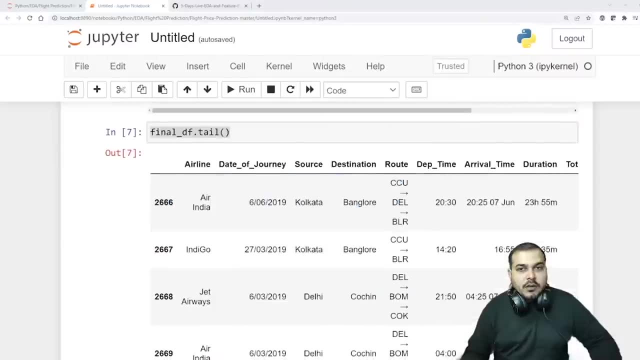 already float 64, but we are starting to focus on different, different features. so, uh, we have done this, so let's go to the next feature now. which one do you want to catch hold of the next feature? which one do you want to catch hold of the next feature? as a case, maybe a? 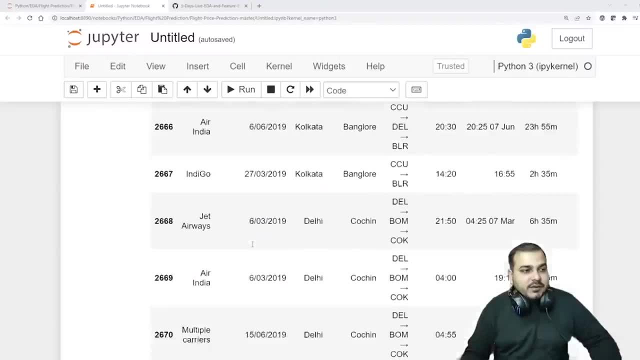 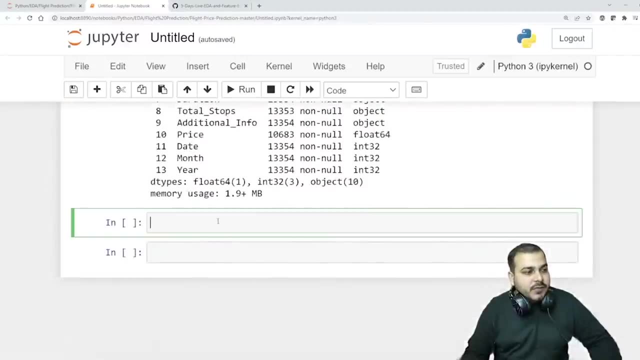 feature. since we have done it, we'll do one more step is that we will try to drop this particular feature now. i don't require date of journey right now, so what i'm actually going to do now i'll just write final underscore df, dot, drop, and here i'm basically going to give my feature name. 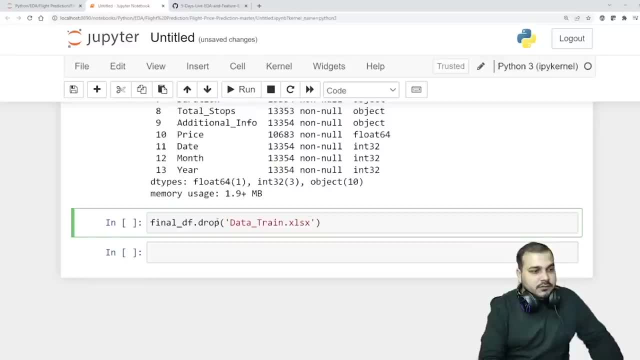 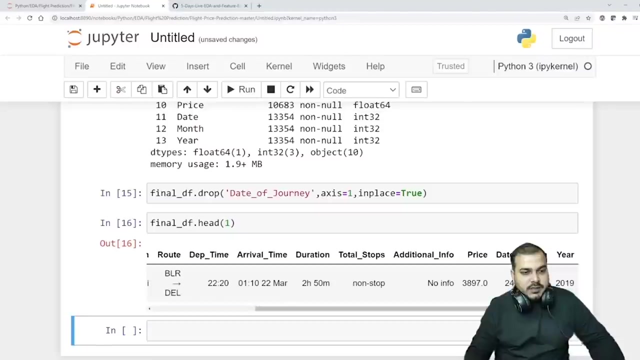 which is date of. i'll just copy this: date of journey with x is equal to one in place is equal to true. this we have already seen yesterday. now, if i go and probably see my final underscore, df dot, head of one, and then here you can see, month and year are there, date is also there. 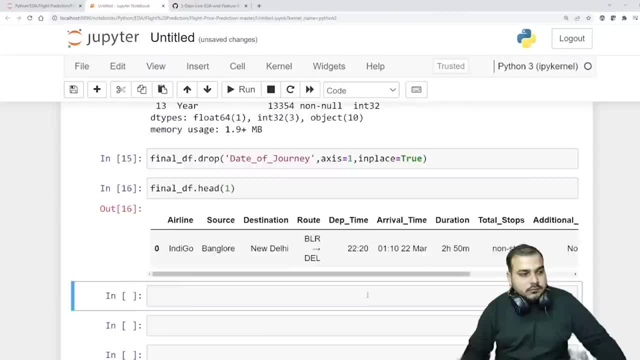 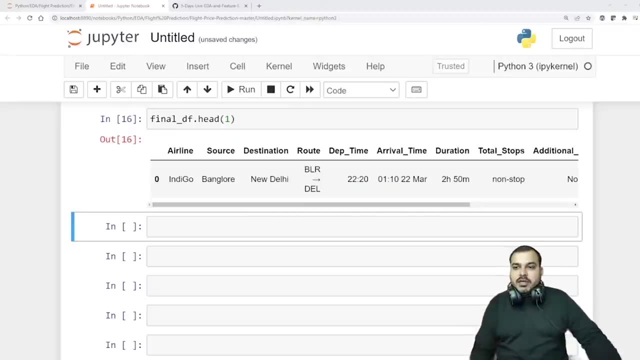 but you don't have any date of journey. now let's go to the next feature. next feature. see, this is how we have to catch one feature at a time and probably do the necessary changes. okay, so the next feature. basically, we will go with respect to route. 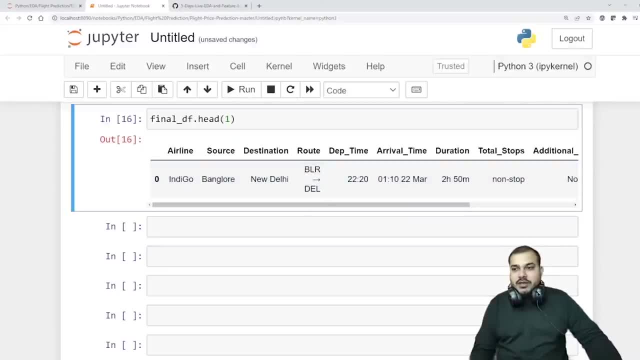 let's say what we can do for this route. also, we'll try to understand: okay, arrival time route, okay, route, let's wait for some time for route. let's focus on the arrival time or departure time, okay. so let's do one thing. let's focus on arrival or departure time first. we'll focus on something and then 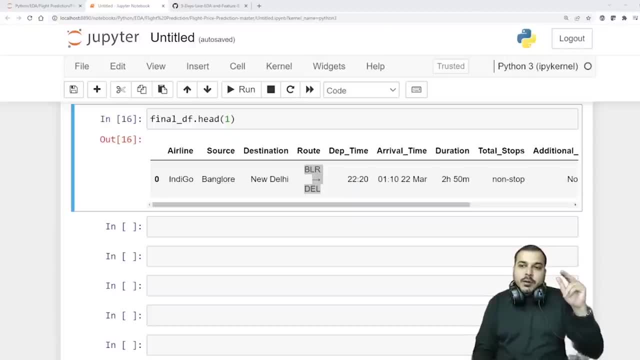 a similar type of fields. always remember when you are probably doing feature engineering, try to catch up similar types of field, which we basically have to do again and again. let's go ahead and take up arrival time now. from this arrival time, what you can do is that obviously you don't require this information, like 22 march, if i probably go and see around. 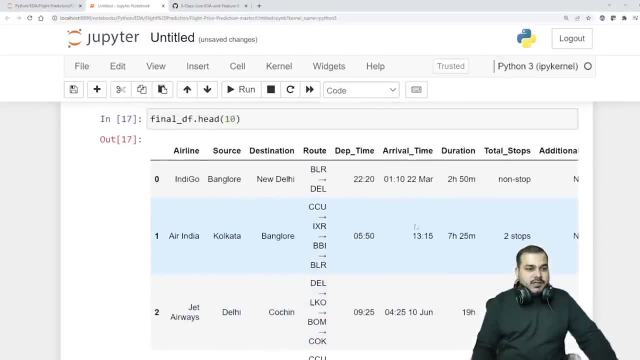 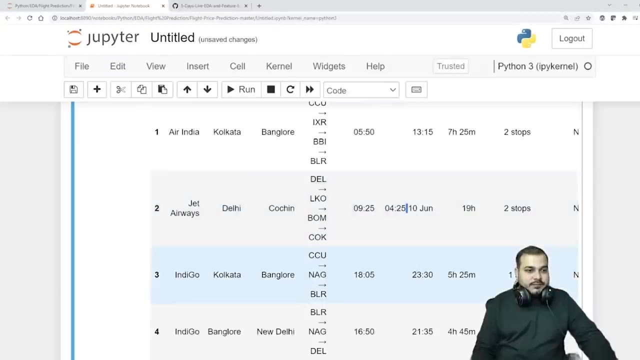 10 records. so here you'll be able to see that wherever there is this gap, this space, how we can split it. let's see if we are using some space over here, we can definitely get something. okay, if you are using this space and probably trying to split it, i will probably. 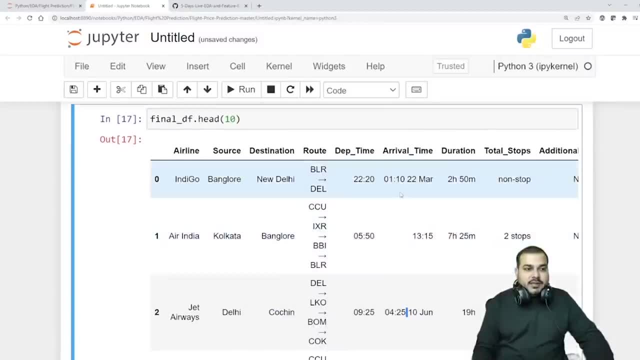 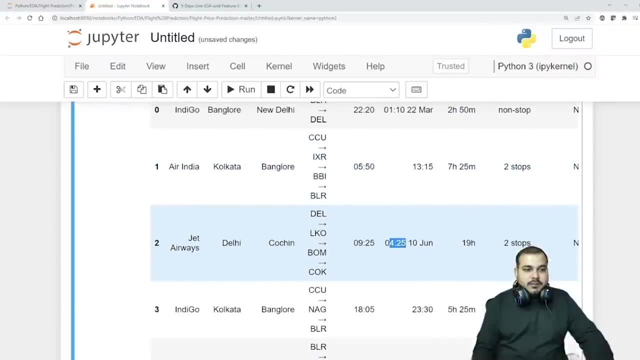 be able to get the arrival time. my arrival time should be in such a way that i should be only able to get this first four important information. think over it, because i don't require this 10 june and all because there is date for that. i don't require that, i need. 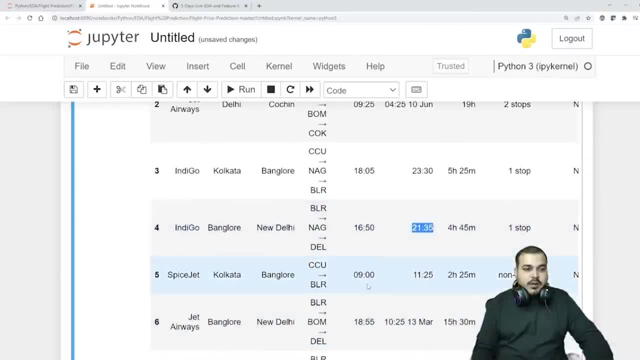 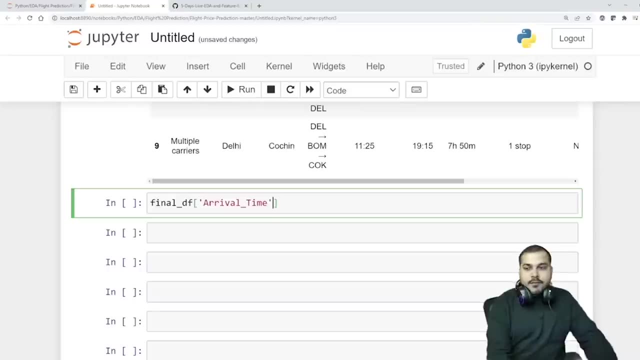 to focus only on this first four values. so how do i do it? so i will write final underscore df of arrival time: dot, htr, dot split. if i split with the help of an empty braces and if i write dot, htr, dot split, i will be able to get the arrival time of the arrival time. 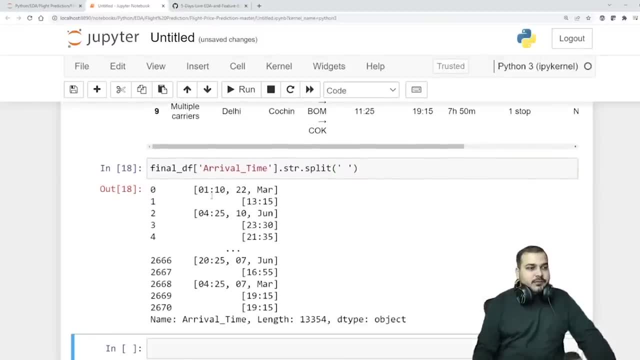 or if i just execute this here, you will be able to see like this: right, so out of all these things, i just need to pick up the first value. see, in the first value i will be able to get all the important information. okay, like 425 715, only the first one i need to. 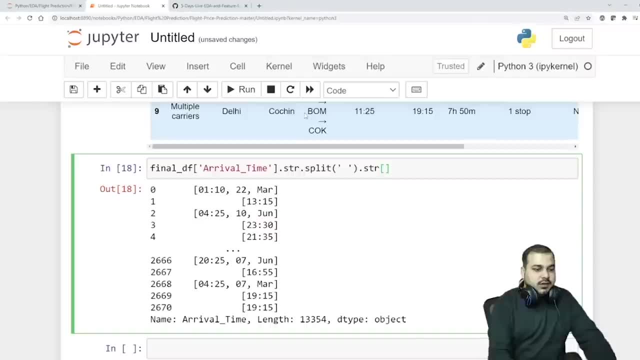 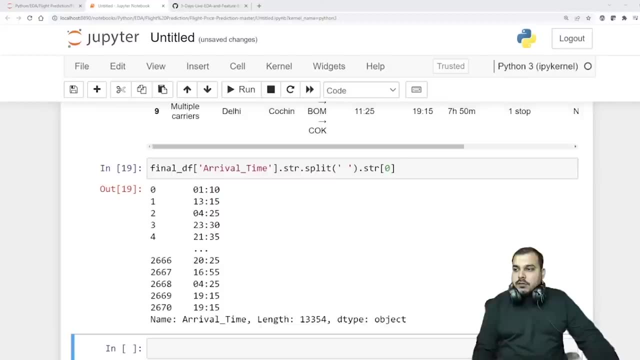 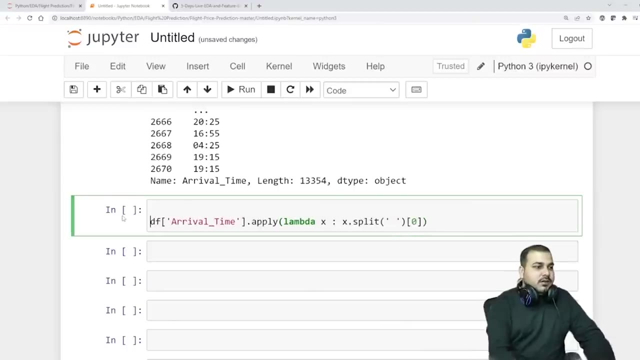 focus on. so to get the first one, i will just use indexing of htr of 0, and if i execute this now, i will be able to get this particular value. to do the same thing, there is also one amazing code which can be done using this lambda function. so here you can see dot apply. 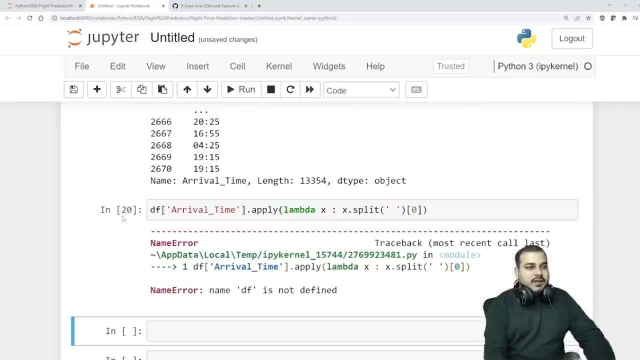 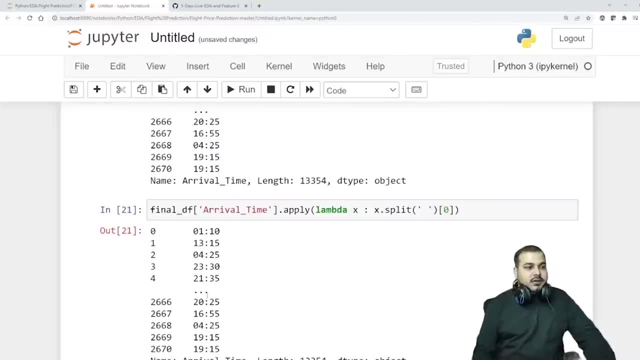 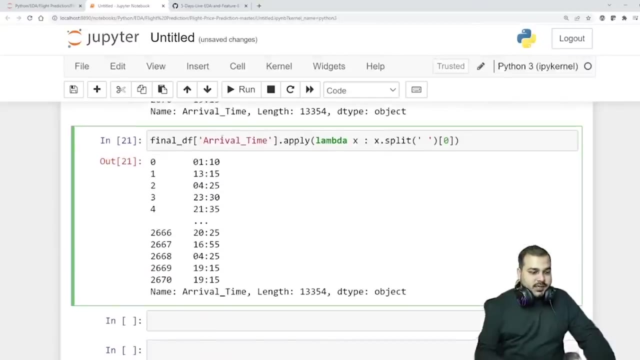 lambda, this, this, this, this. okay, if i execute it, sorry, final underscore df and execute it here, you can also see that i am getting the same information. so what i am actually going to do, i am going to use this particular code and make that changes in final underscore. 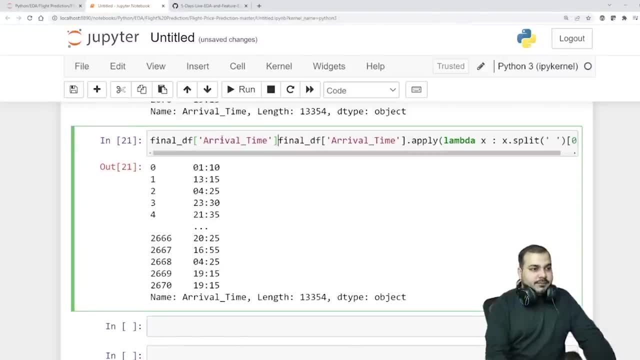 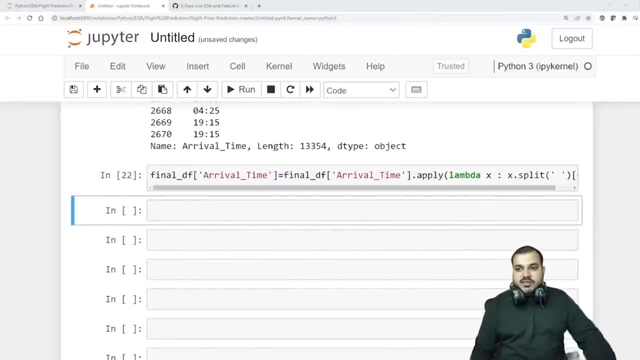 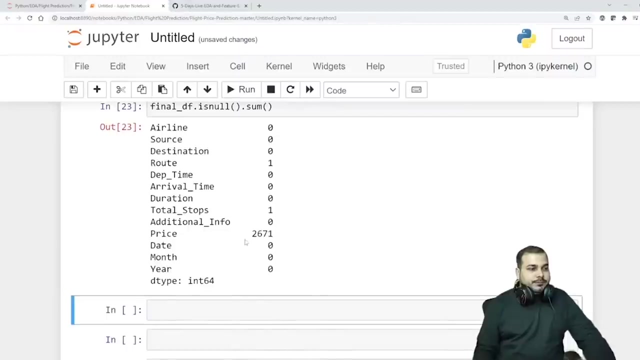 df of arrival time. any one of the code you can basically use and you can do it more, new, new things. you can basically get it in order to do it. one thing that i forgot to check: whether it has null value or not. so price basically has null values. it's okay, that is for the test. data route has one null. 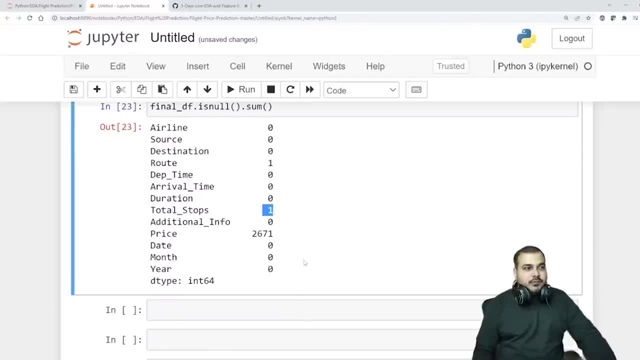 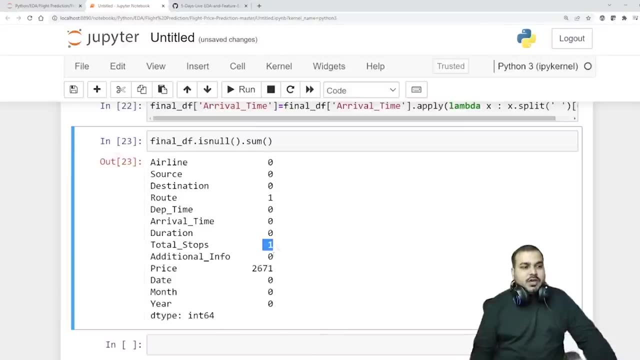 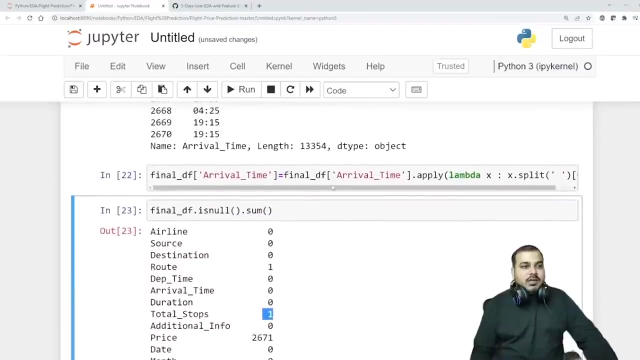 value. total stops has one null value. route. that basically means route in that specific it may be the same row, it may be the other row, but total stops has one null value and this has one null value. everybody clear now from this arrival time: we still have to take out the hour and we still have to take. 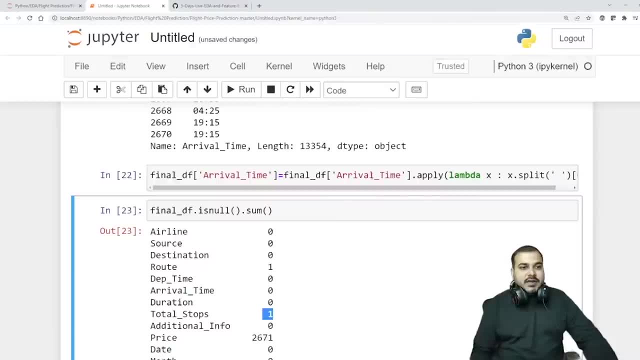 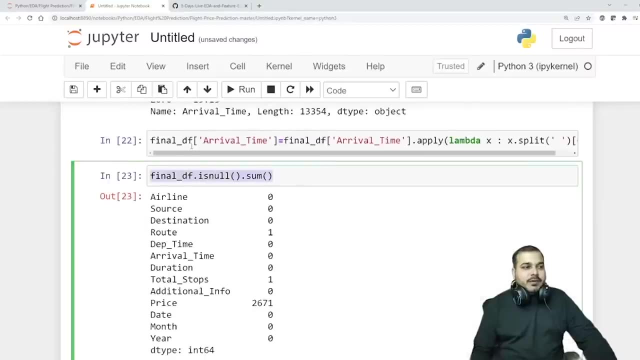 out the what we need to take out from this arrival time: guys, hour and minutes. right, so that specific thing i will do. next step: so here i'm actually going to write final underscore df with the same lambda function or in. in a easy way you can basically do the split, and here i will actually. 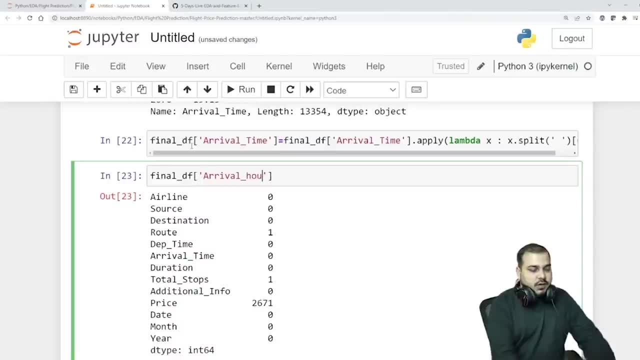 create two more features. arrival underscore hour is equal to final underscore df, arrival underscore time. then you can use dot, apply lambda, or you can also do dot htr, dot split, and this split will now happen with colon right, because within the hours and this one colon is there. 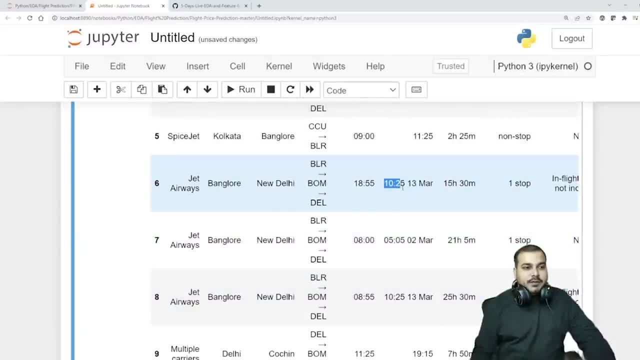 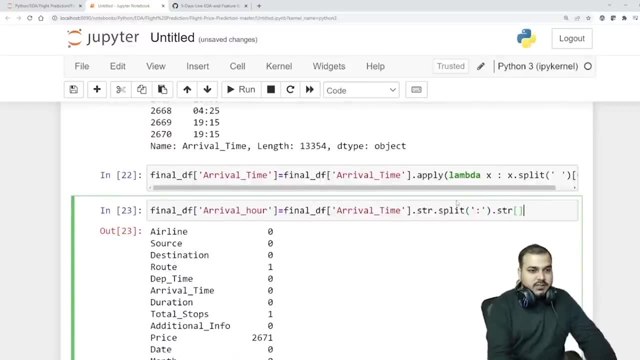 so i'm going to split with the help of colon, right? so when i split with the help of colon, it will be dot, htr, dot, split, dot, htr of zero. if i write like this, it will become my hour. and similarly, if i want to know the arrival minutes, then i can basically write like this, and here i will just 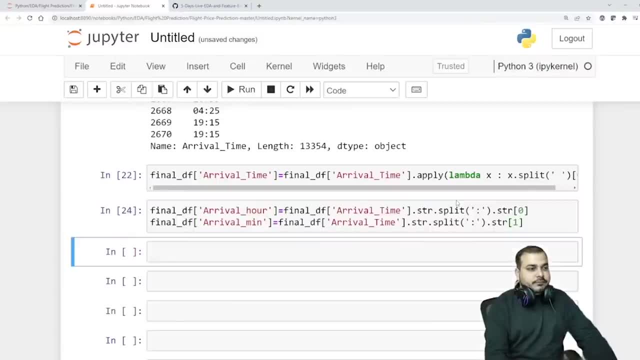 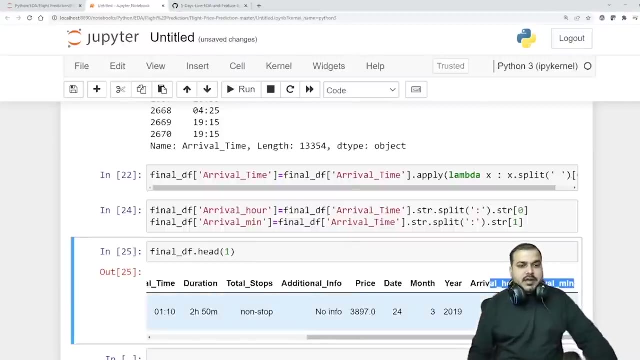 write htr of one done and if i go and probably see now final underscore, df dot head of one, you will be able to see this one and here you have arrival of hour and minute. remember this is still in object type, so i also need to convert this into an integer type. so same. 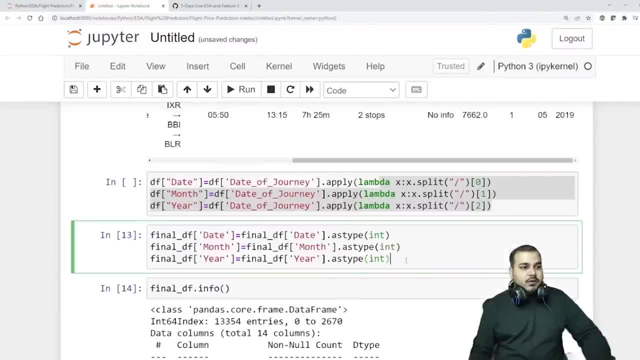 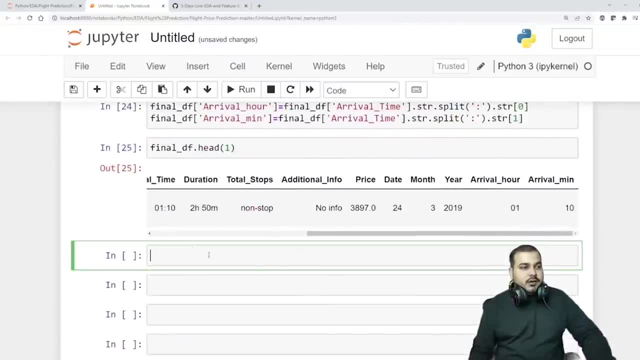 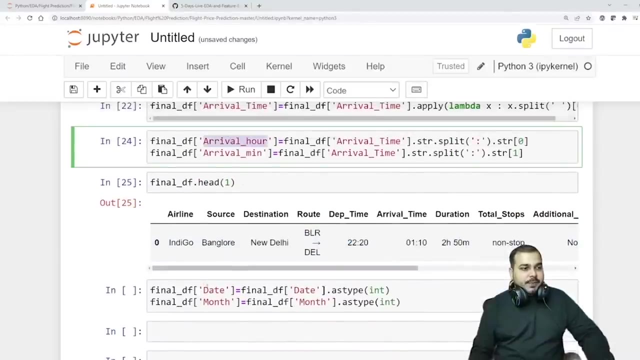 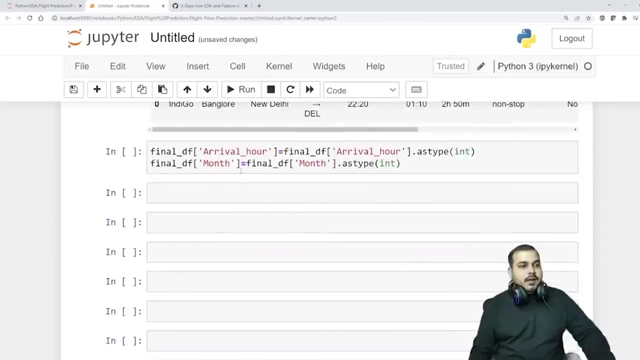 thing. if i go up, i had written that specific code how to do it. i'll just copy this one like this: okay, i will copy the code over here and keep it over here. and here i'm going to basically write arrival of hour and convert this into int type and arrival minute and convert this into in type. 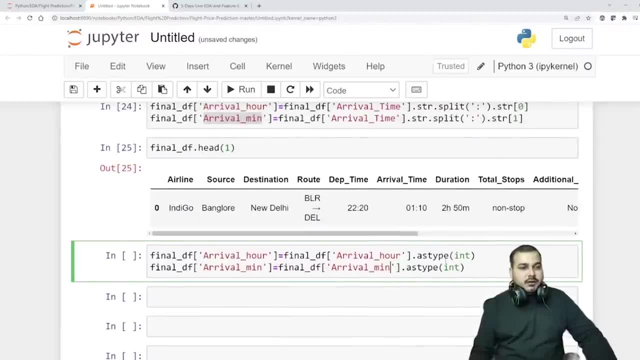 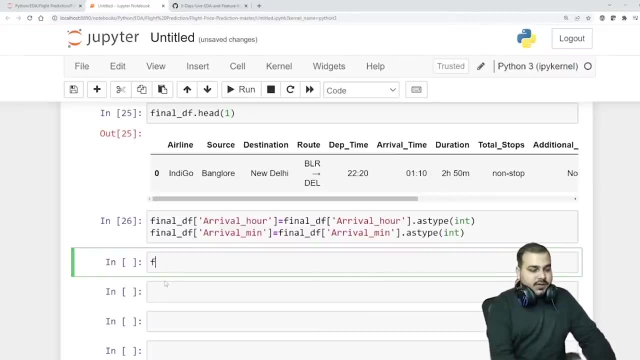 so two steps. one is converting into in type is also done over here along with this. so if i execute it, you will be able to now see that, since i've converted this into an int type. and the second step: if I write final underscore df dot info, now you will be able to see that there are integer values. 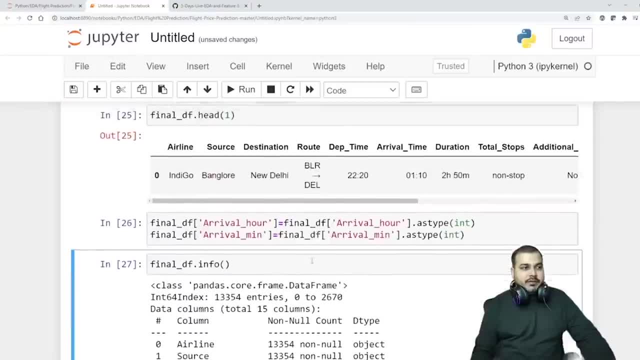 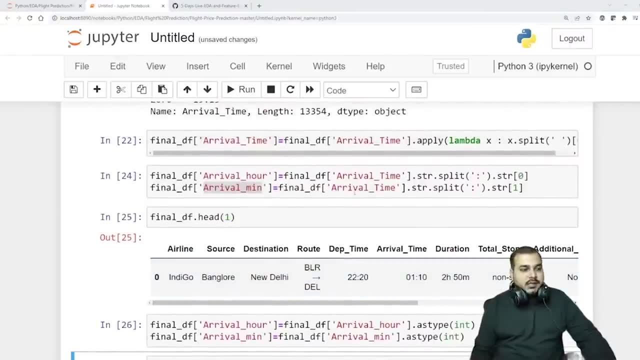 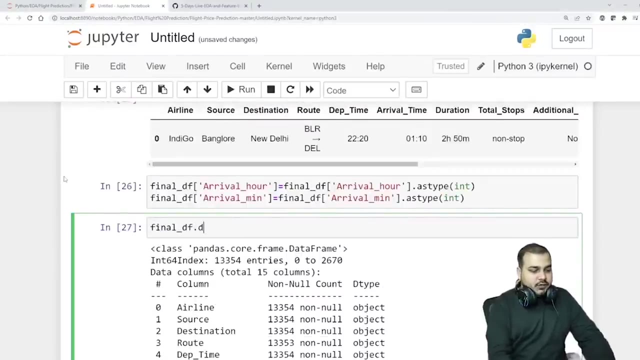 added in arrival hour and arrival minutes. So this is the code that I have actually written and then after that you can drop the arrival time. So here I will write: final underscore: df. dot. drop arrival time. arrival underscore time. comma axis is equal to 1, in place is equal to 2.. 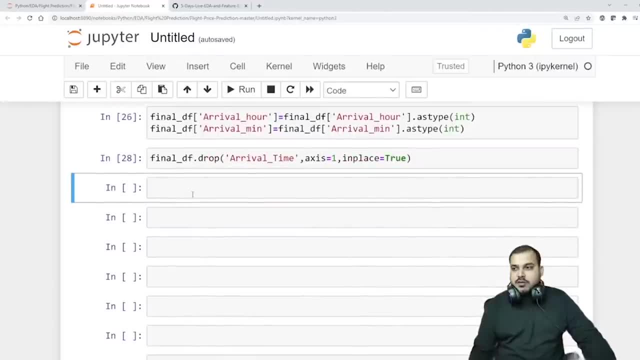 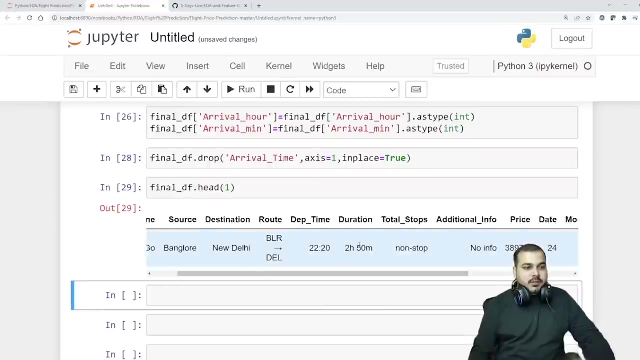 Step by step. we are doing it in a nice way, So I hope everybody is able to see. So now, if I probably go and see my final underscore, df dot head of one record here, you will be able to see. these things are also there. Okay, what about departure time? 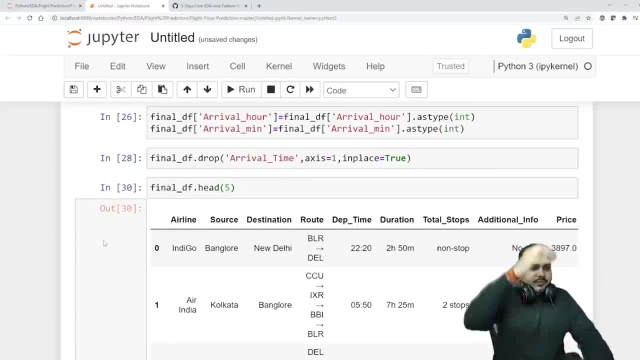 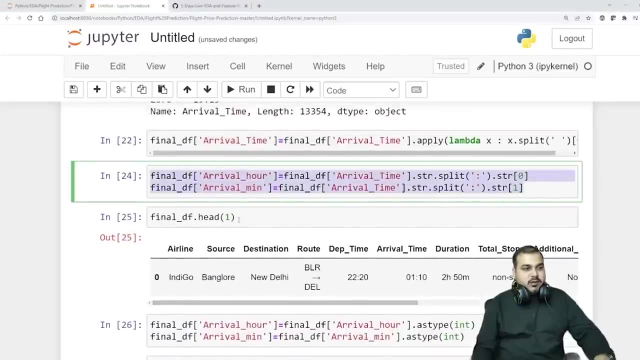 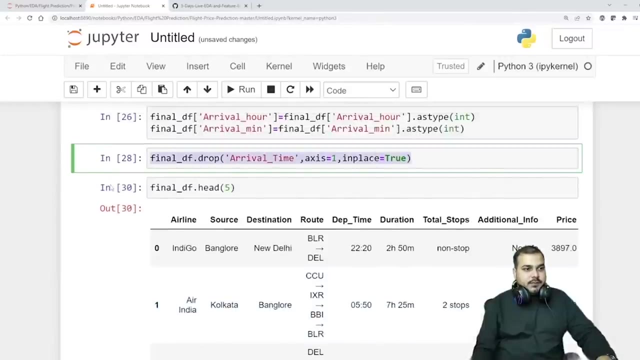 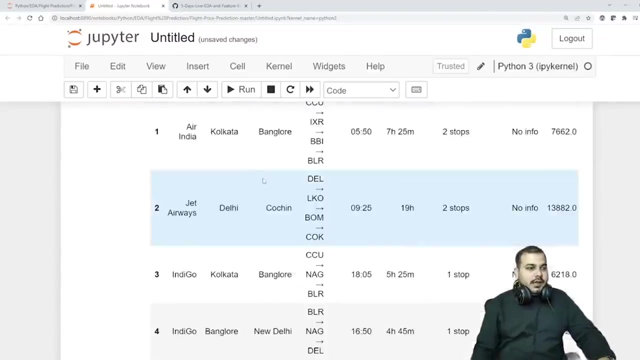 I hope everybody will be able to do the same thing for the departure time. Just do it because departure is also having the same format. So I am just going to copy all the code, paste it over here, paste this Also over here now, paste this two line also over here and finally, paste this also over here and keep. 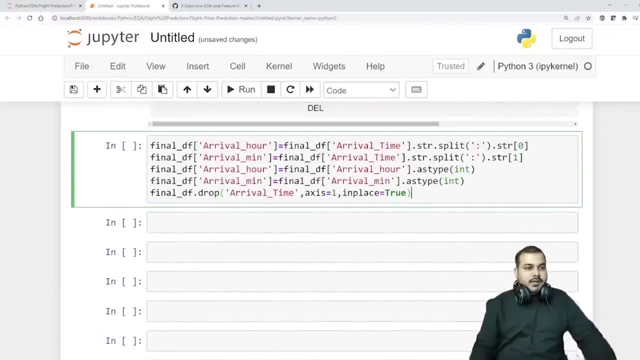 it with respect to arrival time, like that. we had departure time right, So I am going to write departure time right, Depth time. I am going to copy this everywhere, Paste, paste, paste, paste. And here I am going basically write Depth hour, Depth minutes. 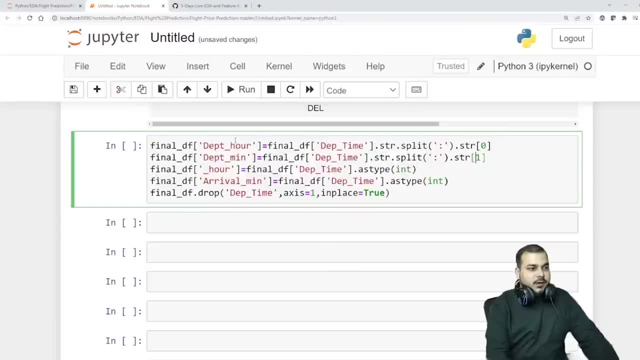 This. I don't require Depth hour And this will be my DEPT minute, So just by doing this, I think everybody will be able to understand that we are going to change it now. Yes, that will also work, Anirudh. 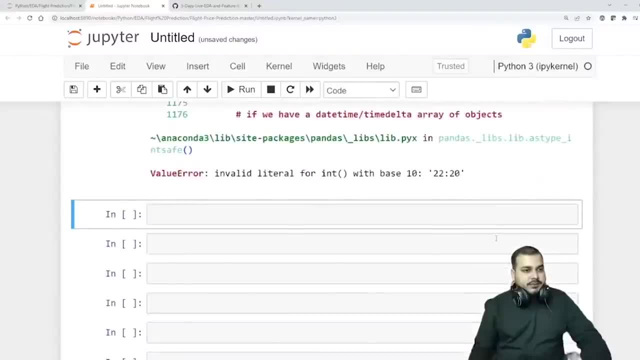 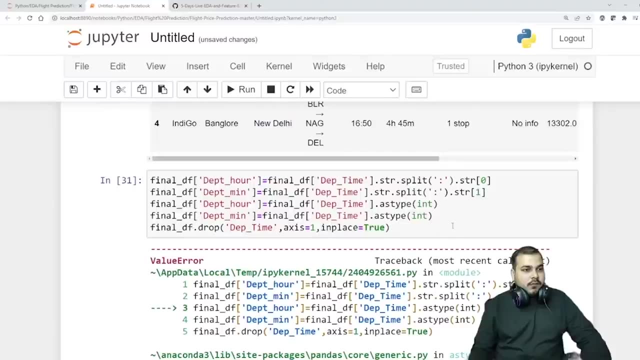 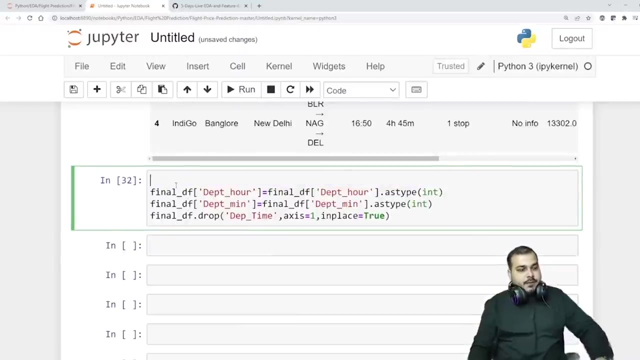 Done. Oh, error is coming. let's see With base 10, 20 to 10.. Oops, this should be department of hour and department of mean, So I don't have to execute this again. So I will just remove this, paste it away. 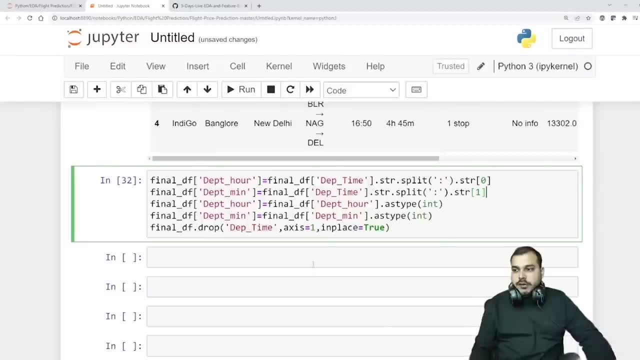 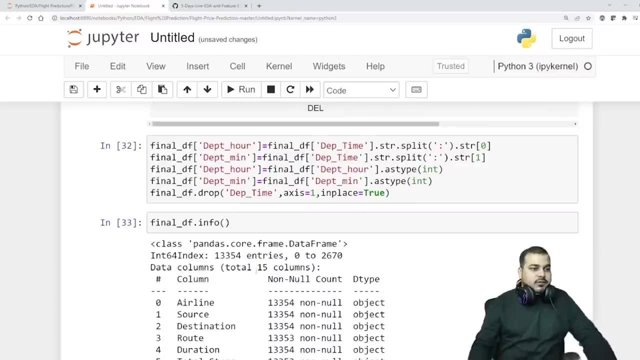 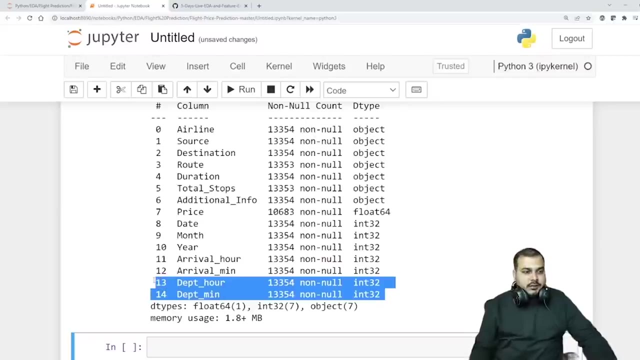 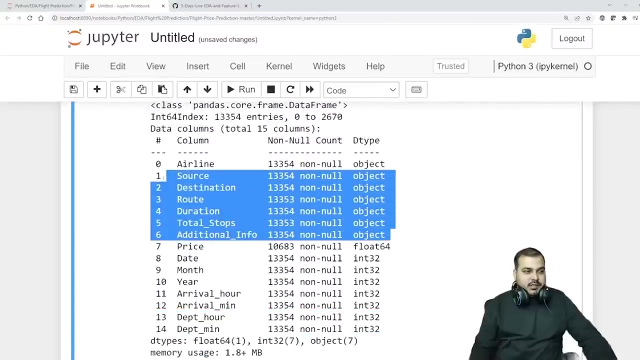 Well done. So it's final underscore df. Now you will be able to see two more features getting added, and it will be department of hour and this one. both will be there. Perfect, we have done this. Now we have to take care of all these other things, right. 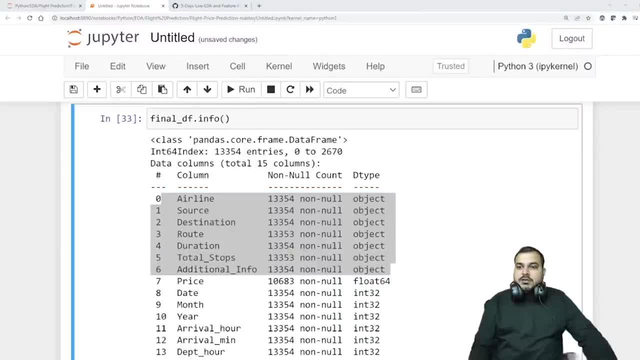 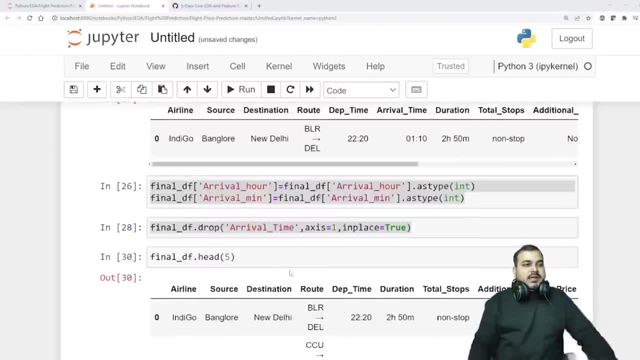 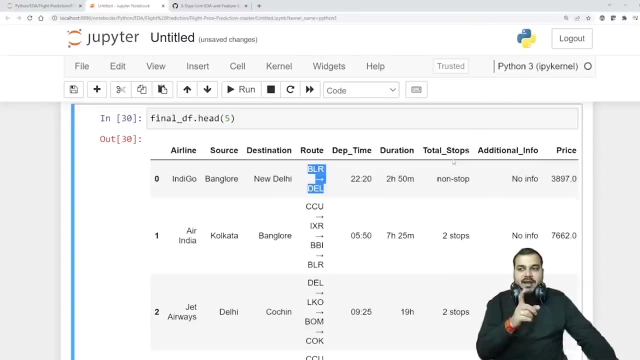 Airline and all are actually there. So departure is done. Now let's catch up route. Now, inside this you will be able to see, Route is basically having this information, like: Bangalore to Delhi, Bangalore to Delhi. okay. 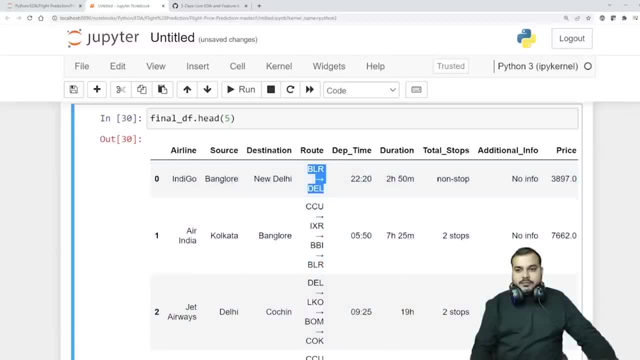 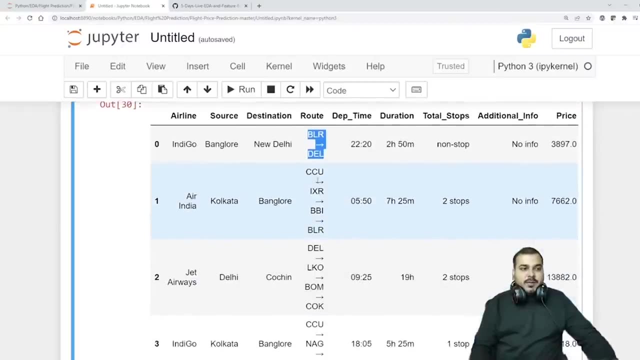 See, anyhow over here you will be able to see that, even though I basically find out, like what is the route? like route 1, 2, 3, 4.. Maximum to maximum over here you can see that there are two places. like Bangalore is the origin, Delhi is the destination. 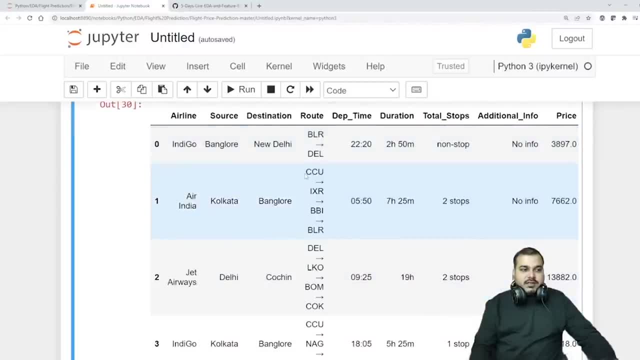 Here you have four different different places. That basically means first year. So you are going from Kolkata to IXR, then IXR to BBI, then BBI to Bangalore. So total number of stops: you have two over here. 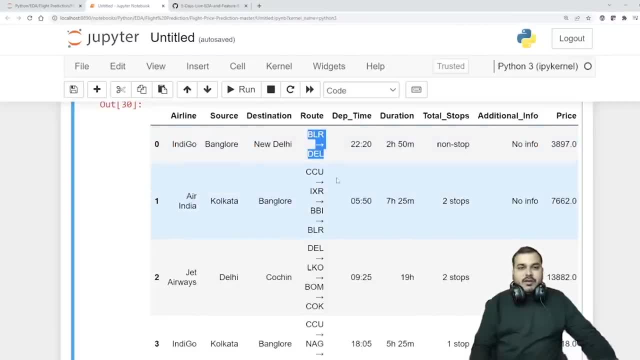 In this particular case, you just have one stop. So what we will do is that we will try to capture the route 1, route 2, all the places over here, Over here in the source and destination. you just have two values, right. 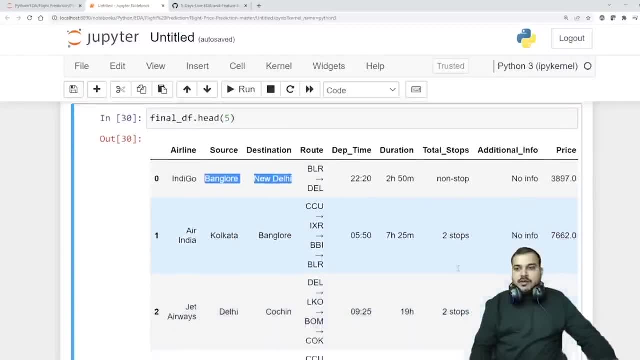 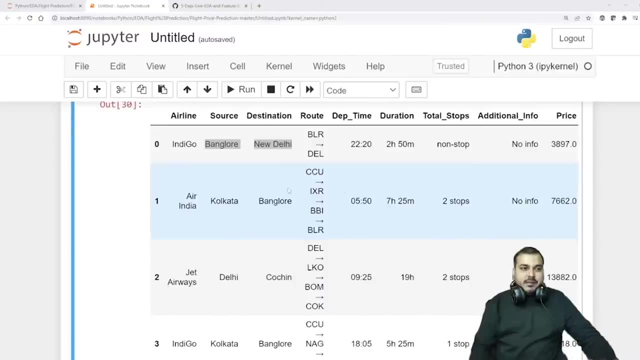 Number of stops. you have 2, 1, like that. you have right. So it is better that we get this specific information very much clearly so that We actually be able to see route 1,, route 2,, route 3,, route 4, like that right. 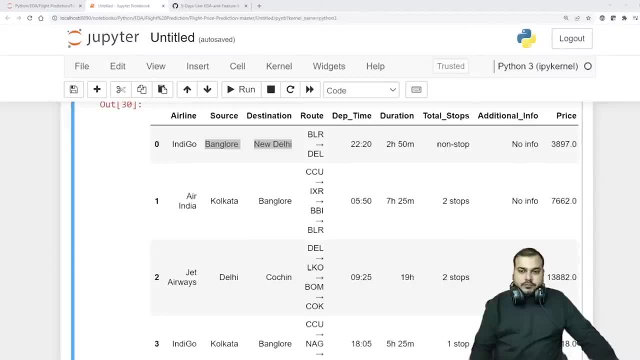 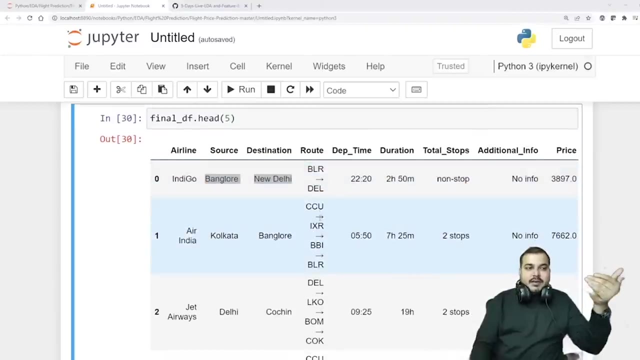 So one thing that you need to know over here is that you may definitely get null values. You may definitely get null values, a lot of null values you may be getting, But understand, null values will be there. for, like, if I want to capture for route 4, definitely null values will be there, okay. 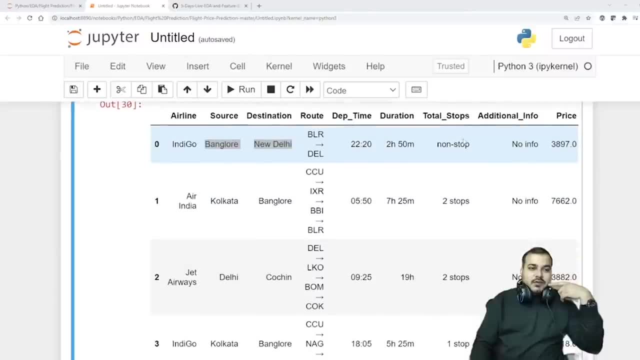 Instead of this also what we can do. we can also delete this And we can just focus On this total number of stops- right, Total stops, like total underscore stops. We can also focus on this particular values also. So what do you think should we do? 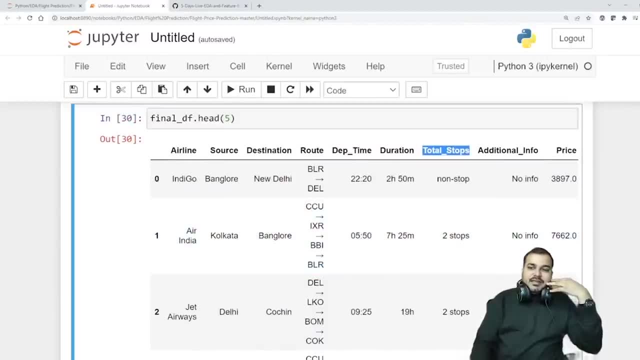 Should we delete this specific feature directly and just focus on, because we have the source and the destination and obviously we have number of stops. But I just think, like as a person, right, We nearly need to focus on two things, okay. First of all, is that, if probably I'm going from 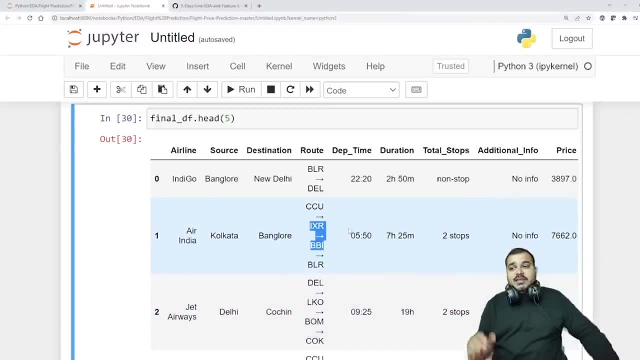 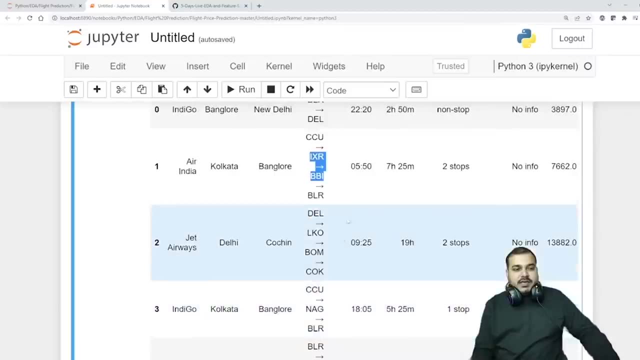 Kolkata to Bangalore and these two places are going, then the price may increase drastically. okay, Just not based on the top of the number of stops. Now, in this particular case, you can see from Delhi to COK. right Here you have Lucknow and Bombay. 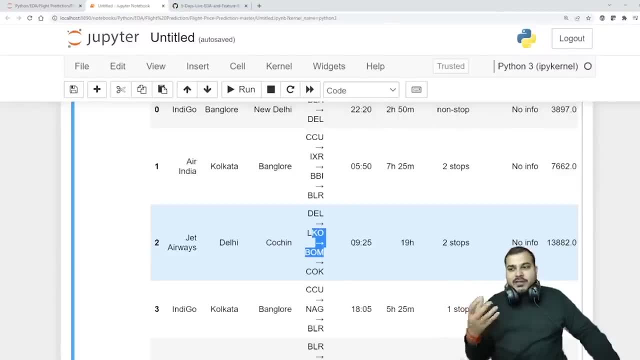 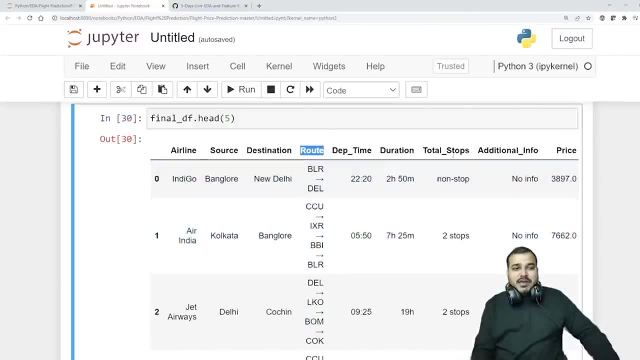 Lucknow and Bombay. you feel that probably more price will be taken place over there. So just see what you need to do. We can definitely drop this route. We can just focus on total stops. But before focusing on total stops, What? 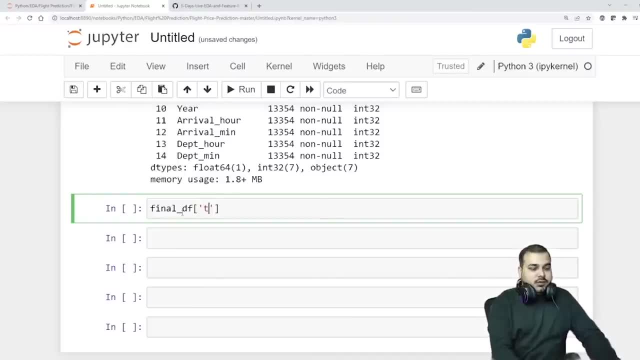 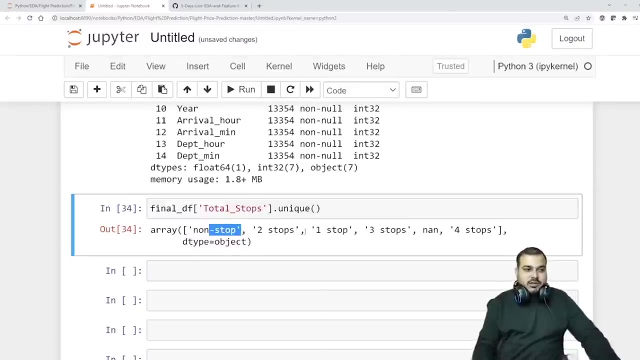 I'm actually Going to write. I'm going to basically say final underscore: dot total. total stops, dot. unique. if I write unique, let's see how many total stops are there. So here you have non stops. non stop basically means probably it's like just a single stop here. 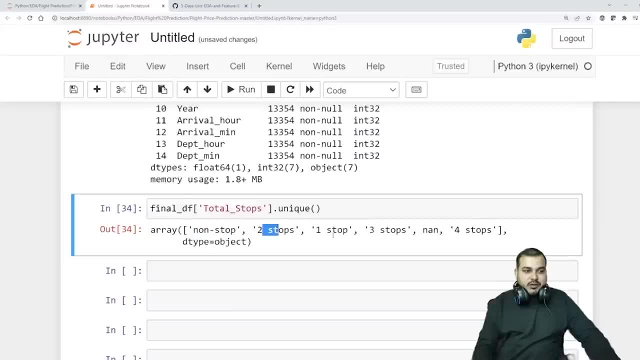 You can see, here You can basically replace this with zero, here You can replace with two, here You can replace with one Three. this nan value- If I try to see that there is one nan value, I guess- is null dot sum. 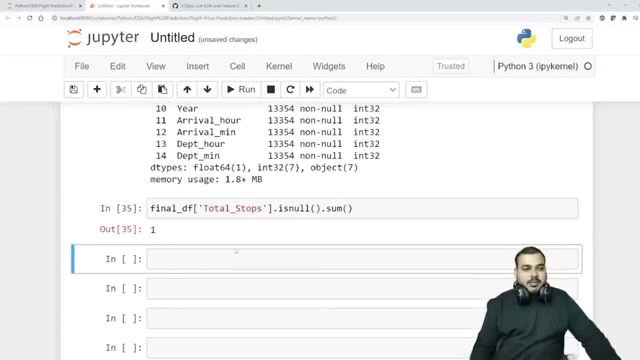 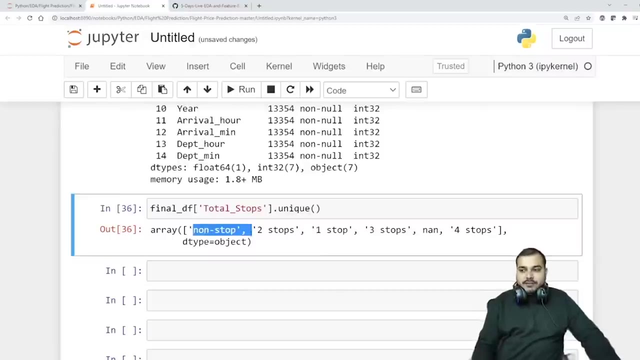 So here you can see one nan value. You can replace it. Uh, which one is required with respect to that? Okay, So, everybody focus on doing what we'll try to convert this into and map this values with zero, one, two, three, four, five, like that. 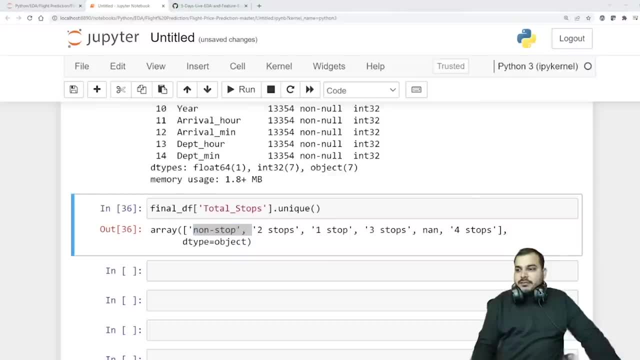 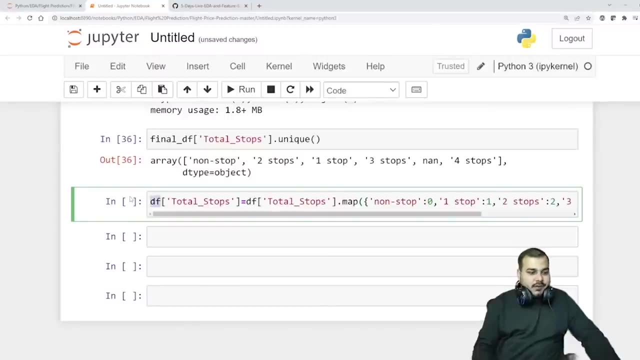 Tell me someone, tell me the code, Amazing. So Rishi has already written the code, So Rishi has basically said something like this by using the map. So here is my final underscore DF, final underscore DF. So final underscore DF: total stops: total stops on map: nonstop is equal to zero. 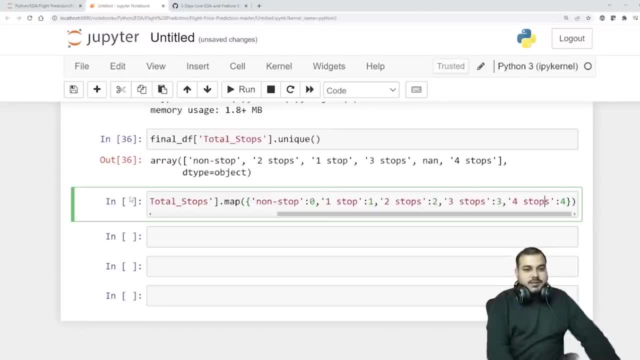 One stop is equal to one. Two stops is equal to two. Three is this for nan Also. if you want to place, place it out, Because there is only one nan value. So for nan also, I will make sure that I can directly see right. which is that specific record. 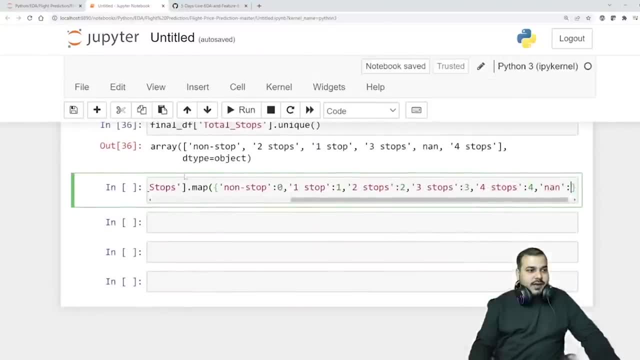 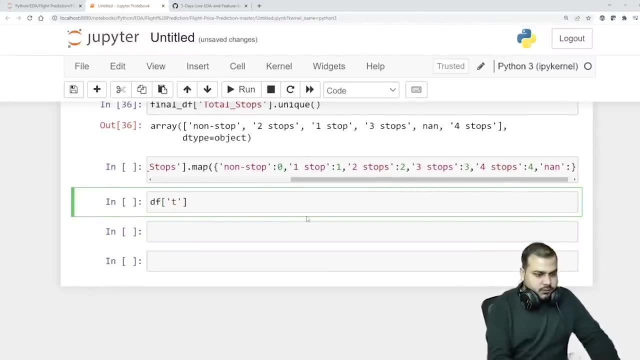 Wait, I can definitely see. which is that specific record for nan. Just a second DF of total. sorry, Final underscore: DF. Total stops dot. um, what i can do is that dot is null, dot is null, and here i can basically write final underscore. 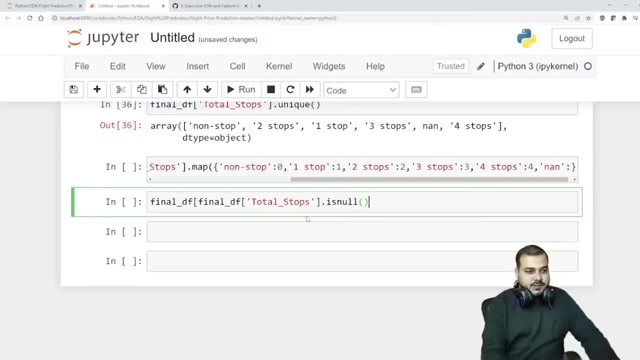 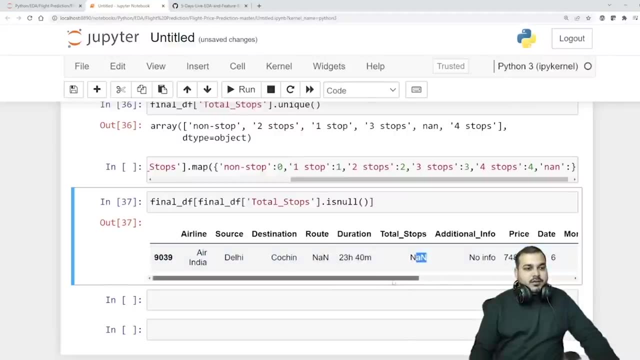 df and i'll try to take out this: specific values. so here you can see, route is nan, but the total number of stops is also nan. so total number of stops is also nan, route is also nan. so here you can see, from delhi to cochin. okay, delhi to cochin? i don't think so there will be a direct flight. 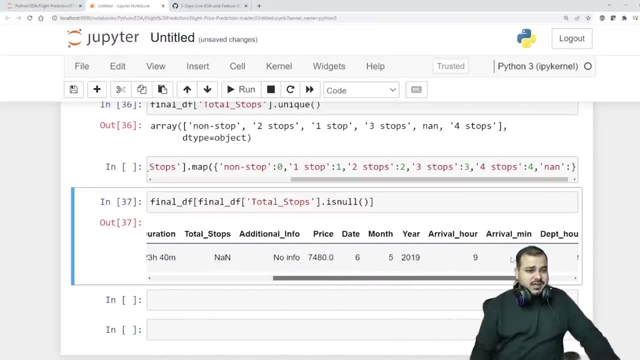 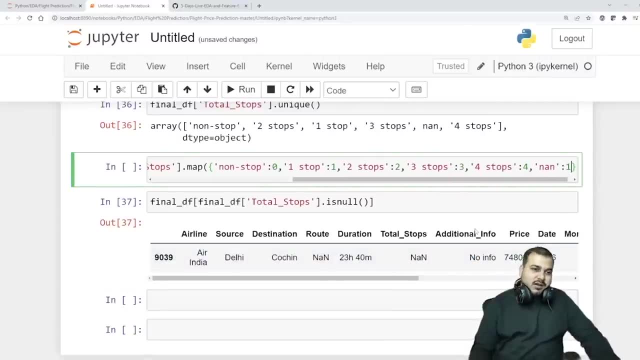 but which value do you want to replace with? since it is just a single record, i think it won't matter that much. so let me do one thing. let me just replace it with one stop, or just common sense, i think for cochin bangalore to cochin, at least one stop is required. so like 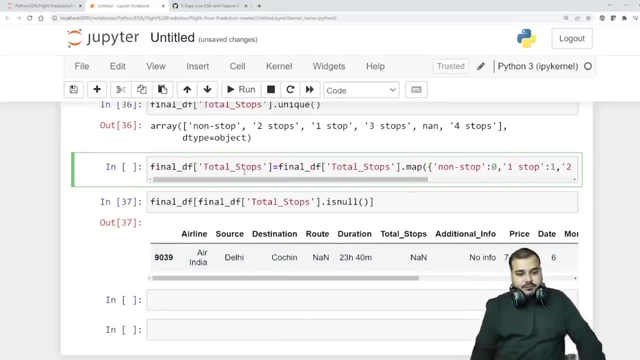 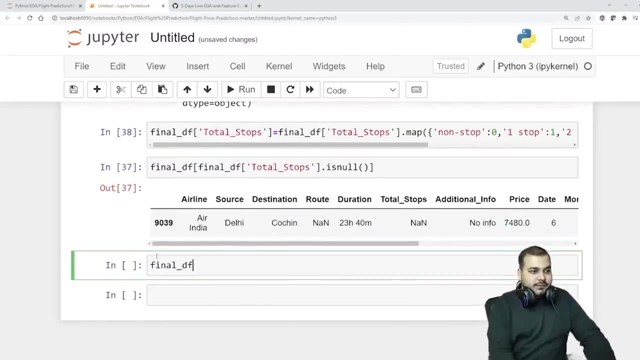 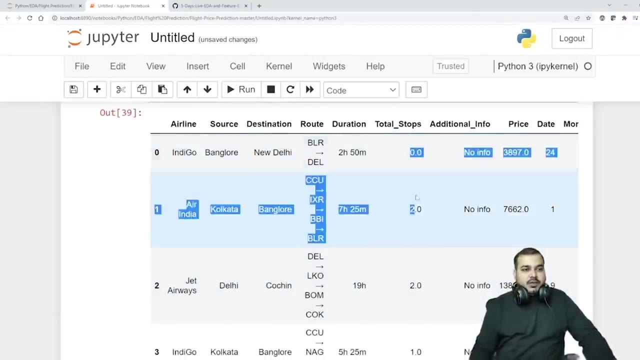 this. i will just try to change it: delhi to coaching. sorry, so i've got executed now. okay, and now, if i go and probably see my final underscore, df dot head, you will be able to see the specific values and here you can see: total stops has been converted into integer floating value. 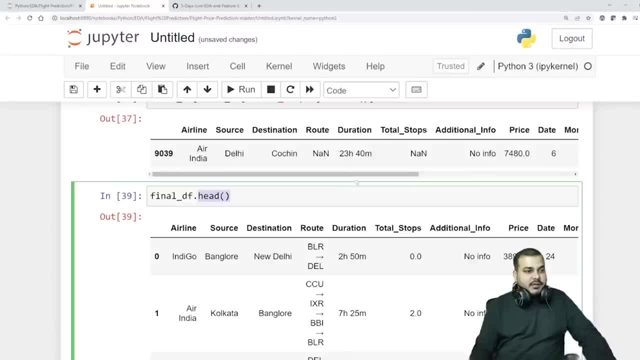 now we can drop this route column. so final underscore df- drop route. um, i'm going to drop route from axis is equal to 1 and in place is equal to true, because i don't definitely require to to information right. so finally, you can see final underscore df dot head. 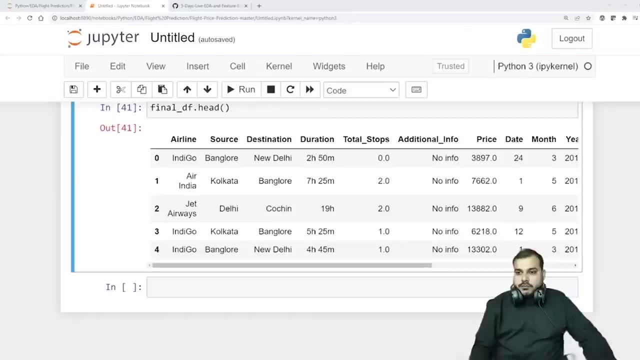 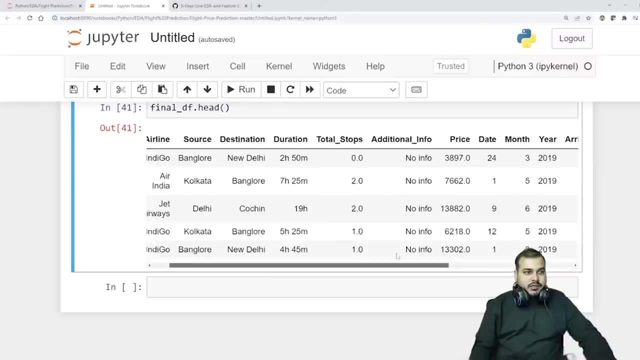 here you have all the values- amazing. now what is the next thing that you should probably want to do? guys, i've deleted everything, right, so we have department department departure hour also. we have dropped total stops is also there. let's catch up. any other one you want to do? 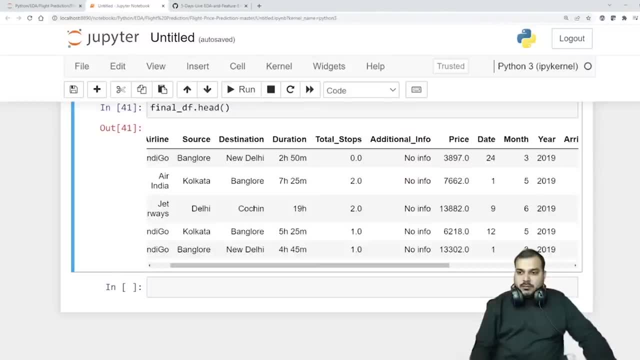 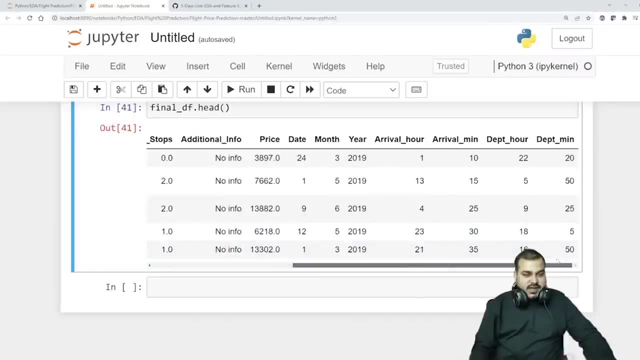 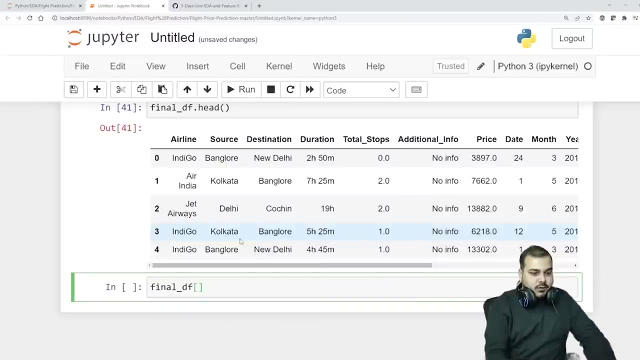 additional info that all will be our normal uh feature engineering, like transformation encodation. we can do any special character if you, if it is there somewhere, probably we have to catch hold of that. so if i write final underscore df and if i go ahead with additional info, additional info dot. 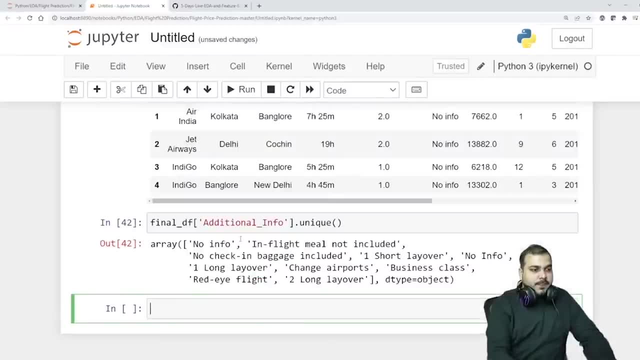 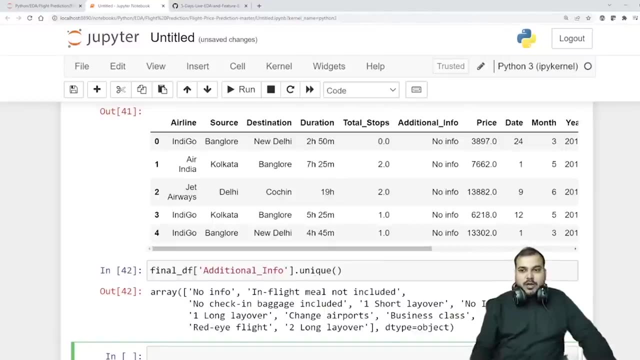 unique. how many unique values are there? so here you can see this many unique values are there. this can be converted into uh one hot encoded format, because there are, say, less number of records. let me just check more anything that we can do with this data set. anyone who wants to do some more things, who? 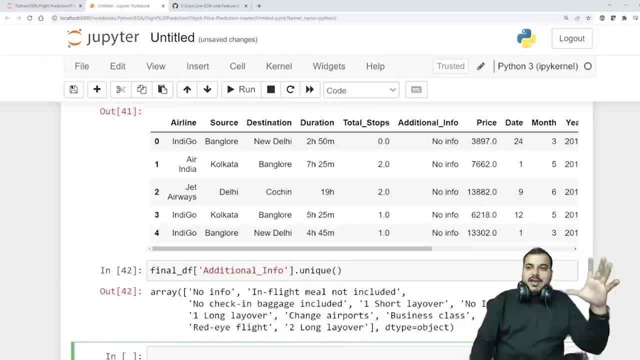 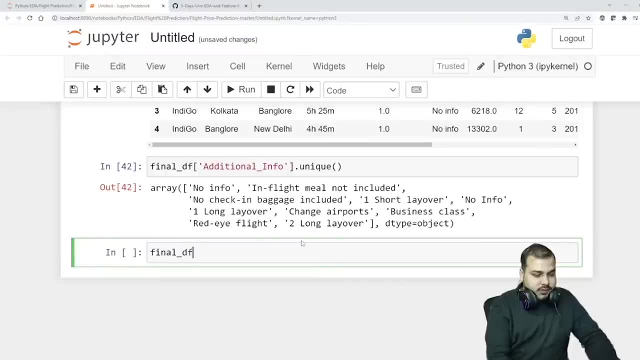 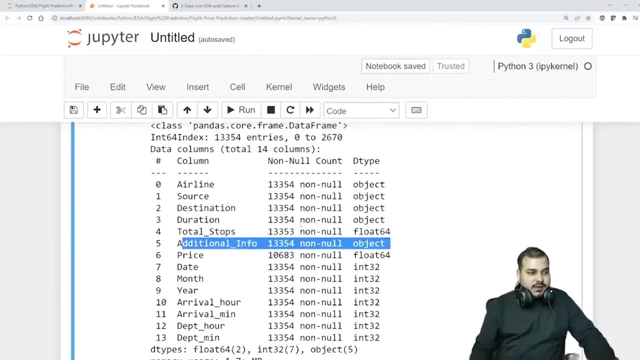 wants to play with this data set? who wants to tear apart this specific data set? let me just see df dot final underscore: df dot info. now here you will be able to see all this. are there additional info in the object? that is fine. duration is still there. 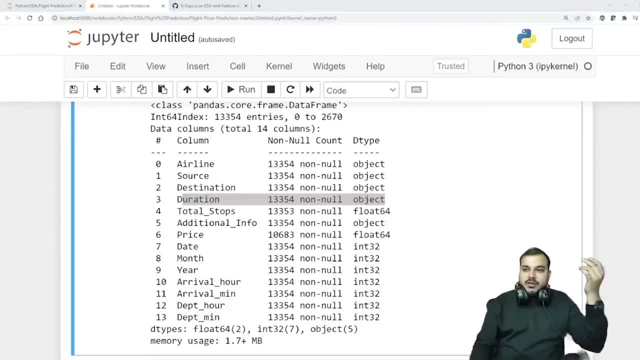 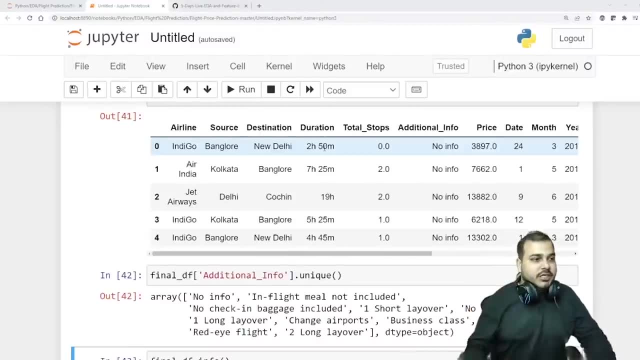 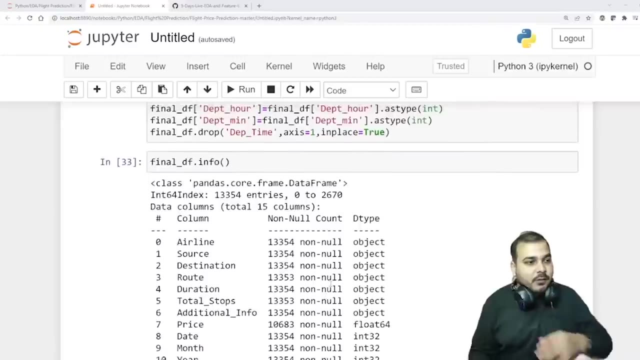 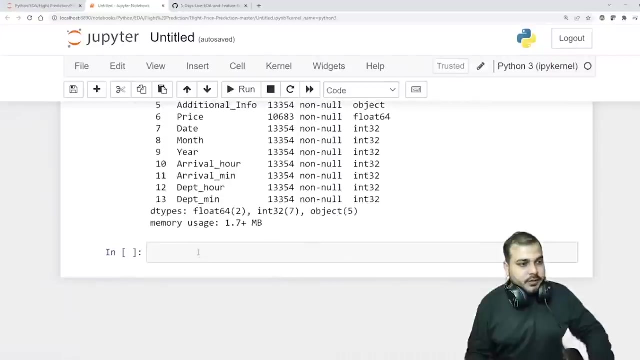 okay, can we do something like convert this duration into something else, duration into minutes? i basically need to convert duration into minutes, right? so this, this, this, this, this. i can basically apply a mathematical formula. i will just take this. let's say: come on, try it out, guys, try it out. so here i'm basically going to write duration. 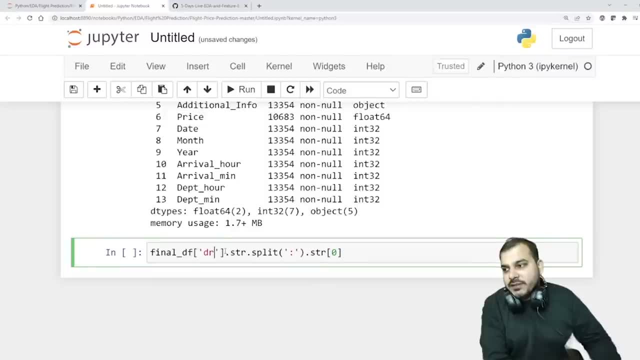 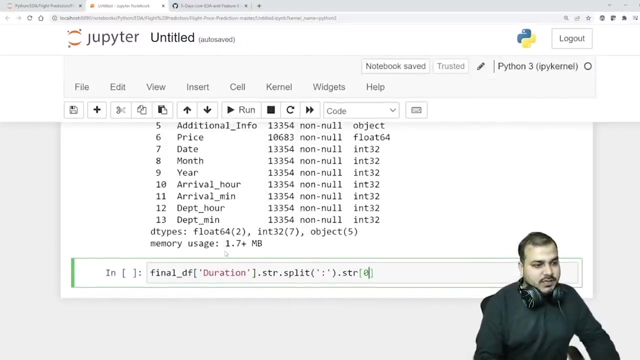 oh, this way, two hours 50 minutes can be mentioned as 2.50. this will also be a good way. um, but what if i convert duration into minutes? that would actually be amazing. okay, so here i'm basically going to say duration. okay, if i do split of zero, that basically means i'm getting my answer as 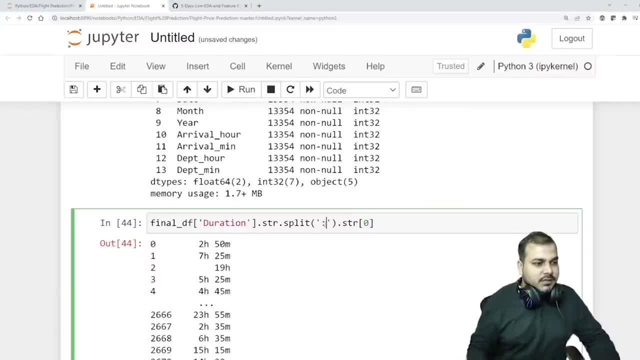 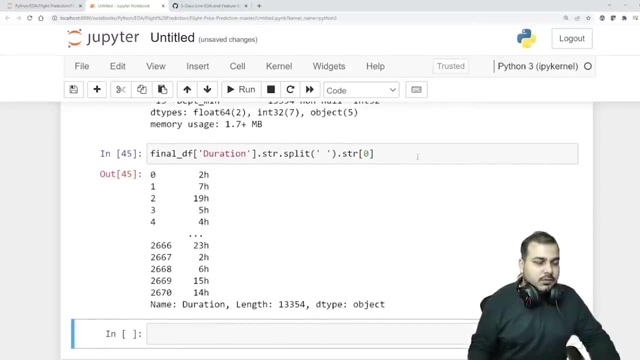 uh, htr of zero split. oh, if i use this blank space, i'll be getting two hours. okay, two hours, two hours, and probably i have to further split it down. i have to further split it down because h is there. okay, h is there. this is becoming a series right now. 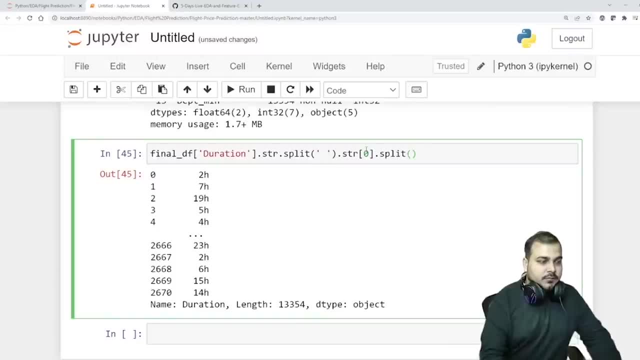 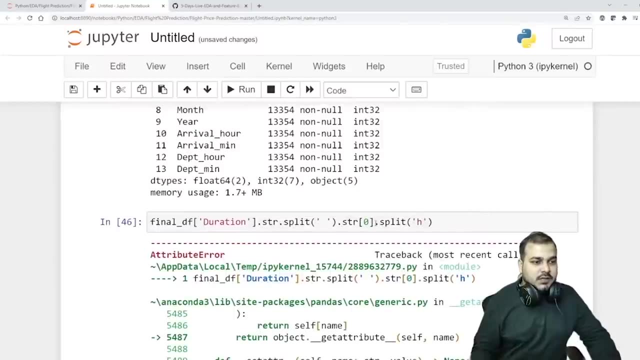 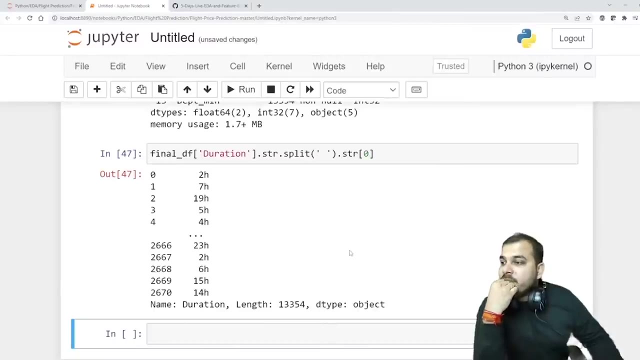 if i do dot split with respect to h. okay, series does not have a split, perfect. so if i have, like this duration, two minutes, sir, can you run split it down with h? yes, dot replace, dot replace will work over here. see, this becomes a series right now. okay, if i execute this. 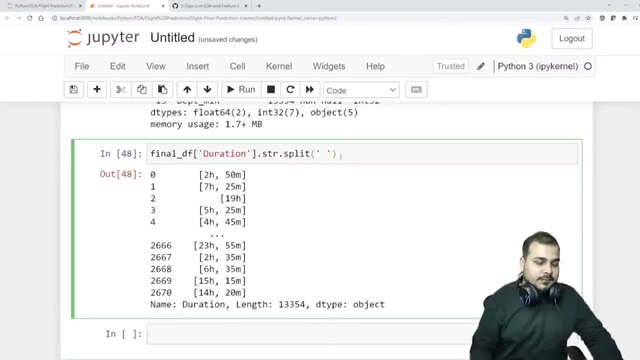 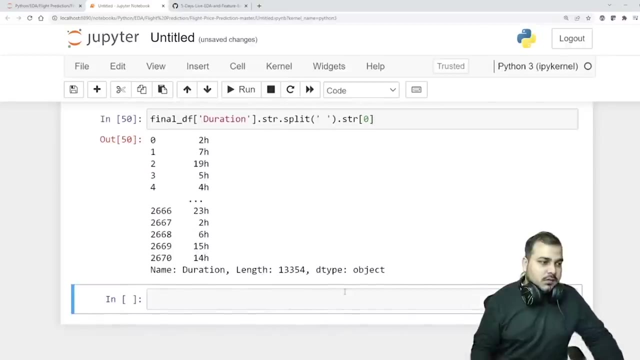 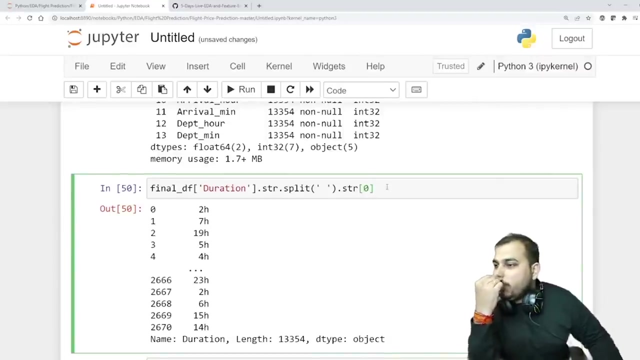 and i'm actually getting something like this. okay, then if i write htr of zero, comma zero, no, this will also not work. zero, zero, zero, zero. come on, anybody. string dot replace. this is a series. okay, this is a series. this is a series. guys understand, we cannot do string dot, something like that. 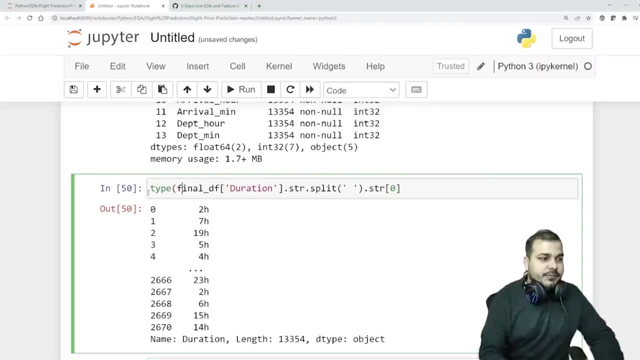 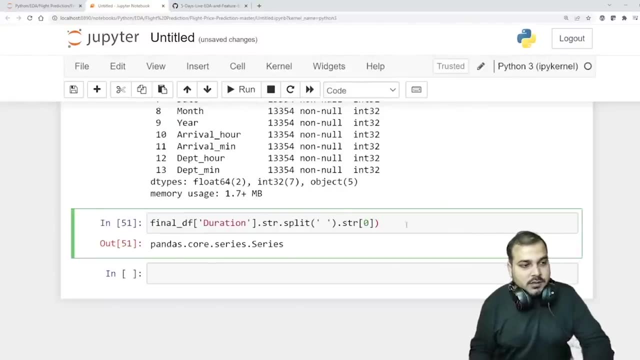 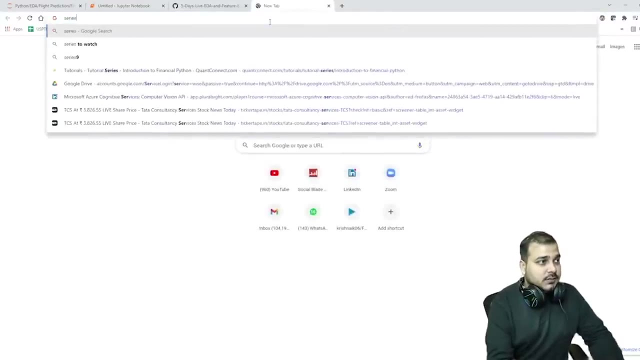 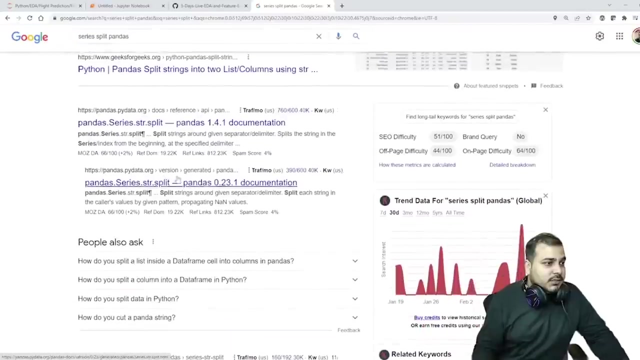 see if i go and probably see the type of this. this will definitely become a series, but it is not going to do string dot, something like this. okay, how to start with string dot. one is not going to create a стр. a word type width helps me build it. 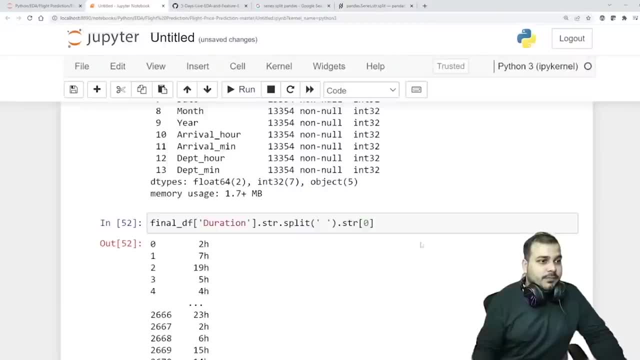 to printing. so because this 400 is also the number, get apart: plus, plus qui, plus do ". so for this one is it has to be kind of split dot split, and here i'm going to basically use h- see, i'm getting it right, and then i can basically 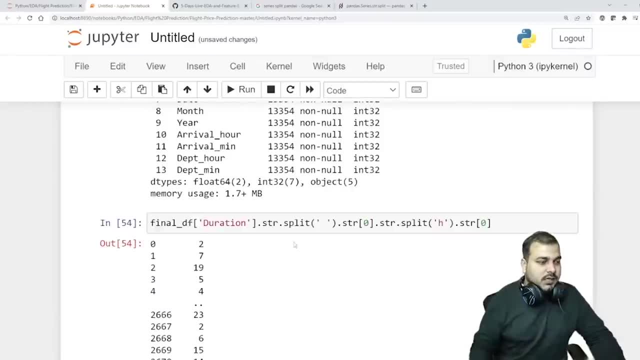 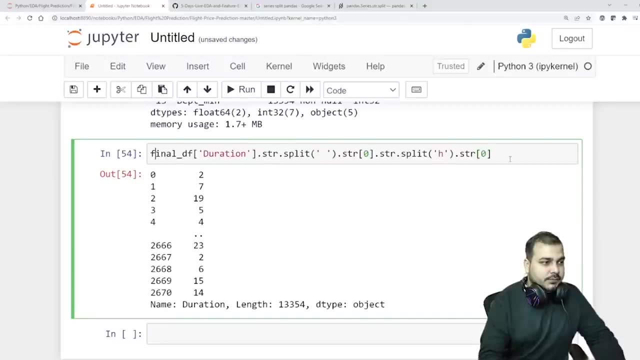 again write htr of 0. so here i'm actually getting all the values. this should be multiplied. this should be converted into an integer. no, this will actually be okay. so here i'm actually able to get all this information. okay, this will basically give me the hours if i want to convert this into. 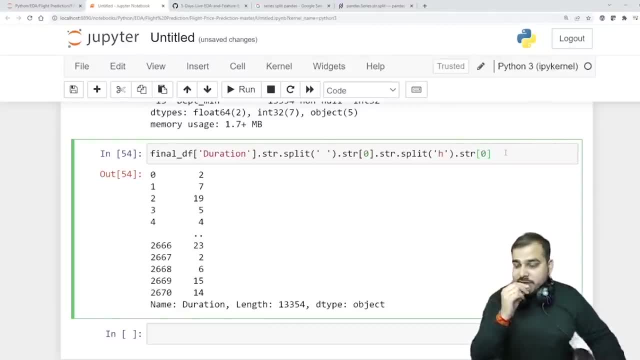 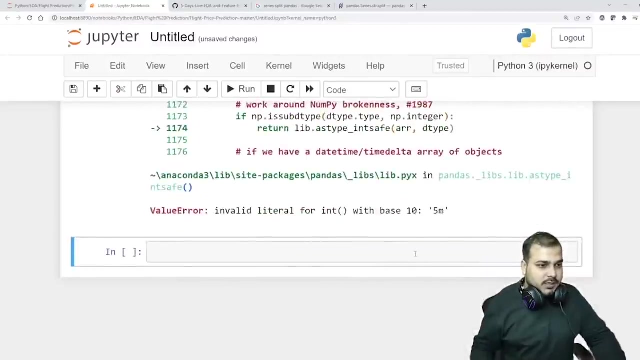 minutes. okay, if i want to basically convert this into minutes, what i have to do? um, now, this is entirely series. if i want to convert this into minutes as type, yeah, as type can work. dot as type. int. no error is coming, probably. no, it will not work. but htr 0 will work. 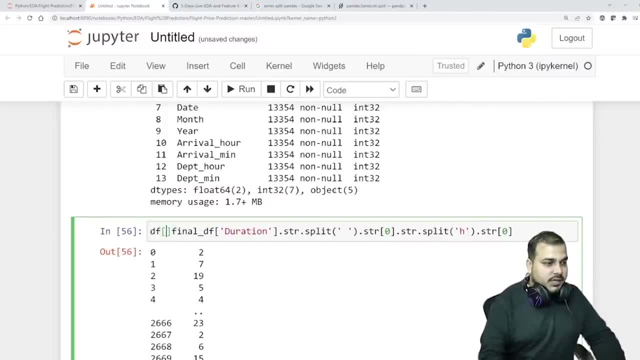 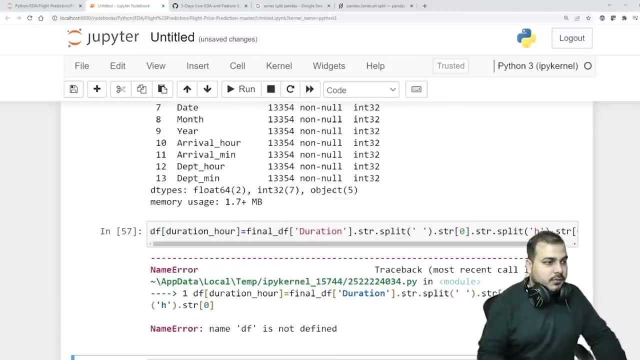 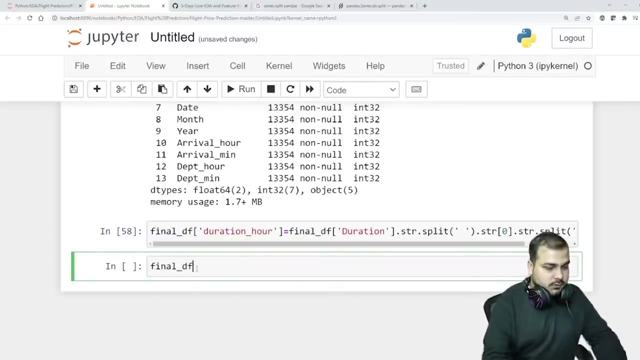 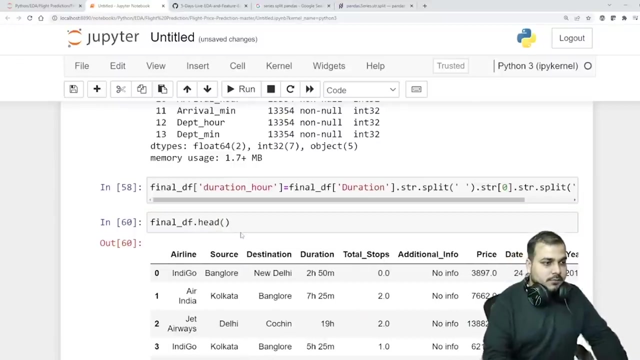 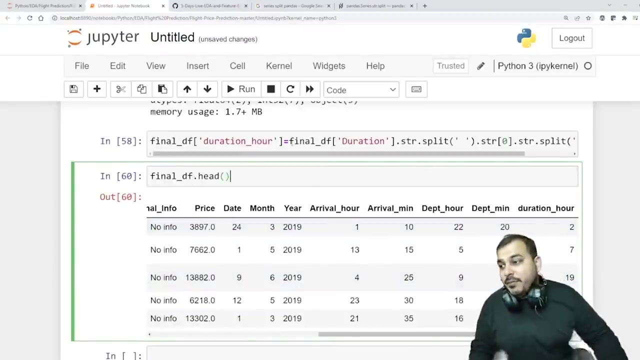 so let's consider that i'm converting this into df of duration. underscore hour is equal to this one duration of hour, final underscore df. if i execute this final underscore df, dot head, so duration hour i have actually got. so, with the help of duration hour, we will be able to do it. 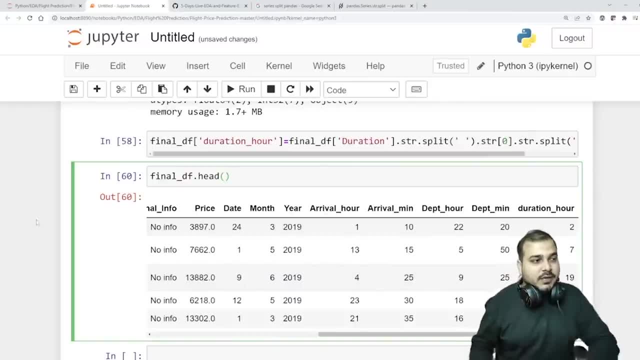 okay, but you also have to get the minutes, because minutes are also very important. but before that, what i'm actually going to do, i'm basically going to write htr of df dot head. so duration hour i have actually got. so, with the help of duration hour, we will be able to do it. 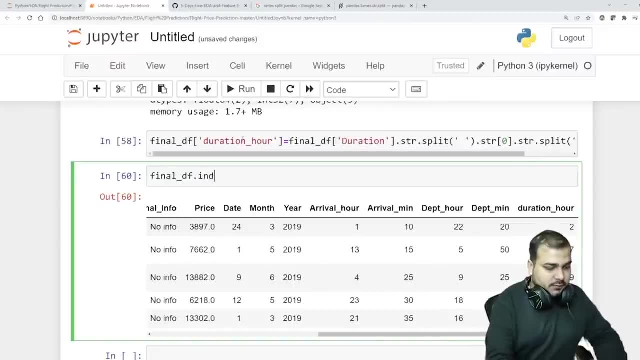 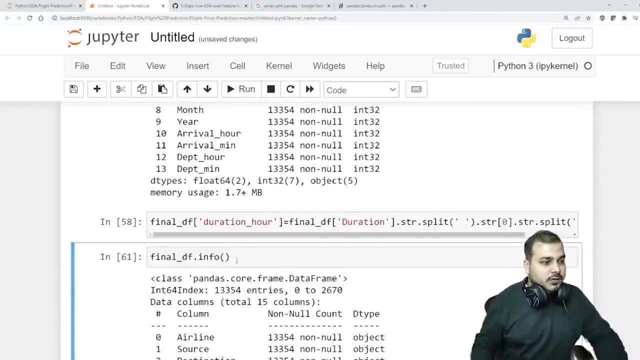 uh, final df for dot info, because i want to check whether this is still in object. right, so what i'm actually going to do? i'm basically going to convert this as type: okay, final underscore df. okay, guys, for me also. same thing, i'm also facing the same difficulty. what you face. right, but we need to think of an approach. if you are able to think as an approach, you may be a free piece. or if you doandle think as an approach, if you are able to think as an approach and you're able to consider your waste of assault as to time and time again, you know many differentoudnt. if you are able to think as an approach, you are able to consider your wasted house. so because you don't, you don't necessarily doing this time and time like a self. and time doesn't mean all this is an easy day or anything else, but you know when you're in that cap policies, considering delivery data. 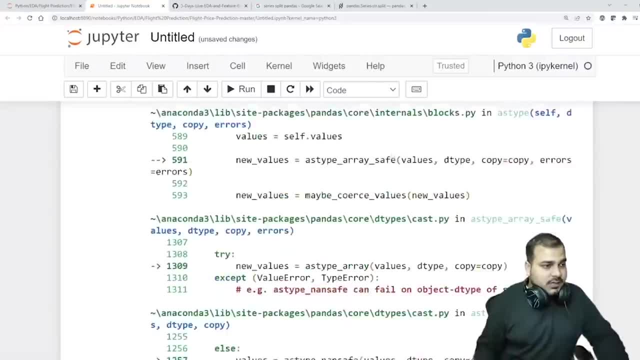 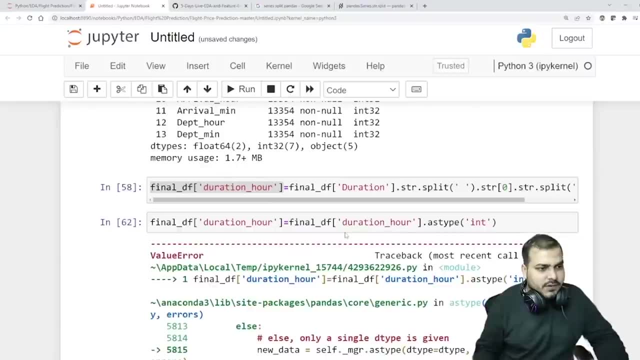 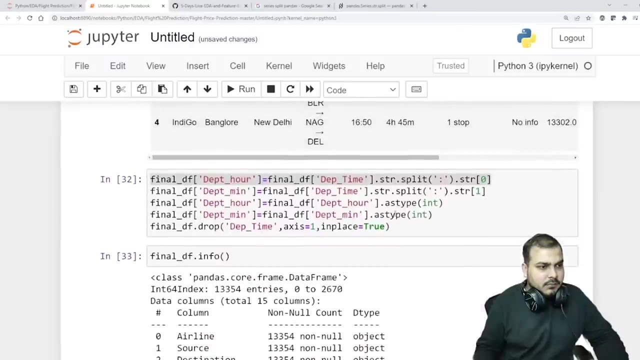 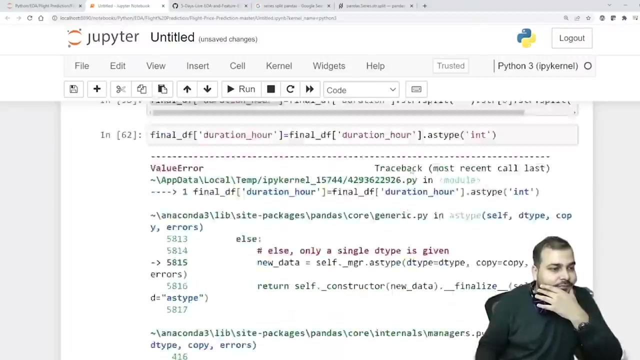 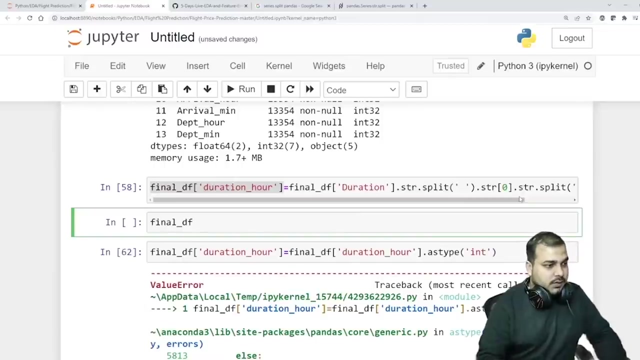 an approach. obviously that will get solved. what is the error for int? there is 5m somewhere, somewhere. 5m is there. I hope I have done the syntax correct. definitely 5m is there somewhere. 5m value is there. final final underscore: df of duration double is equal to 5m. 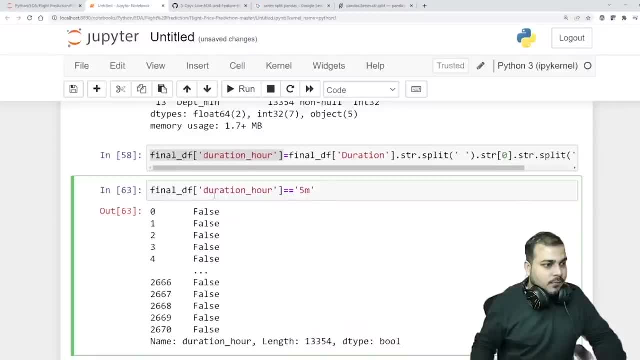 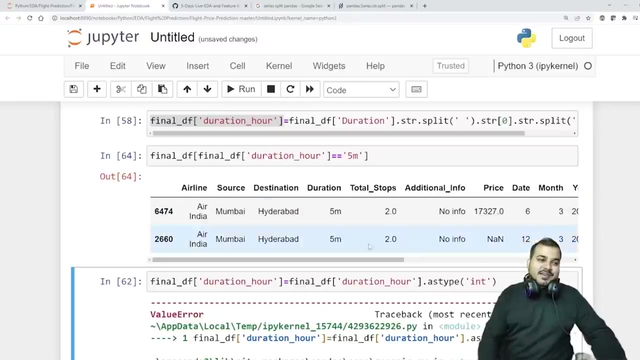 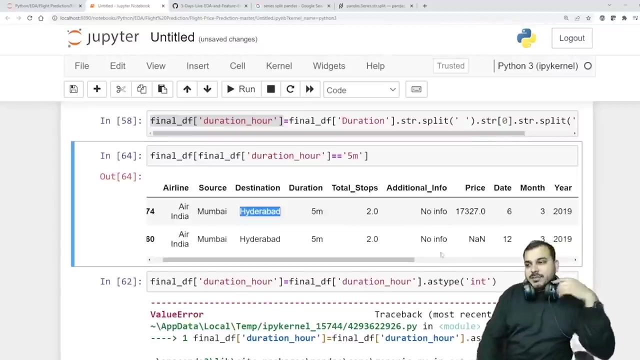 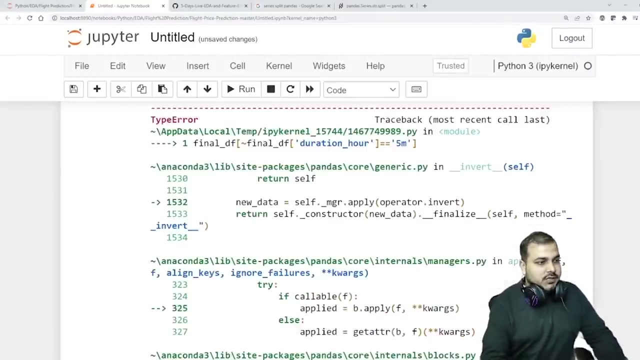 final underscore: df: okay, five minutes. okay, duration is also there for five minutes. okay, this is the problem. but how? how come five minutes? Mumbai to Hyderabad will take only five minutes. how this is possible? it is better we drop this. we drop this features, right. so if I just use this, 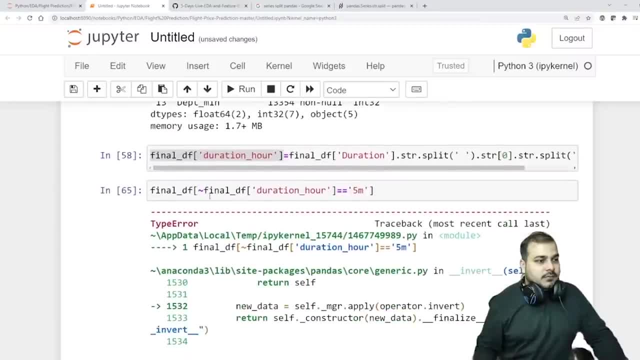 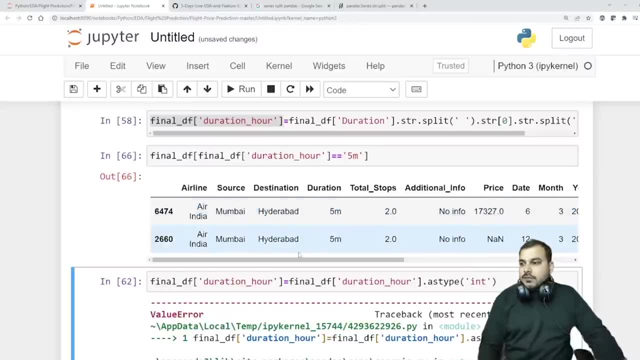 is equal to this one. not possible, right? so how? how this will be possible. so tell me, if you want to remove this, what you have to do: halt, halt duration. okay, halt duration. that is the total duration, right? so this is the total duration, right? so this is the total duration right. 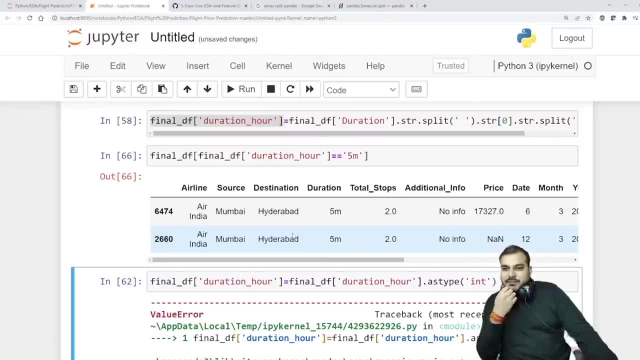 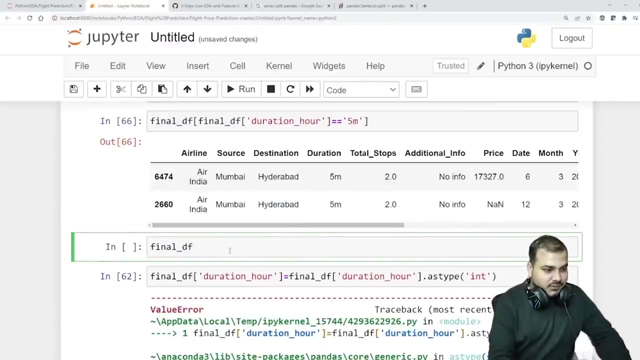 you have to probably drop this records, right? okay, tell me how to drop this records now. drop row axis zero. okay, perfect. so, if I like, final underscore DF, dot drop. and here I'm basically going to give my index number, should I use I lock to drop it, because here it will ask. 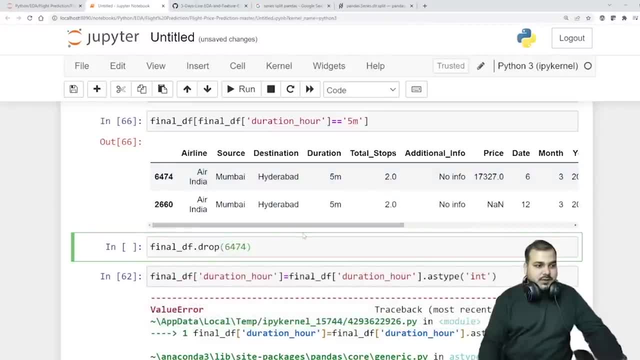 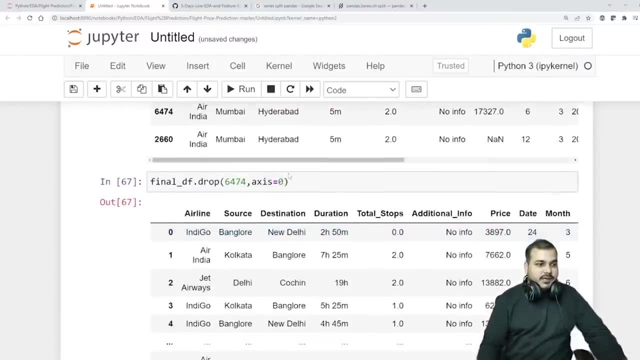 for labels. so suppose if I give six, four, five, seven, four comma axis is equal to zero, you'll be able to see that it will get executed. right, it is getting executed. then let's say: in place is equal to one and same thing. I will probably do it for two, six, six, zero. 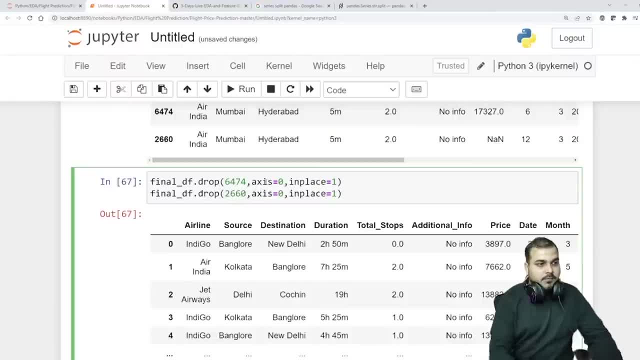 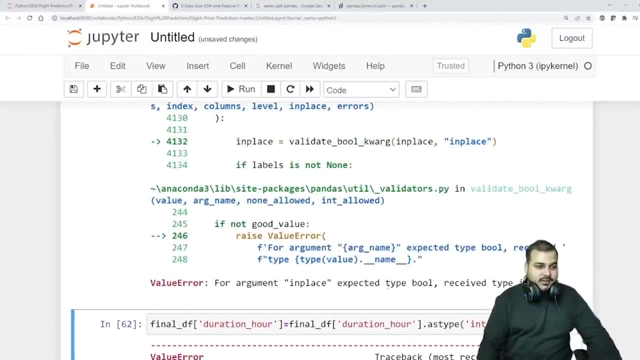 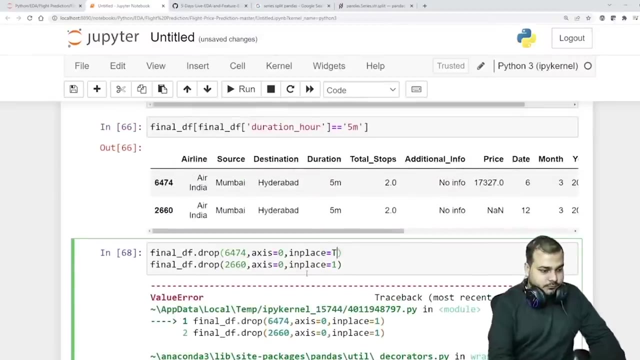 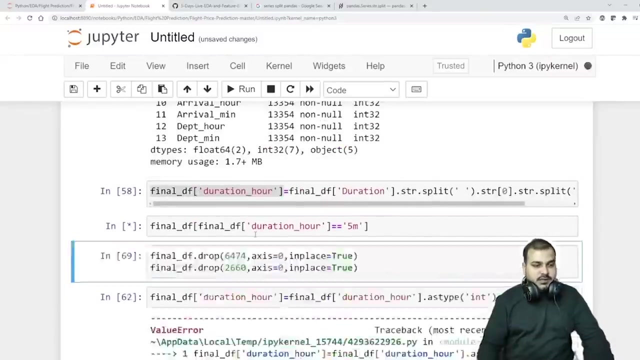 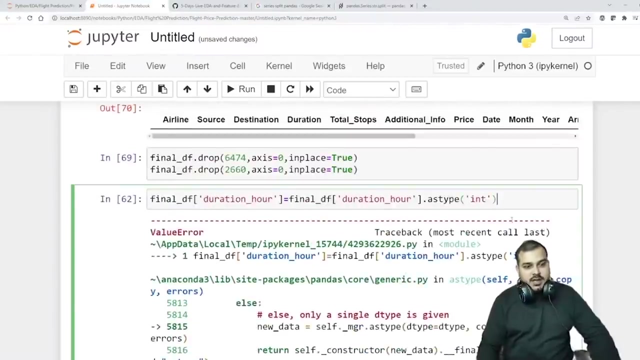 two, six, six, zero. received type as input for argument: in place. expected type boolean: oh, in place is equal to true. true, so executed. this is working fine. now, if I go and see this one, I'm actually getting empty now. okay, so I have actually fixed this. I will convert this into as in type done and then I will multiply this all by 60.. 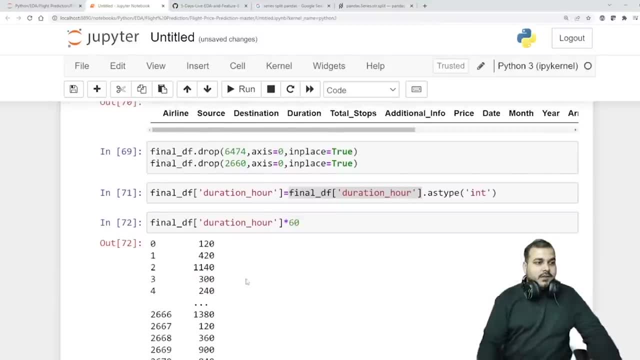 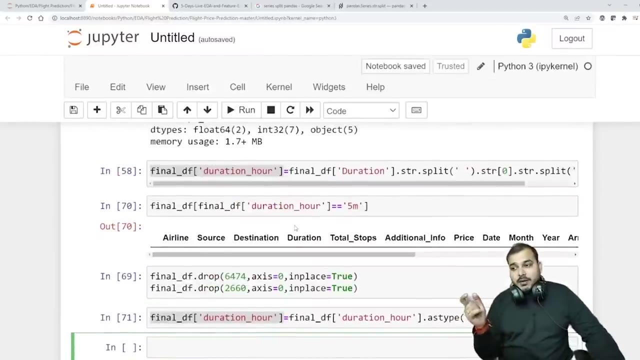 multiply by 60. so here you can see I'm actually able to get this in the form of minutes or let it be in hour only. then no problem. if you don't want to do also, it is fine. at least hours will increase, but if you are considering the minute part also, so try to use that. 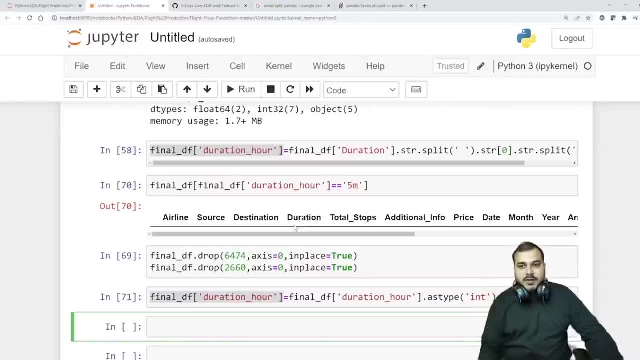 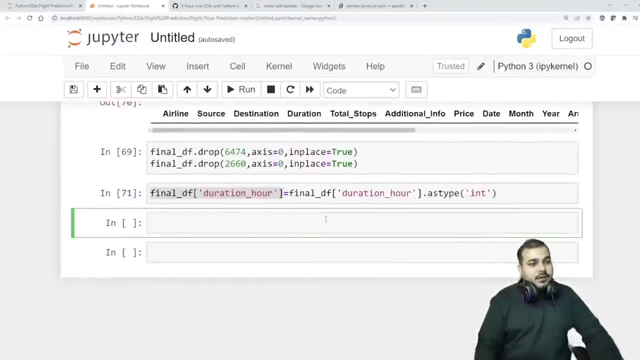 okay, and try to convert that. that is just given to you as an assignment. please try to do for the minutes also try to get that specific data. what I have done for minutes. okay, everybody, you have to basically do it. okay, don't say that crash, you did not do in the class so we are not going to do. 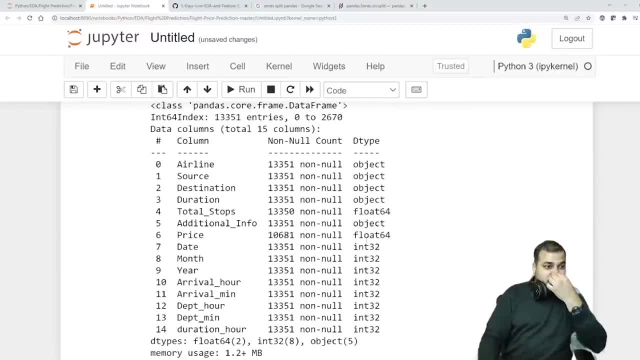 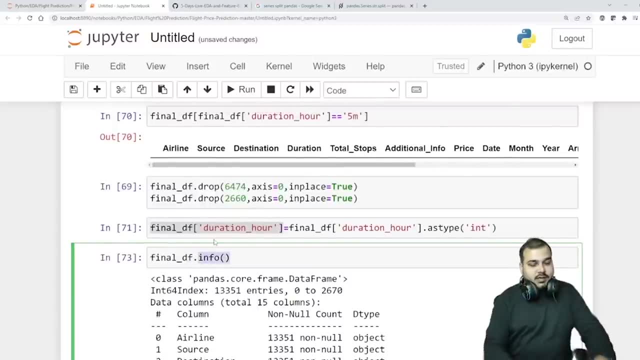 don't do it. so here you have integer integer. integer integer price is float. additional info is object. then you have duration. now we can drop the duration. final underscore: df- dot. drop. final underscore df- dot. drop. okay. duration with axis equal to 1: okay, and then in place is equal to 2. so this is done. 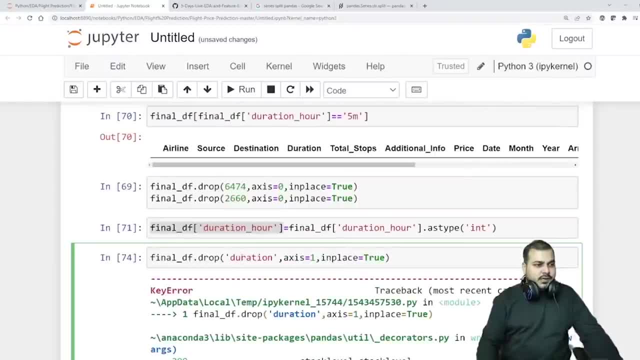 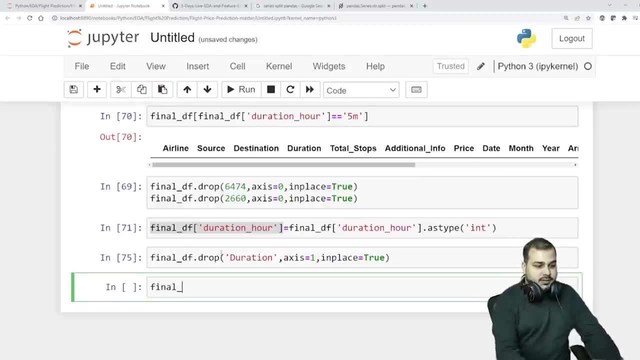 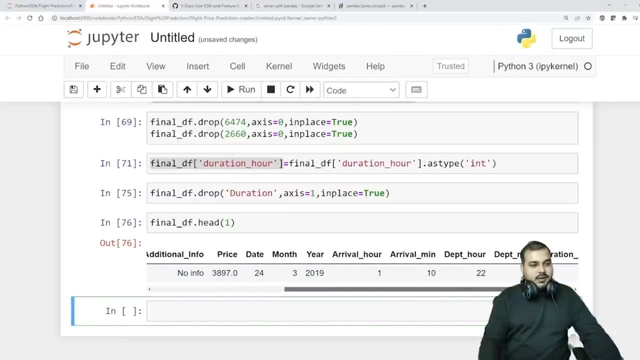 yy, yy, yy. capital D, capital D, capital D: okay, duration done. and then, finally, we have final underscore: df, dot, head of 1. so here you can see I have all these things remaining. all have been converted. remaining, all are category features. so, in order to do for 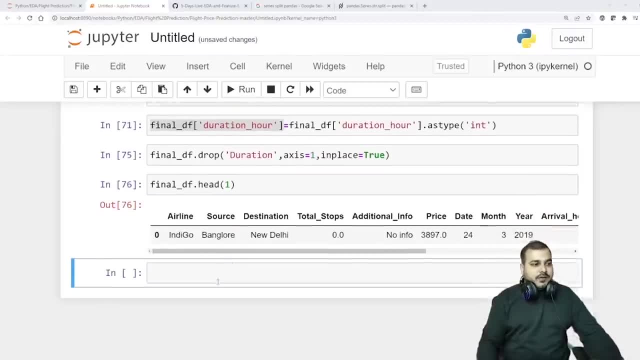 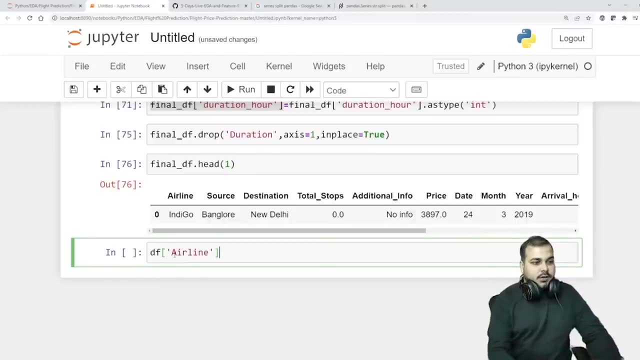 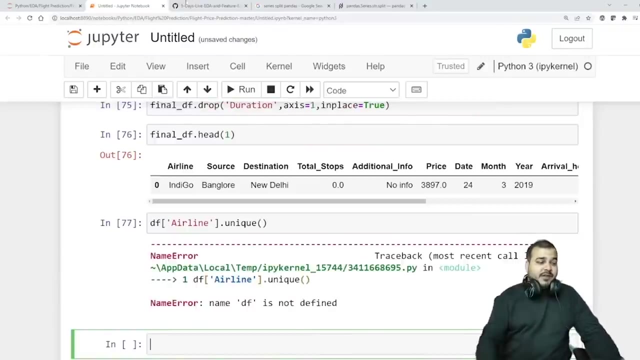 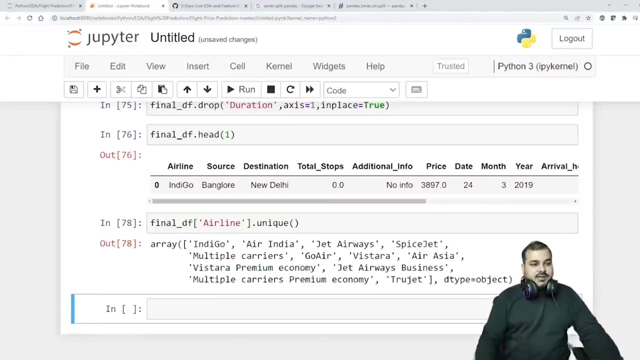 the category features one we need to do simple. we will try to first of all see, with respect to airlines, so airline dot unique, if I try to see this, how many are this specific airline? final underscore DF. final underscore DF. so here you can see only this many airlines are there. 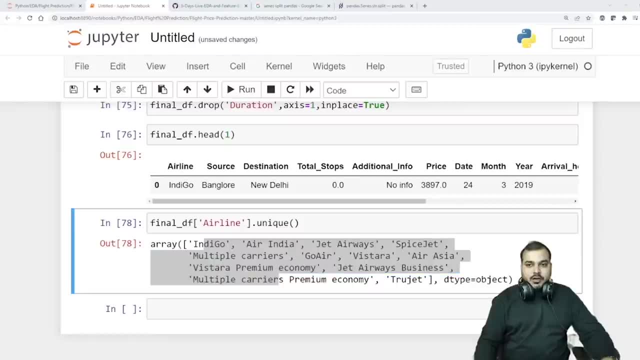 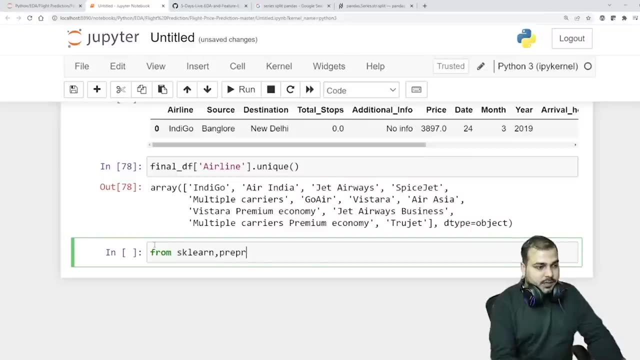 so we will try to do label encoding for all of them. now, in order to do the label encoding, I will write from SK: learn dot. pre-processing- dot. pre-processing- import label encoder. many people are saying: right, Krish, why you're doing get dummies. get dummies can also be done, but since we try to work, 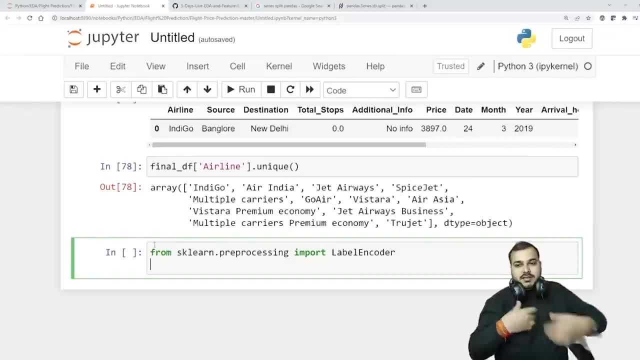 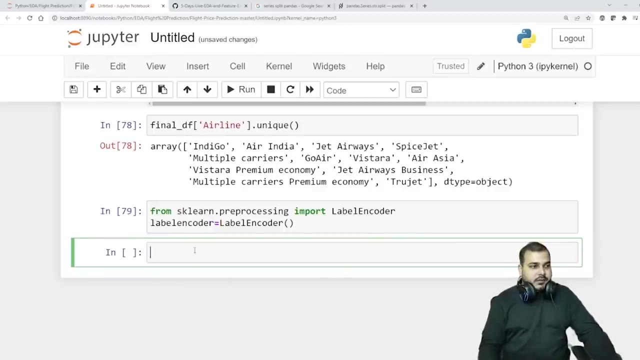 with train and test data. so it is better to use the data. so its better to use the transform techniques, right? so here i'm going to basically use: label encoder is equal to label encoder, okay, so label encoder is there, and then finally you do it for every. 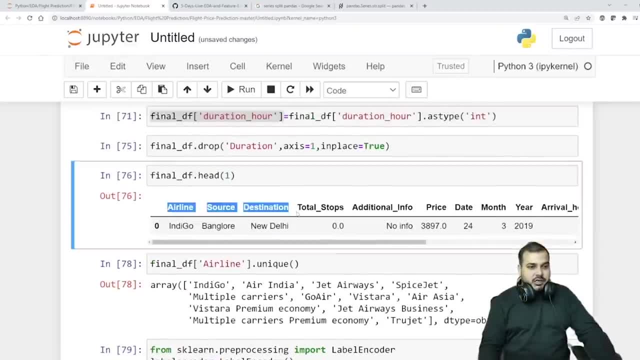 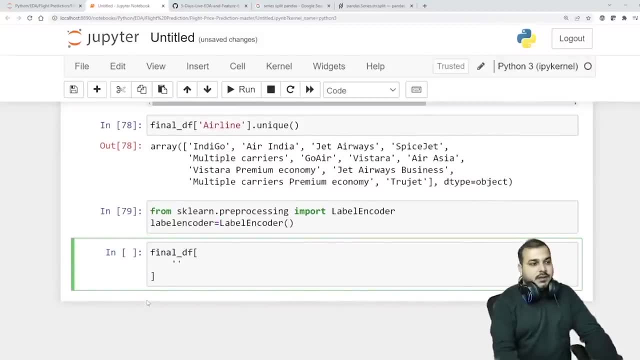 data set that you want, like airline source, destination and additional info. so there's four features. so here you have final underscore df and here you can basically write airline- airline okay, label, encoder, dot, fit, underscore transform. and here i'm basically going to give my feature, that is final underscore dm on airline, right. so like this i've written for this: 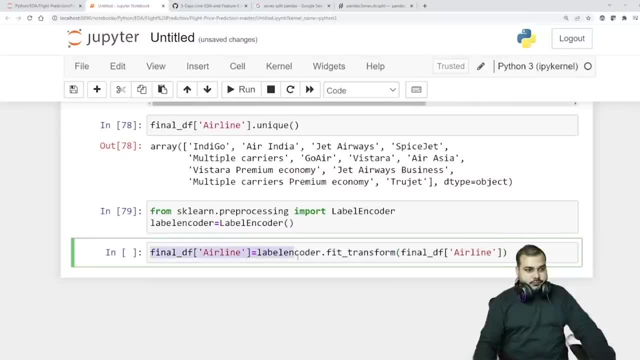 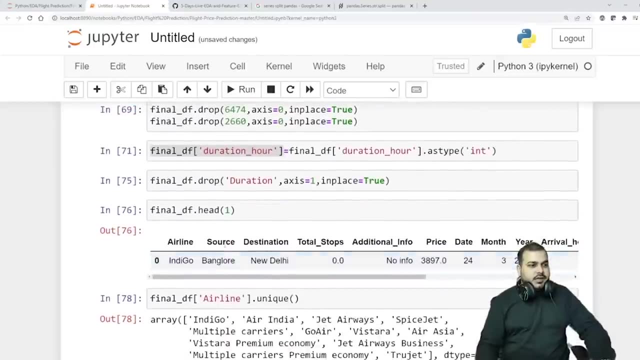 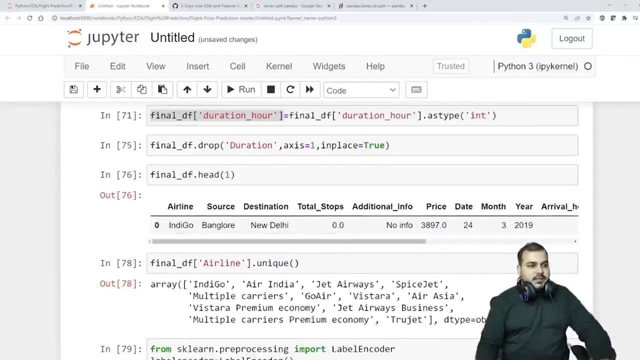 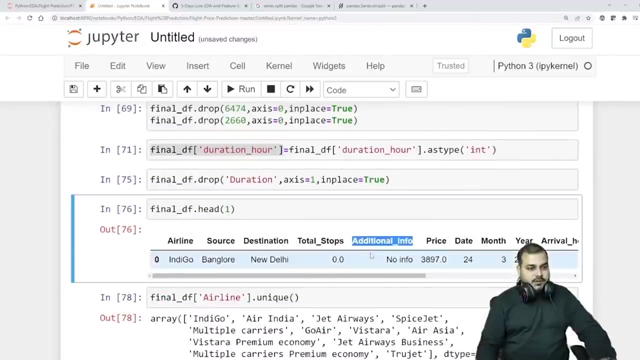 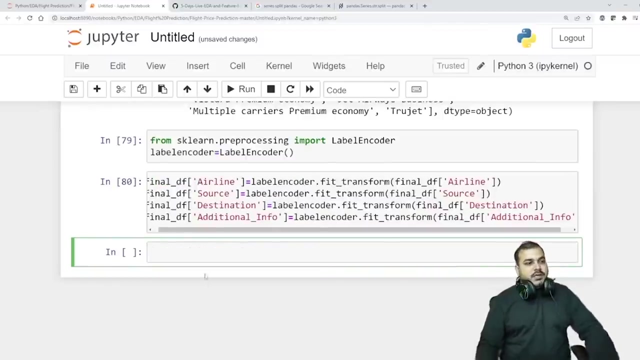 now you do it for other features also like this same way. you. how many features? are there? four right. then you have source- source, you can put it over here. then you have destination and then, finally, you have additional info. so, once you do, this done, and this is your final underscore, df dot. 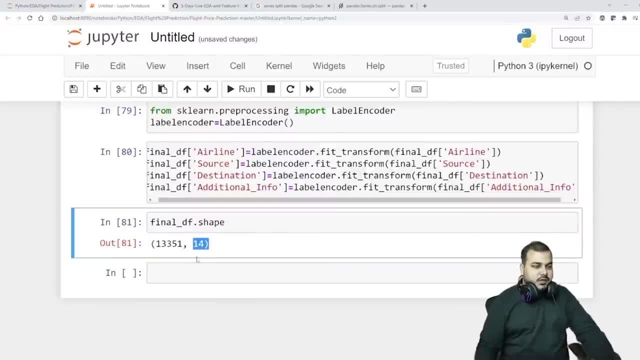 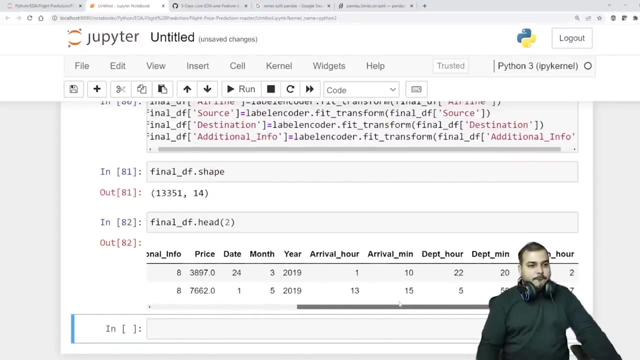 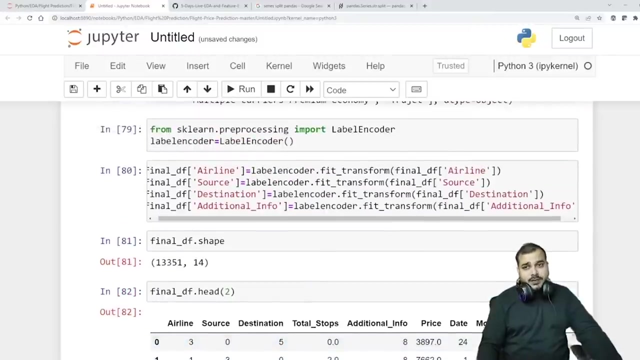 shape. if i try to see they are on 14 columns, which is good enough, and if i want to probably see my final underscore date dot head of first two records, then you can see all these things. perfect. okay, i've done, just done label encoding. you can also do other type of encoding. that is one hot. 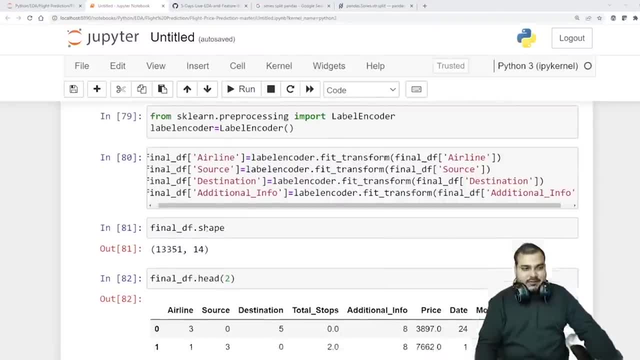 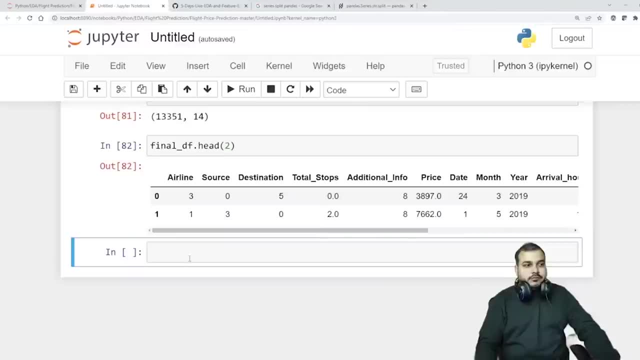 encoding. it's okay, guys, i've done label encoding. now one more step you can do is one hot encoding from sk. learn dot pre-processing. import one hot encoder, just do it. no, kevin, don't do it with get dummies, because, see, whenever we have a test data, we need to. 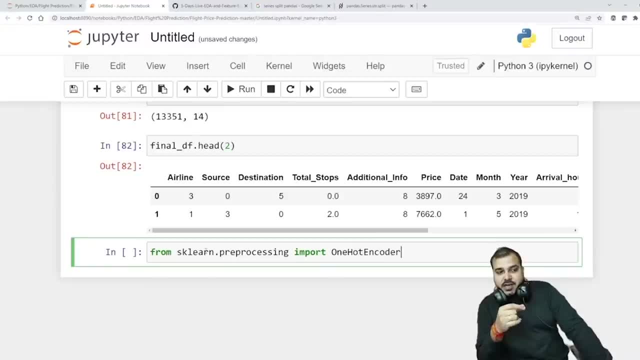 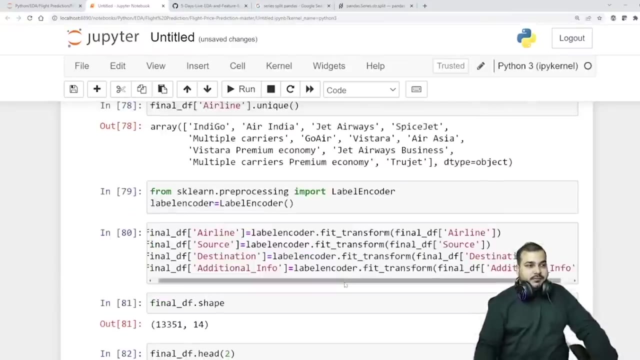 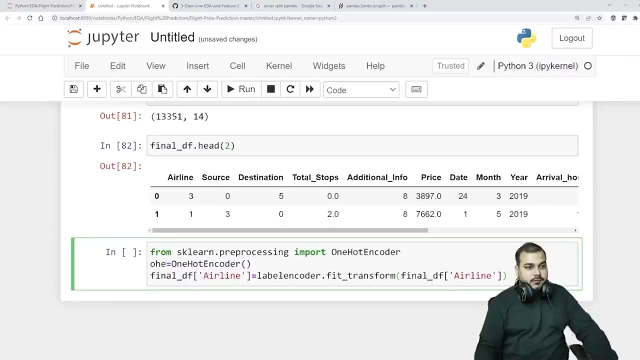 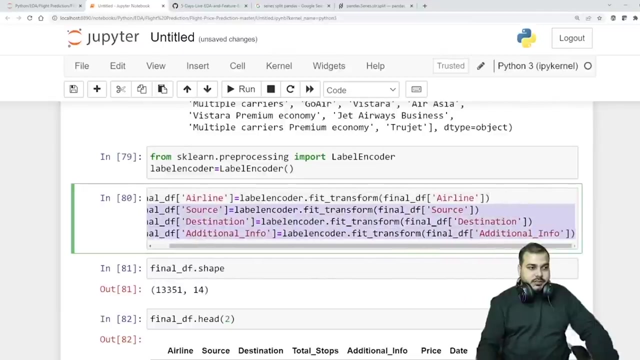 transform that test data, right, so we can save this encoding in the form of pickle file. right? so one hot encoder. so o h e, i will write it as one hot encoder and then you can do the same thing where you are specifically saying this: okay, airline o h e dot fit transform, okay. and then you have all the necessary other information. 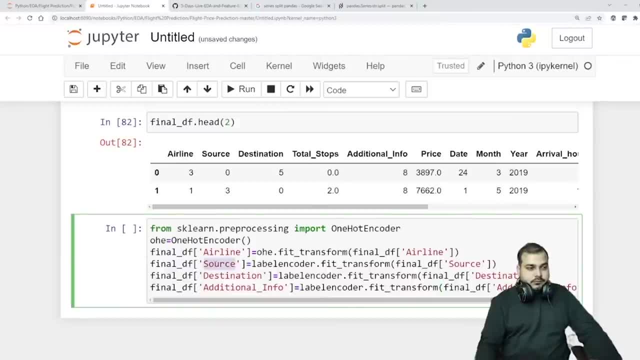 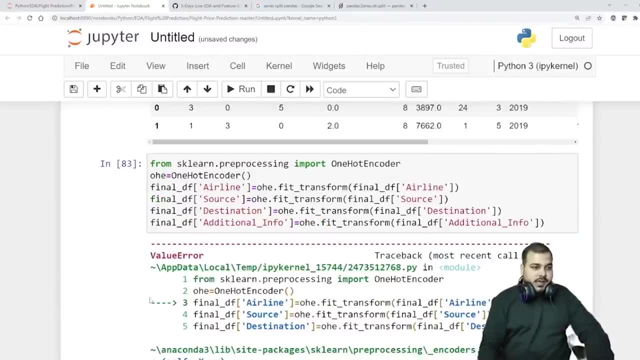 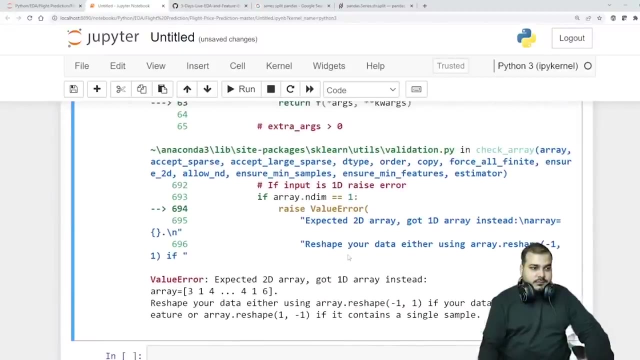 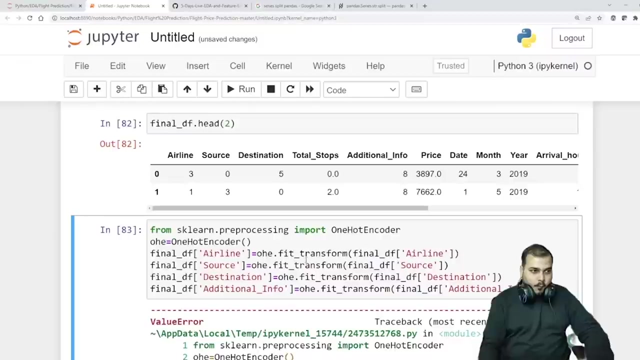 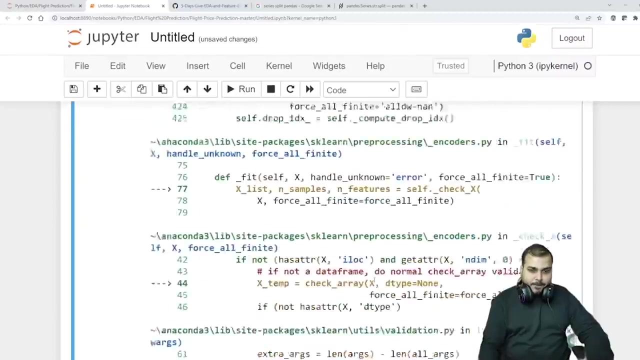 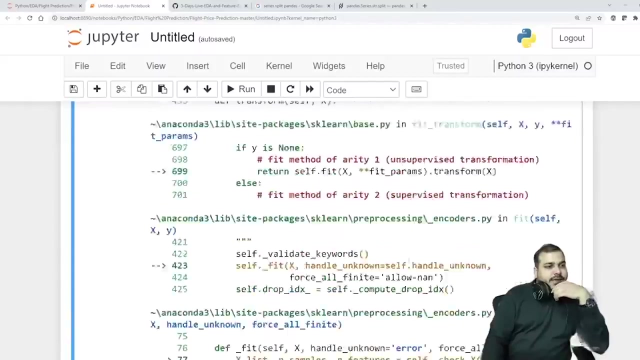 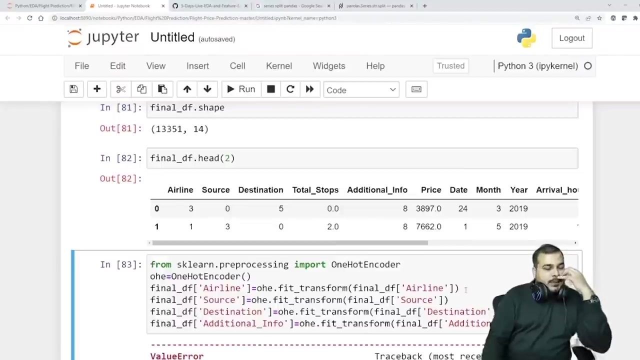 done okay and do it okay. i'm getting the hang of it. here we go. okay, here we go. some error. what is the error? expected a 2D array. expected a 2D array over here. reshape your data, ok, I understood what is the problem. what is the problem? I understood? 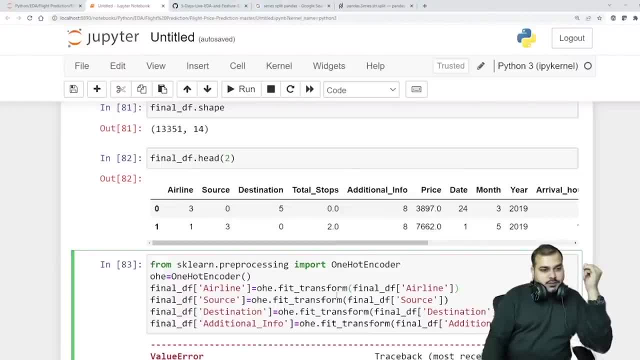 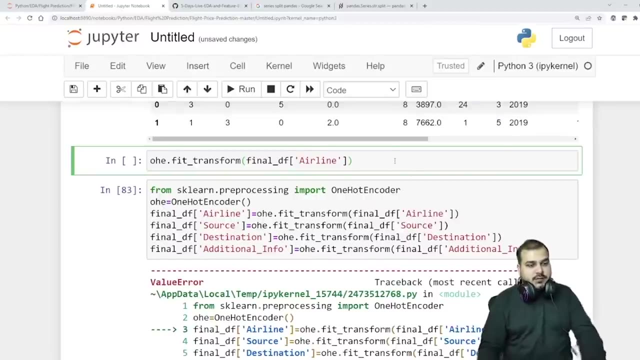 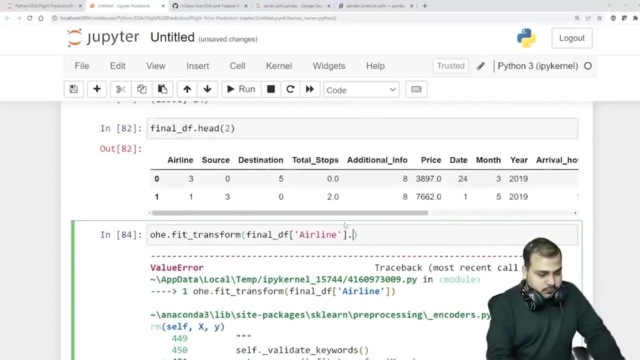 you have to give it as wait. I will execute it in front of you. till then, just see what is the error that we are getting in this. I have understood the error of a transform C. if I execute this, I will be getting an error expected. 2D array dot series. ok, 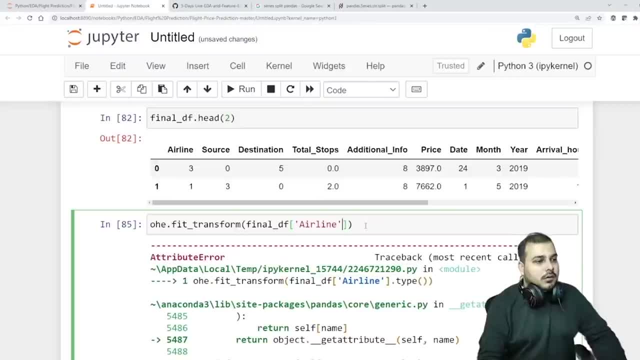 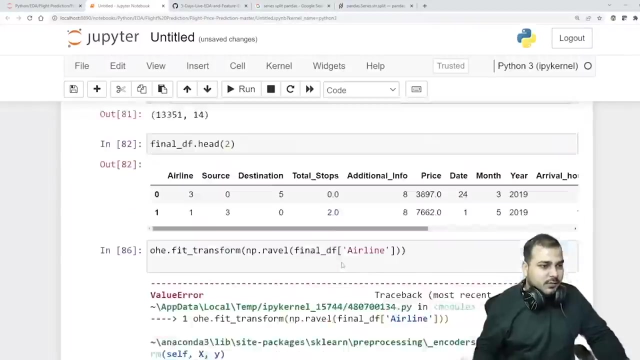 this is a series: dot dot, dot, dot, dot, dot dot. OHE transform npravel. yeah, npravel. ok, but I don't think so this will work. There will be an error. expected a 2D array instead of getting one. I can understand this. 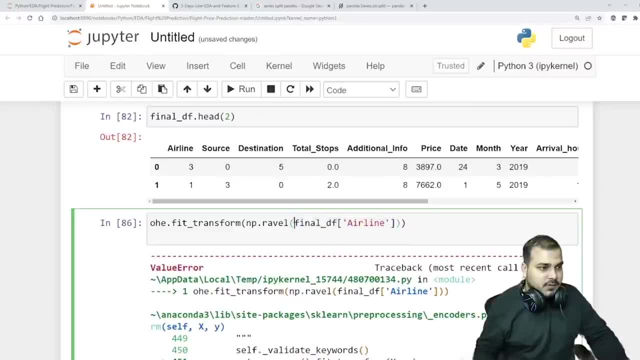 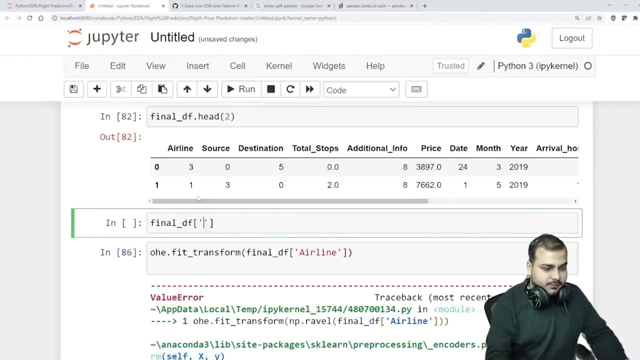 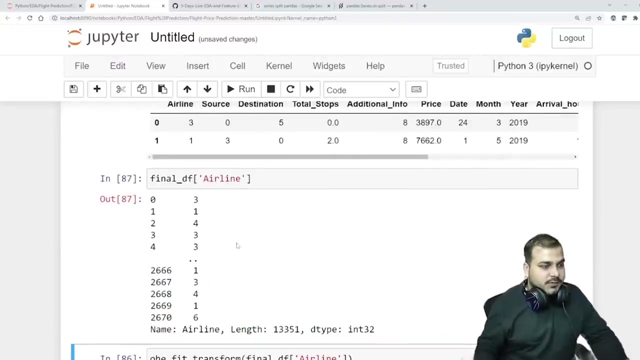 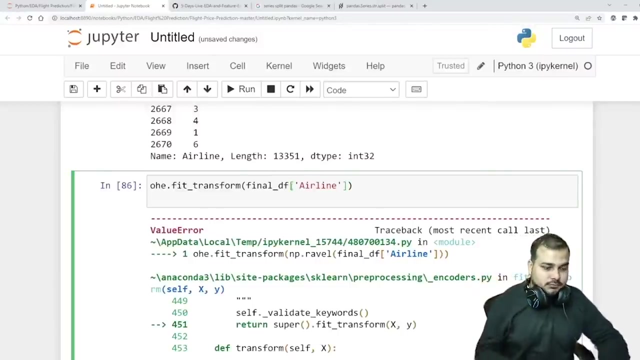 I should not give this in the form of series. ok, that is the problem. I should definitely not give in the form of series. so if I write final underscore df of airline, so here you can see that I am writing in the form of series. this should not be in the form of series. use two brackets. 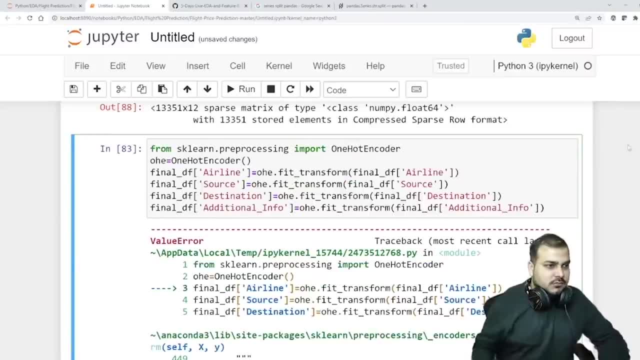 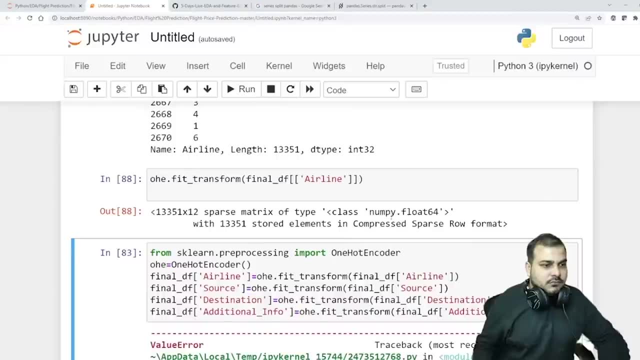 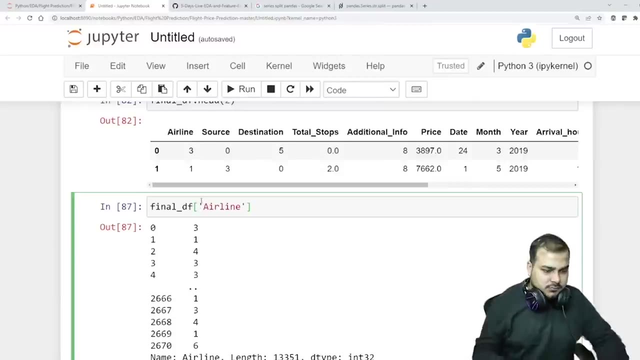 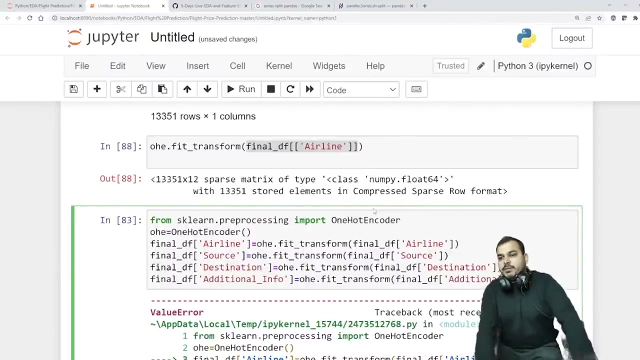 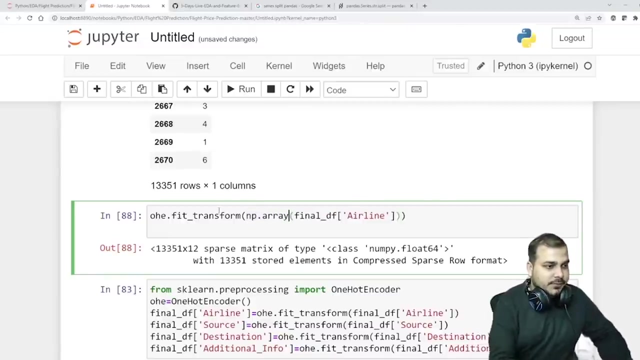 like this you think now, then it becomes something else. final underscore df- ok, now, double cases. we are getting compressed parse row format: nparray df of airline- ok. one way I can basically do over here is like nparray. final underscore df of airline- dot reshape. 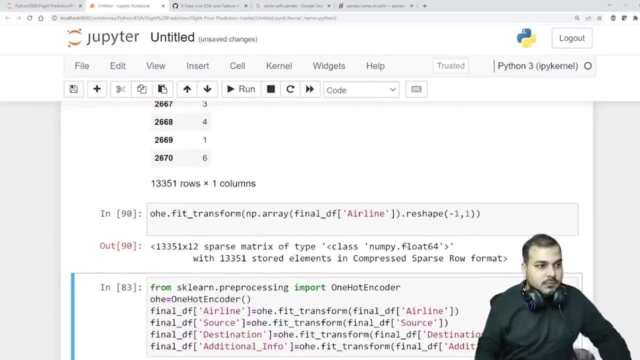 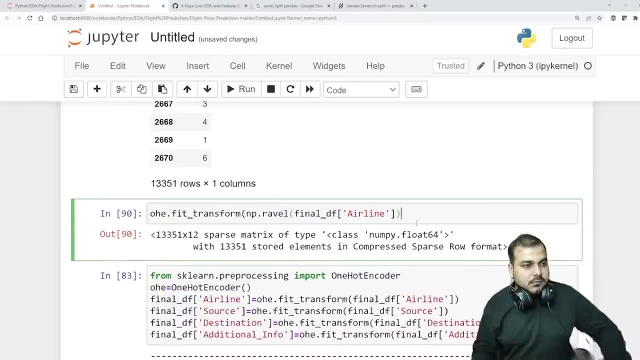 minus 1 comma 1.. Same thing we are getting. Ok, that means I need to get in this, So let's find it. I will call it the minus 1 comma 1.. We can see that, Ok, And now. 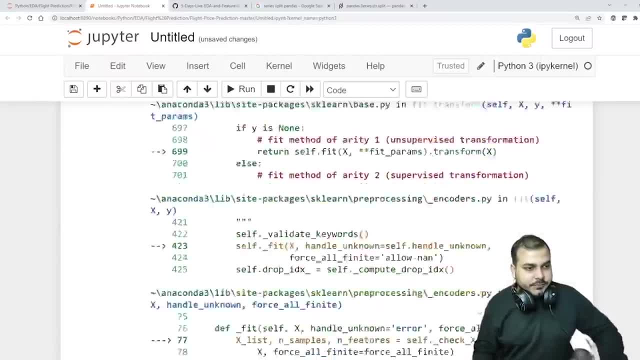 I can put in that I am going to get in this. So the next one is like minus 1 comma 1.. I am going to write it in this. This is a problem. I am going to write only like one comma. 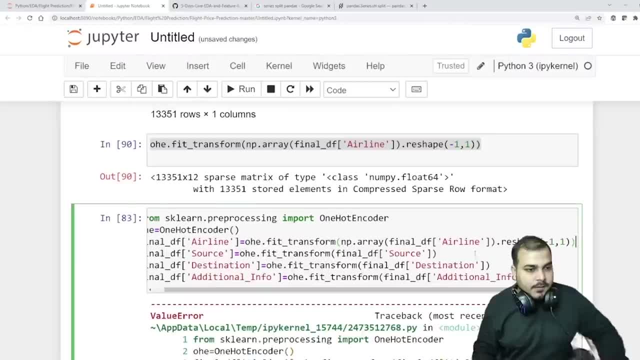 Ok, let's Ok, got it. Now I am going to do some translation where you want to go. Let me just go to this page and I am going to go here. So I am going to go to the HTML page. 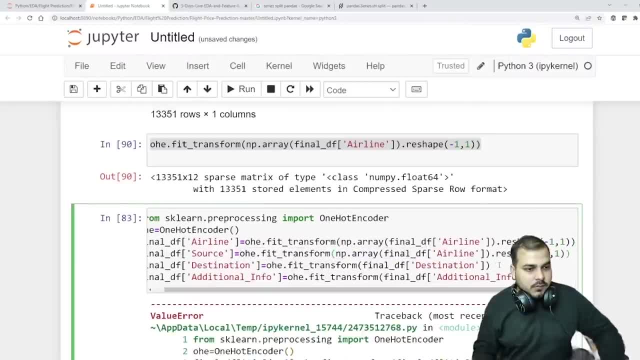 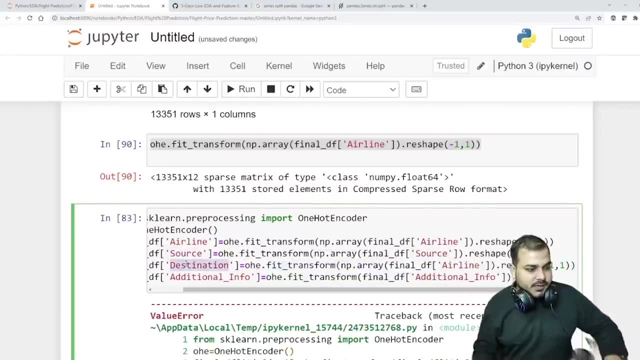 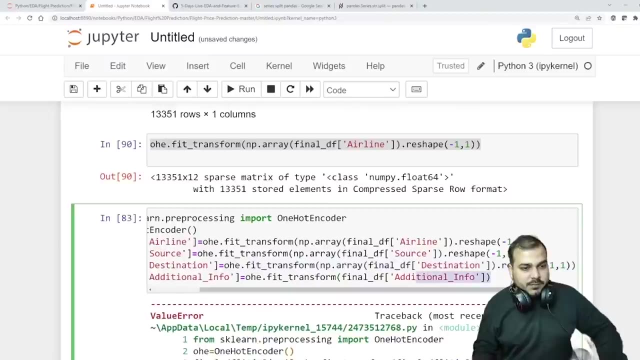 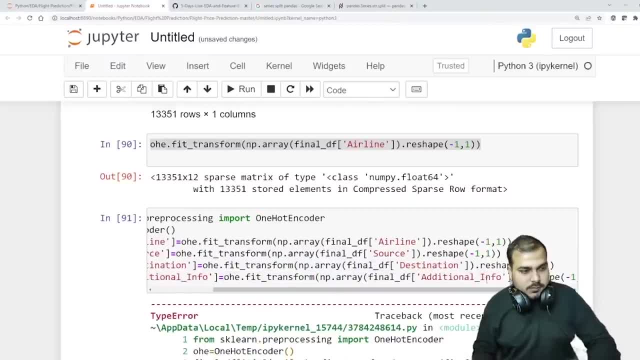 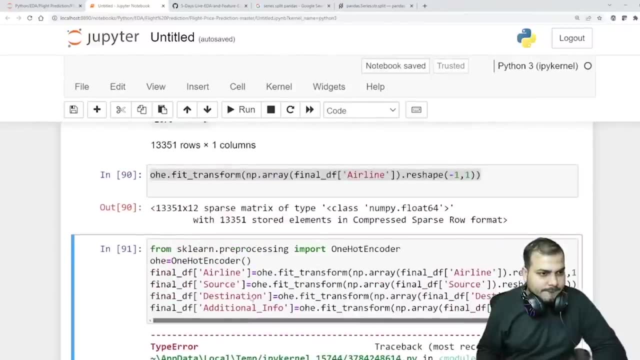 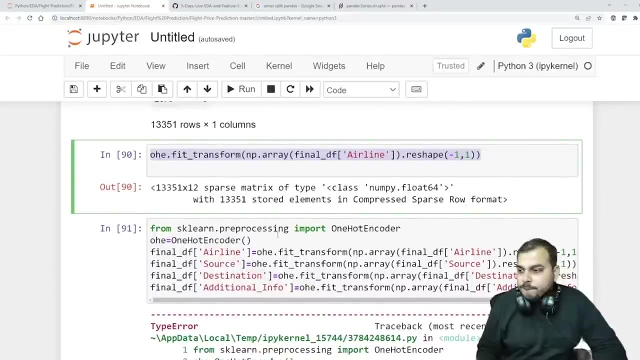 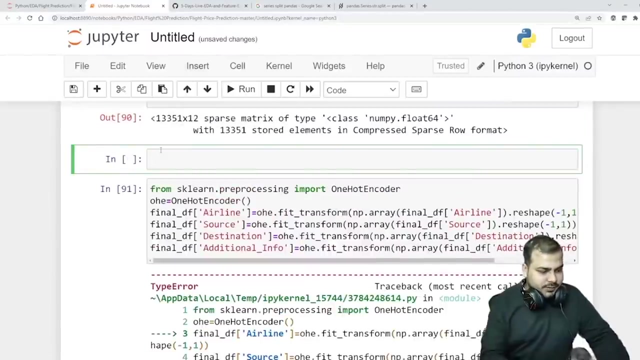 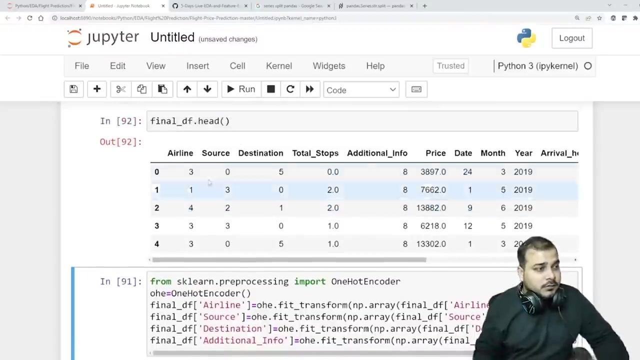 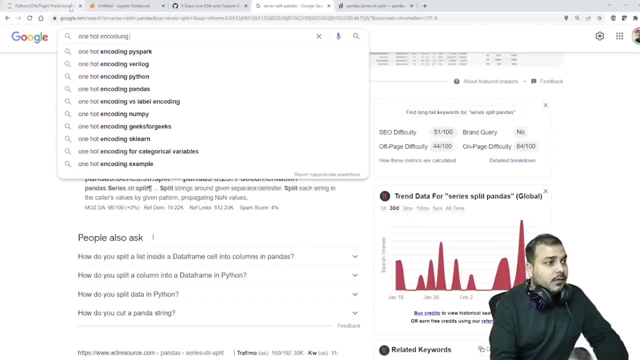 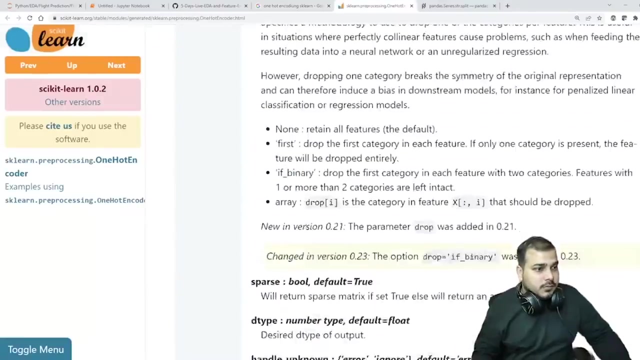 This is one hot encoding we are doing already. encoding is done, Wait, wait, wait, wait. let's see final underscore: df dot head. so this is one hot encoding. so if I probably search for one hot encoding, let's see the documentation you are encoding. 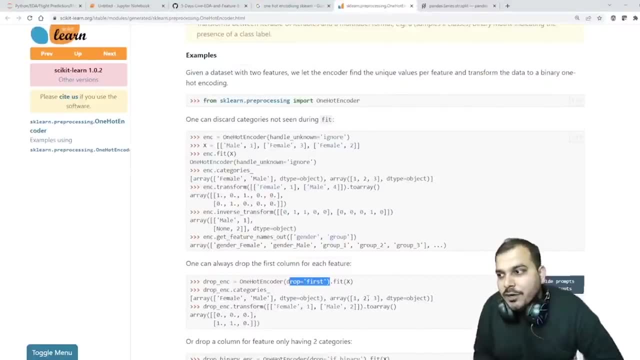 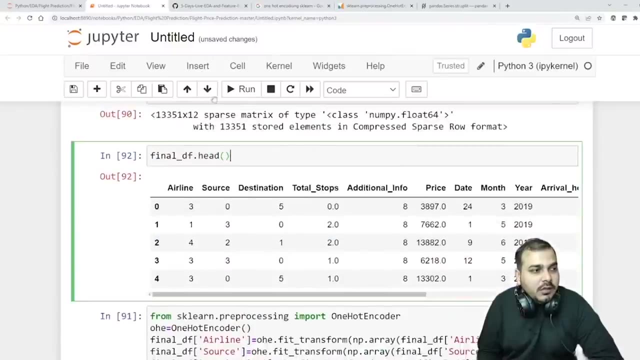 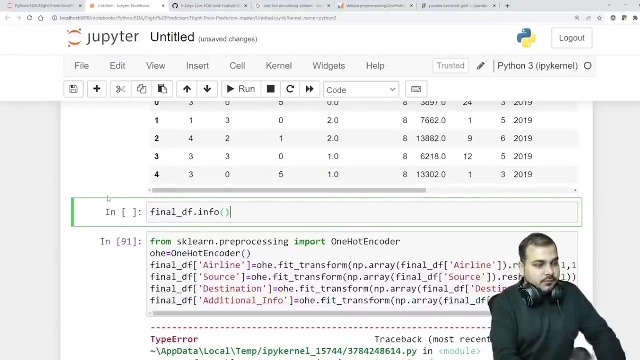 many times. No, I did not encode many times, I just encoded one time right. So after encoding, that value has got converted to this right now. if you go and see final underscore df- final underscore df- dot info. so here you will be able to see that this. 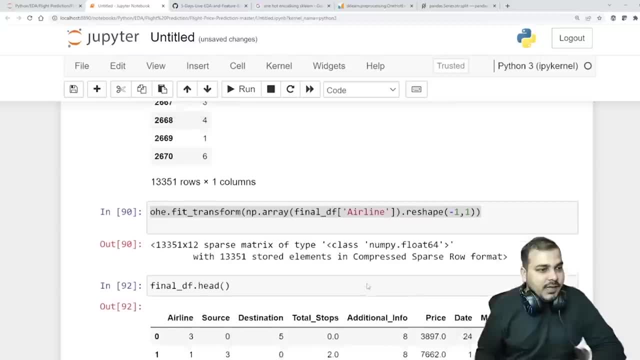 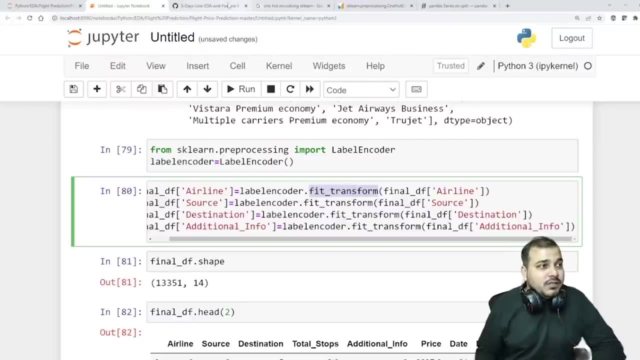 is all converted into integer types. okay, I know I should not had done this encoding separately like this fit transform. instead of this, I could have focused on one hot encoder. it would have done, But it's okay. let's do one thing now, simple. if this is not working, I am just going to 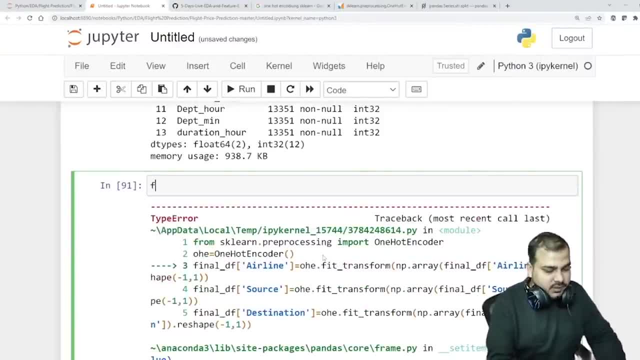 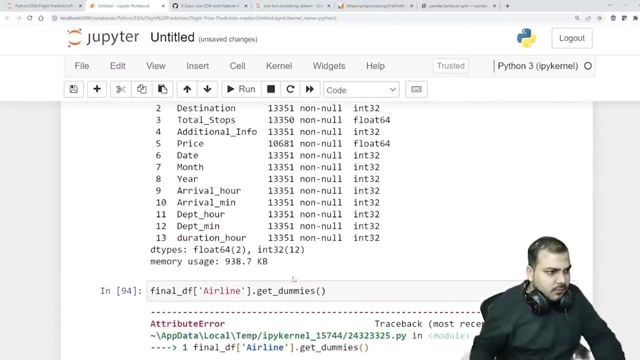 do a very simple thing, So I am basically going to do final underscore: df dot of airline dot. get underscore dummies. oh, get underscore dummies is not there, okay, PDF, PDF, PDF. PDF, PDF, PDF dot. get dummies right. 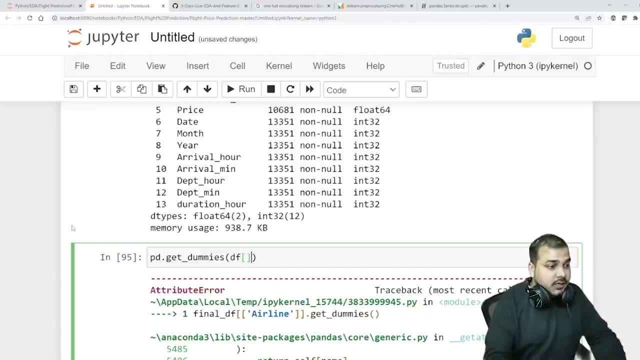 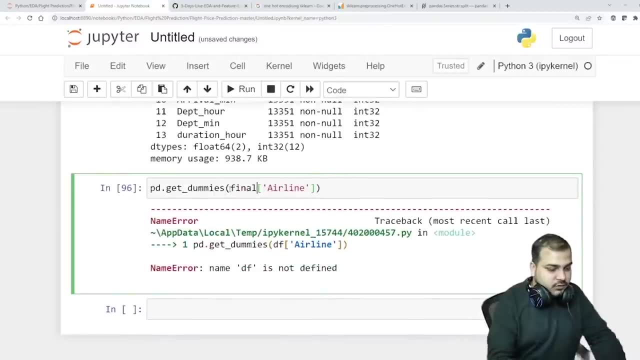 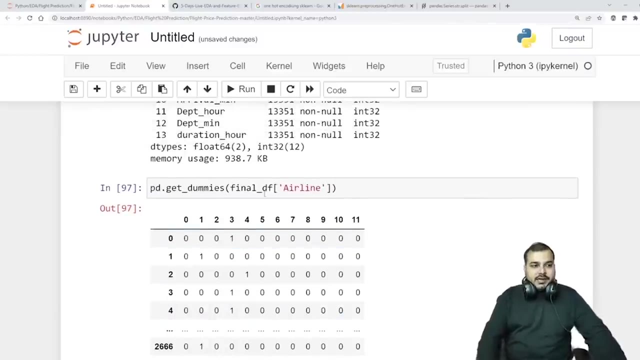 Sometimes syntax. it's very difficult to remember all the syntax- df of airline, final df. so let's go ahead and do this and then you will be able to get it. Try to create a different data frame. let's say this is df one. then I will create another data frame which is: